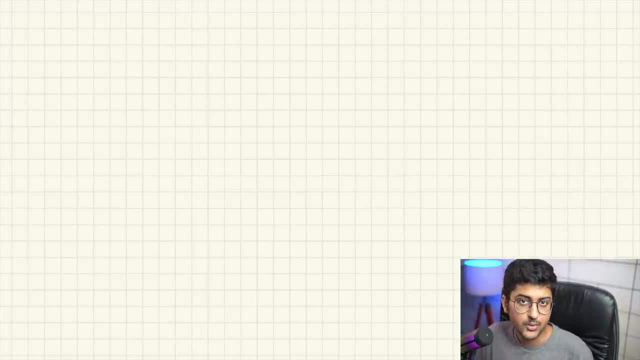 than happy. you know you can share about it in the links in the description, But once you watch this entire video you will know that there isn't So space and time complexity analysis in this section. one more thing I want to share is that this is the only video that you need. If you don't know. 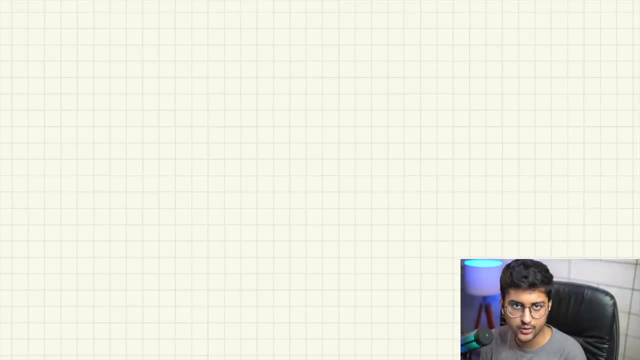 anything about space and time complexity. this is the only video you need to watch to go from beginners to advanced. It's going to be a really long video. We're going to cover everything in detail. So let's see what we are we are going to be covering and let's also see, like, how you can. 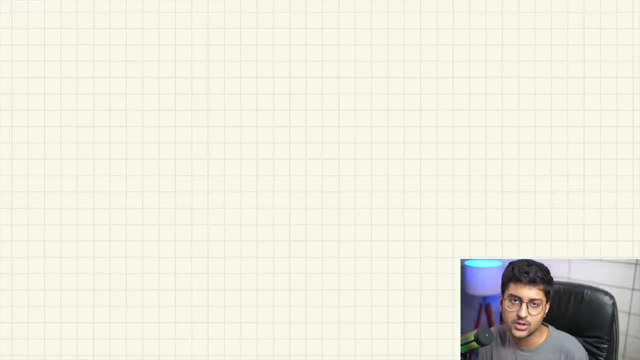 you know, get started. So, by the way, this is a video of the course that we are doing: the complete data science algorithms plus interview preparation course. You can check out the link in the description. There's an entire playlist. We are covering literally everything you need to clear your FANG interviews or whatever, and all these other coding rounds or 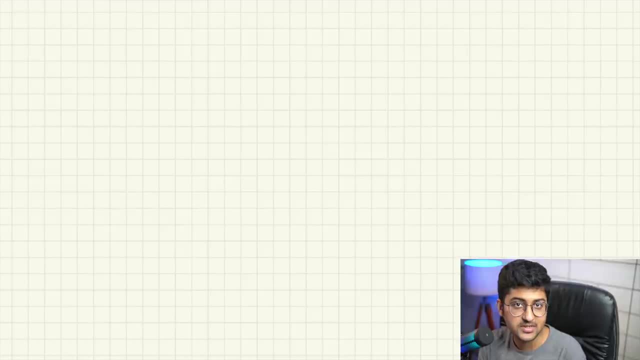 whatever, Make sure you check out the links in the description and please make sure you subscribe as well. So subscribe right now if you haven't already. It's really going to help the channel. But in this video we're going to look into- and so this is the agenda- We'll look at the introduction. 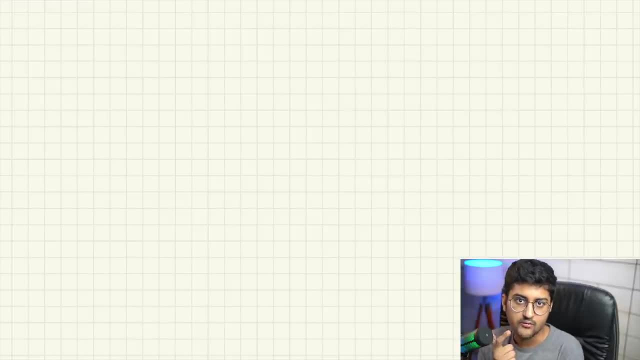 of space and time complexity. We'll compare various cases. We'll look at, you know, what is the big O notation, or whatever- big O, big omega, big theta notations? What is the mathematical aspect of it? What is the intuition behind it? What does it mean in words? We'll look into that. We'll look at how. 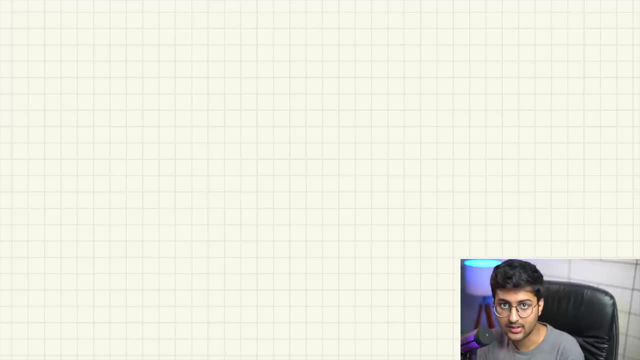 you can solve recurrence relations So linear recurrence divide and conquer recurrence. If you don't aware of this, we've already covered it. The link is in the description. We already covered it in the previous video of recursion. Already covered it in detail. Okay, we'll talk about this is the 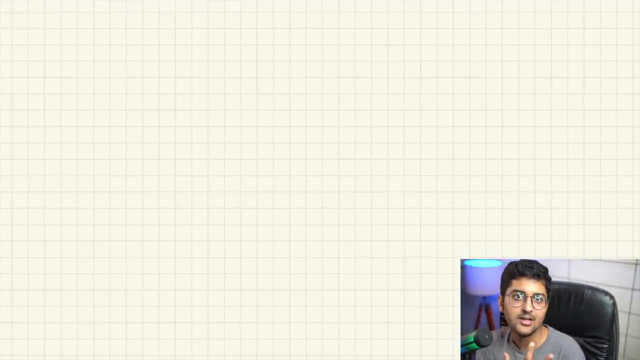 highlight of this video. actually, I'll teach you some amazing, magical methods via which you can get this Solving linear recurrence relation. we did in the previous video, Fibonacci number. You will be able to find the nth Fibonacci number is just one single step and I will actually teach you how to. 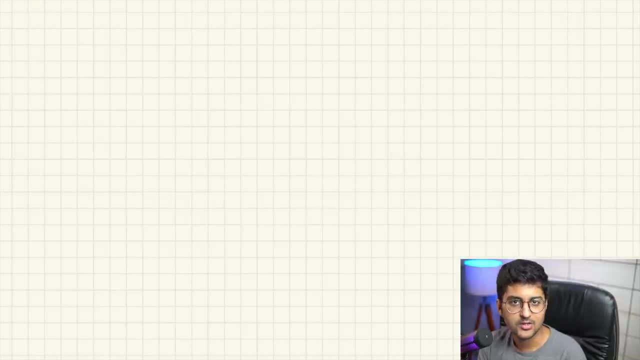 get that formula I will teach you in this video itself. We'll also learn about little notations. We'll also learn about, you know, get the equation in the equation of like the relation in the best and easy, easiest approach. We'll obviously, you know, discuss about the complexity of the problems. 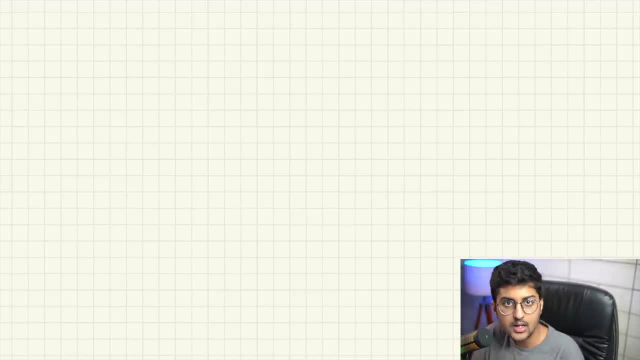 we have done and we already have discussed about it so far: after every problem We'll also look at space complexity, auxiliary space. We'll also look at some memory management things and memory allocation, how these things. you know we have already covered that, but we'll still. 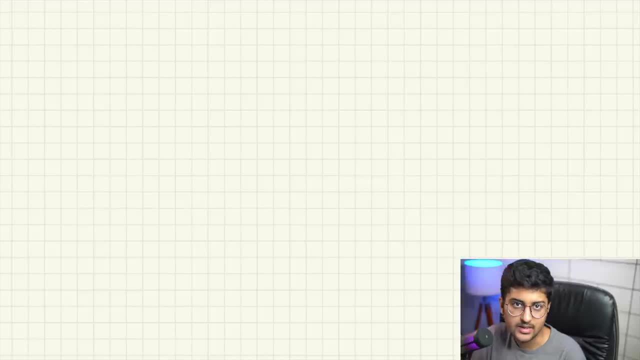 take a look into that. We'll also give you an introduction to NP completeness and hardness and what all these things are, and there's actually a million dollar price actually in reality. So to one who solves these problems- and we'll talk more about that later- It's going to be a 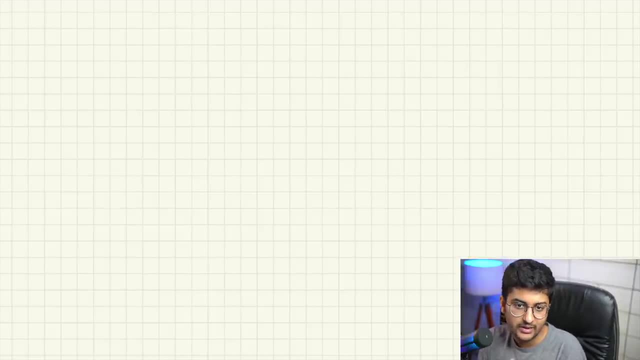 great lecture. Make sure you subscribe and like and, if you enjoy this video, please share with your friends on social. Join the hashtag DSA with Kunal Hashtag: 60 days of DSA Learning in public initiative where, if you share about the course that you are learning from my 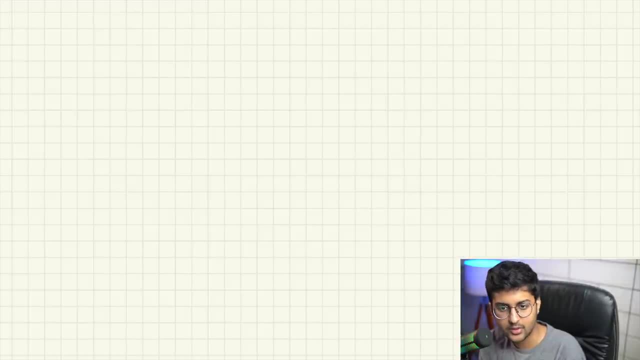 YouTube channel on socials. then other people will get notified about it and you can check out the assignments and everything. The links are in the description of the, all the code samples and the notes as well. Without further ado, let's get started. Before we get started, I just want to 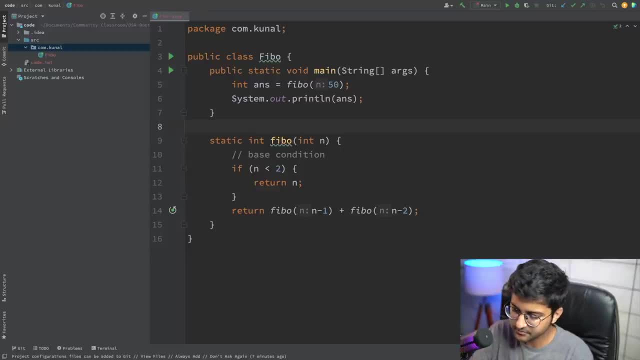 share that. let's say we have a problem like this online. okay, So this is the problem we did in the previous lecture. So if I try to find the 10th Fibonacci number, this is something we did in the previous lecture. very simple stuff. if you haven't watched that already, 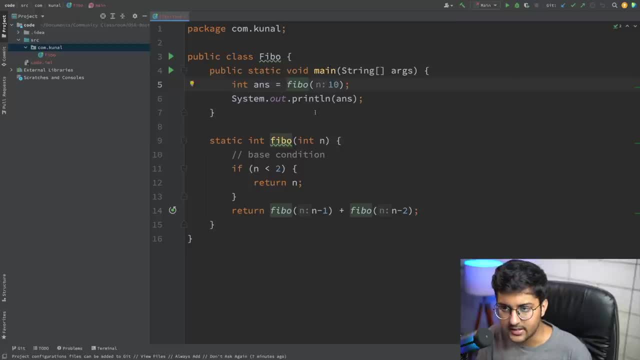 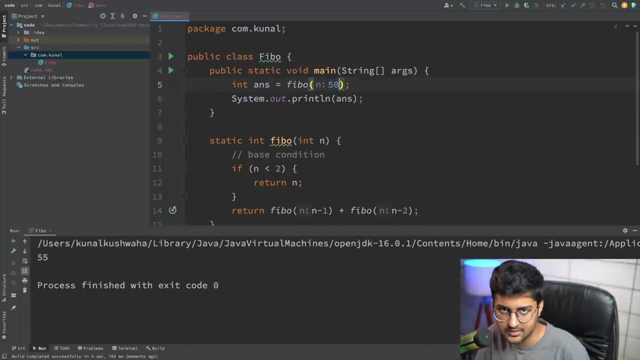 do so. so, as you can see, in the previous lecture we did finding the nth Fibonacci number. let's say we try to find the 10th Fibonacci number. let me run this. let me run this real quick. so it's giving 55. let's try to find the 50th Fibonacci number. 50 is a very small number in. 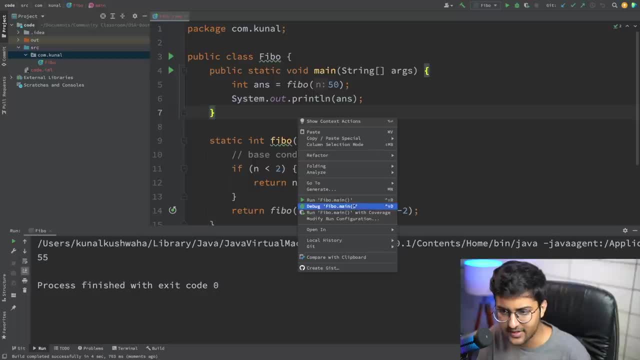 computer science. okay, depends on what you're doing. so let's say we find the 50th Fibonacci number. Fibonacci number can go like till infinite in that context, like 50 is nothing. let's run this. we tried to find the answer. it's not giving the answer. we covered this previously. this is exponential time complexity. 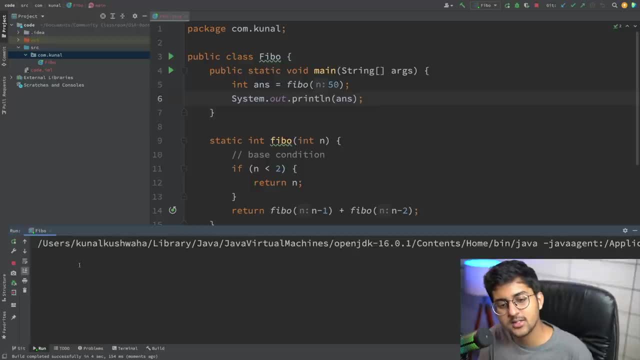 what is exponential time complexity? why is it not giving the answer, Kunal? why is the program still running? it's been so long it's still not giving the answer- been like 5-10 seconds. if you wait even more, it will not give the answer. why is it not giving the answer? we covered it already. 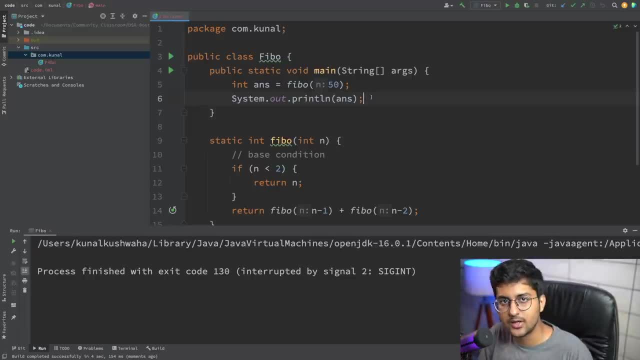 is actually re-evaluating the same things over and over again. so if you want to look into it, there's a lecture of recursion: introduction to recursion. the link is in the description. you can go to the lecture and in the lecture there's also a timestamp for fibonacci number. you can click on that and 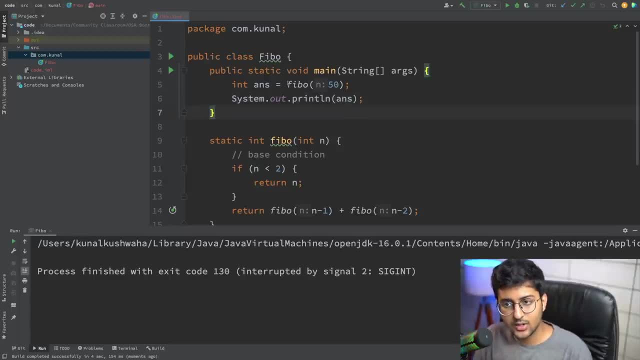 then you can see why it's not working. okay. so we'll talk more about this in detail. we'll talk about that recursion tree in detail. we'll talk about that, uh, how we are actually getting the complexity. what is actually, in reality, the complexity of this? it's 1.6, something raised. 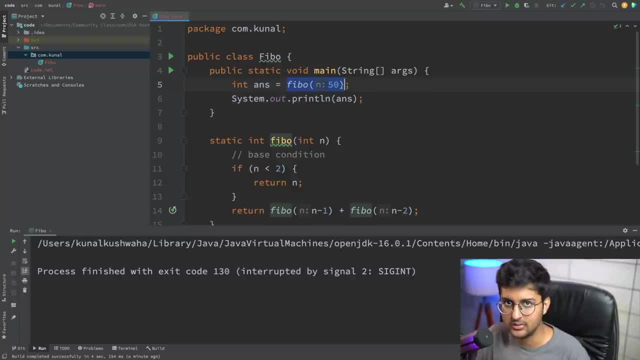 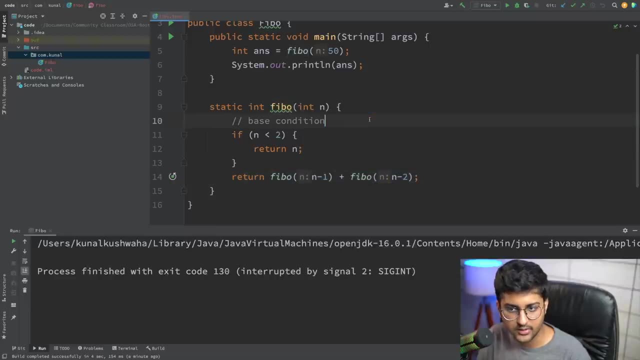 to power n. if someone says it's two raised to power n, they are wrong. it's not two raised to power n. okay, and then we'll also see how we can optimize this a little bit. and this is a recurrence relation. we already covered this previously, but we will actually now dive into 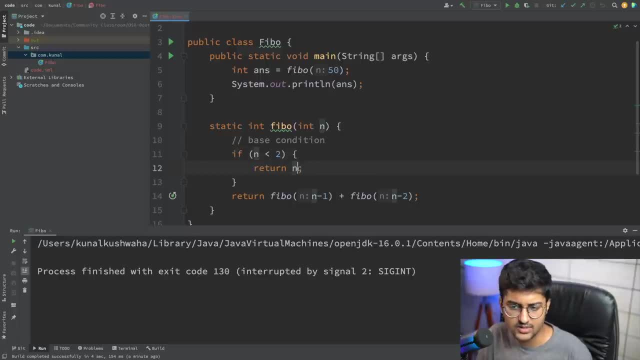 the details and even, like i'll cover it from the you know scratch as well, it's not nothing, nothing new, uh, it's uh. totally fine, i can do it again. so we'll look at the recurrence solution then. from this we are going to derive a formula, we're going to derive the time complexity of this. 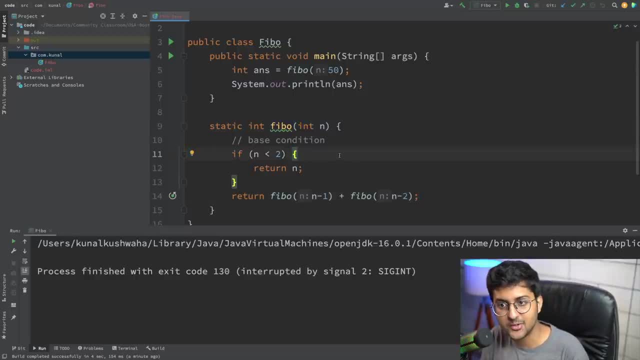 in a very easy manner. all right, so let's get started. make sure you follow the link in the description. if you have any questions, please feel free to ask them in the comments section below the notes. i'll be uploading the notes as well. there's going to be a lot of notes in this section. 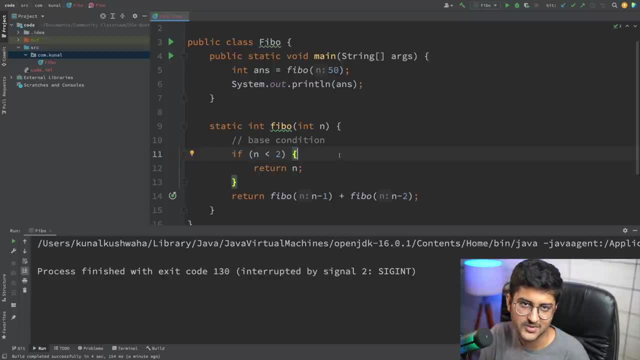 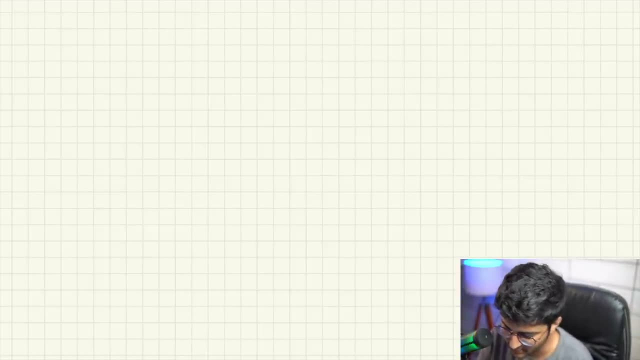 and it's going to be a really amazing, perfect section for you all to understand space and time complexity. let's start from the basics. so let's get started with the main topic first, which is: what is, uh, space and time complexity analysis? what do we mean by it? okay, let's talk about it. 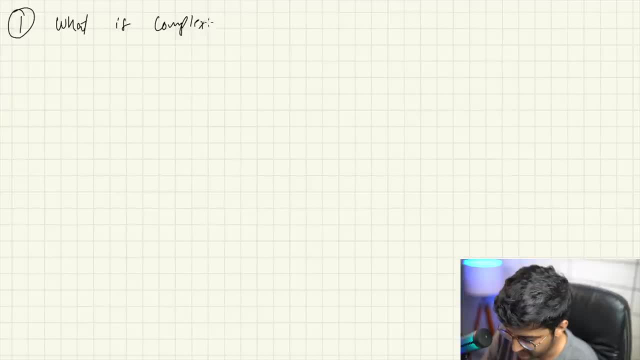 what is complexity? what do we mean by it? what is this thing? let's say, we're talking about time complexity right now. okay, so we can talk about time complexity and space complexity later on. okay, so let's talk about what is time complexity. before we answer this question about what is time complexity, let me ask you a question. let me ask you a question. 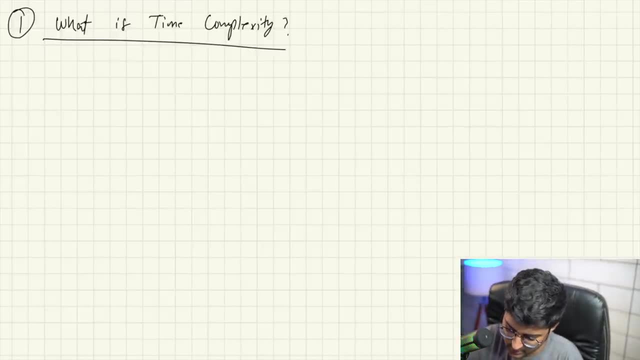 let's say i have two computers- okay, one is a really old computer- okay, old computer- and one computer i have is a brand new m1 macbook. m1 mac book, it's very fast, very fast. okay, we are starting from the basics. we are looking at what is time, complexity? 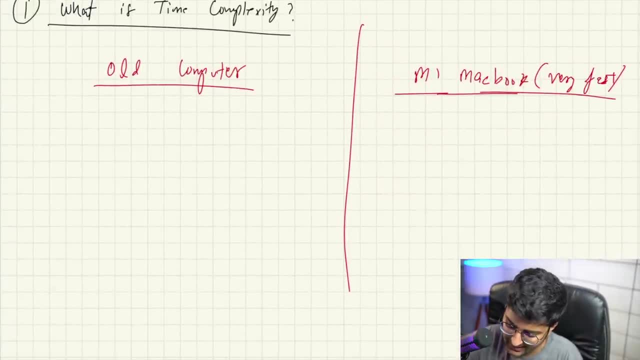 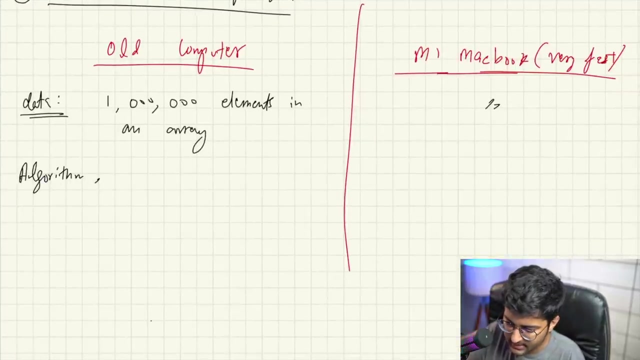 okay, so this is very fast. now i run an algorithm. i have a data. data is, let's say, one million elements in an array. this is same for this as well. okay, same data is available on the both machines, same everything. okay, one million elements. i run an algorithm. i run an algorithm, let's say, linear search. okay, i run the. 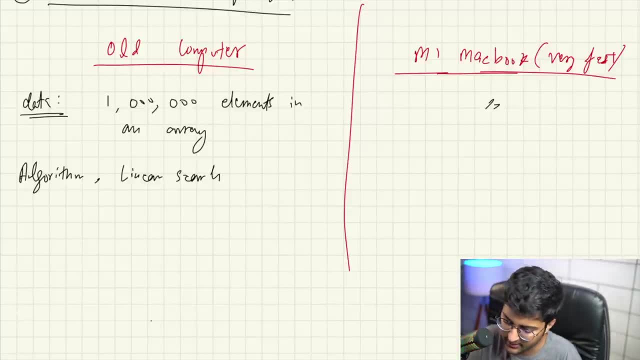 linear search algorithm. let's say on this total number of elements. let's say for the same target or whatever. for target for to search a number that does not exist in the array. okay, for target that does not exist in the array, i run linear search on this array. this array is same in both. i run this algorithm over here as. 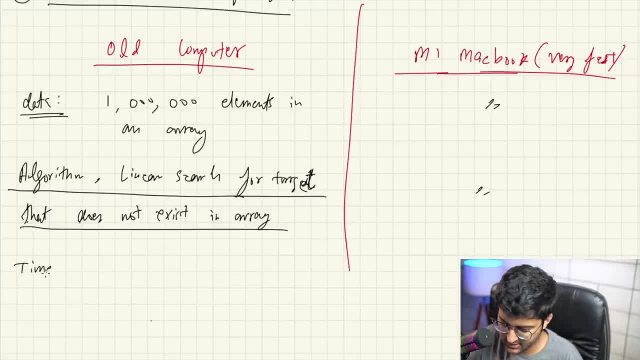 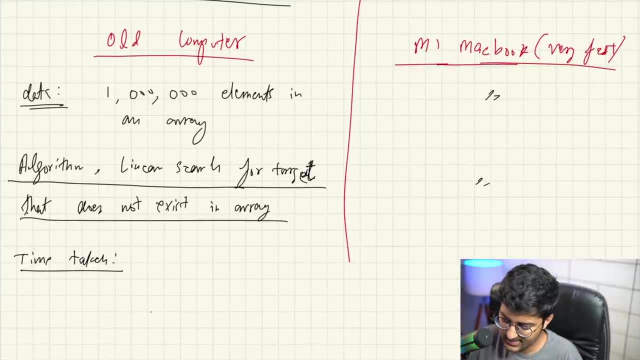 well, on the same time taken to finish algorithm. okay, let's say the time taken to finish the algorithm on the older machine is, let's say, 10 seconds. let's say the time taken for the same date for the same algorithm on the macbook is, let's say, equal to one second. 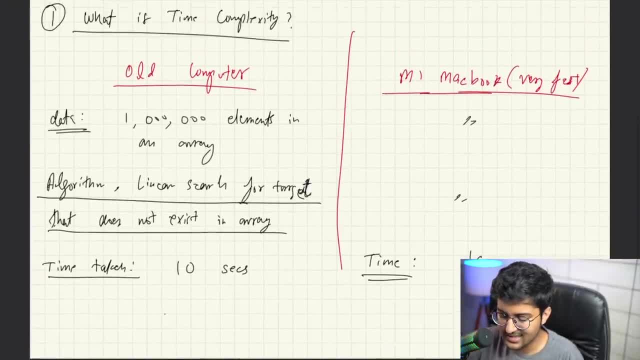 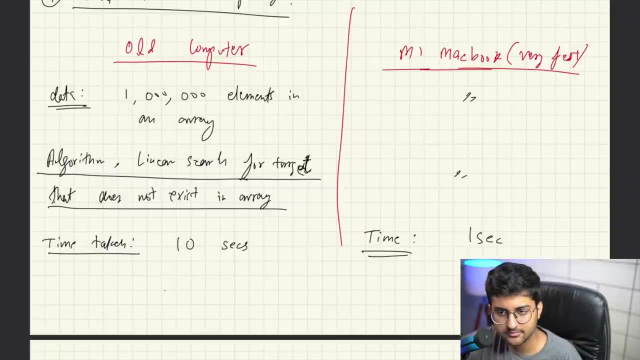 okay. so my question to you is: which machine has a better time complexity? is it the old computer or the new computer? pause this video. think about it, okay. if you said the old computer, you are wrong. if you said m1 macbook, you are wrong. the correct answer is both of these. 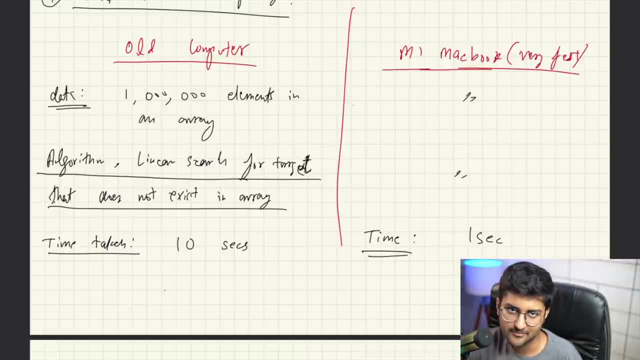 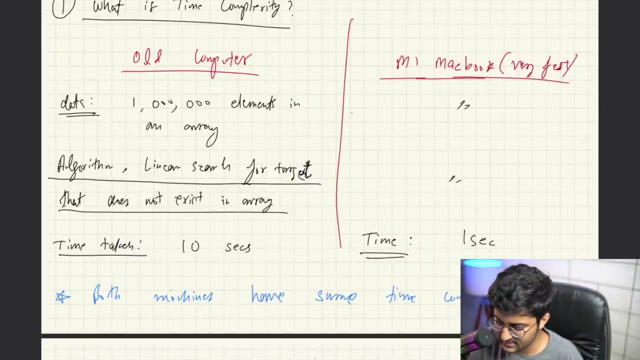 machines have the same time complexity. okay, so both machines have same time complexity. now you will be confused. you'll be like kunal. what do you mean? they have the same time complexity. macbook is taking less time because it's very fast. old computer is taking more time because it's very 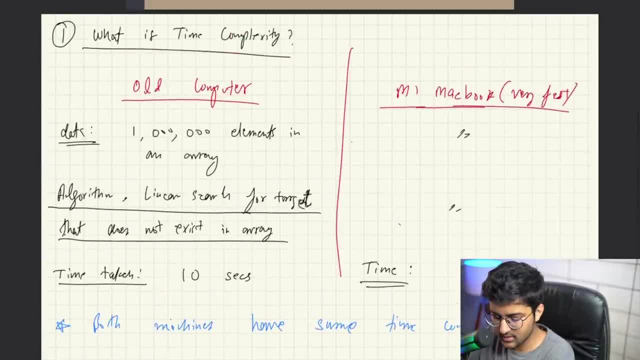 you know slow old computer. so how come these machines have the same time complexity? because it's very fast old computer is taking more time because it's very. you know slow old computer. so how come these machines have the same time complexity? so how come the time complexity is same for both of these? 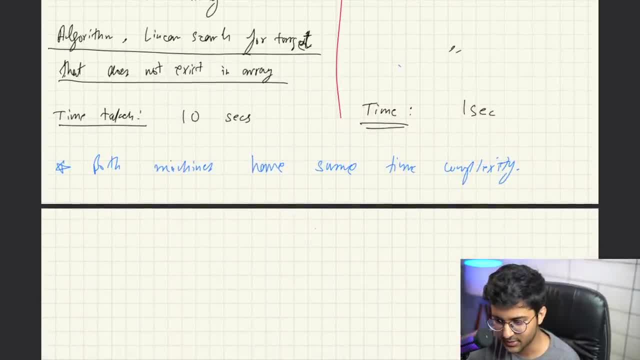 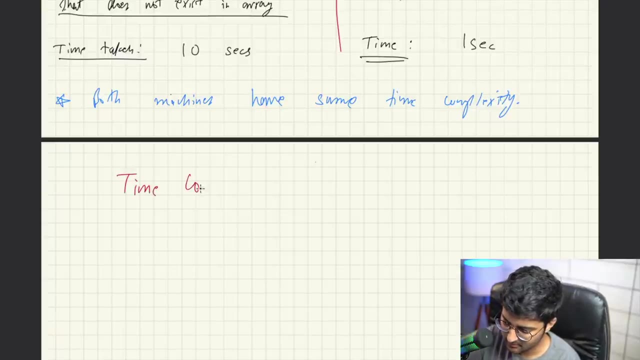 what conclusion do we get from this? you tell me. i mean, how can you tell me? um, you think about it. what conclusion do we get from this statement? so the conclusion that we get is time complexity. time complexity is not equal to time taken. you may have heard this many times: the time complexity is equal to total amount of time. 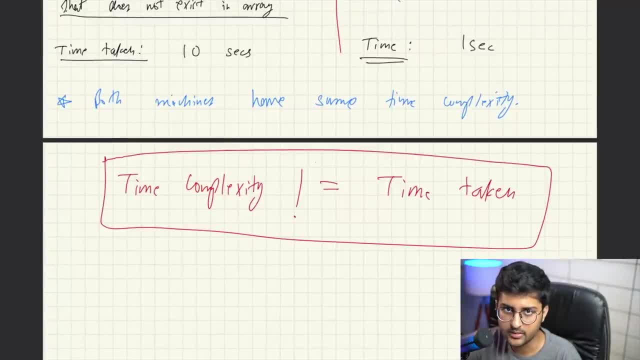 taken to run the program. that is incorrect. it's a wrong statement. time complexity is not equal to time taken, understood, okay. now you may ask: well then what is time complexity? if it's not the time taken, then what is time complexity? okay, let's say we take the same example of old machine and new. 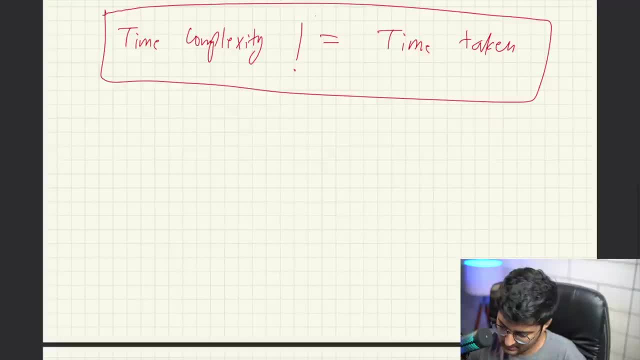 machine, old machine and new machine. so, if i take the example of old machine and new machine, again old machine and m1 macbook. yeah, so let's say i create a graph. this is actually the size of array, this is actually the time taken. this is actually, let's say, the size of array. this is the time taken. 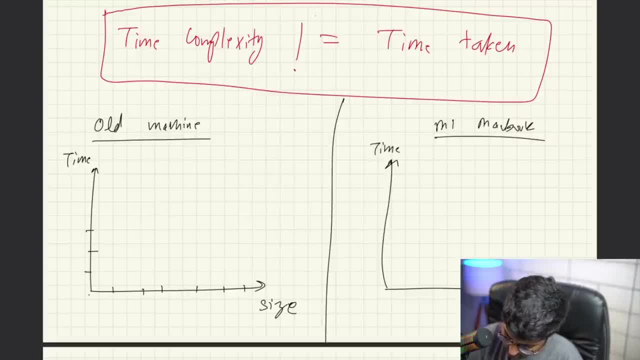 okay. so let's say that for the size of the array, let's say we have 10, 100, 200, 5000, 10, 000 or something. okay, and 100, 200, 5000 and ten thousand. okay, that is the size of the arrays. let's say for 10: size of the array, it's taking somewhere. 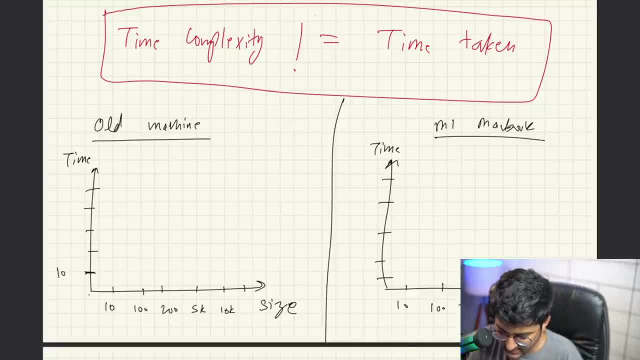 around, let's say, 10 seconds. let's say, for 100 size of the array, it's taking somewhere around 100 seconds. let's say, for 200 size of the array, it's taking around 200 seconds to run the same algorithm. okay, five, uh, five thousand size of the array. let's say it's taking something like 5.1. 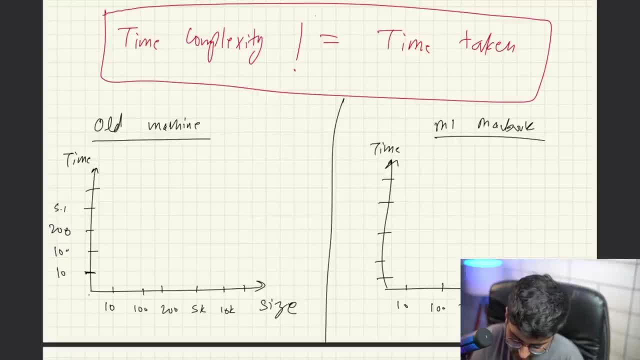 seconds or something. okay, no problem, 5.1 thousand seconds. 5.1 thousand seconds for 100k, for 10k. it's taking, let's say, let's say something like 9k seconds or something, so it can vary. can you all see that when i plot a graph like this? oops. 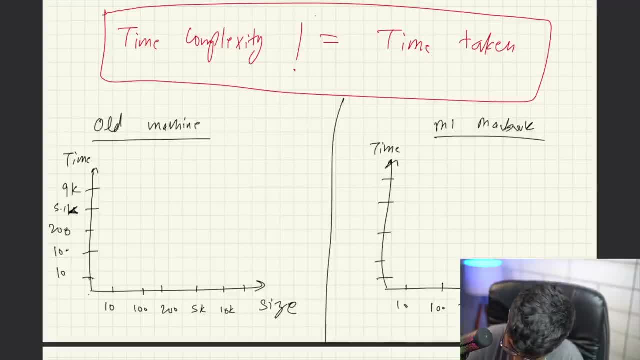 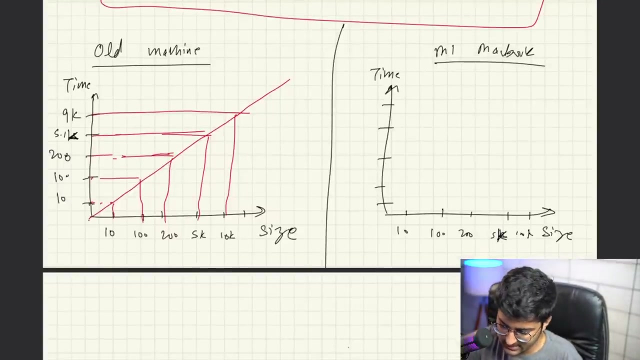 can you see that if i plot a graph like this, if i plot a graph of the time taken and the size, can you see that it's sort of like a straight line. can you all see this for the same data? if i run the same algorithm, let's say for 10, it takes 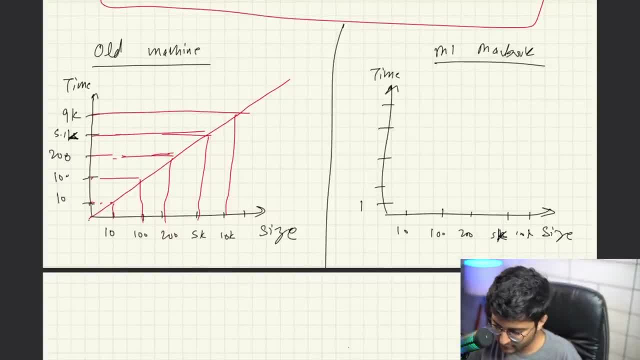 around. let's say: you know, one second for 100, it takes around. let's say 10 seconds for 200, it takes around 20 seconds, or 90 seconds, or 100, it takes around 20 seconds or 90 seconds or 90 seconds seconds or whatever. let's say 19 seconds for 5000 it takes. let's say 500 seconds, 10 000 it let's. 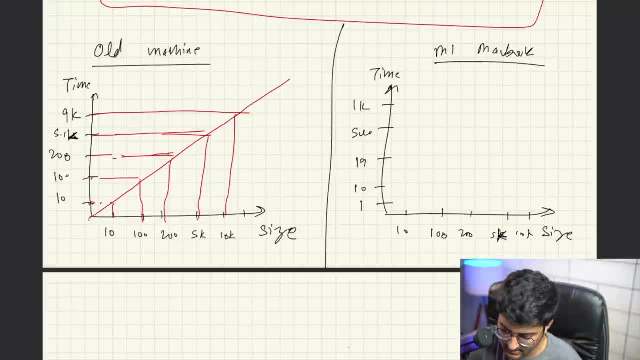 say it takes 1000 seconds or something like that. can you see that if i plot a graph for this as well, this will also be a line, but it will be like a little bit steeper line with less slope. with less slope, okay, because i have 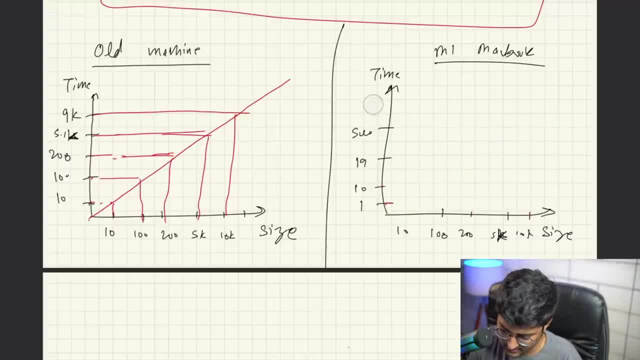 9k over here and 1k over here, so no problem, i can do it something like this. if i am doing the same, you know something like this. i can say: this is, let's say, if this is 10, um, this is like, let's say: 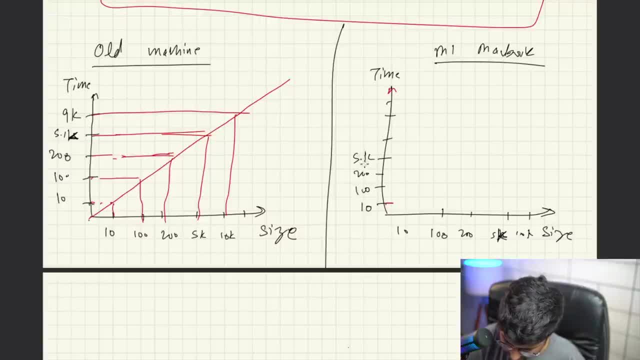 100, 200, 5.1 000 or 9 000 or whatever. 10 takes one second. it will be somewhere over here. 100 takes 10 seconds. it will be somewhere over. 10 takes 10 seconds. it will be somewhere over. 10 takes 10 seconds. it will be somewhere over. 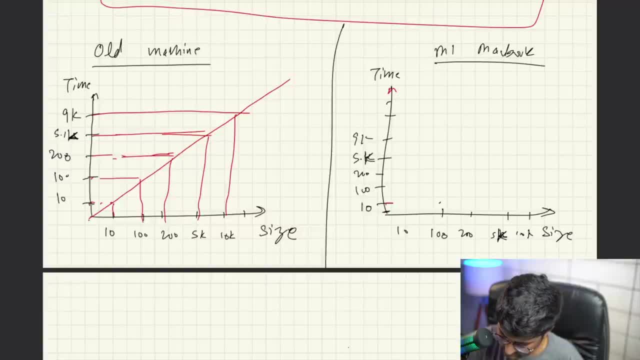 here, 200 takes 20 seconds. it will be somewhere, let's say, over here. this 5000 takes 500 seconds. it will be somewhere over, like here and then here and here. this is also sort of like a straight line, as you can see, but the slope is reduced. can you see that? 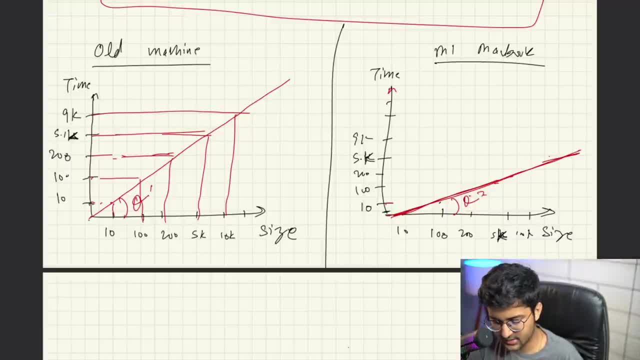 can you see? the slope is reduced. this theta angle is smaller than this one. okay, so, even though the time taken is different, but the relationship between the size and the time is same, linear. if i give you a question, what if you had, let's say, over here you had twenty thousand size? can you give an estimate of the amount of size? amount of 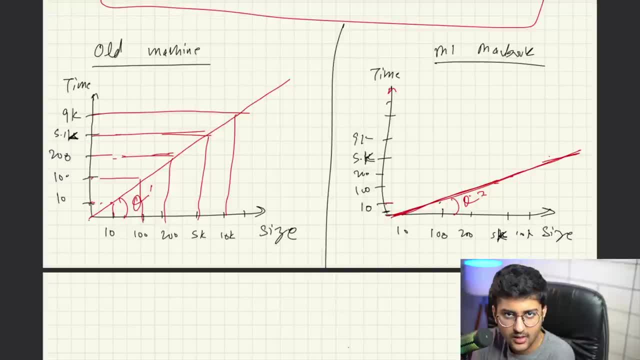 time that will be taken in this case, if the size was twenty thousand, around twenty thousand seconds. if the size here was twenty thousand, same algorithm then from this machine will take around two thousand seconds. you are able to give an estimate right with common sense, how, by looking at this graph, you know this graph is going in a straight 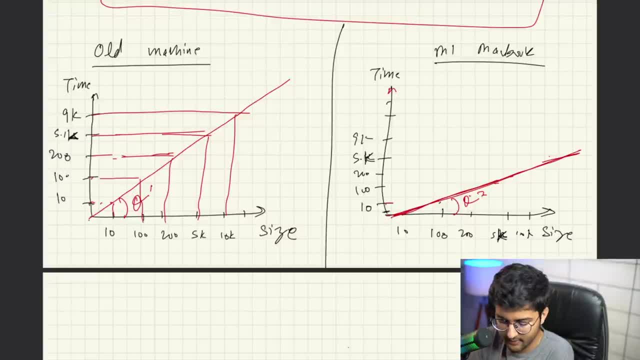 line and all the future points will also lie in the straight line. one lakh size of the array will take around one lakh seconds. one lakh size of the array over here will take around ten thousand seconds. you are able to give this estimate. how? how are you able to give this estimate? 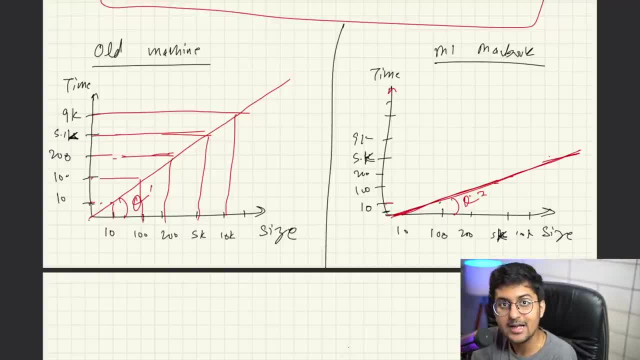 because of this graph. so what is time complexity? time complexity is this graph. time complexity is this mathematical function. this mathematical function is known as time complexity. so what is time complexity? it is a function that tells us how the the time is going to grow as the input grows. that is time complexity over here. 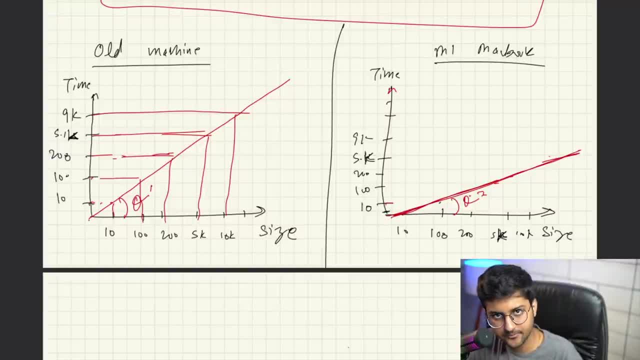 time is growing linearly as the size is growing. okay, over here also, time is growing linearly as the size is growing. in both the cases it's growing linearly. value may be different, but it is growing linearly. right, y is equal to x, y is equal to k, some constant into x. that's the simple graph of. 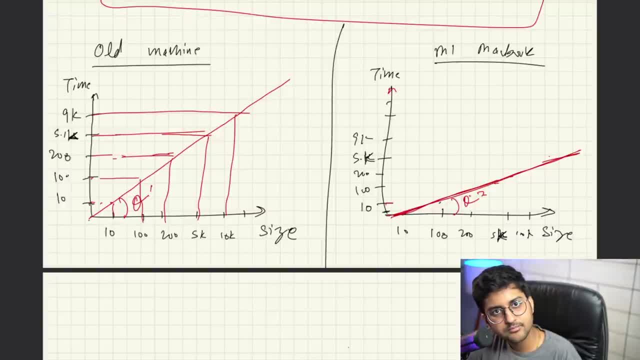 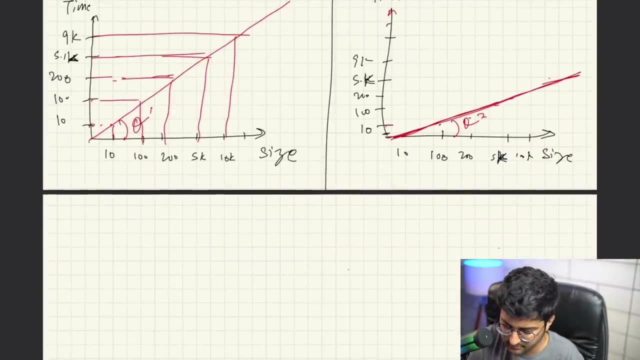 this size is equal to some k times time- as simple as that, linear. this is known as time complexity. time complexity is what time complexity gives us. so it's not. it does not give us the time complexity. it's actually a function that gives us the relationship about how the time will grow. 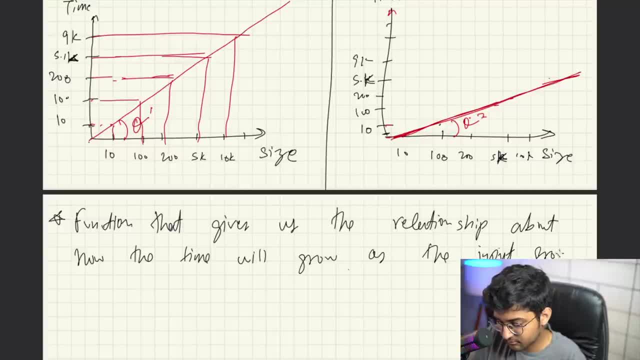 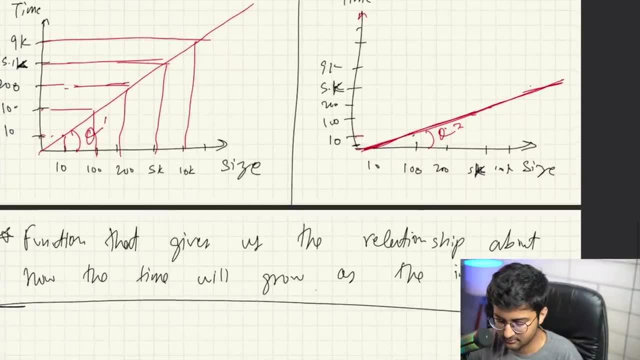 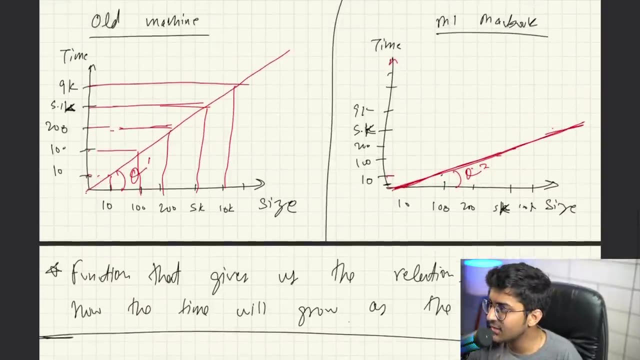 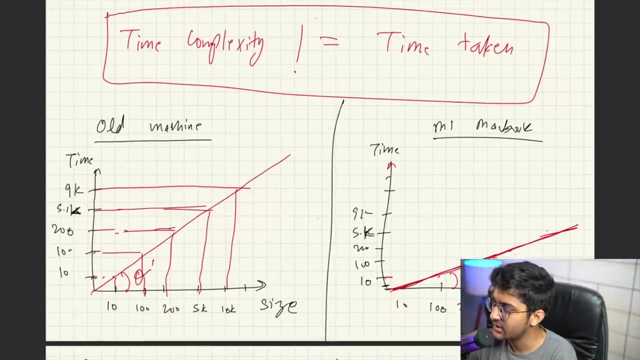 as the input grows. okay, this is the time complexity as simple as that. cool, very simple stuff we represent these into, like big o notations and stuff which we'll look into here, like right now. okay, so in short, this was the answer. so, if anyone says time complexity, 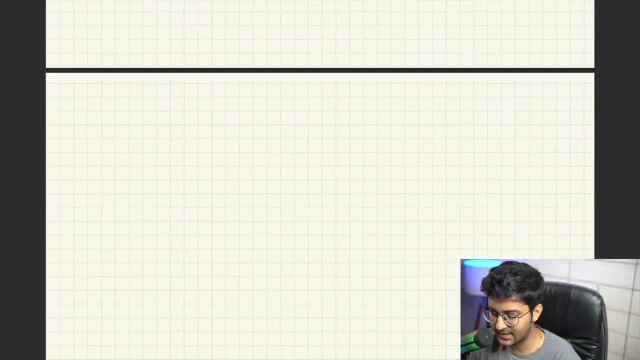 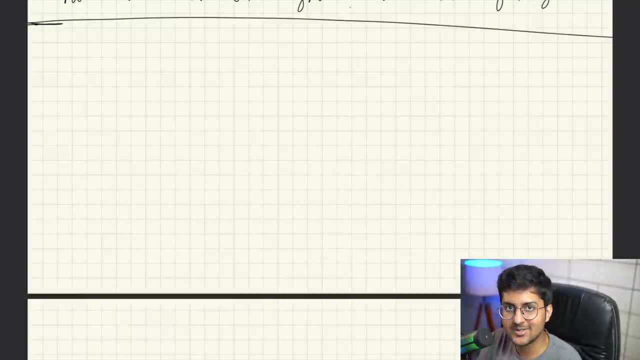 is equal to time taken to run the algorithm. that is incorrect. it's not the time taken to run the algorithm. it's actually the relationship between how your time will grow as your size will grow. now let's see why this relationship is important. okay, why do we care? 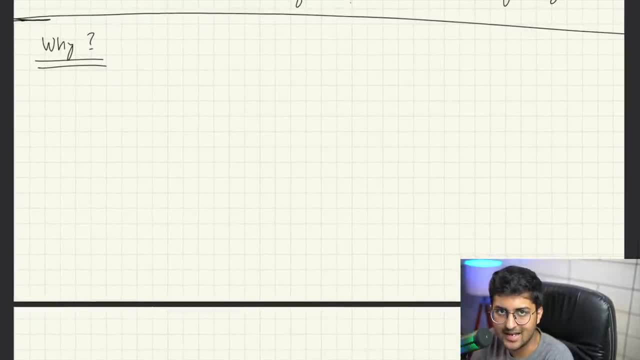 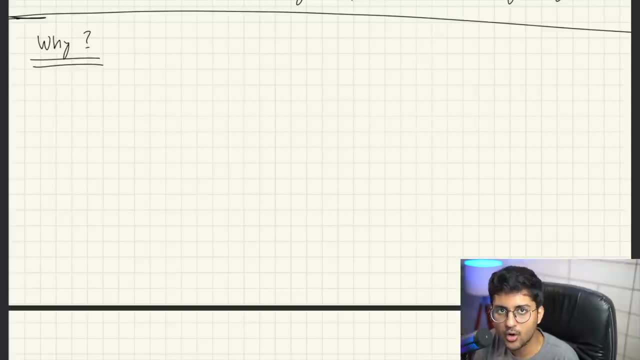 let's talk about the two complexities of this most simple algorithms that we've already done. so we know that binary search has a complexity of log n and linear search has a complexity of o of n, the worst case complexity. we'll discuss about that as well. we'll actually derive this. 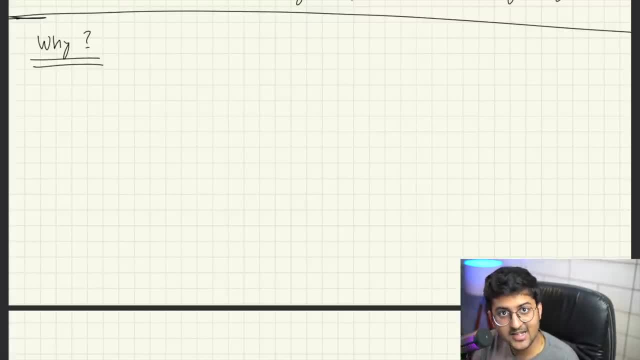 as well. i'll talk to you. i'll talk to you about what is big o notation, and in this lecture also, i will teach you why do we ignore less dominating terms, why do we ignore constants or whatever. i will teach you right now and we'll talk about that in the next lecture. bye, bye. 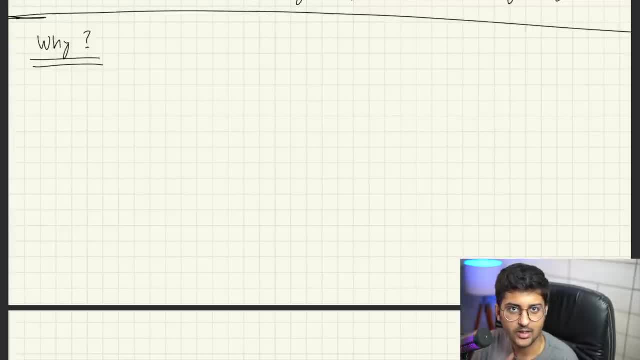 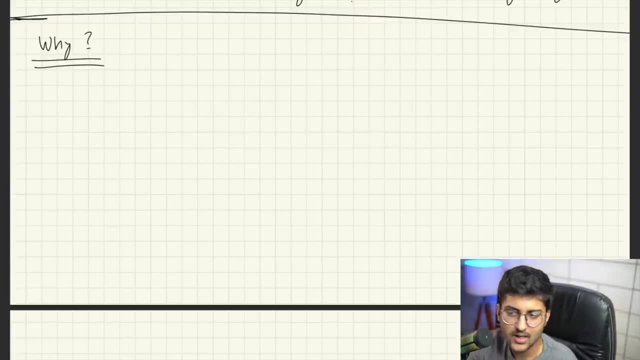 do we actually take the worst case? i will teach you that right now as well. okay, but so far we have discussed that uh linear search grows uh linearly like uh which n and um binary search grows with log n. what do we mean by that? okay, let's look into that. so let's say, i have something like this: 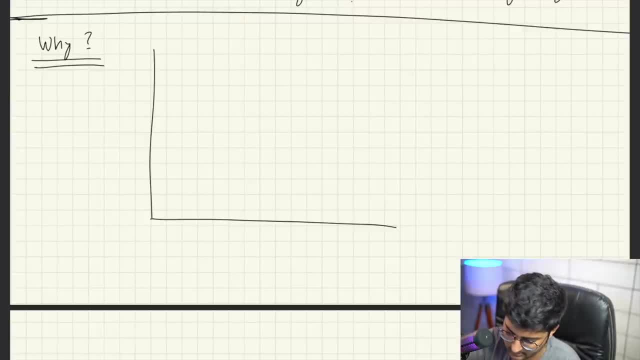 okay, this is a graph. let's say, i draw this for, uh, something like linear search. let's say, i draw a simple linear search like this: this is the graph for linear search because it grew the time. complexity is linear. we have discussed this already in the previous lectures. if you haven't already check out the linear search lecture. 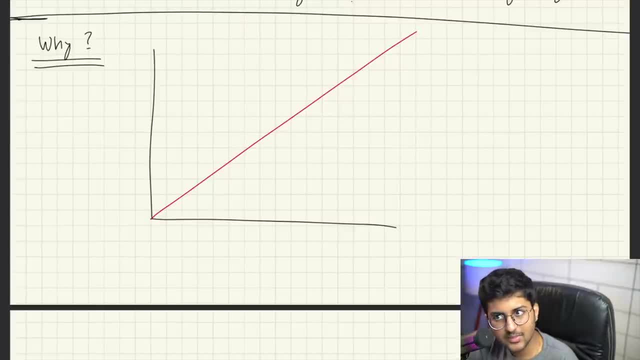 and over there in the thumbnail you can find the timestamp, you can find the complexity analysis. okay, binary search is what binary search is- login. so login graph can look something like this: login graph can look something like this: let me just change the color- something like this: okay, if i draw it much more like, let's say, crossword. 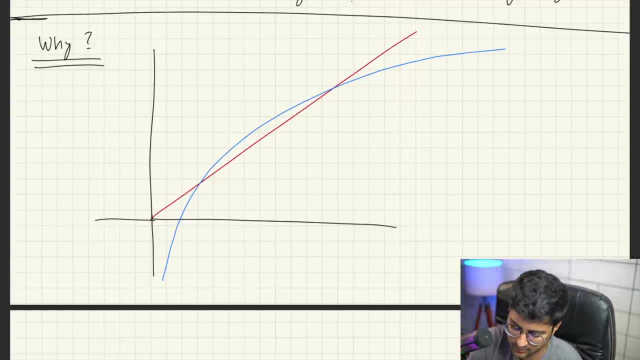 this is a log graph. okay, log graph can look something like this and you have over here your size. this is your time. now notice something. why does it matter? okay, this is login. this is n. don't worry about bigger notation. we will cover what is bigger notation later on. 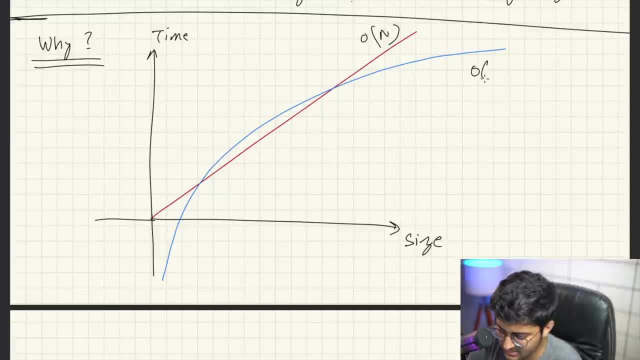 so far. you know, it's very common sense that this is growing linearly and this is growing in login times. can you see that if i fix the size, if i fix the size for larger numbers, if i fix this, if i fix the size for larger numbers, it may go, like you know, above and beyond. it's going very. 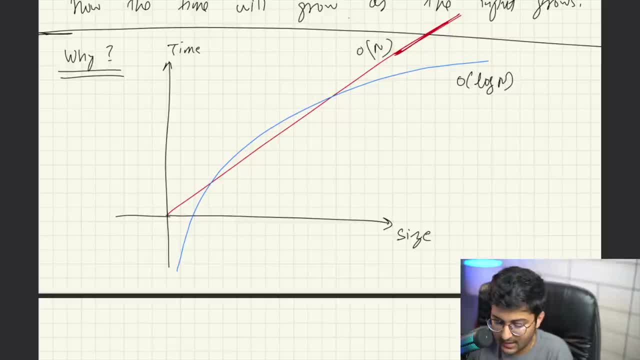 nicely over here. okay, for larger numbers, if i fix the size like this, okay, if i fix the size, can you see that? can you see that the time taken by linear search is actually greater than the time taken by binary search? can you see that, okay, okay, so that is why, for larger numbers, if i take, like somewhere over here, as you can see, if i take, 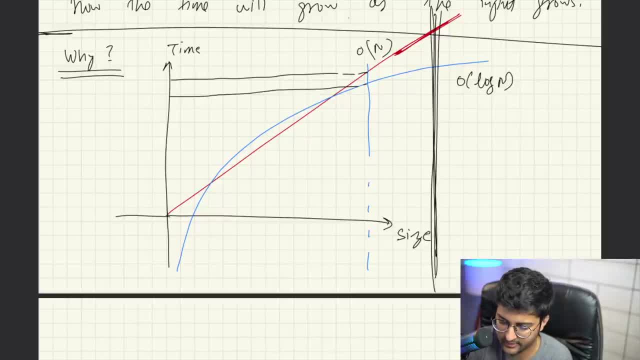 somewhere over here like this for the same size of array. so this is like the size is fixed. you can see the difference is increased. now this difference is increased. this means for the same size, this log n complexity will take less time and linear will take more time. very simple stuff. 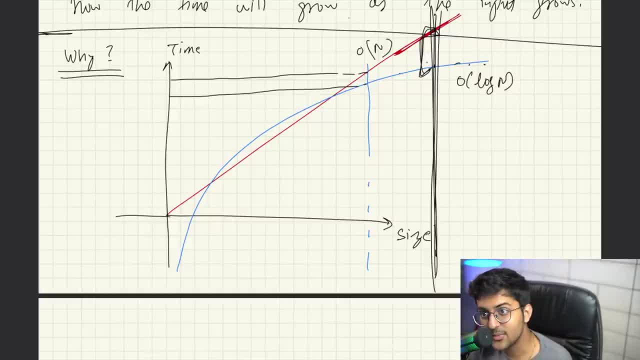 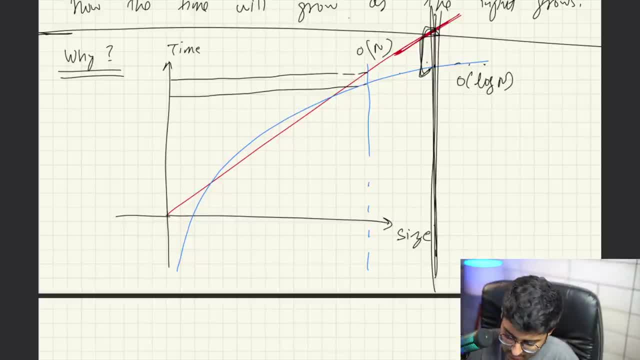 this is why we care. let's say we take. this is why we care. let's say we take about. let's say we take a constant time about. let's say we take a constant time about. let's say we take a constant time. complexity, complexity, complexity, constant time. complexity can be like just 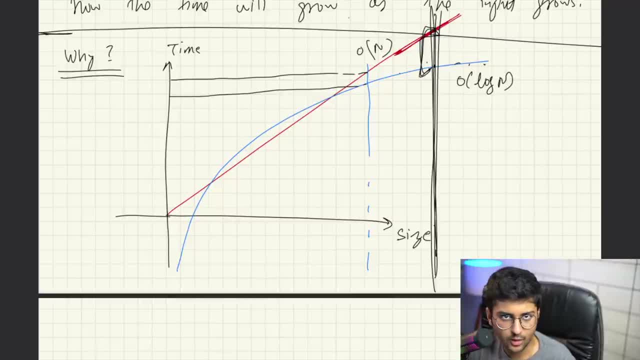 constant time. complexity can be like just constant time. complexity can be like just constant means. does not matter what the constant means, does not matter what the constant means, does not matter what the size is. time will always remain constant. size is time will always remain constant. size is time will always remain constant. something like this: 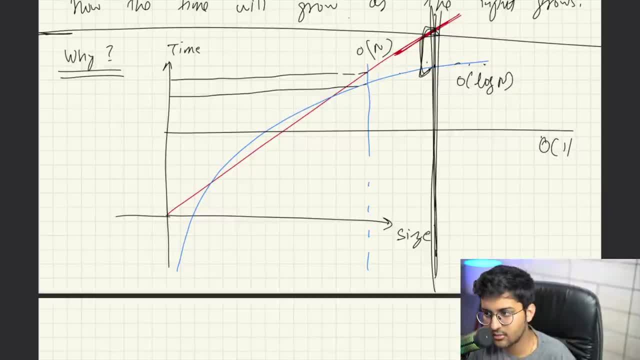 something like this: let's talk constant time, complexity. we go off one constant now, even though for smaller number, let's say it's taking more for, for let's say smaller, for smaller size, let's say over here. let's say log n is taking more time, uh, linear is taking less time, constant is taking the most time. okay, but the point to be noticed. 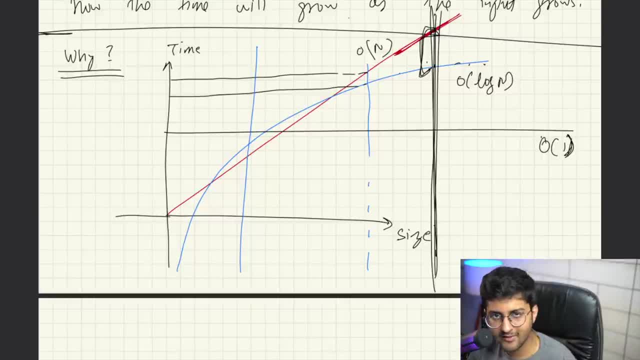 is we don't care about small numbers. why we don't care about small numbers we'll talk about later on in time complexity. always look at bigger numbers. always think about when your data will grow large in size in that case. what will happen in that case? over here we can see, even if i try to you. 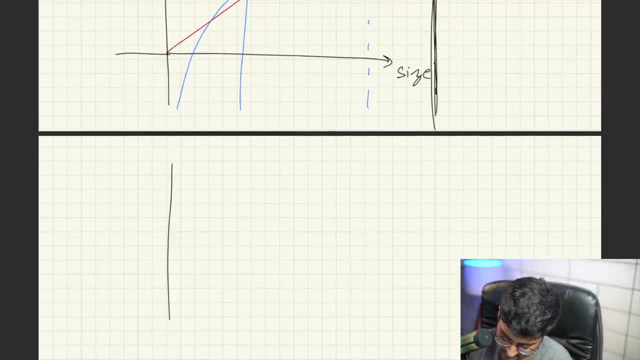 know, explain it even much more, in a better way, in a neat way. this is, let's say, like this: then i have a linear complexity like this, then i have my log complexity like this: okay, so now if you create a, now if you create the graph, okay. 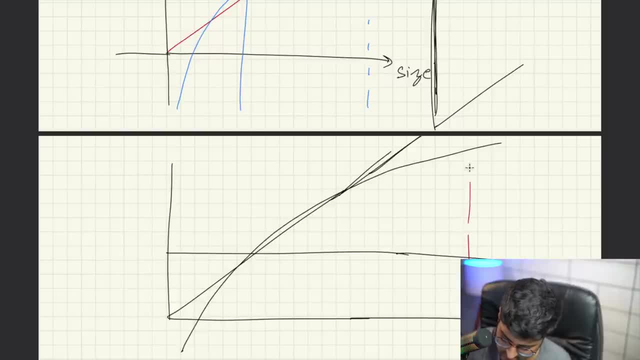 something like this: create the fix, the size, fix the size. you can see linear is taking the most time. then log n, then constant. so constant is obviously better than log n. i actually, like you might be confused with, like: is it greater than or is it not? so, complexity wise, which one? 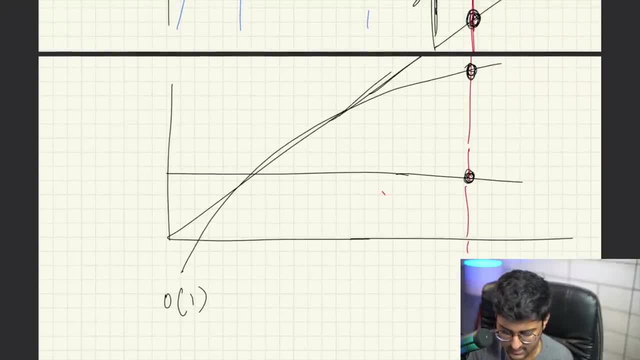 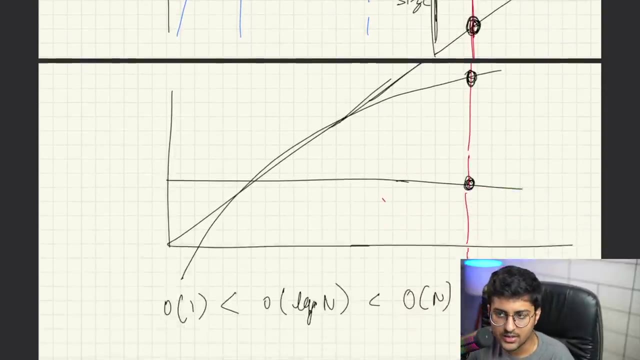 is the smallest, like smallest time taken, constant. then log in. then and what is the big o notation and everything i'll talk more about later on. so i hope you are able to understand why we care about complexities right now with this graph, as you can see, when the size i fixed for the same amount of data, n, was taking the most time, then log. 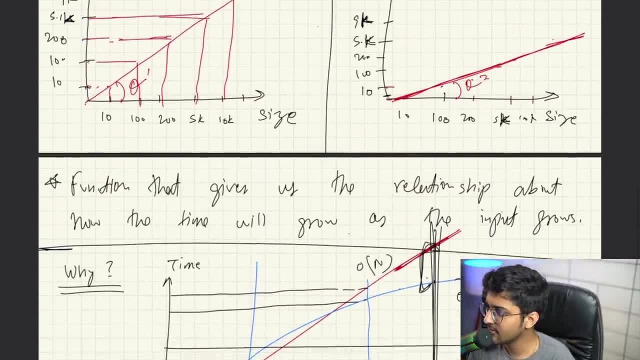 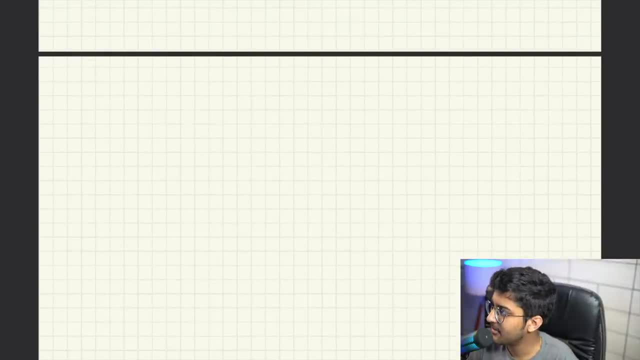 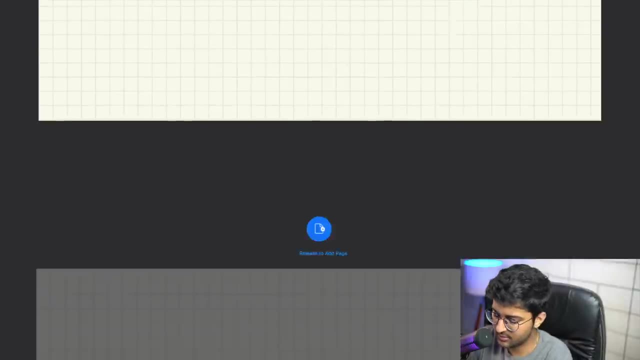 in, then one means constant time. okay, so that was the example of linear search versus binary search, hence, which one is better? binary search is better, binary search is better. all right, cool, so let's talk about the most more important part. what do we need to consider when speaking about complexity analysis? okay, 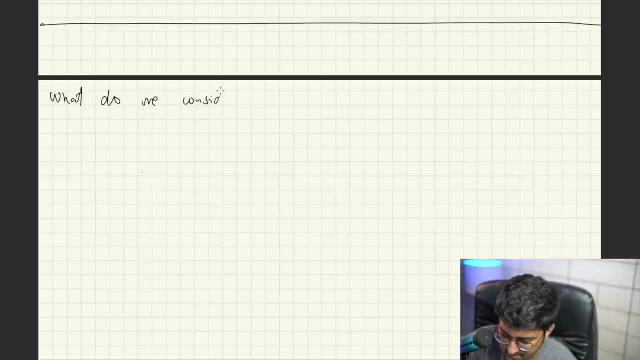 so what do we consider when thinking about complexity? what do we actually need to consider when thinking about complexity- and this is very important, because i will literally show you this a proof of this as well- in mathematics. whatever thing we are assuming right now, i will show you a proof in mathematics. 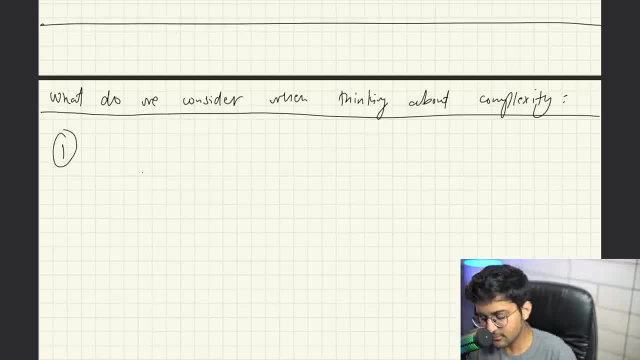 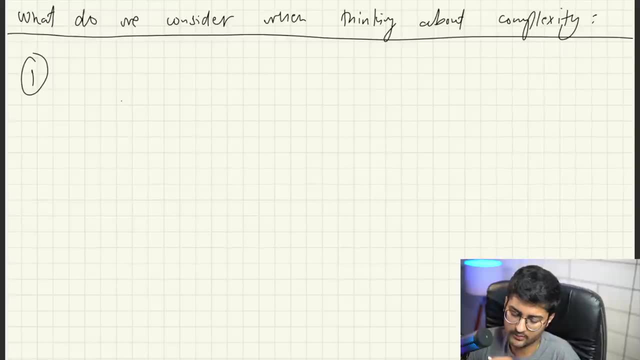 also point number one. point number one: i'll try to explain all of these examples with common sense. uh, common sense, common sense example. how can we give a common sense example over here? um, okay, let's say you have your application running. let's say you have your application running, your website. 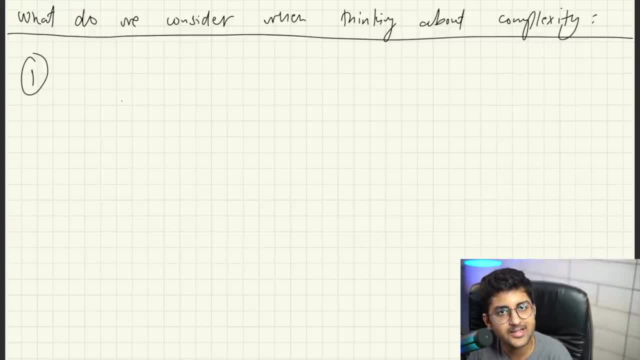 is running okay. it's a very common sense example. so your website is running. 10 users are using your application. is that more worry of concern for your infrastructure and your code optimization or is the worry about uh, what if 2 million people start using your application? 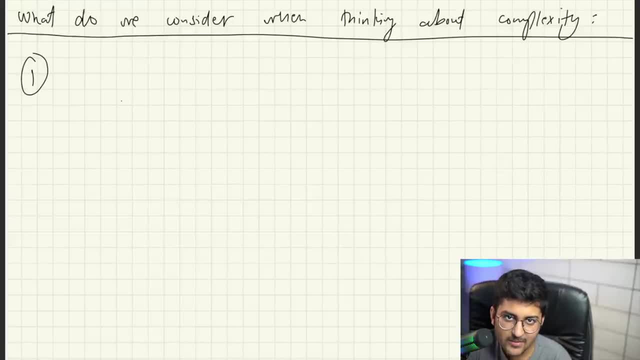 which has higher chance of crashing your website? 10 people using your application, or 2 million? say it with me: 2 million, that is my worst case. okay. so when thinking about time complexity, what do you need to look at? always look at the worst case: time complexity. so, with this common sense example, are you able to? 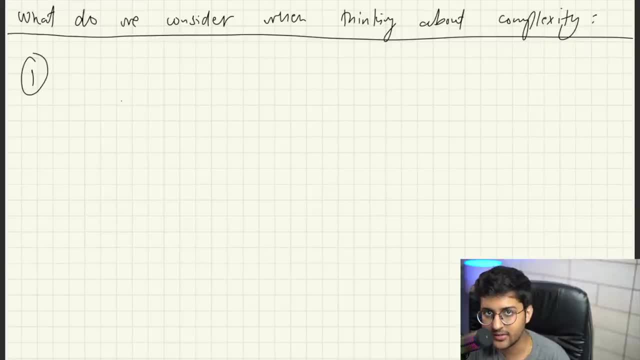 understand why we are actually taking about the worst case example, the worst case complexity. are you able to understand that? i think so. so always look for worst case complexity when designing your algorithms is what i'm trying to say. always look for worst case complex. definitely, you can optimize your best case as well. 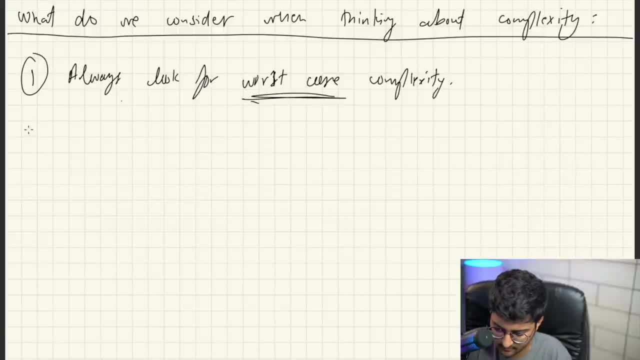 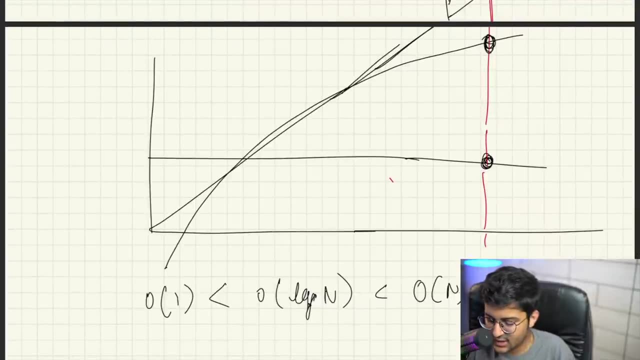 but the point of concern over here is worst case complexities. okay, let's say for size of the array 0 to 100. what to? how do i undo this? never mind important, and you will the idea. okay, you get the idea. so let's say for size of the array um one, two. 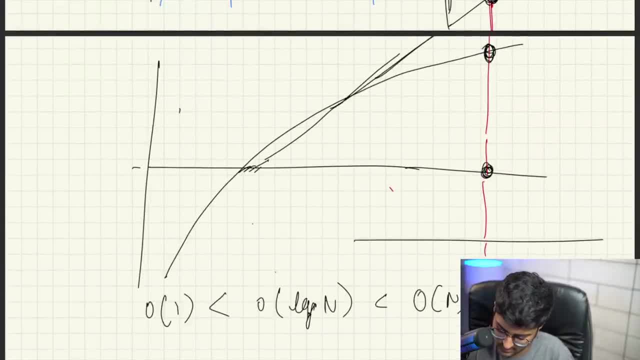 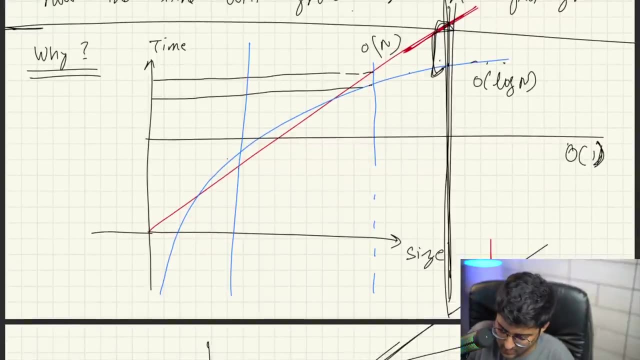 let me just fix this thing real quick. okay, that looks good, let's say for size of the array. let's say around in this house. only this was. this is a nice example. so in this case, you can see that, in this particular case, if there is some number of others known by many others, of course, on that particular case, this type of number is 10. 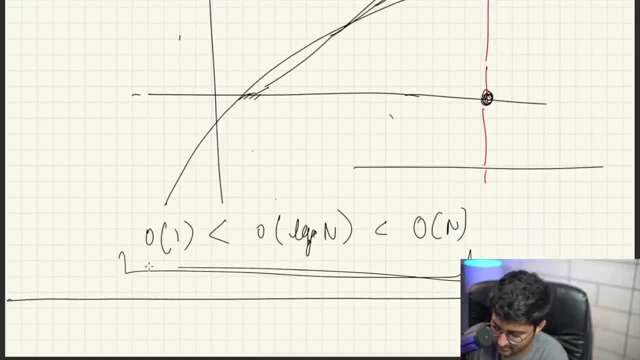 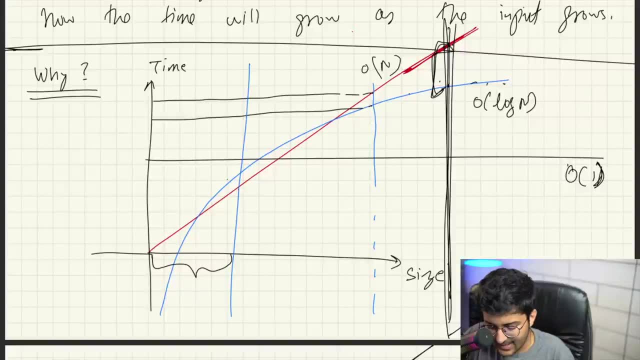 point. this is not really holding true. you're like Kunal. you said constant takes the less amount of time, but when the array size is just starting, constant is actually taking the most amount of time, Kunal. and then log n and then n. I'm like, yeah, you are correct, that might be possible, but for small amount of data. 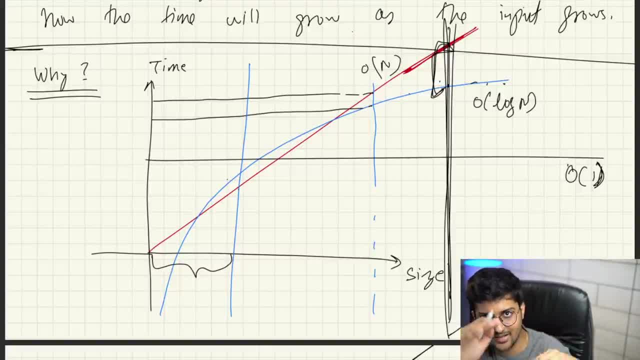 you know that even though relatively it will be taking more time, less time, randomly or whatever, overall the entire time for all the ones will be small because the data is small. can you all understand that? but the trend that we try to see, the trend that will not change, will be after this particular 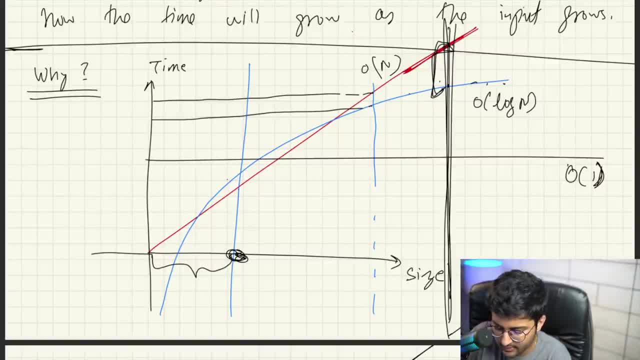 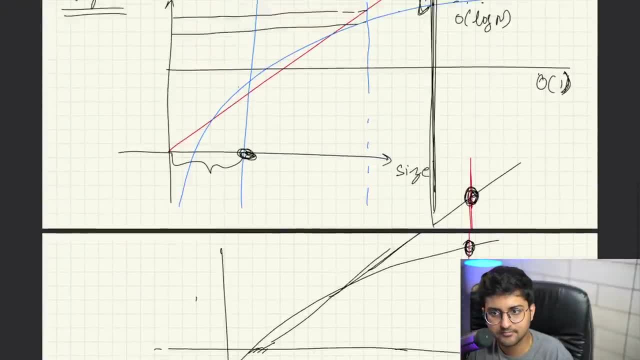 point. the trend will not change after this particular point. when this particular thing is holding true, you can see that this true will hold for indefinitely as the size increases. can you all understand that? and you know that you don't really have to care about small data. you don't really have to care about small data because it will hold true. you. 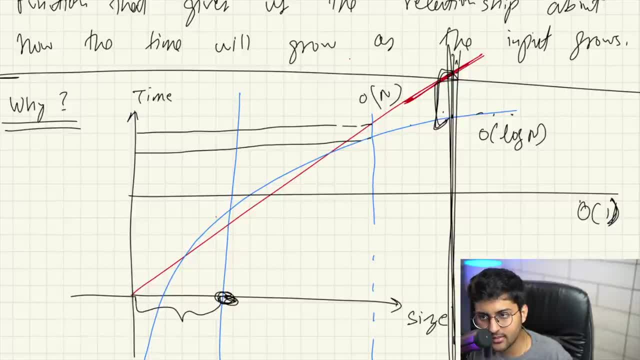 because small data complexity- it will never it. if your code is like that much optimized, it will handle small data irrespectively, does not matter which complexity it's working on. but the problem will arise when the data size has started to increase a lot. that is when you need to worry. 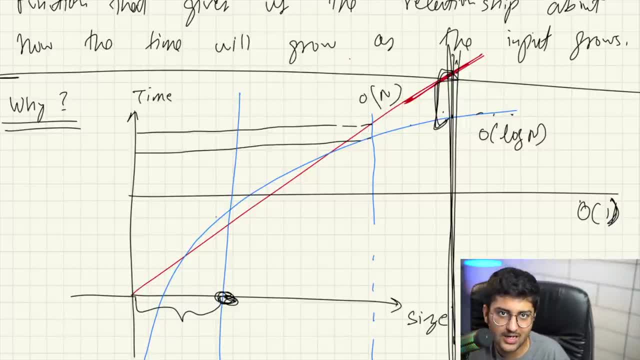 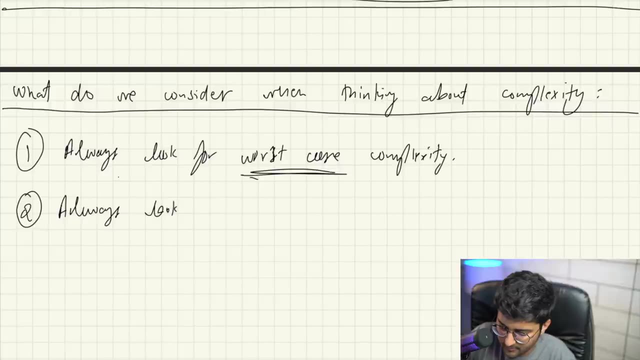 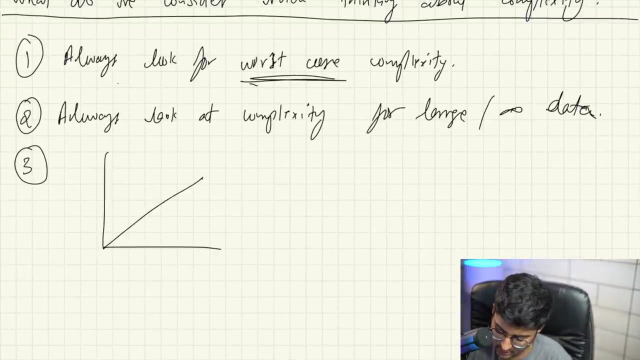 so are you able to understand why we are worrying about large size of data? okay, so, even though the complexity initially might be anything, we always look for complexity for large data. okay, always look at complexity for large, infinite data. point number two. point number two: third point: you know that if i have a graph like this, or if i have a graph like this: 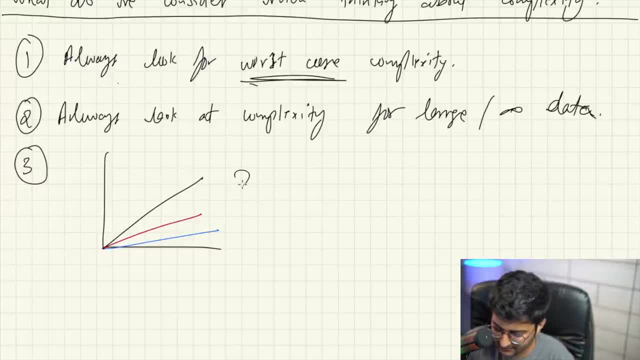 or if i have a graph like this: all of these have the same complexity, big o of n, linear, because they are growing linearly, but you can see the actual value is different. this can be something like you know: y is equal to, let's say, something like x. second one can be: y is equal to 2x. third one can be something like y is equal. 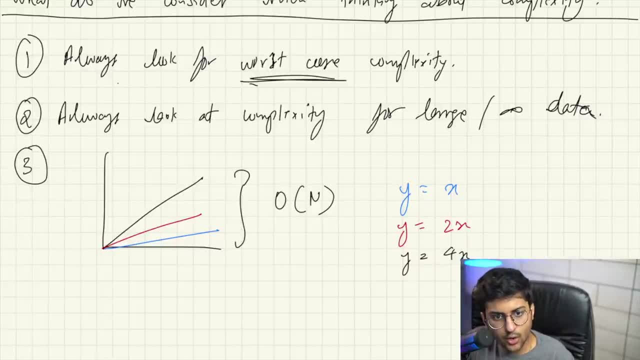 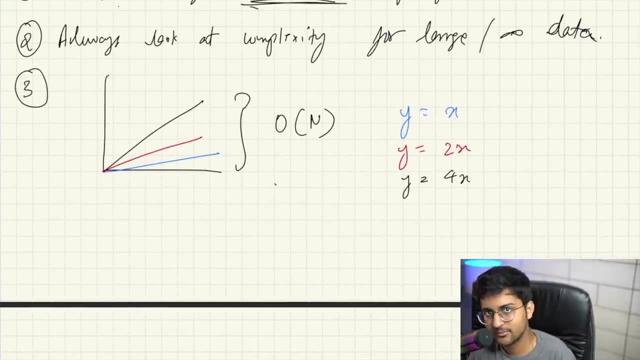 to 4x or whatever. so even though you can see that the values are different, you can see that they are actually growing linearly. only can you see that point number one. so point number one is: even though value of actual time is different, they are all growing. 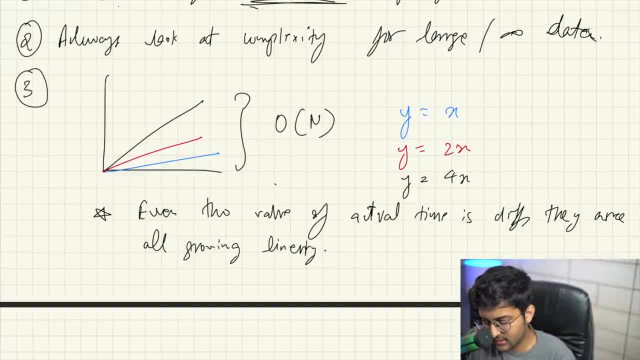 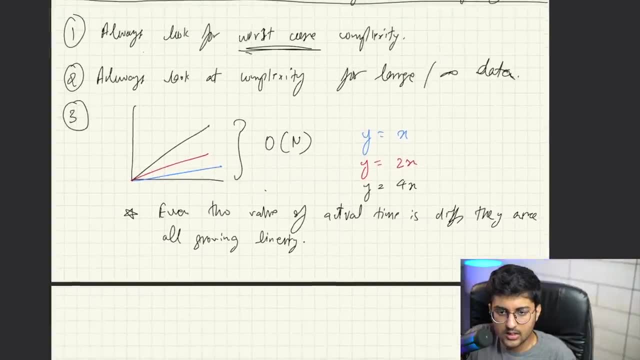 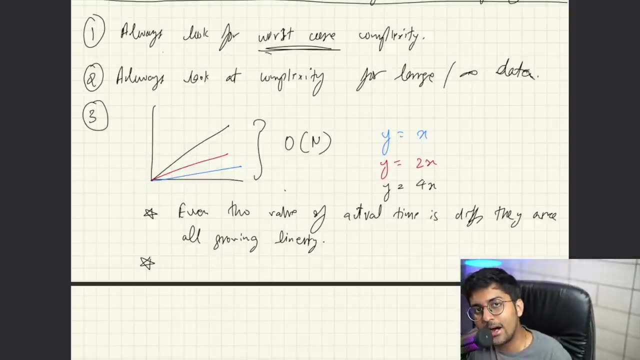 linearly. for those of you who don't know, under basic mathematics, these constants are actually the ones defining the slope of this. okay, so now the question is that, what is the question? question number two is: we don't actually care about what the actual time taken is. we know that we don't care. 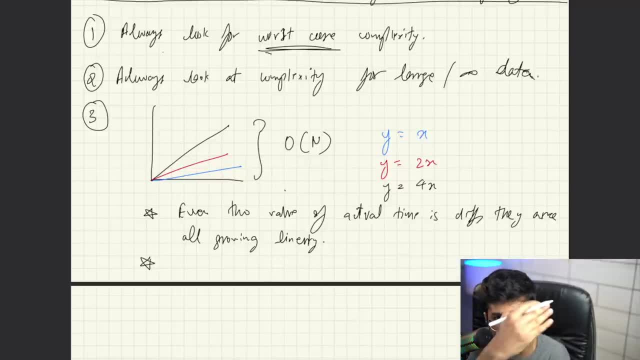 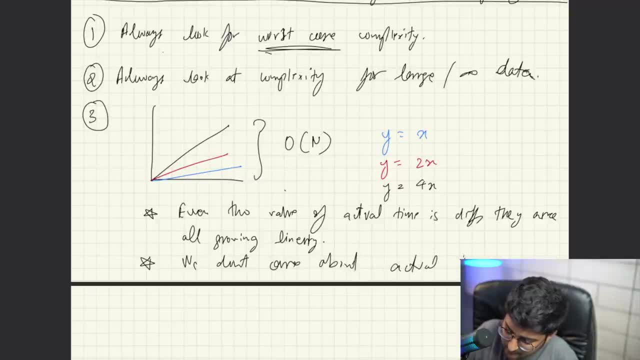 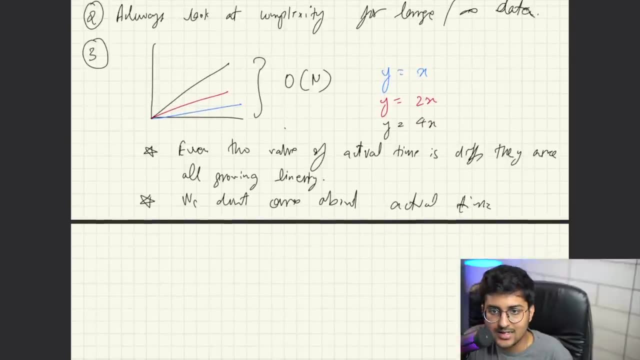 about actual time. we don't care about actual time, we just care about, uh, how this input is growing, as the how this time is growing, as the input is growing okay n time. then the question is, do we really need to worry about these constants? then if i say the slope was something, 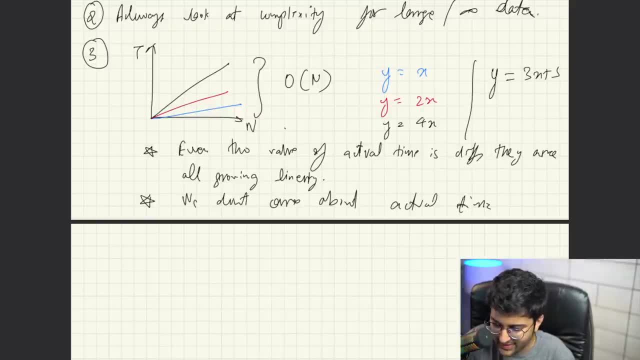 like, let's say you had something like: y is equal to 3x plus 5, even though this is giving the correct answer related to how much time will be taken. but do we really need that correct answer or we only need the relationship? yeah, you may have something like this: for x is equal to 0. 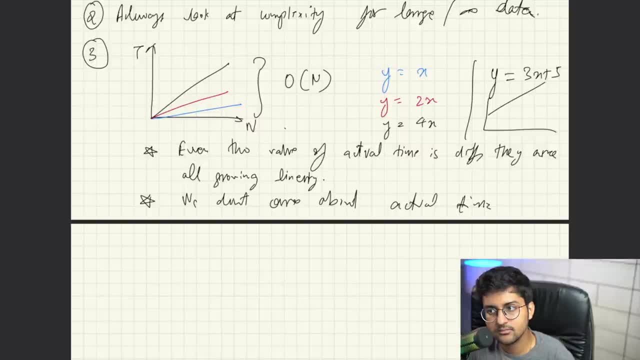 y is going to be equal to 5, somewhere like this. all of these will have the same complexity of n, linear. do we really care about what this extra time it's taking is, or whatever? no, we only care about how the line is going, how it's growing. hence, do we? 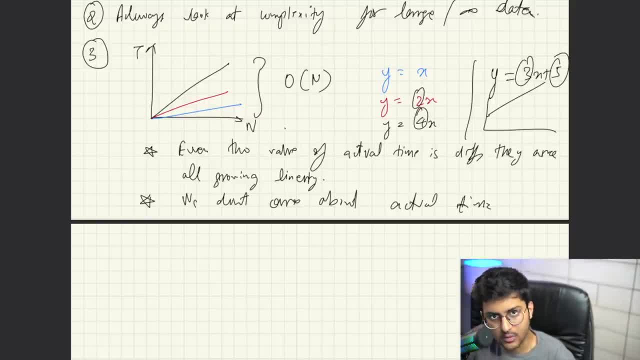 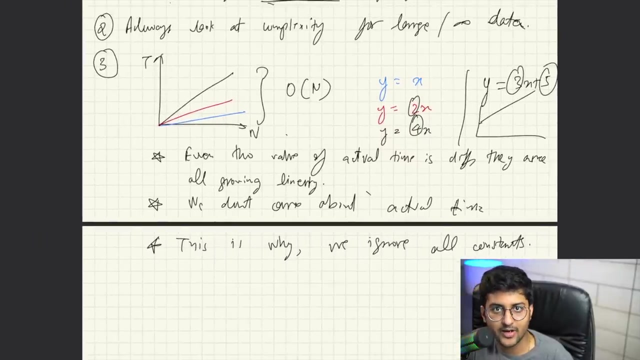 really care about these constants? no, this is why we ignore all constants. this is the reason for all of these points that i have mentioned. we are not done here. i told you for a reason. this is the one of one of the best time complexity lecture you can find on the internet. all of these three points i will prove mathematically also. 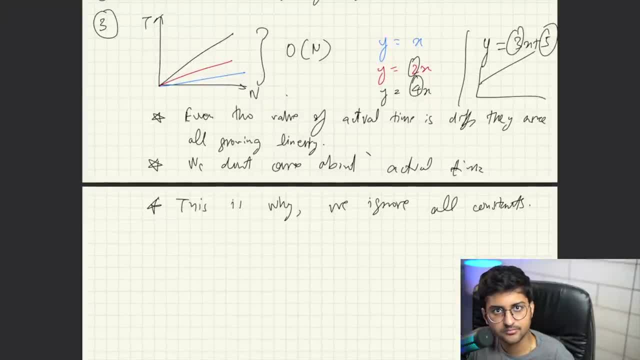 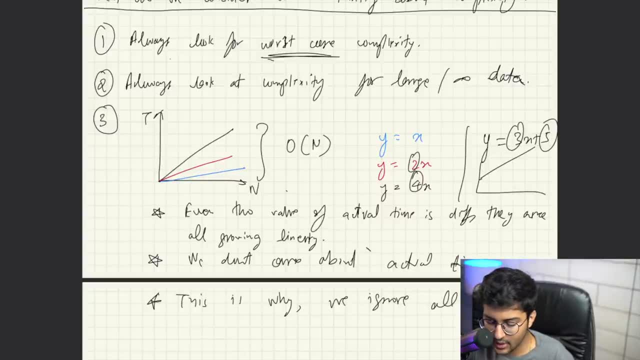 right now when we explain what is big o notation. i hope you were able to understand what we are doing. when we are considering about time complexity, always look at the worst case. we explained that. always look at for infinite, like the large amount of data. always ignore constants. 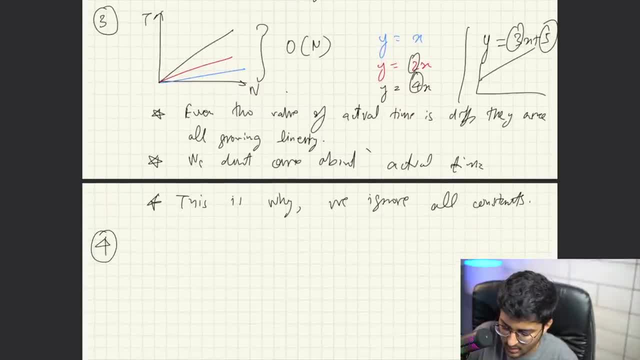 fourth point, also very important. fourth point is something like this: let's say you have complexity. something like big o is equal to 3x plus 5, even though this is giving the correct answer, let's say the graph is something like: let's say n, n cube plus log n, something like this: 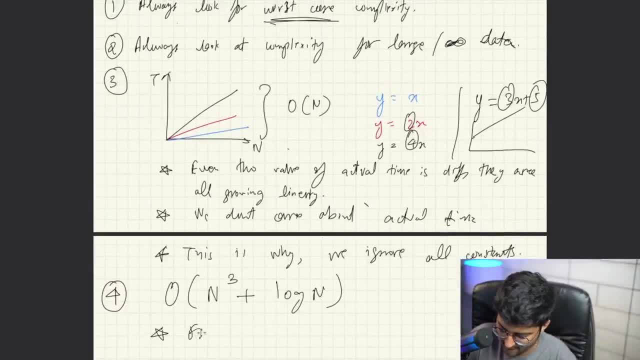 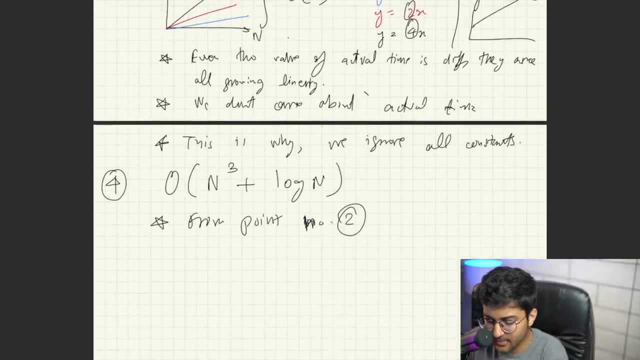 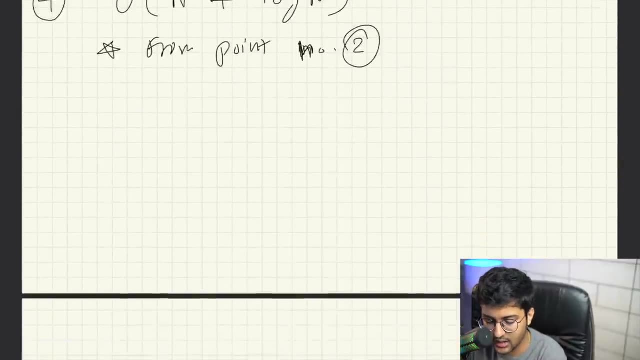 from point number two. from point number two notice something: what i'm trying to say over here. point number two says what point number two says: when you always have to take large amount of data into consideration when talking about complexity analysis. so if i am talking about large amount of data, let's say 1 million amount. 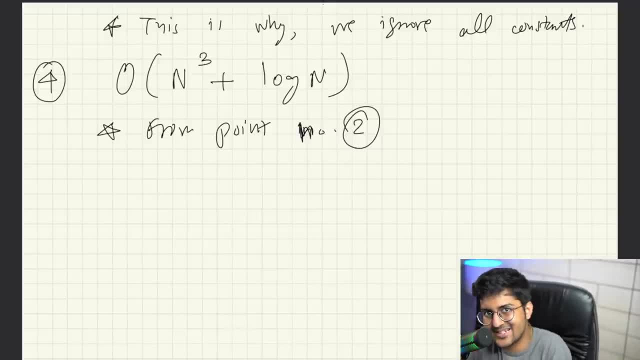 of data. what is the total time that will be taken? let's say, on an estimate- if i try to decide over here, this is a random time, i'm throwing at it- let's say for n cube. let's say for 1 million size of the array, it's taking something like you know, 1 million cube seconds. 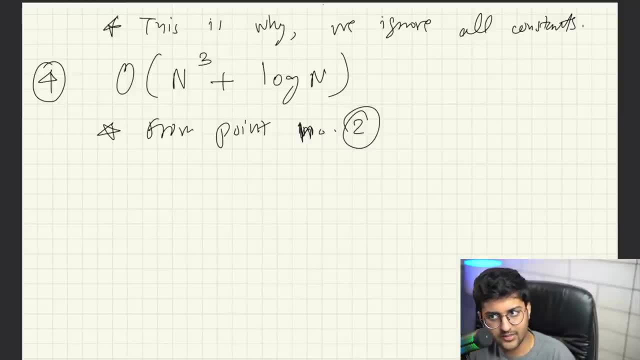 of data, for example, it might not be possible in real case- or 1 million time units of data, 1 million seconds, or okay, no problem, because it's hypothetical, so okay. so, as you can see, let's say for large amount of data. from point number two, let's say: if we're talking about 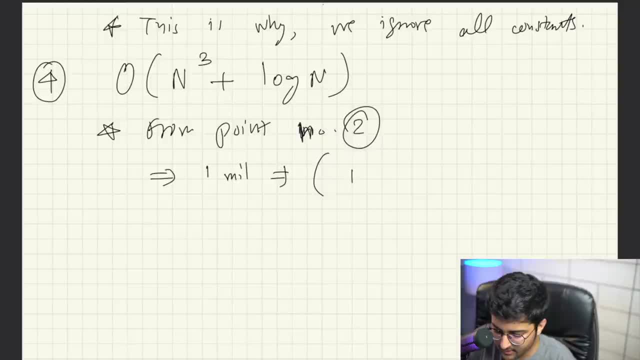 1 million size of the array is running this algorithm, it will take 1 million cube seconds plus log of 1 million. it's going to take around how much then? what is log of 1 million 6? so it's going to say 1 million cube seconds. now this is going to be taken by the i and i sum, which is realizing. 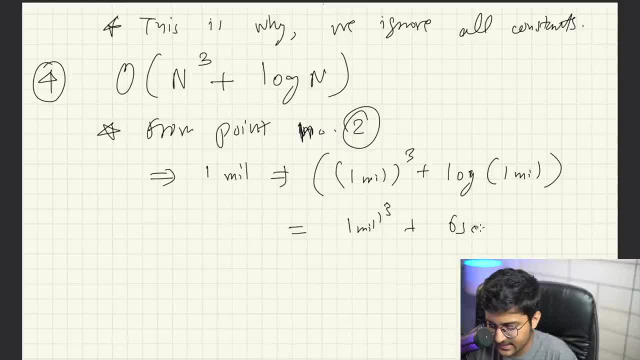 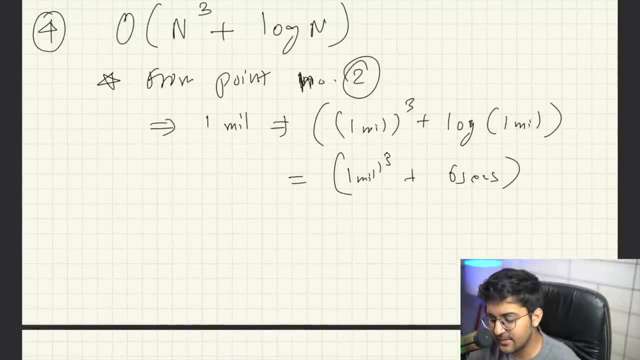 it's going to take around 1 million cube seconds. so it's going to say around 1 million cube seconds, seconds plus 6 seconds. your total time is, according to this complexity, 1 million cube seconds plus 6 seconds. 1 million cube might be something plus 6. 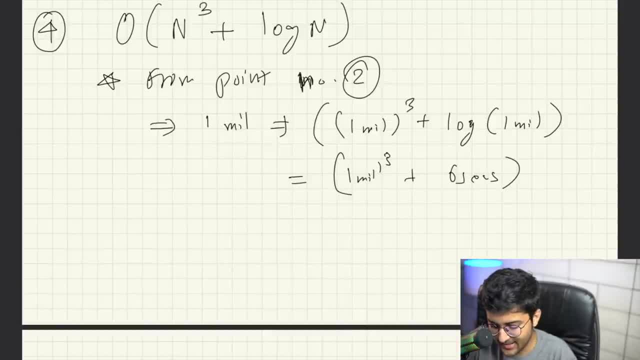 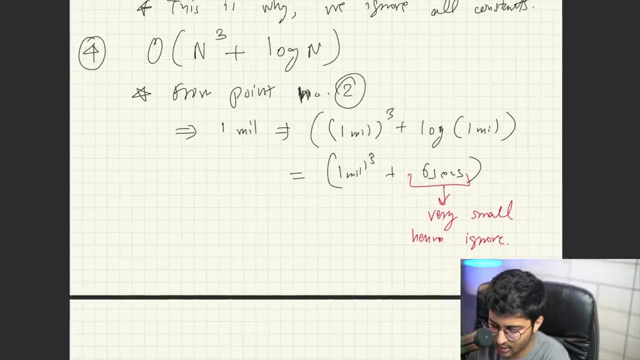 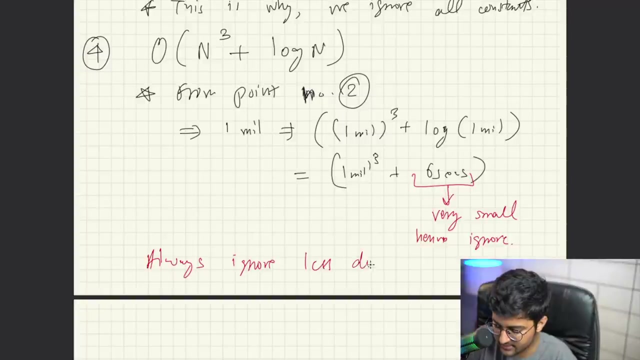 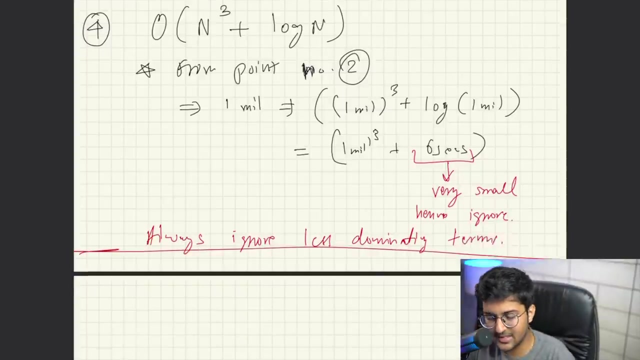 seconds. does this 6 seconds when compared to 1 million cube seconds? as any significant has any significance, this is very small, very small, very less value. hence ignore it. hence ignore. what does this mean? this means point number 4: always ignore less dominating terms. with these four points, you can derive the complexity of any equation, literally. 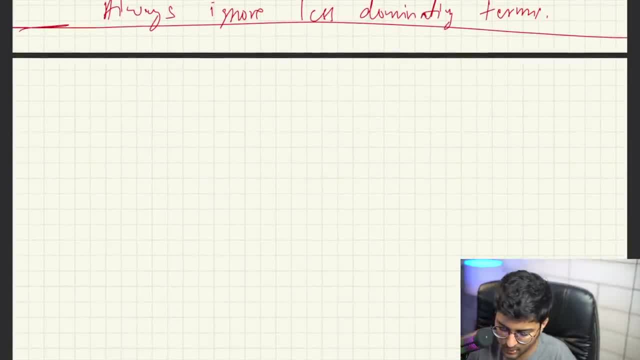 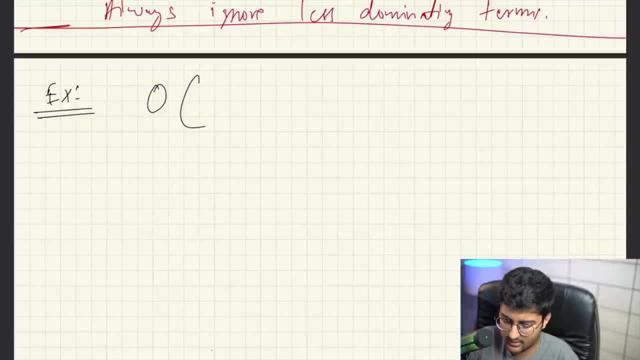 okay, let's say an equation is given to you. we will cover more about that later on. let's say an example can be given to you, something like this: let's say we're given something like big O of 3, n cube plus 4, n square plus 5, n plus 6, something like this. point number 1 says: 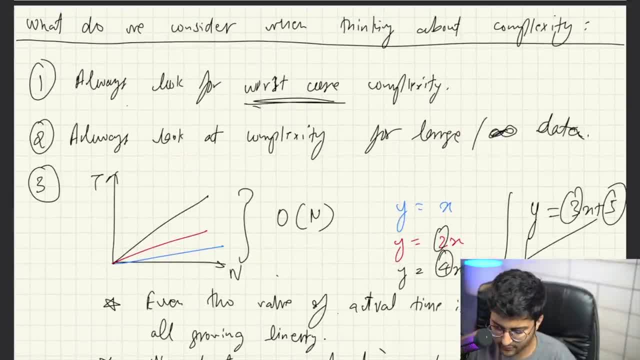 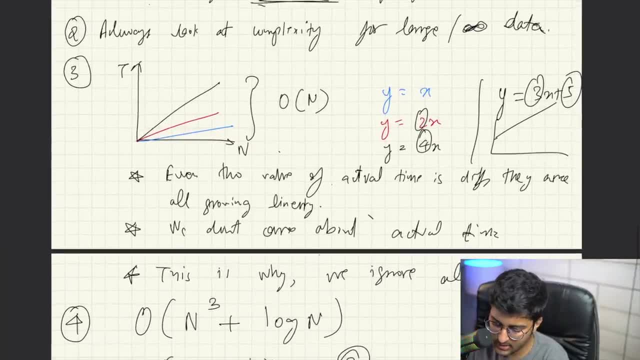 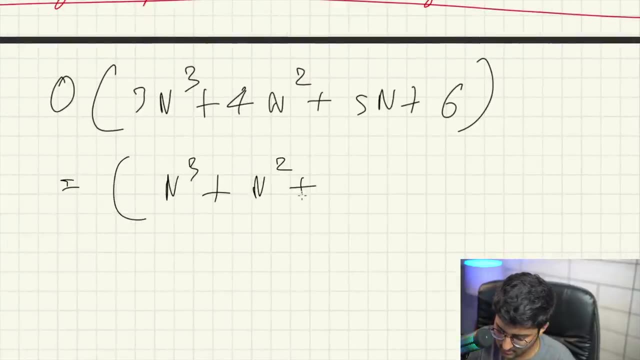 what here we have. point number 1 says: always look for worst complexity, always look for large value. okay, point number 3 and 4 are the ones that with which you can solve any equation. point number 3 says: ignore the constants. okay, I have a will ignore the constants, so this will become n cube plus n square plus n. 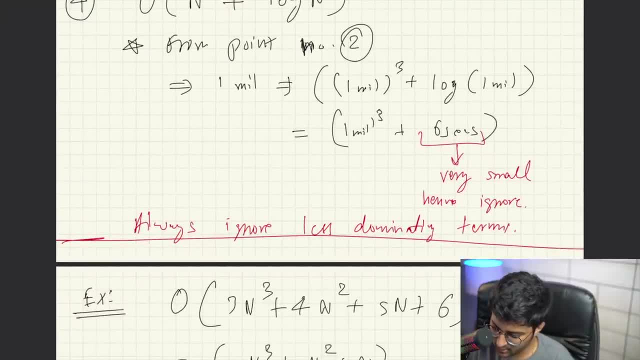 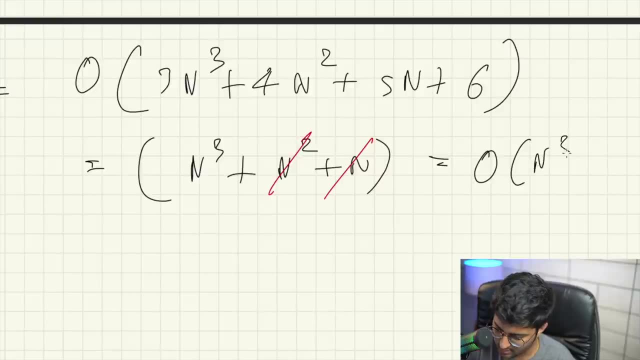 point number 4 says: ignore the less dominating terms. so I will ignore this. and this answer is actually equal to big O of n cube. I will prove this with mathematics also. so this is actually equal to this. this is actually equal to big O of n cube. 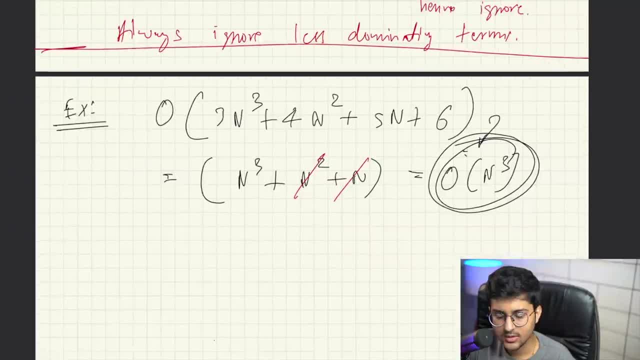 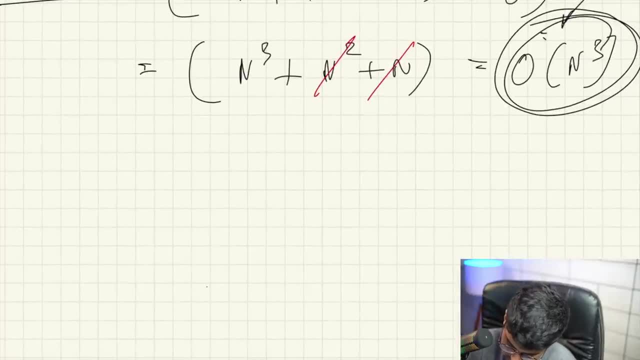 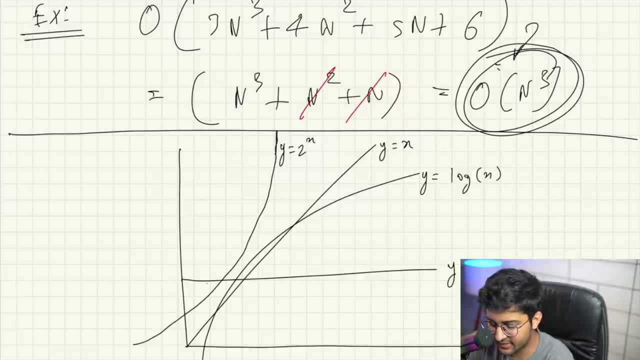 all right. so if I try to draw a graph of complexities like this, let's just draw a graph like this. let me draw a little nice, nice little graph for you all over here. in this graph, can you see that? you can see that for such a small amount. 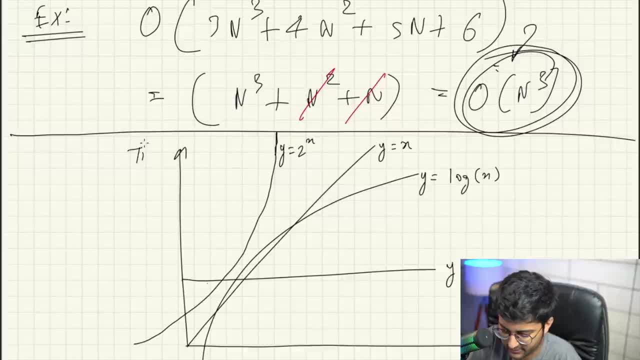 of size- if I have size over here and time over here so you can see y is equal to C- will always be constant. so it will always be less than whatever value you provide for all. what for? for anyマゼ todas, or for whatever value you provide for any. as for the catfish we are applying for, n and n is equal to 1, and 1 and n minus n associated to em will always be less than whatever value you provide. so it will always be less than whatever value you provide for all whatever, for Master, for any games, by win a shoutup question. 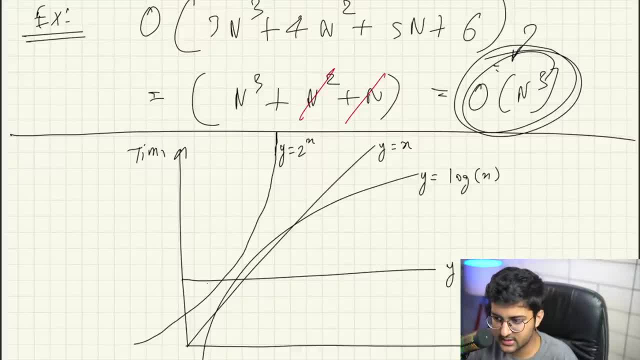 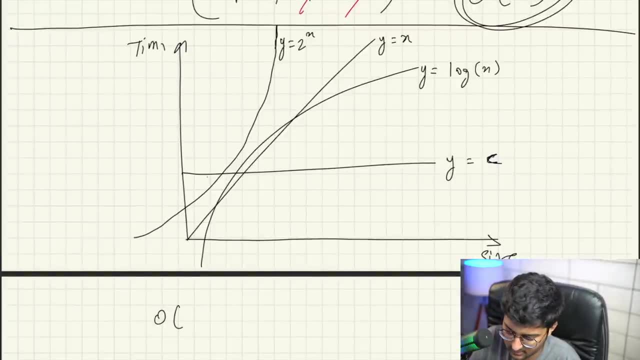 value that is greater than a particular threshold, like. obviously we consider large numbers, so you can see that y is equal to c- will always be the very best optimized. that's why constant is the best one. after that you can see log x. so if i take some large amount of data over here, 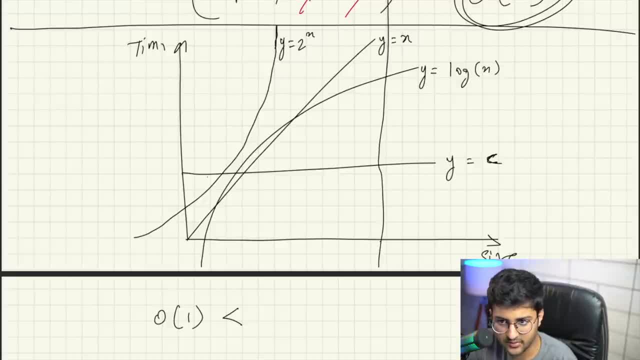 okay, for same amount of data. you can see y is equal to c will be giving the less amount of time. after that the time will be with the. y is equal to log n, so log of n. okay then the next amount of time a little bit more will be in. y is equal to n. 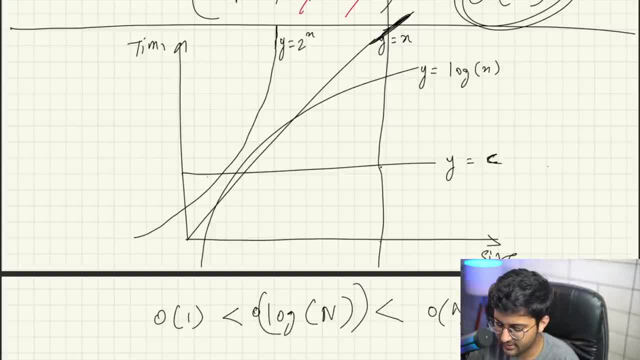 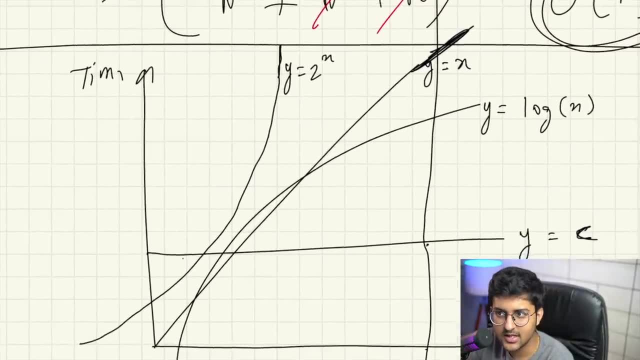 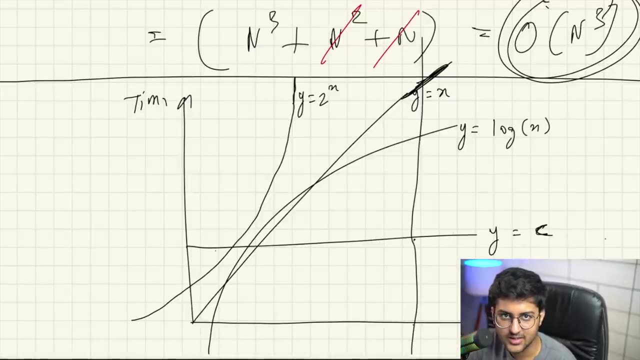 this is big o of log n, this is big o of n. and then, as you can see, this is the very, very, very bad complexity, which is y, is equal to 2n, which is exponential complexity. exponential complexity, fibonacci number example: that was exponential for such a small amount of data. 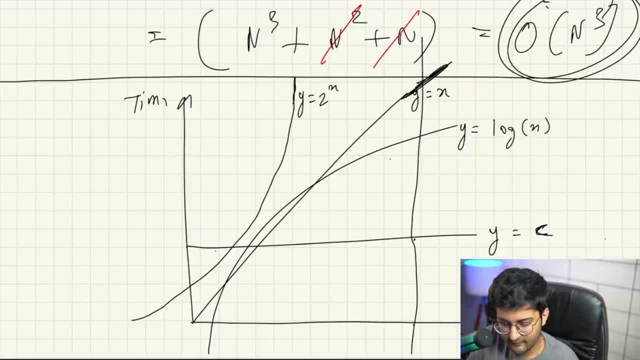 time limit has exceeded it a lot, but just for such a small amount of data, it's taking so much amount of time that it's already not even visible on the graph. that's why this is very bad. that is why for n is equal to 50. 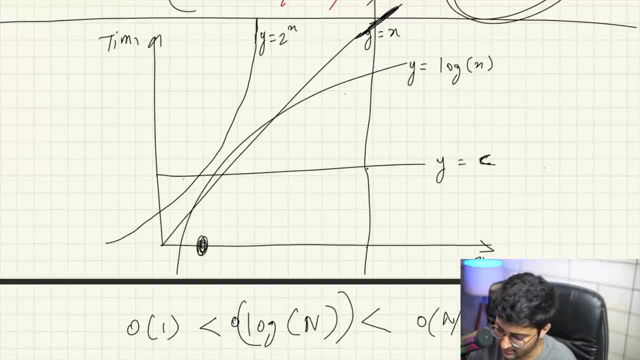 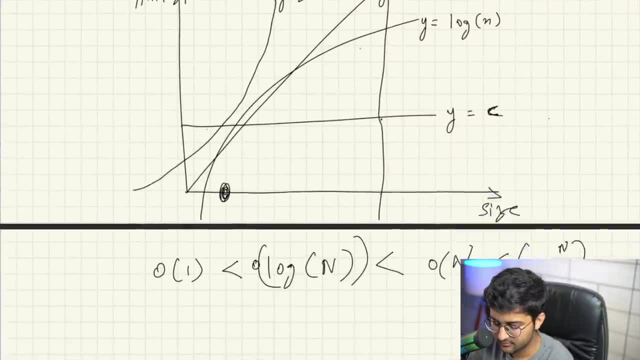 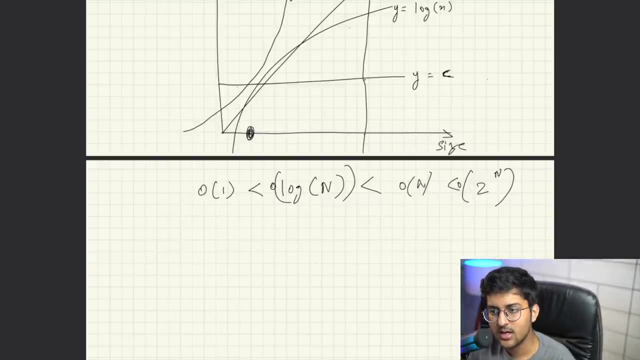 you are not even getting the answer for fibonacci number. here we have then exponential complexity. okay, this is sort of like the, so try to. we are always going to try to put it as less as possible. now, this is not like the you know standard, all the like that these are only. 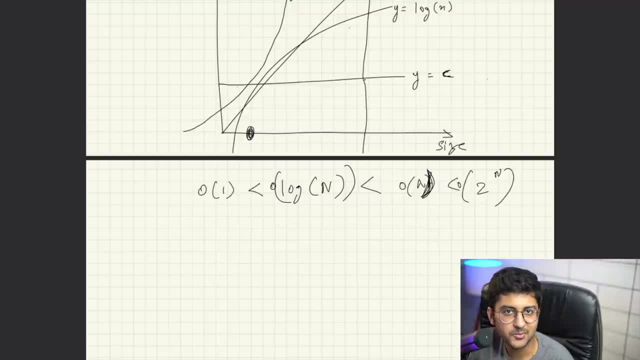 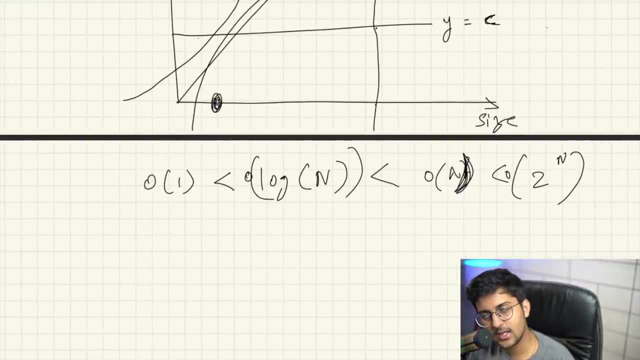 it's not like these are the only complexities that exist. no, you have to figure it out, like, for example, what if i gave you n log n, then clearly you can say n okay, n into log, and if i'm talking about larger numbers, it's definitely going to be more than n, so it's going to lie. 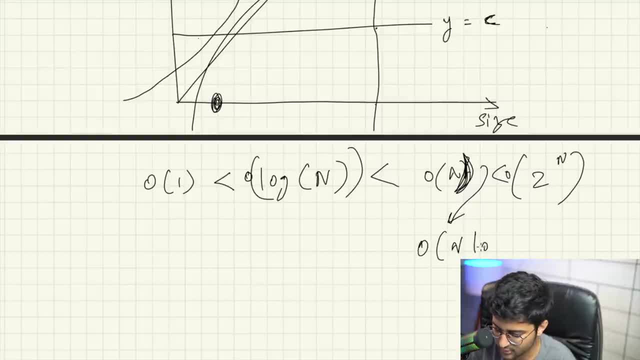 somewhere over here. somewhere over here and log n is going to lie. n square log n will lie where n square log n will lie after this and before this. it's very common sense. okay, you have something like this. i am multiplying this with something else, so obviously it will be. 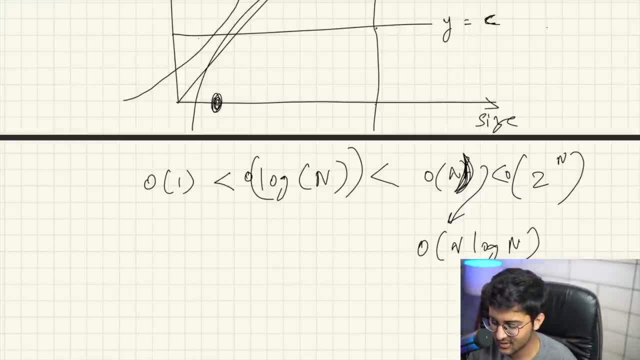 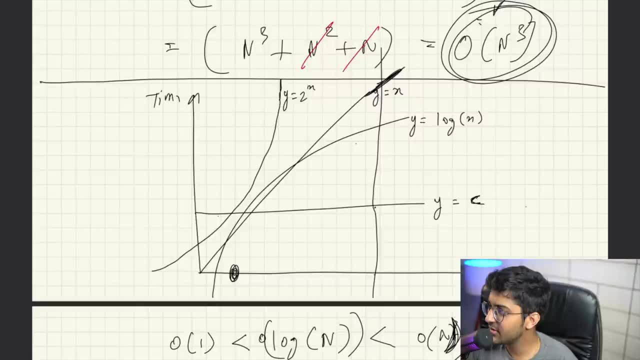 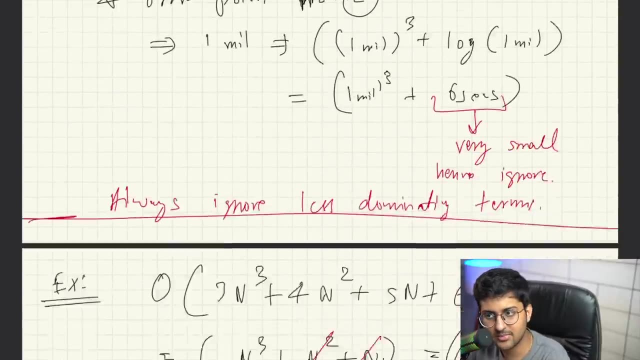 greater. okay, cool stuff. this is basically about why we care about these functions. all right now, before moving forward, let's get to the main part, which is big o, notation and all these, and proving all of these things with math. with mathematics it's going to be very simple. mathematics don't. 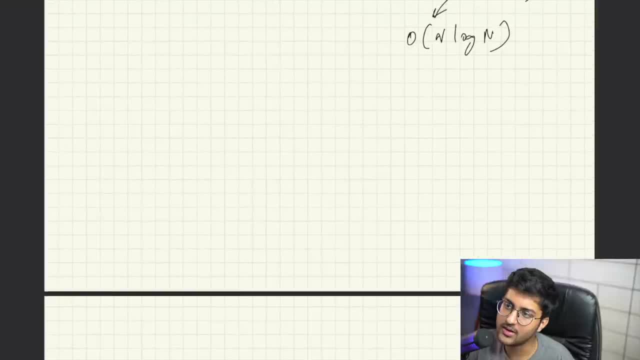 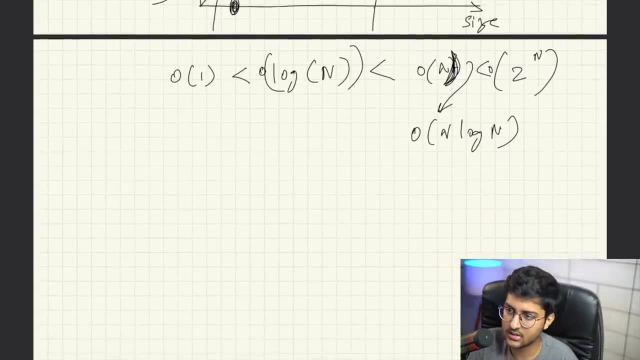 worry about it. no prerequisites are like as such. only you need to know when we learn about recursion, but if you're already following the course, then no prerequisites are required. let's talk about big o notation and all these other notations. what do these actually notations mean? 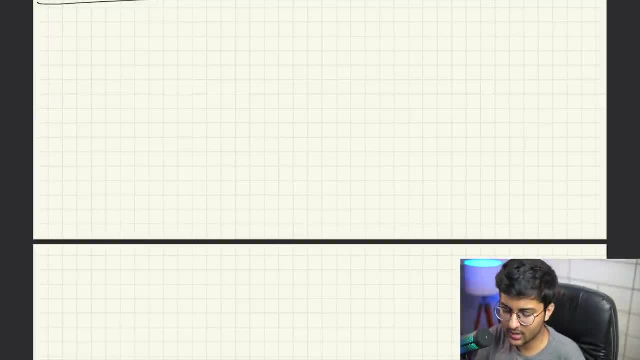 what do we mean by big o notation and what is all these things? now, what does it mean by big o notation? okay, let's see: big o notation. what is this thing and why are we actually cared about this? we will also look at. we'll look at two things in order for you to understand this. 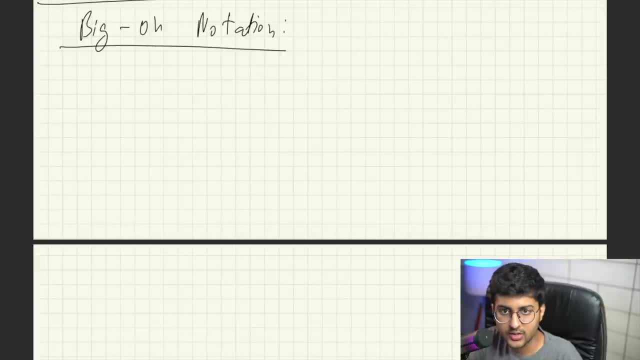 first we will look at the wordly definition. what does it actually mean in words? second we'll look into is the mathematical definition. what does it actually mean in words? second we'll look into is the mathematical definition. what does it actually mean in words? second we'll look into is the mathematical 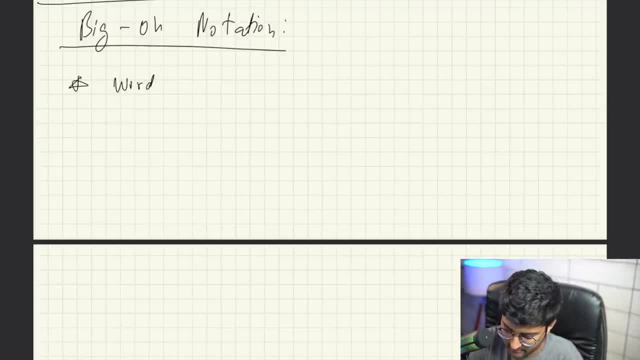 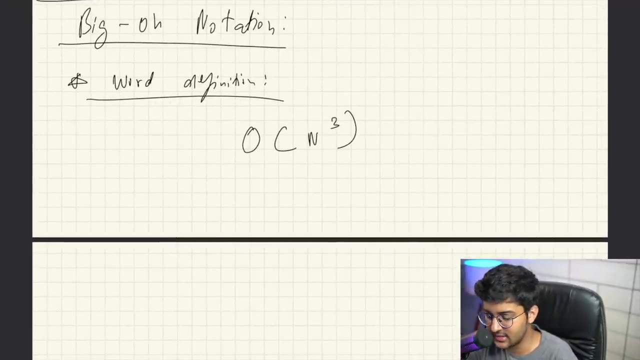 representation. so word definition, word definition. so if i say that an algorithm has a complexity of, let's say, big o of n cube, okay, let's say an algorithm has a complexity of big o of n cube, let's say interviewer sells you or whatever. you have a discussion, you say, hey, the complexity of my solution or algorithm that i have written. 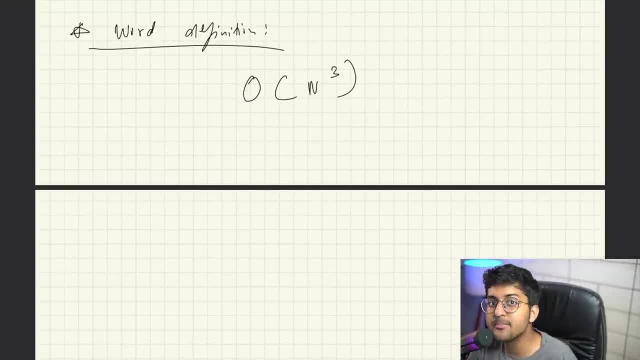 is big o of n cube. what does it mean in words? what does it mean in simple language? in simple language, it means that this is the upper bound meaning. my complexity, my. you all know what n cube means. you know that the size of the array will grow as the input grows in an n cube fashion. okay, let's like we saw with. 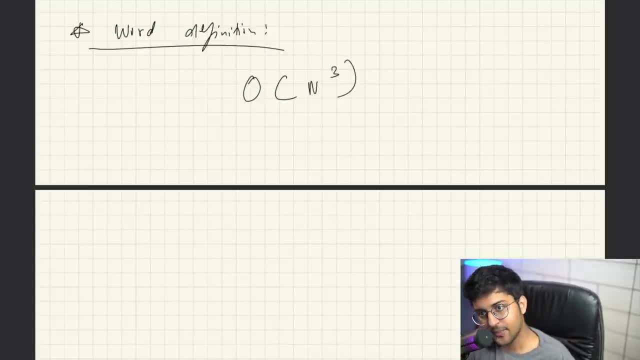 binary search or linear search or whatever, but what is this big o saying? big o is saying: okay, you have the graph, or whatever. that's fine, but what is this big o saying? big o is saying that this is the upper bound, this graph that you have is the upper bound. meaning in simple language, in: 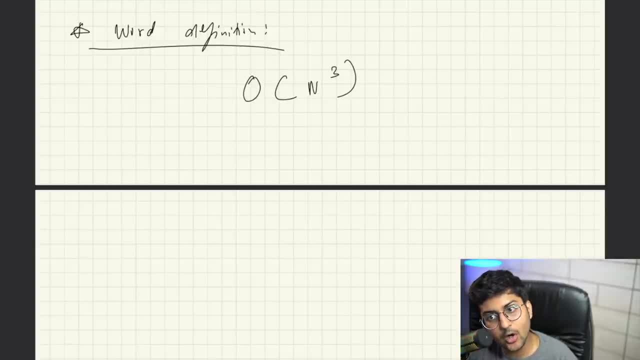 simple language, the graph, the relationship. it can not exceed n cube, for example. your algorithm that you have written may be solved in constant time. it may be solved in o of n time. it may be solved in o of n log n time. it may be solved in o of log in time. it may be solved in o of n square. 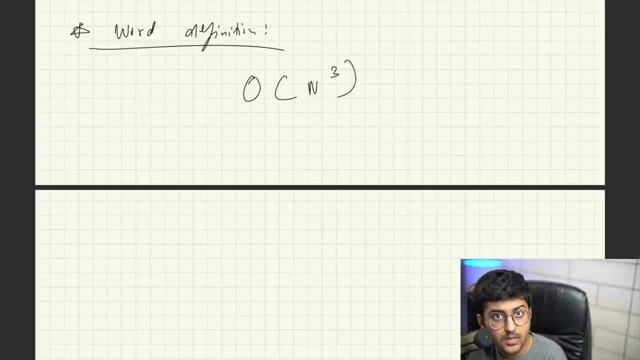 time. it may be solved in o of n squared log n time, but it will never be solved. it will never exceed the time complexity relationship. the graph might depend distinctly on the data. i haveateed the chart, the time complexity certain, but the relationship cannot be화 32: 00. the graph is only a validation. of n is the square messages, the a zero, n is the bishop times. nothing but this pentagonal height relationship. it is complete one of the main structure to pregunta to question this question: the graph: what is a painters of a in Bertram or something else? the minimum value that a能. 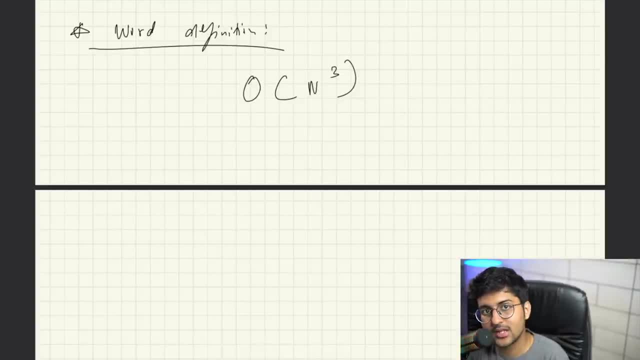 graph the function value. it will never exceed more than n cube. that that relationship thing that we talked about. it will never be like o of n raised to power, 4 of o, or o of n cube log n or whatever. that's the wordly definition, meaning the complexity. basically, this is the upper bound. i. 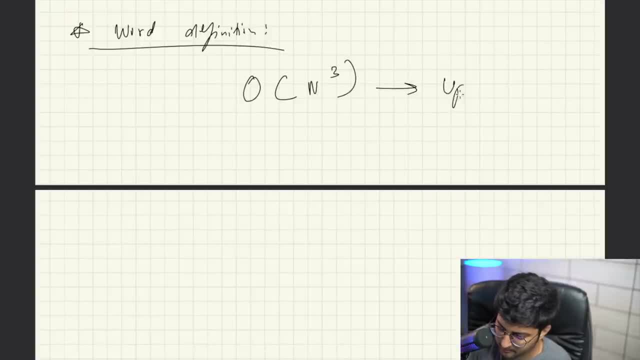 don't think i should write this. you can write it yourself. upper bound, upper bound, so it will not exceed this. your algorithm may be solved in n square. your algorithm may be solved in um. you know um n cube also. your algorithm may be solved in n square, log n. your algorithm may be solved in. 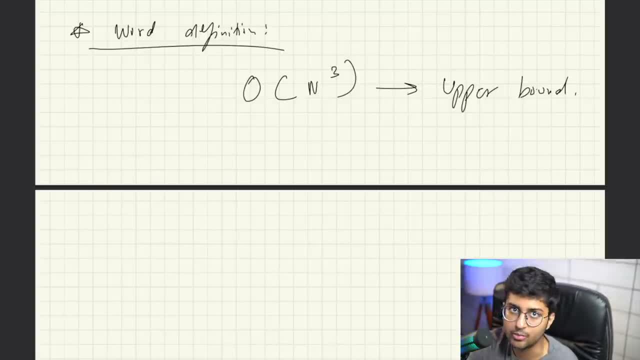 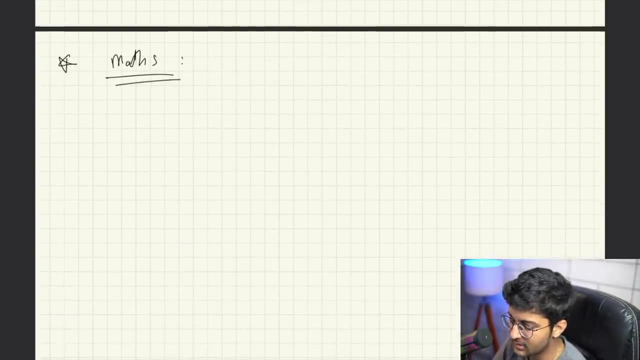 n square, log n, log n, but it will never exceed n cube. that is what the wordly definition is. okay. so if i'm saying, like the mathematical part, what is the mathematical representation for this? and here is where i will prove all the points previously, all the points that we took previously. so if you're saying a function f of x is equal to 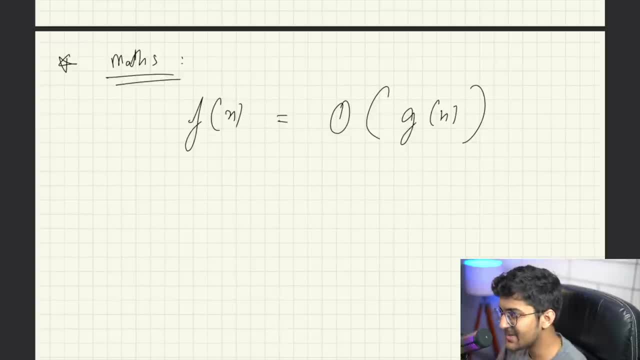 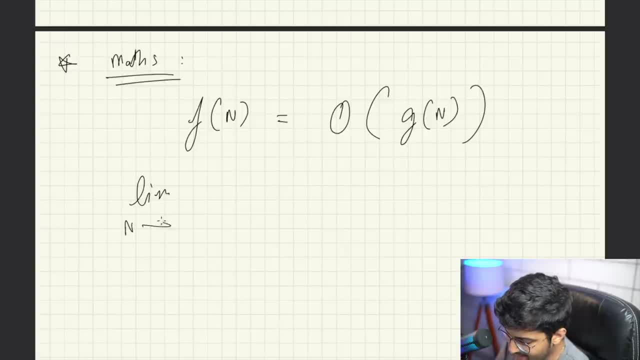 it means that limit n tends to infinity. you must, we must, have learned about limits in high school. f of n upon g of n is less than infinity means it's actually some value, a finite value. explaining this theorem, explaining this algorithm in terms of words is very simple. it's nothing. 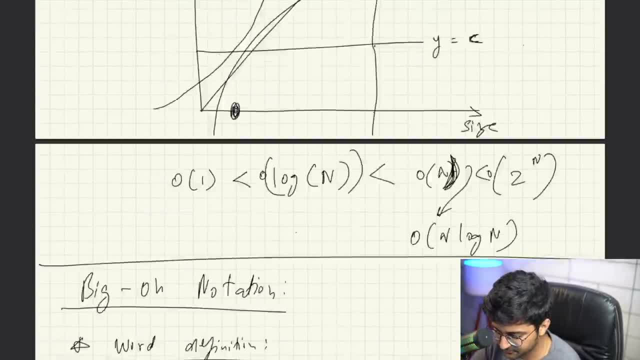 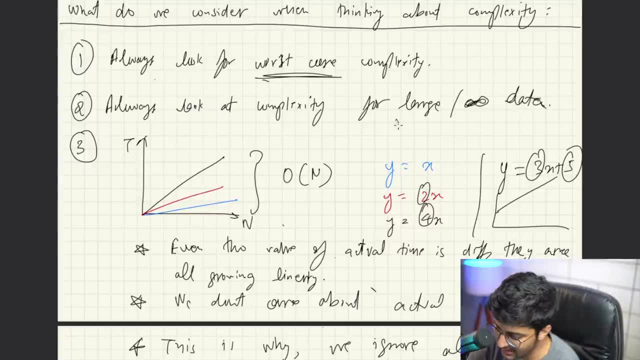 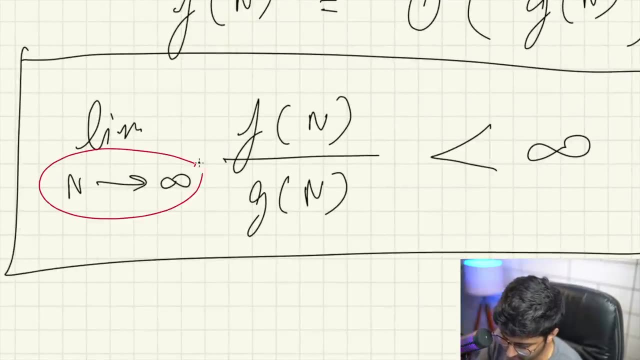 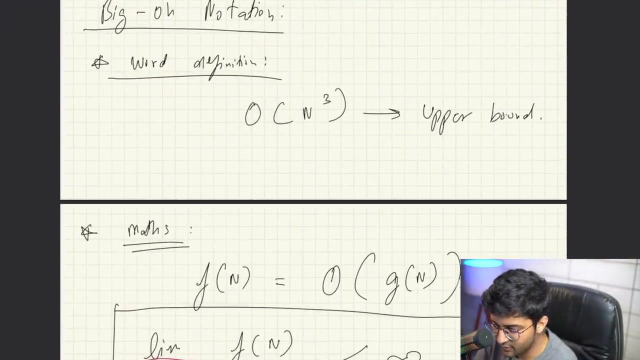 new. we have already covered this in this lecture. let's see, we have said that um, infinite. number 1 and 2 says that always look for worst complexity, always look for large values, infinite data. we are doing that. we are doing that over here. okay, we are saying that it's an upper bound, so it's a finite value will come over here. 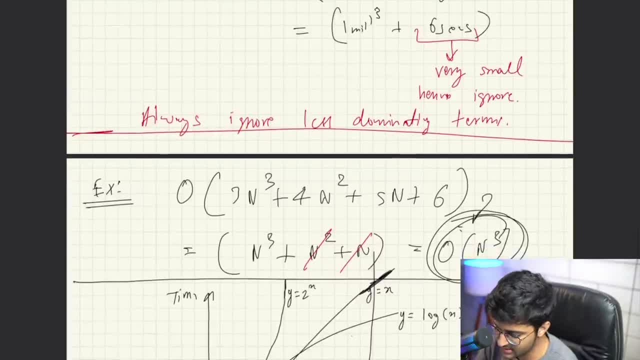 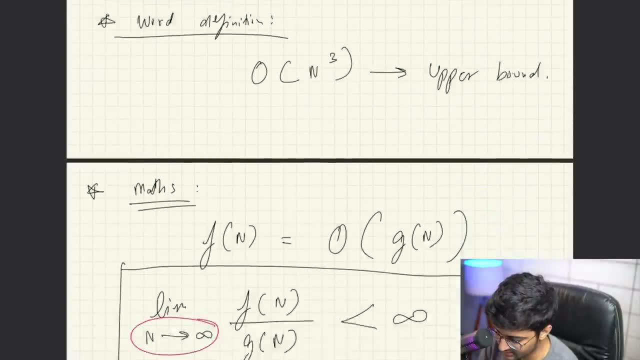 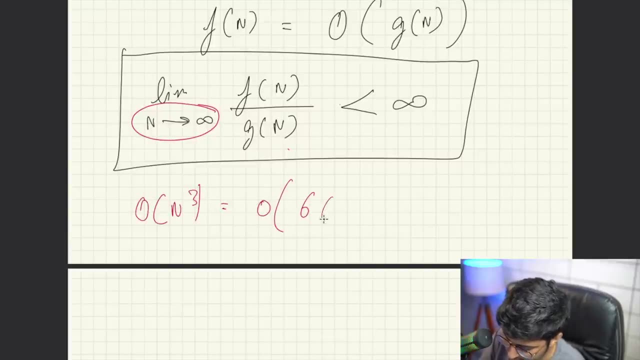 so, for example, let's take our example only, let's say this example that we took previously: 3 n cube plus 4 n square plus 5 n plus 6 is equal to big o of n cube. okay, so let's say, according to this example- i have said that big o of n cube is equal to big o of 6 n. 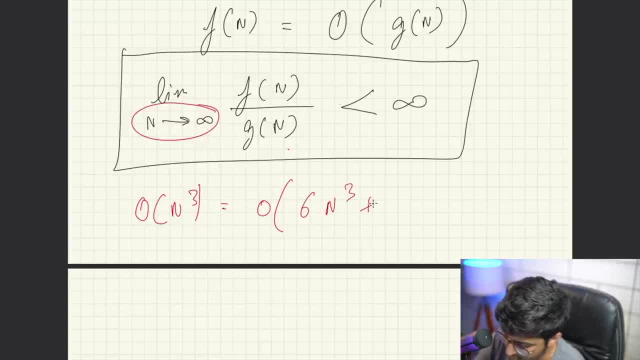 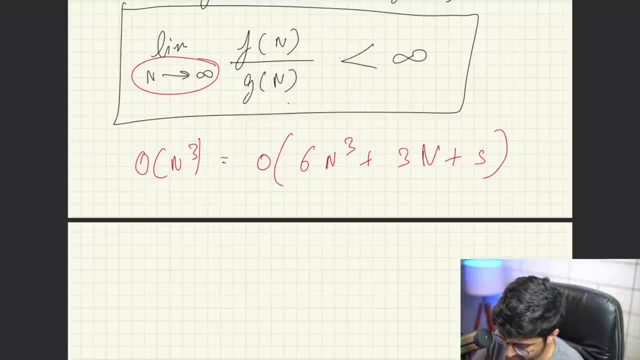 n cube plus 3 n plus 5 or whatever. so if i put this in this formula, if i say something like you know, this is f of n, this is g of n. so i can say something like: um limit n tends to infinity, 6 n cube plus. 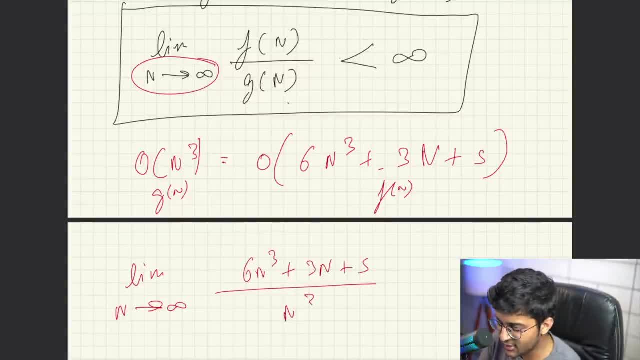 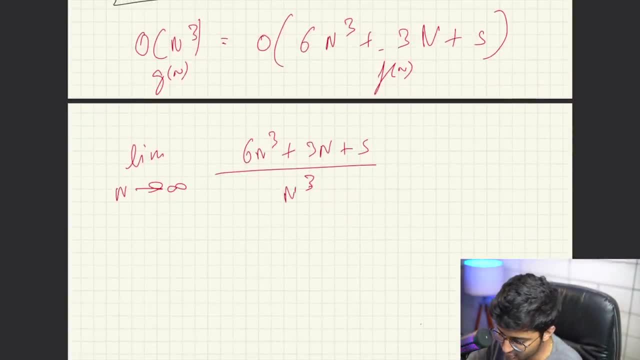 3 n multiple n positive without n into any bound: n plus 3n plus 5 divided by n cube. i'm not going to teach you limits. limits is very simple stuff. it basically means when the value of n in reaches infinity. that is basically what it's saying. close to infinity. 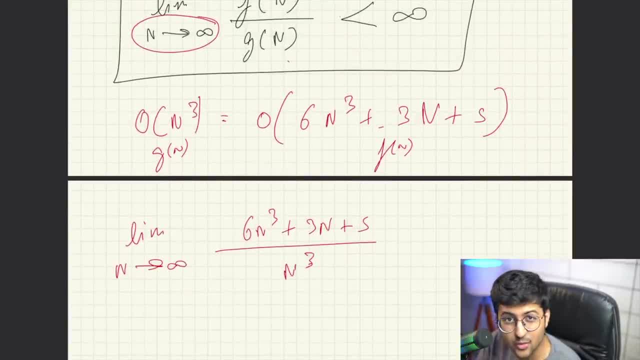 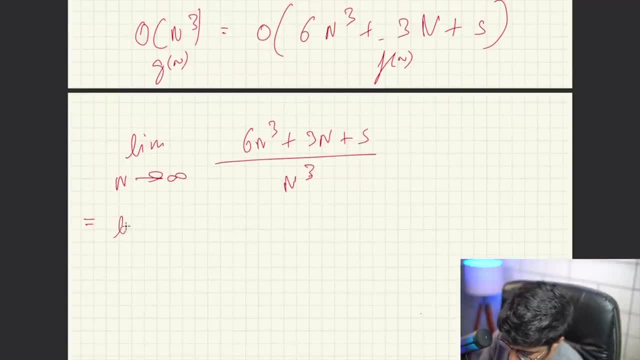 so there are already many lectures on limits on youtube. you can watch it. but this is high school mathematics, that's why i'm not teaching it. um, if i just divide it, so this is actually equal to what limit n tends to infinity. divide this 6 plus 3 upon n square. delete 3, 1, 2, $-n$n$0!$$!1. 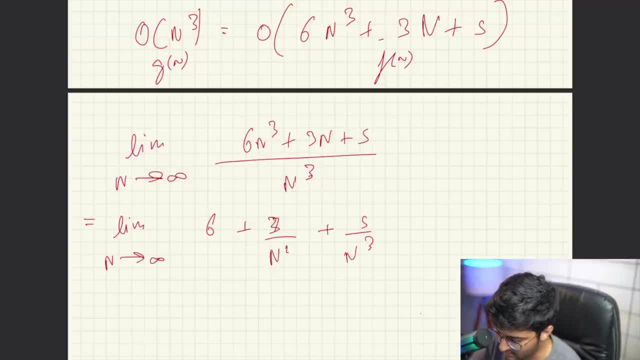 5 upon n cube. if i put n over here in this formula i'm actually going to get. this is equal to 6 plus 3 upon infinity, plus 5 upon infinity. this is actually equal to 6 plus 0 plus 0, because anything divided by infinity is equal to 0, and this is going to give me equal to what? 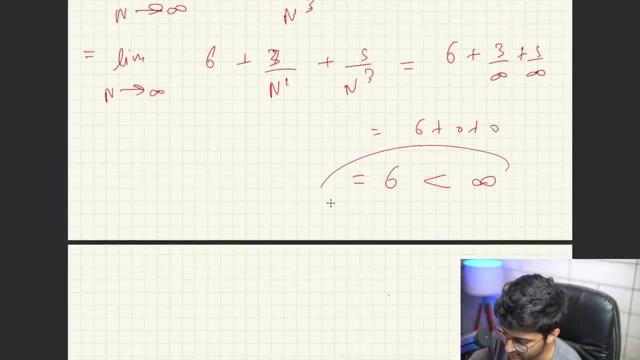 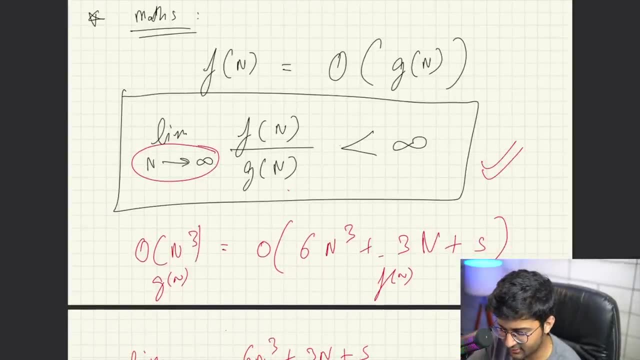 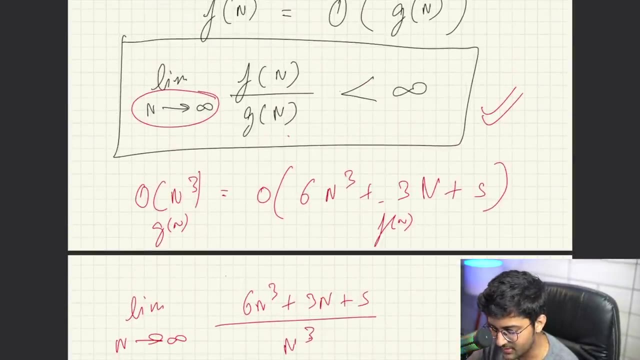 this is going to give me equal to 6, which is actually less than infinity. isn't this what this we are saying? isn't this now valid? isn't this formula valid now, after putting it in this formula? less than infinity? so if i'm saying that big o of n cube is equal to big o of this, 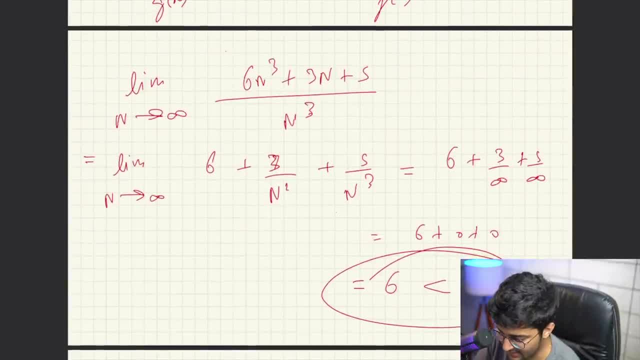 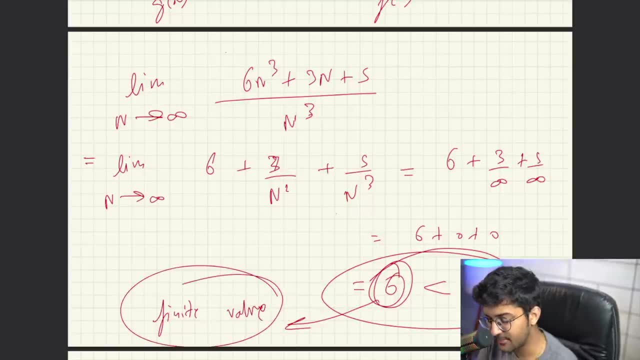 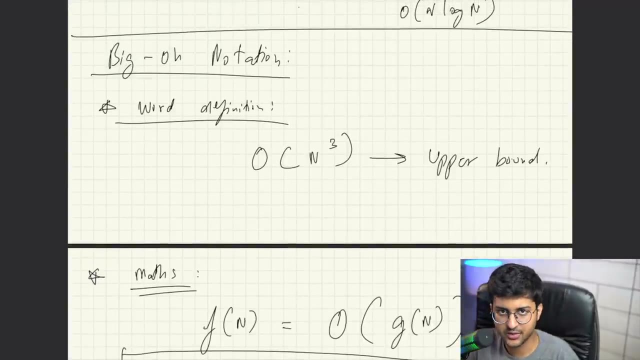 entire thing. then, after putting this formula, i should get some finite value, and i am getting the finite value. finite value because this is showing is an upper bound. okay, it's an upper bound. that is the mathematical representation for this. this is what is known as big o notation. again, in simple words. 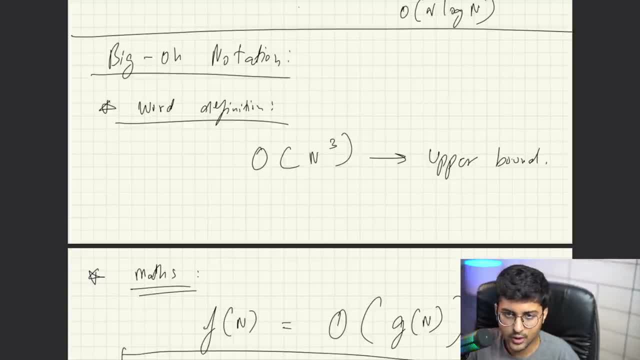 it basically means means that you know our algorithm will never exceed the complexity of this. it will. it can be better than this it will never exceed. similarly, if your binary search has the complexity of of login, it can also solve it in like less complexity. we see, like some other, it might. 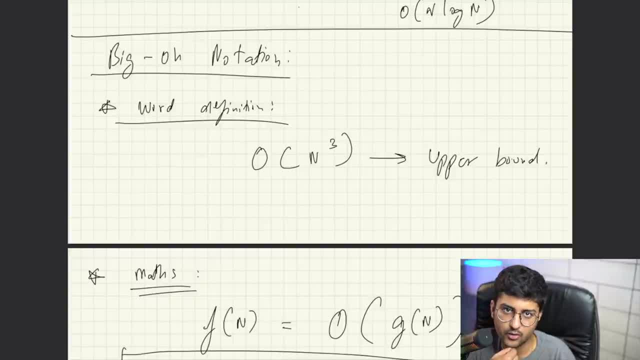 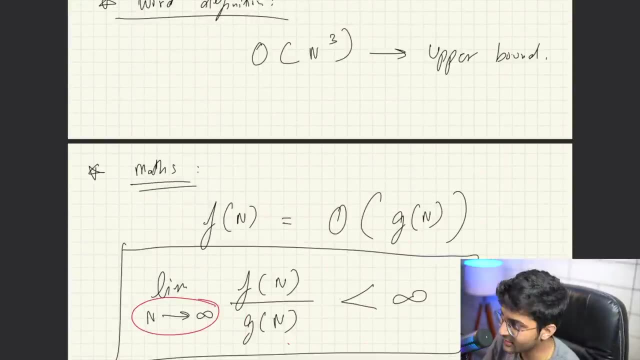 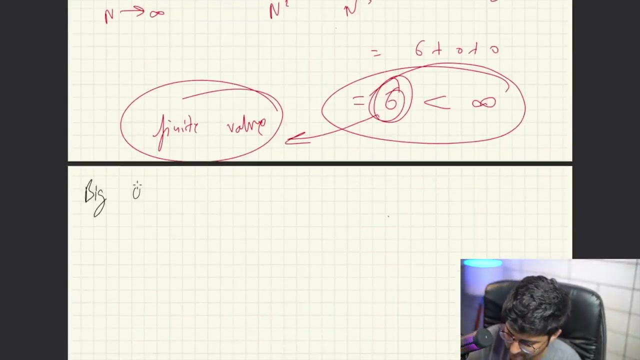 be able to solve it in, like you know, lesser complexity than login, but it never, in any case it will never, exceed login, this login and everything in just a function that i have already discussed. alright, cool. let us move forward to the second notation, which is big omega notation. big omega notation- this is actually opposite of big O notation. 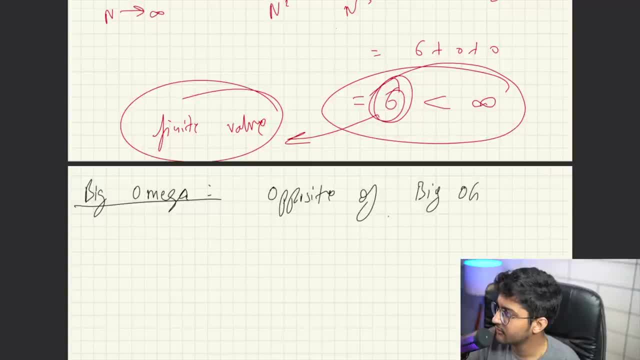 big omega notation, okay, is actually opposite of big O notation. so if you're saying a, if you're seeing, like in words, if you're saying that an algorithm has a complexity of big O of n cube, this means that it will take at least n cube time. complexity lower bound, it will take at least n. 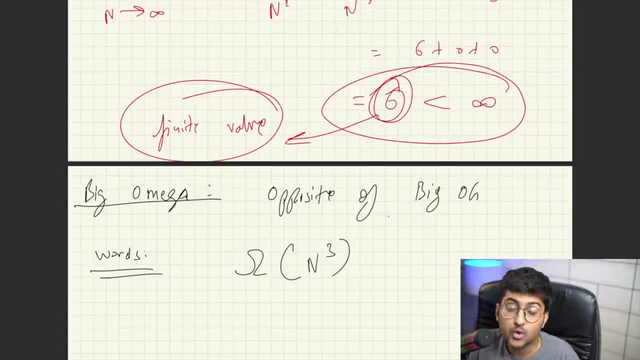 cube. it can also take n raised to power 4. it can take n cube log n. it can take n cube into 2 raised to power n or whatever, but it will never be less than n cube. this is a lower bound, minimum n cube. time complexity will be required. the graph: okay, lower bound. 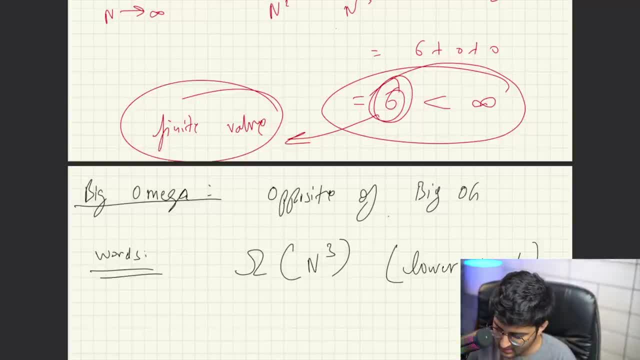 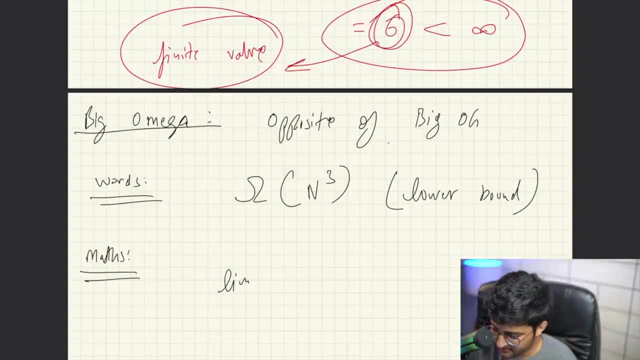 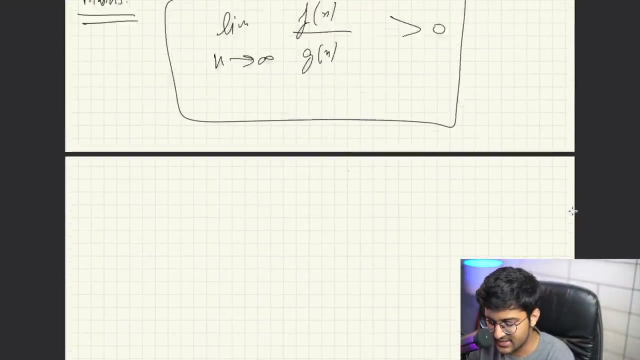 in mathematics it's very simple. limit n tends to infinity. f of x upon g of x should be greater than 0. cool, it's very simple stuff and I don't think it needs any explanation. so basically, just the opposite of big O notation. but we actually care about big O notation. 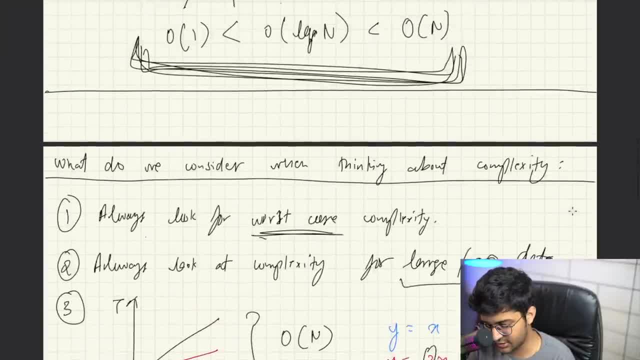 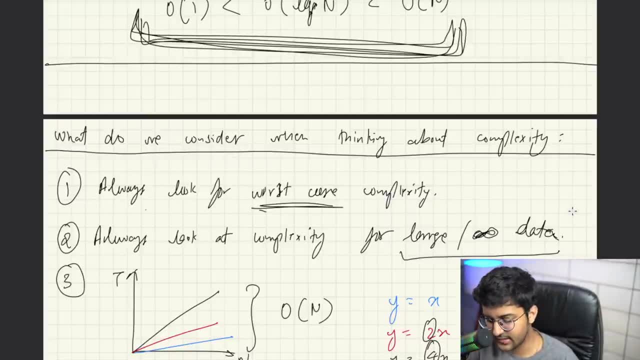 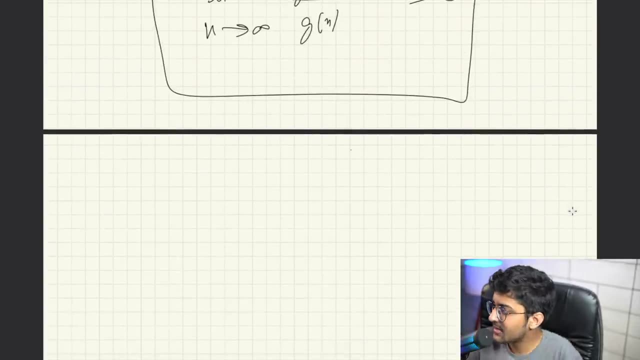 because why we always- everyone in the interview- also ask big O notation? because we always look at the worst case. with big Omega we're not actually getting the worst. it can be like more than that as well, but we need the worst case. okay, big Omega, cool. now sometimes we also want to specify the running time. 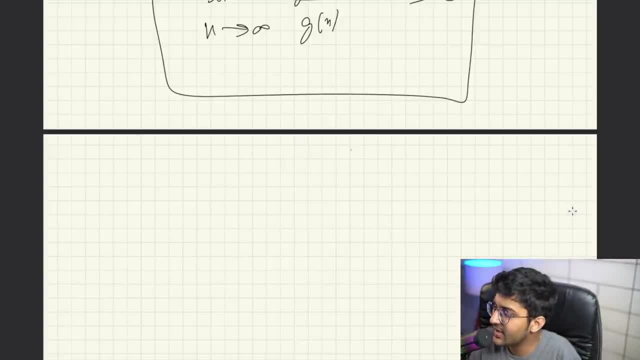 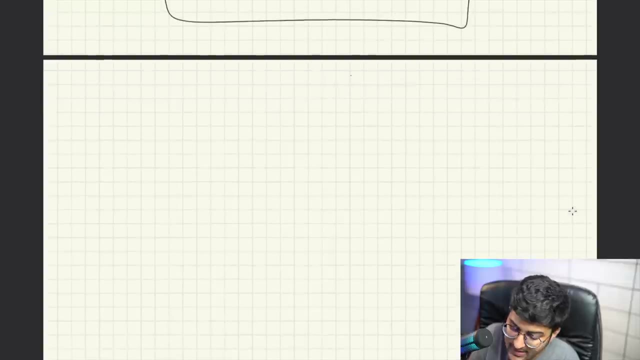 that is precisely like, equal to whatever equation that we have, like both upper bound and lower bound combined. okay, so how can we do that? how can we do, let's say, an algorithm runs in, you know, in the let's say the algorithm has a. basically, what I'm saying is what, if the algorithm has a lower bound and an upper bound of? 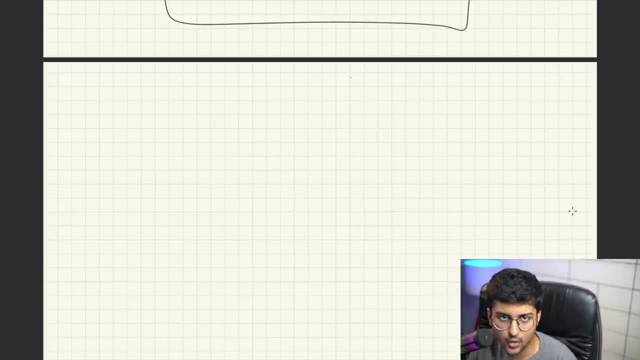 n square. how can we know? how can we show that? so question: what if an algorithm as lower bound and upper bound, as big O of n squared, sorry, as n squared, as n squared, how do we represent this? we can do something like this. we can say: it's. 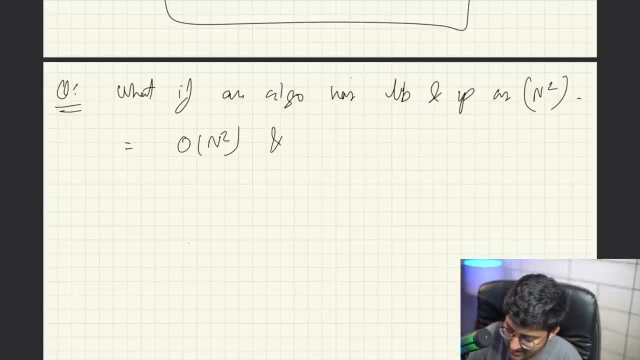 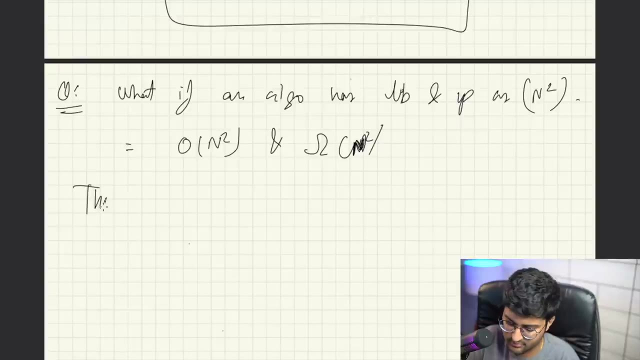 equal to big O of n squared and big Omega of n squared 5. so from now we have given over here the step to the right, and from the left we have the till. so from now it becomes one over n to the one over o, if we 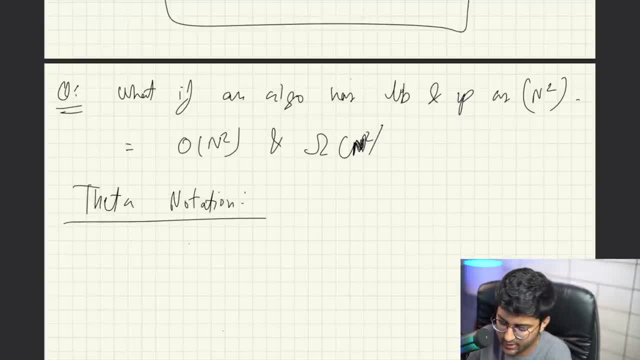 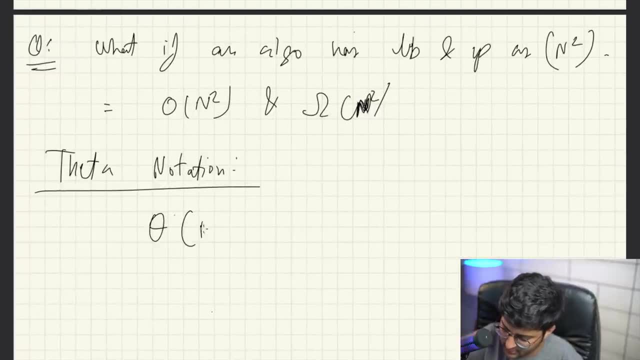 Jerry, considerably move on from here. therefore it is 3-theta of n squared, then we are going to closing from here. we have the little y of the方, the rest means we're going to closing the потому from suppressed. so we're going to limit. n tends to infinity, f of x upon f of n upon g of n, less than infinity, basically combining both. 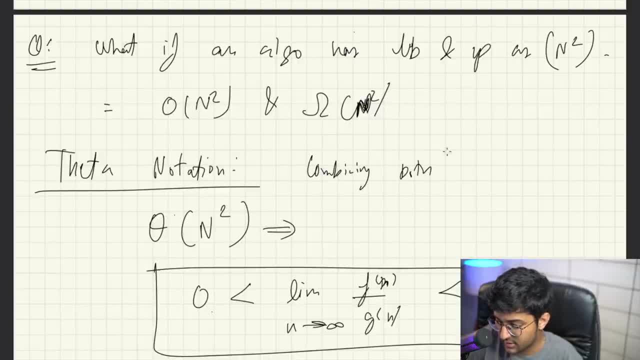 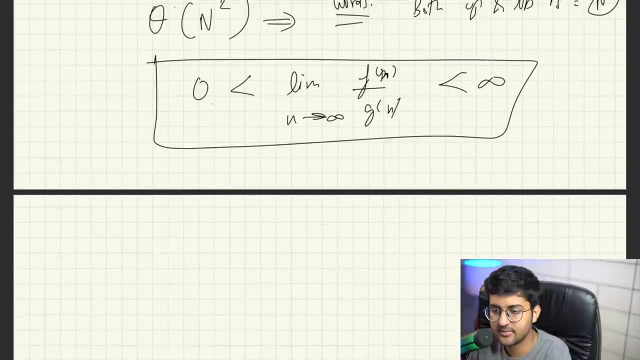 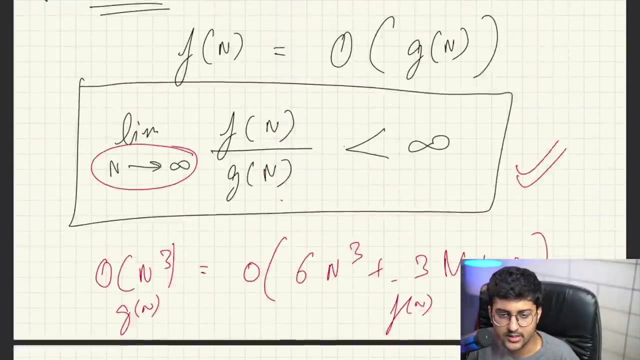 so it means that both upper bound and low- if you are in words, i can say both upper bound and lower bound- is equal to n squared in words, combining the both the formulas, that's it. very simple stuff, all right, but in reality we only consider because we're talking about the worst case. so we consider big O notation. 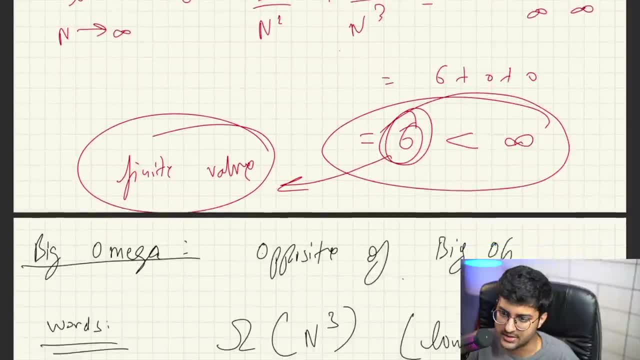 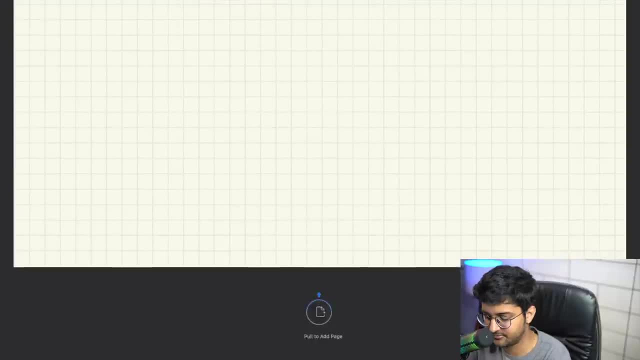 okay when we're talking about interviews and stuff, because you only care about what is the upper bound is right if you order. we have some use cases might be happen for this as well, but that's it all right. so i hope you were able to understand the complexity analysis now. we did. 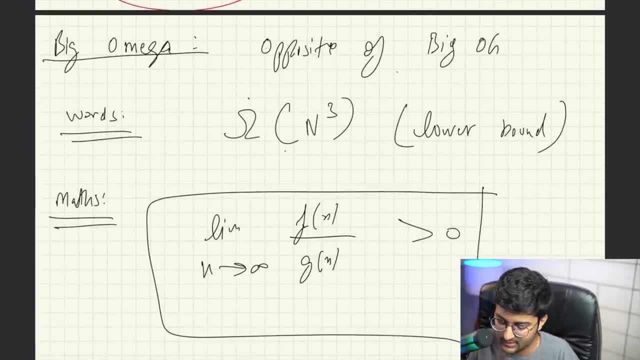 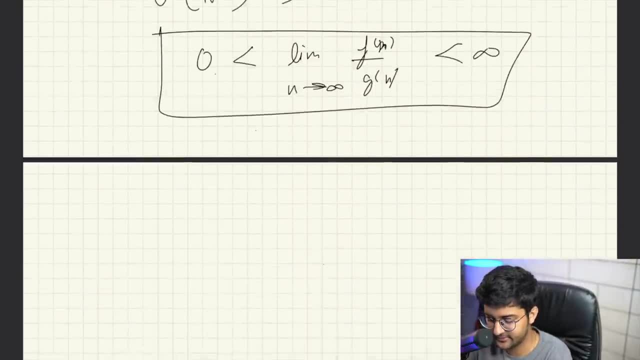 not skip anything. i literally told you everything you need to know about the complexity analysis. now, we did not skip anything. i literally told you in detail, you know, um mathematic formula, how mathematical formula is, read words, simple language. everything we covered. all right, there's one more thing, which is little notations. let's 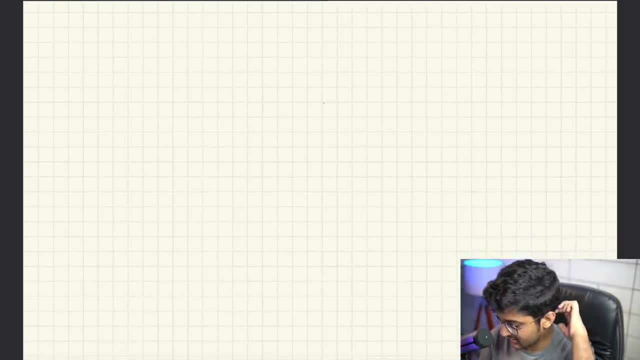 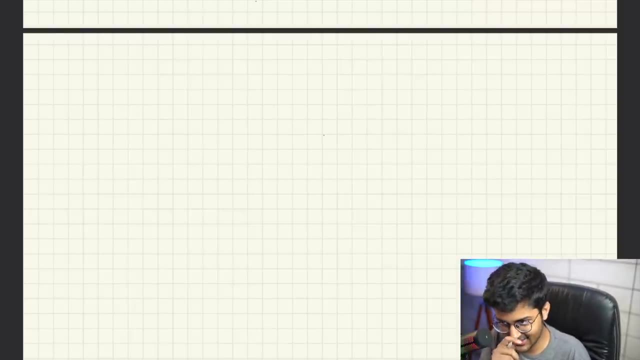 talk a little bit more about that. now let's look into two more. uh, so these are like the three main: big O, big omega and like the theta notation. but there's two more. there's like the little O notation and little omega notation. people don't get confused, it's very simple. uh, just 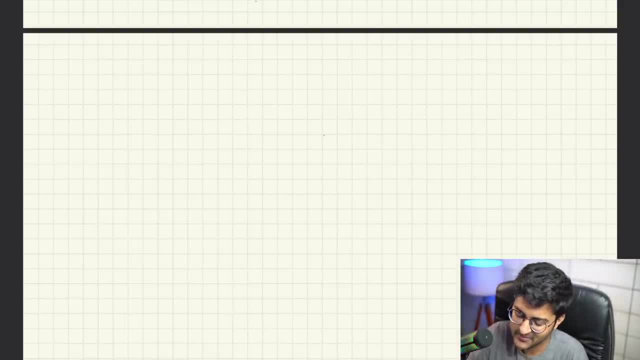 listen very carefully to what i'm saying and you will not get confused, okay so because i will explain in simple words. so little, little o first. okay, little o little o notation. so we know that the big o notation was giving the upper bound. this is also giving the upper bound. only this is also giving the upper bound. 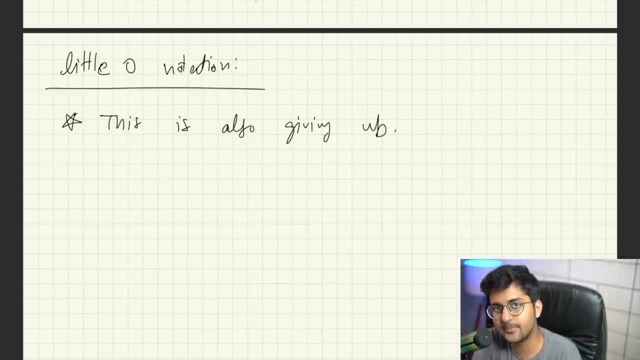 but what is the distance? this is not strict upper bound. this is not a strict upper bound in simple language also. i will explain. so basically, what i'm trying to say is in words: this is a loose. it is a loose upper bound. for example, in simple words, this is like: 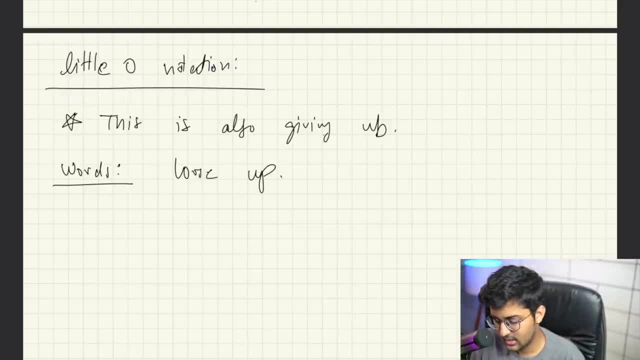 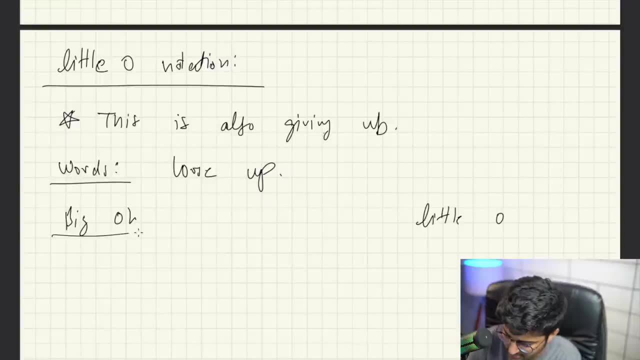 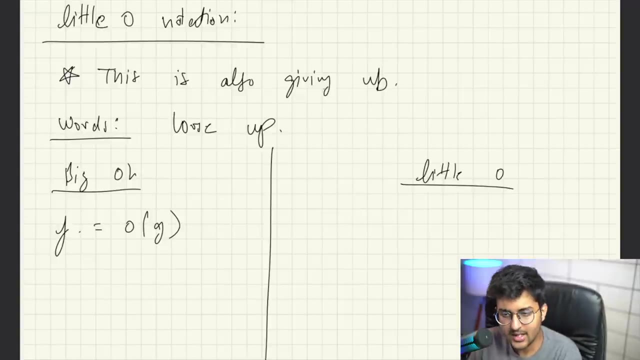 um, lose upper bound. so big o notation versus little o notation. okay, in simple words, in words, i can say: like big O and little o notation. okay, in simple words in words, i can say: like big O and little o notation. explain so if i'm saying f is equal to big o of g, it basically means that. uh, it basically means what? 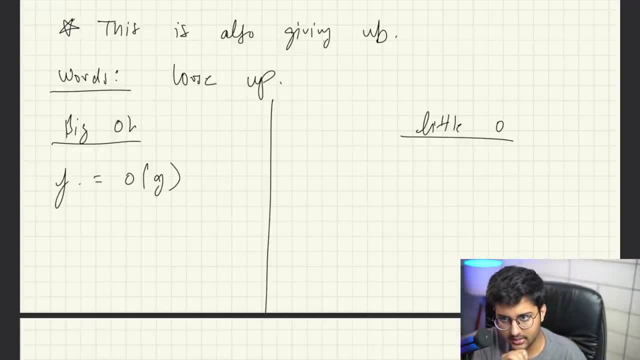 the growth of f is: uh. it basically means that the growth of f is no faster than g. okay, so basically i can say something like this. i can say something like: uh, growth of f is no faster than g. then i can say: it should be less than equal to g, something like this: 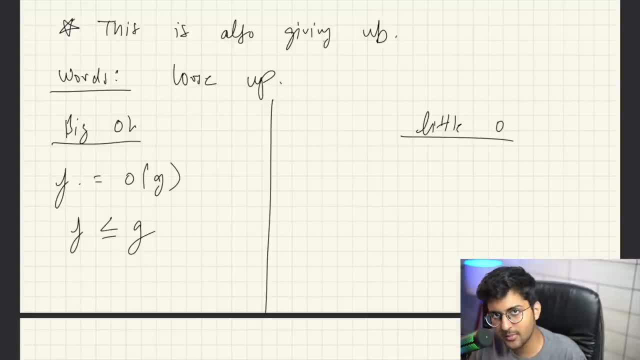 very simple stuff. it can be equal to g as well, but cannot be faster. on the other hand, this: if i'm saying f is equal to little o of g, it basically means that it is more like smaller than g, like this. that is what it means in simple terms. 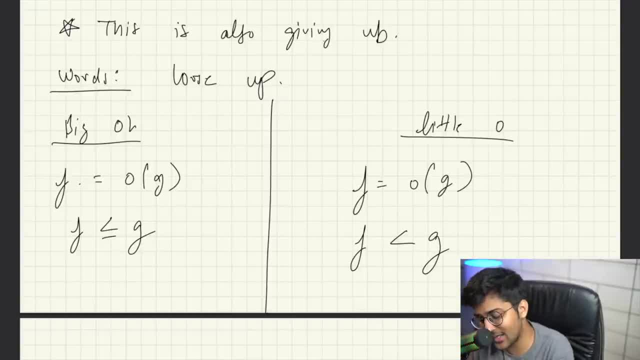 okay, strictly, strictly slower than g, strictly slower. that is the difference. so this is like less than equal to and this is just less than that's it. okay. so both are describing the upper bound, but this is a more stronger statement. i'll write it as in red: stronger statement. that is little o. 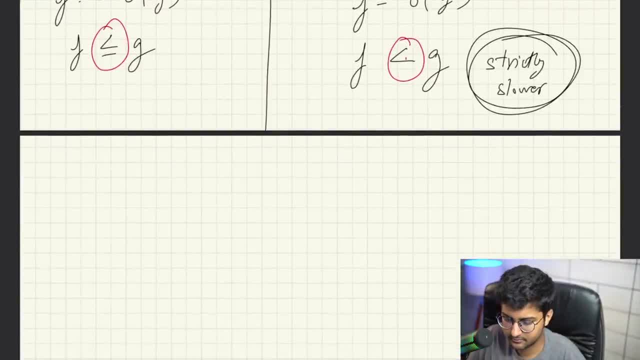 all right, mathematically it's very simple. in mathematically it's: uh, it's saying that it's strictly lower. so if you know, if i, if you're saying f is strictly lower than g, then you can say: numerator is lower, denominator should give you zero for infinite. so limit n tends to infinity. f of f upon g of n. 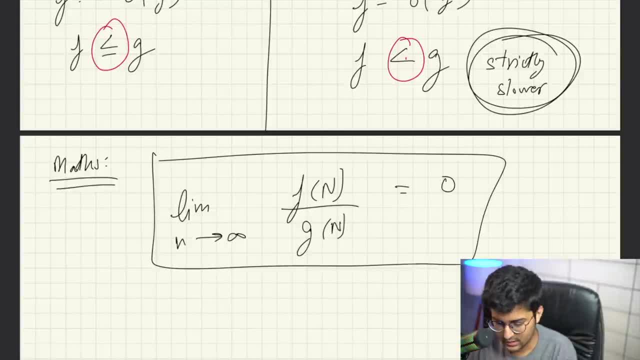 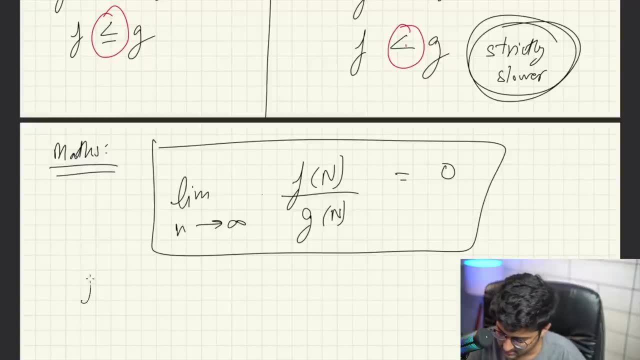 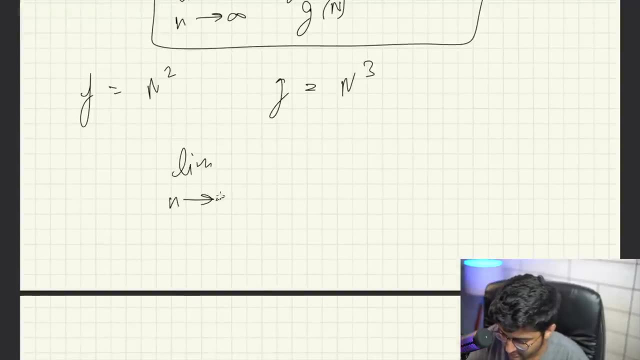 should give me zero. so if you can say: hey, um, you can say something like: f should be strictly slower than g, okay. so if i say: f is equal to n square, g is equal to n cube, and then i can say: limit: n tends to n is an example. n tends to infinity. you can say: 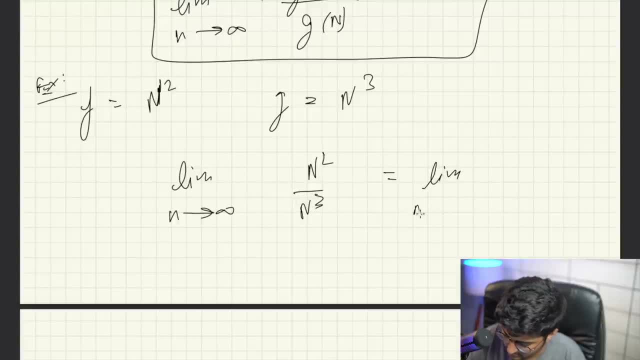 n square upon n cube. this is equal to limit. n tends to infinity, 1 upon n, which is equal to 0. very simple stuff, all right. that is little o notation. i think little o is equal to infinity, one upon n, which is equal to zero. little o is equal to infinity, one upon n, which is equal to zero. 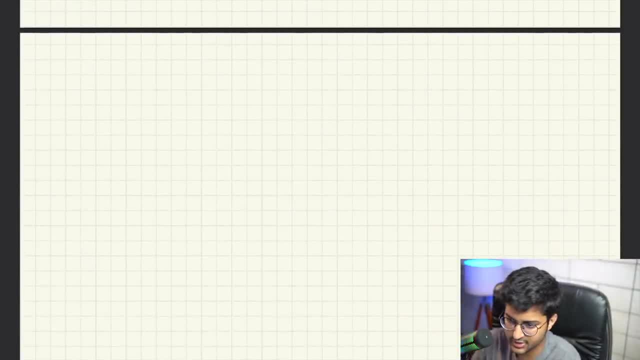 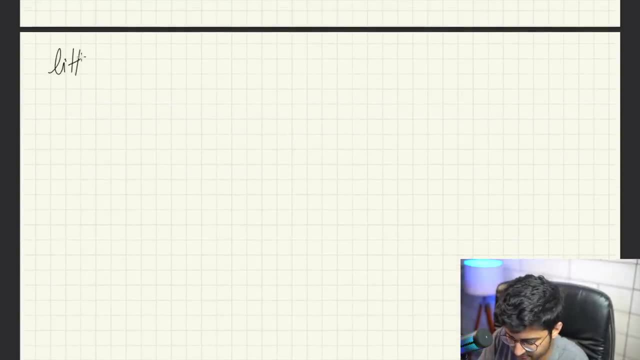 little omega is self-explanatory, so i can just write little omega notation as well. this is, uh, i think, self-explanatory. so big omega was giving the lower bound. this is also going to give the lower bound, but it will not be like tight, okay, so it's going to be like strict, uh, like loosely lower bound. 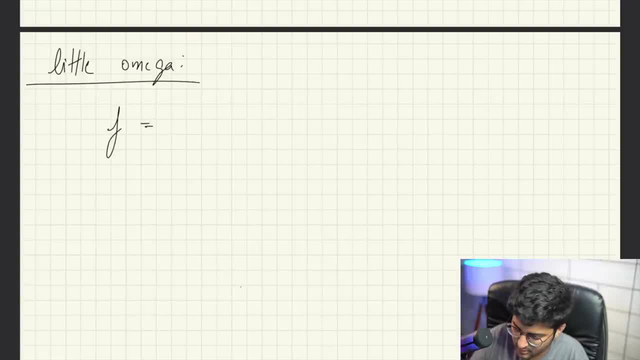 so if i'm saying f is equal to little omega of g, this basically means in mathematics that uh, you know it's going to be greater. so it basically means that. let me just write it in a clear way. just write it in a clear way in words. let's say: 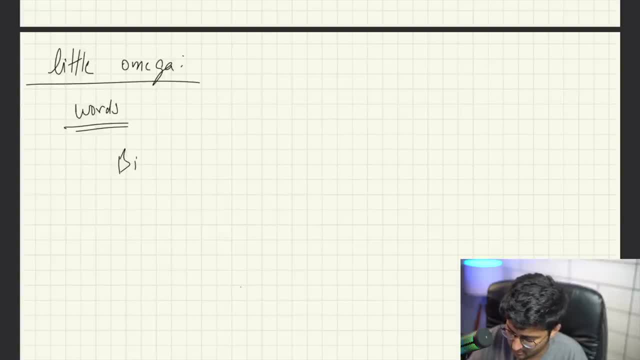 in words, if i'm writing, then big omega, little omega. so big omega basically meant that if i'm saying f is equal to big omega of g, this basically meant what this basically meant. f is greater than equal to g. it's giving a lower bound. it can, you know, increase more than that. this basically means: 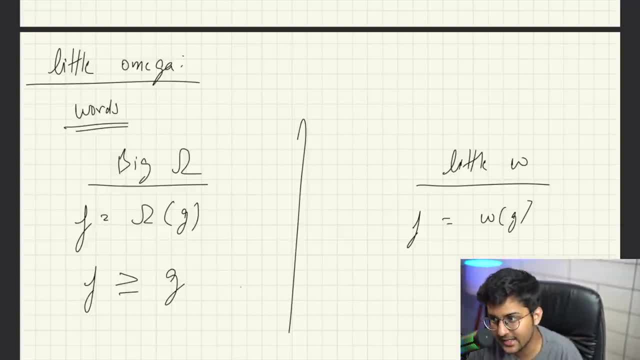 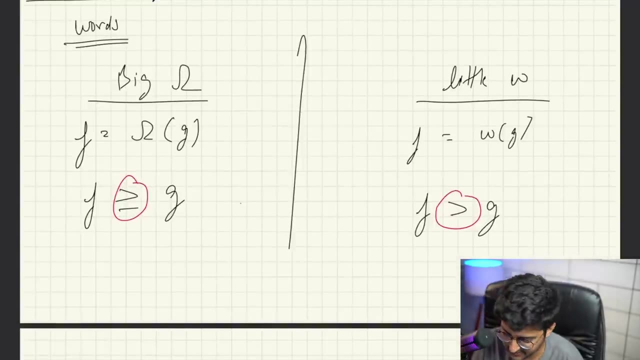 strictly, strictly lower bound means strictly greater. this is the only difference. okay, this is the difference. so this is the only difference. okay, this is the difference. this f is greater than g, then limit should be what should give me infinity if numerator is greater than denominator. so i can say in mathematics: 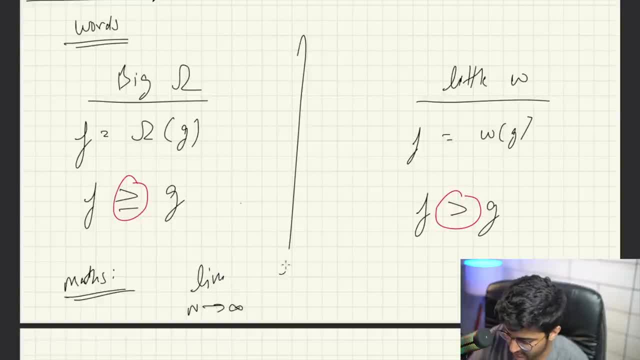 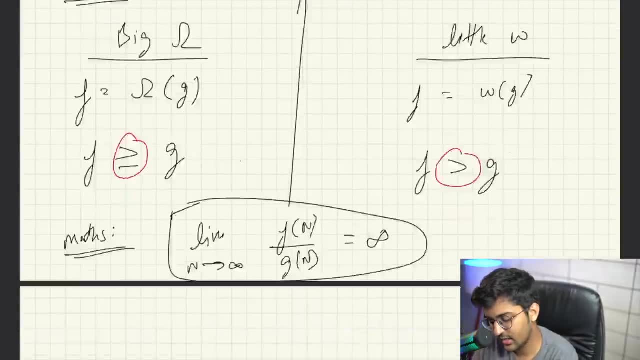 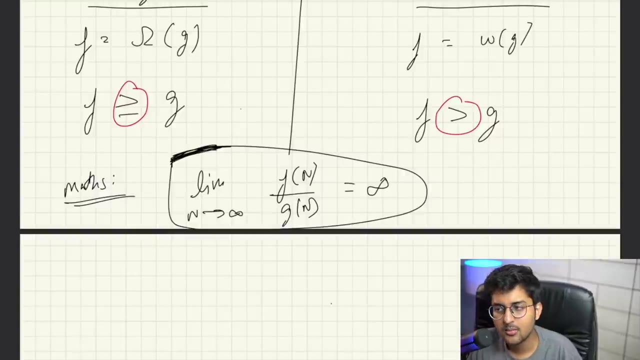 it can be something like limit n tends to infinity, f of n upon g of n is equal to infinity. okay, so when, when, when would you might want to use it when you want like something like strictly greater, 63, strictly less than or whatever, but in reality we use like for algorithms and com. 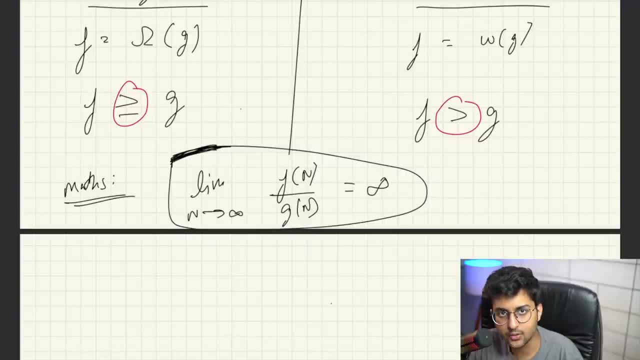 like in comparative coding and in your interview preparation and all these things, we use bigger notation only. this is just for general knowledge that i'm sharing with you. so example can be something like this: limit n tends to infinity. n cube upon n square is equal to limit n tends. 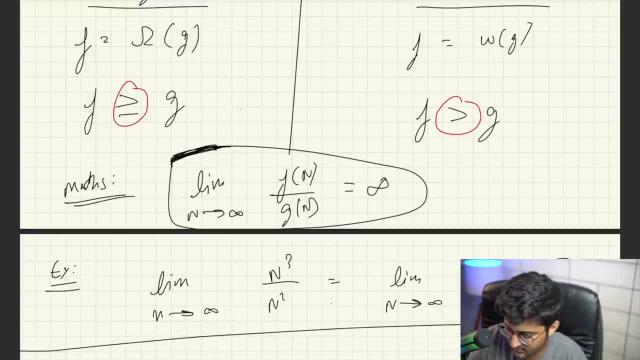 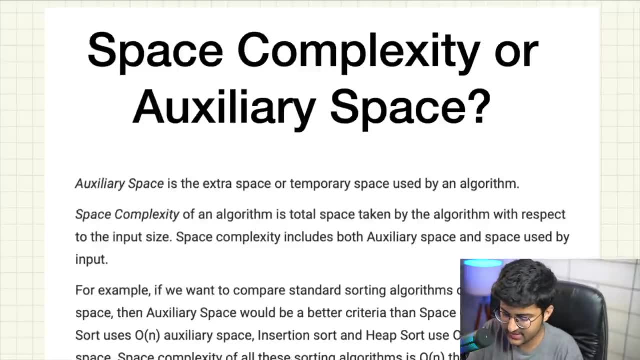 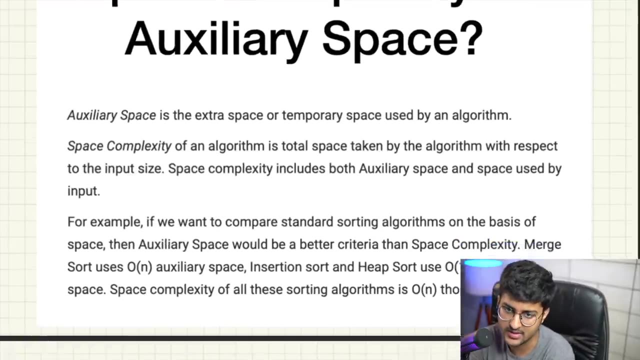 to infinity. n is equal to infinity. all right, very simple stuff, cool. let's move forward. let's talk about the space. complexity, or whatever it is, in simple terms, is equal to the input space plus the auxiliary space. now, what is auxiliary space? auxiliary space is the extra space or the temporary space taken by an algorithm. 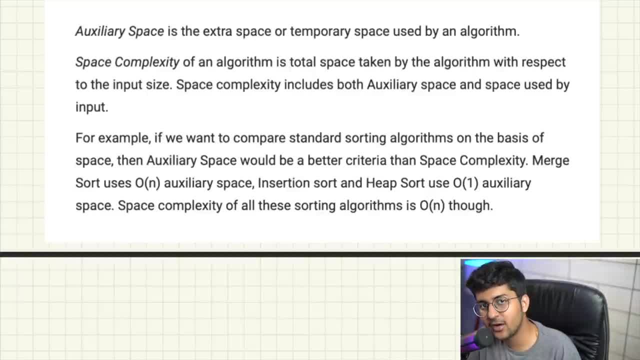 so if the question says: hey, take an input of array of size n, do something with it. so the space complexity is going to be the input that you are taking of size n plus the extra space the algorithm is using. okay, something like that. that is the space complexity. people often say that the 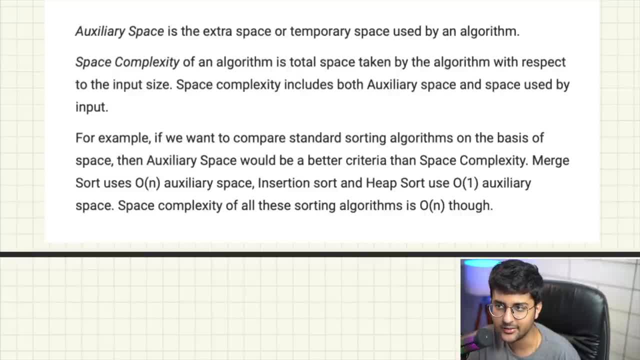 space complexity is equal to some, like you know, only the extra space that we are taking. that is wrong. space complexity is actually equal to extra space plus the original space that the input requires. okay, so when we are talking about interviews and all these things, we can't really. 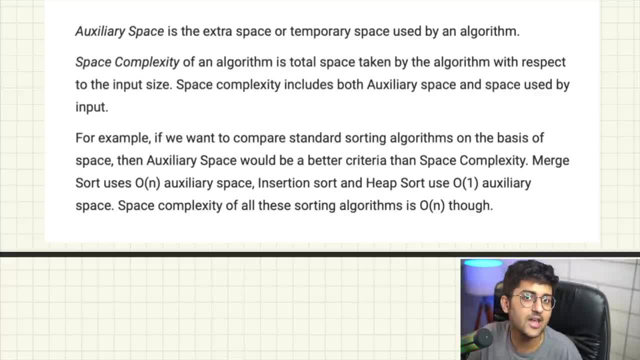 do anything about the thing we have to take input for. we only care about how much extra space is the algorithm using, for example when we were doing binary search. okay, so in the binary search the space complexity was constant. that means auxiliary space was constant. it was not taking any extra space. you may ask questions like: hey, kunal. 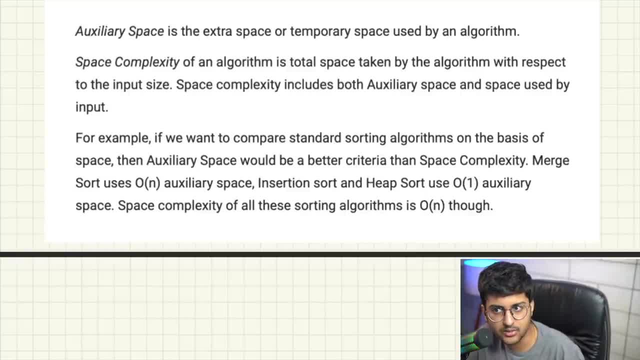 it was taking some extra space. you were taking some three variables: start, end and middle. you are taking these three variables. these variables also take some extra space. kunal, how can you say there's the space? complexity is constant. then think about it. if the array is, if the array is. 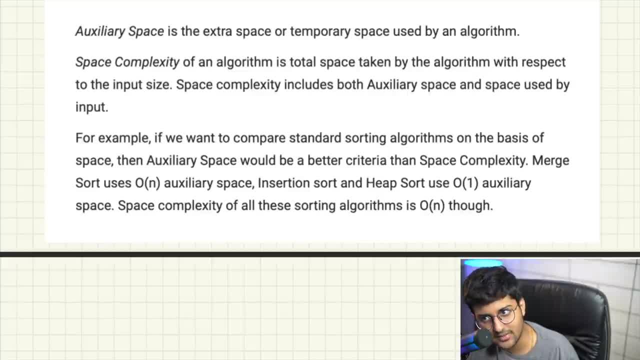 of size 100. if the array is of size one thousand, ten thousand, eleven thousand, two million, three million, every single time it's only going to take three variables, hence constant. okay, if you get a question like: hey, take an input of size n and uh, create a new array of uh size 2n. 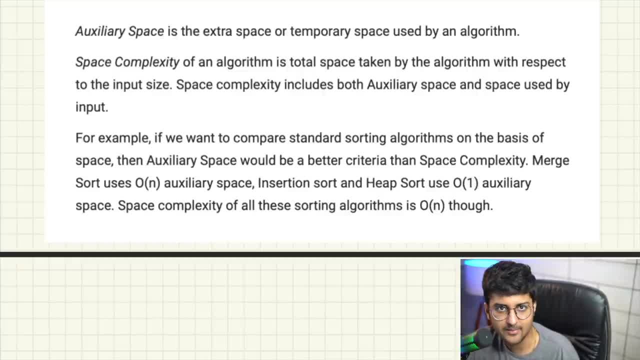 and add the duplicate numbers in it. in that case what is happening? space complexity is equal to n, which is this input that you're taking plus the entire. you know you will be creating another new array and in that you will be copying the old elements, then adding the new elements. so 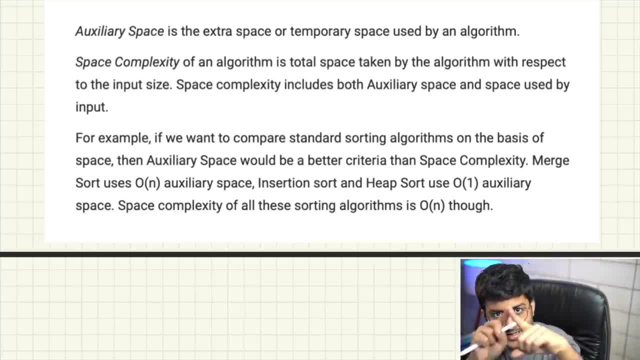 in order to solve the problem, a new array is created, and that size is actually dependent on the size n and space complexity is o of n. linear space complexity is equal to the input space plus auxiliary space, and we always talk about auxiliary space. okay, so, as you can see, merge, sort and heap. 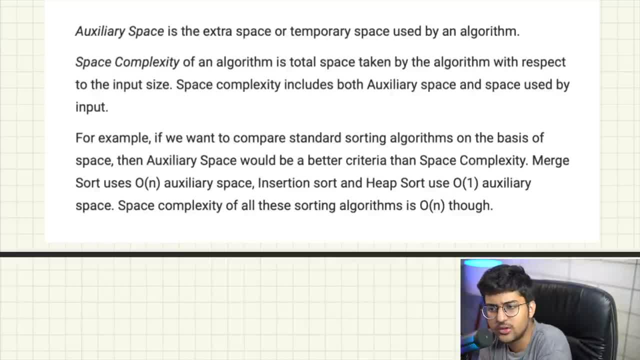 sort and all these other things we'll be learning about later on. so during that time only we will discuss the space complexity. so far we have done binary search, space complexity: constant, linear extra space or anything constant we have done. uh, we have done bubble sort- constant because it's. 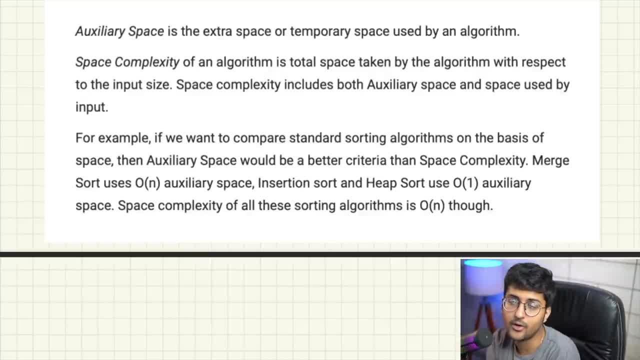 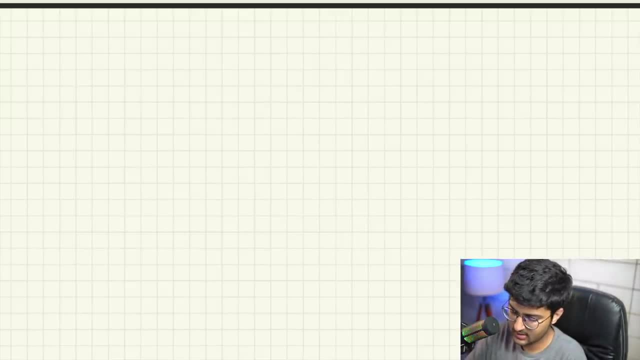 in place sorting algorithm. we're not making any new array where we have talked about uh, insertion, sort, selection, sort, count, sort and all these things. so all of these are taking constant space. complexity means no new arrays are being created. all right, now let us look at a question. okay, so the question says that you have a for loop like this, so you have something like: 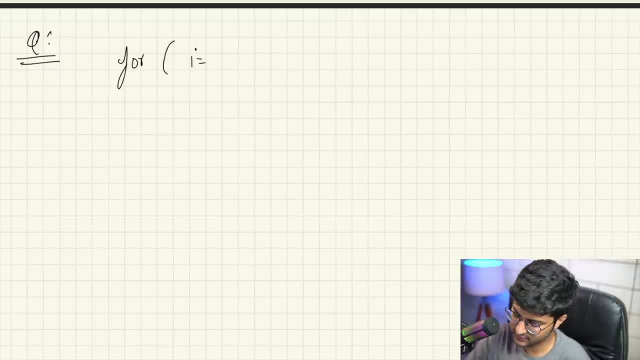 for i is equal to starts from, let's say, 1. i goes less than equal to n and it's not incrementing over here. let's say we have another internal for loop that is like: j is equal to starts from one. j is less than equal to some variable k and j plus, plus, okay. 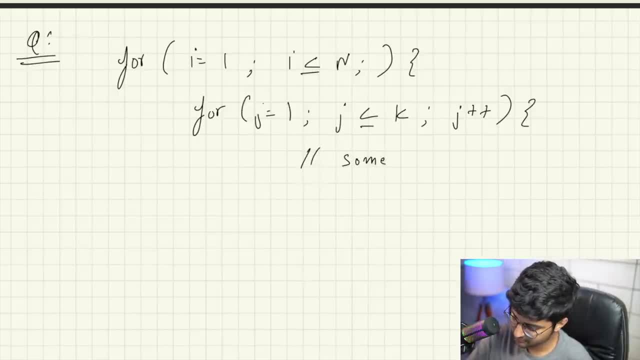 then you do some operation that takes time equal to t After this for loop has run. I am not doing i plus 1, I am saying i is equal to i plus k. That's it. Find the time complexity of this particular program, this algorithm. Pause this video, think about it, let us know. 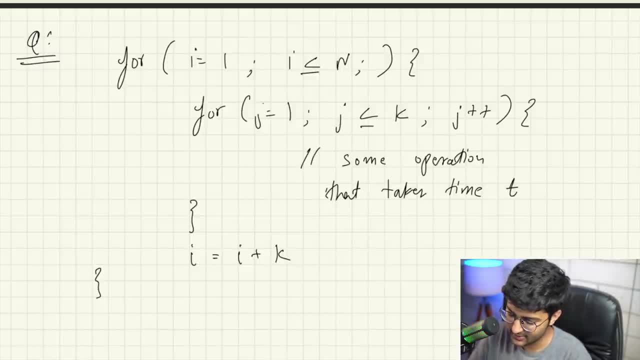 Now that you might have tried it, let me see how we can do this. What is time complexity? I know that this is taking some time t I just need to figure out how many times these loops are executing. I know that the outer loop is executing n times, So time complexity. 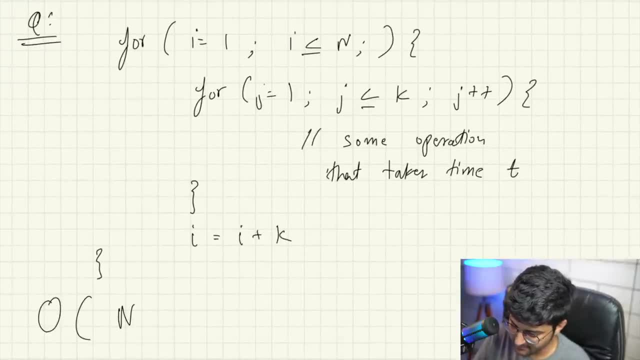 is actually equal to O, into whatever time the internal loop is taking. That is wrong. Outer loop is not executing n times because i is not equal to i plus 1, i is equal to i plus k, Hence this is wrong. Let's think about how much complexity the inner loop is taking. Inner loop, I can say: 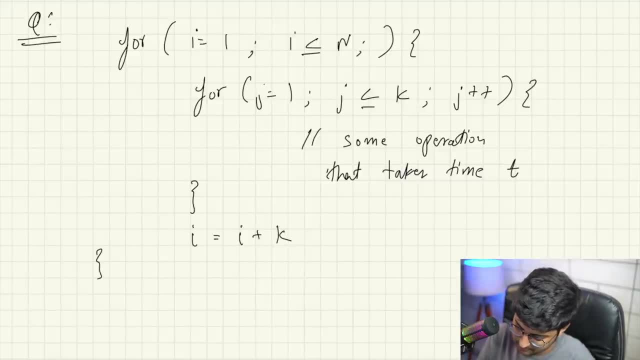 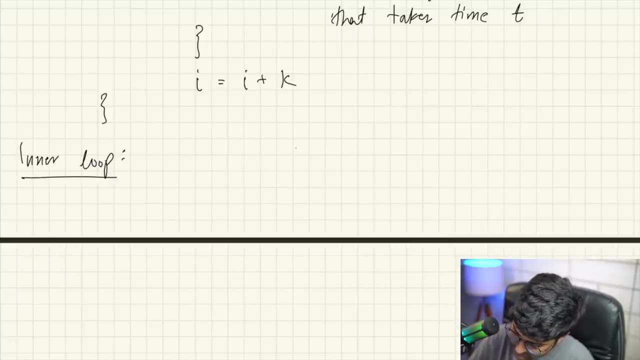 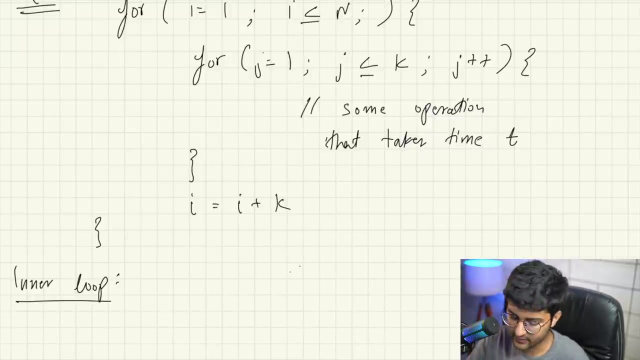 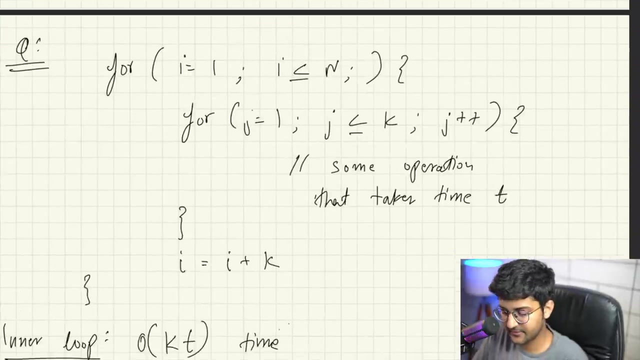 every time it is running k times. So inner loop, Inner loop, Inner loop is running k times and for every time it is running it is taking t t amount of time. Total how much then? k t time. That's it. We go off k t If inner loop is running once it is taking t. 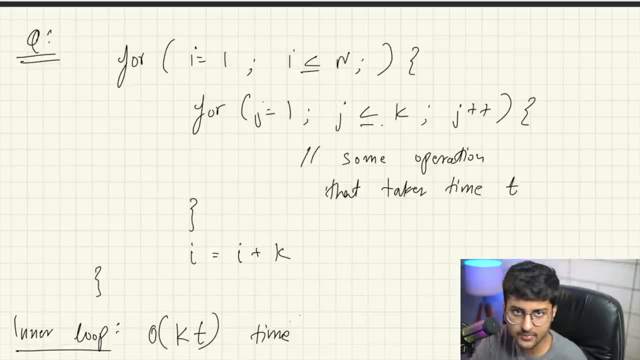 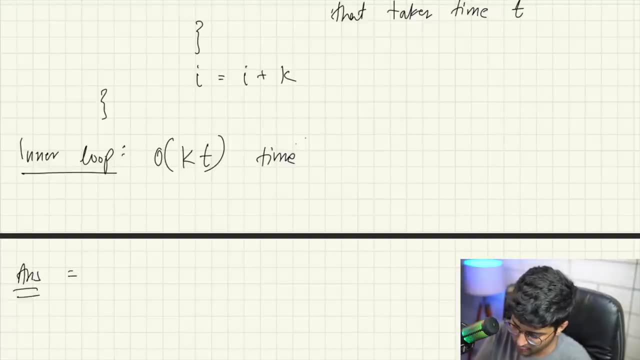 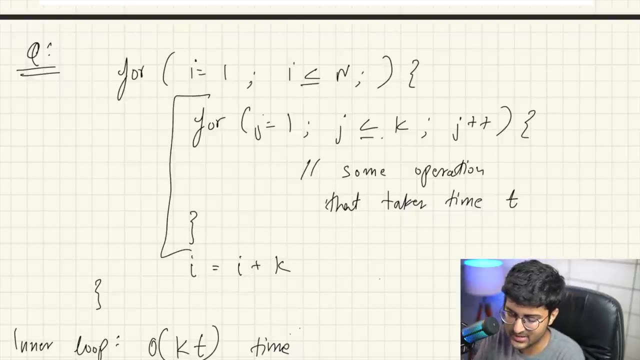 amount of time. So here I can see it is running k times, hence kt. That's it. So the answer is equal to what? So the answer is equal to what? So the answer is equal to what? to big O of KT, into how many times this entire program internal loop is running. 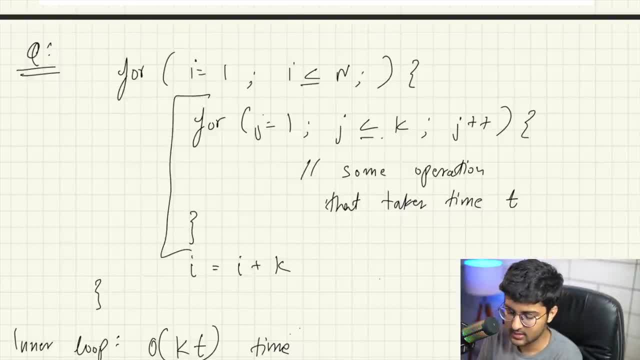 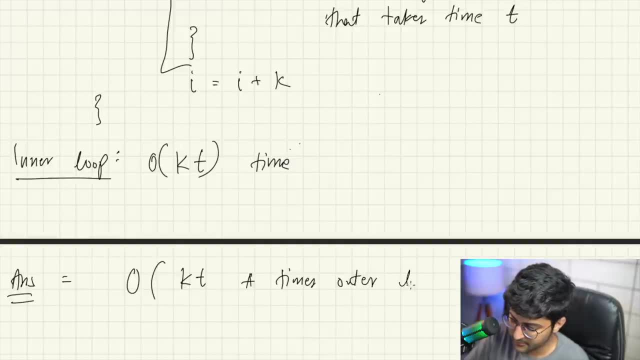 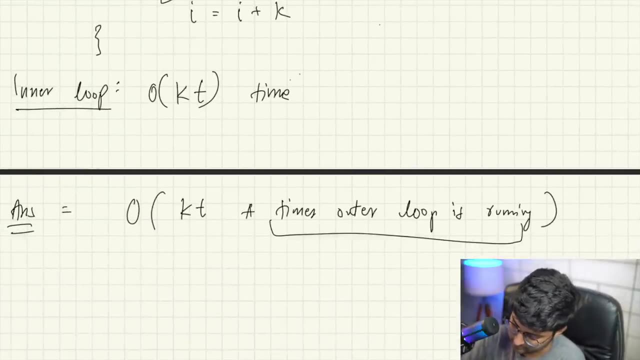 which is how many times outer loop is running. so KT into number of times outer loop is running. that's my answer: outer loop is running, how many times outer loop is, and that is what we need to figure out. this is something we don't know right now. okay, so outer loop condition is given to us. I starts from. 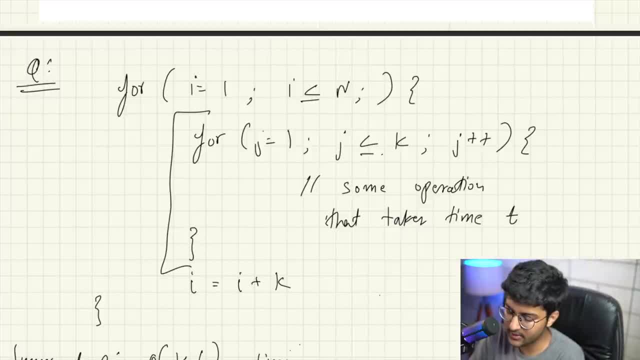 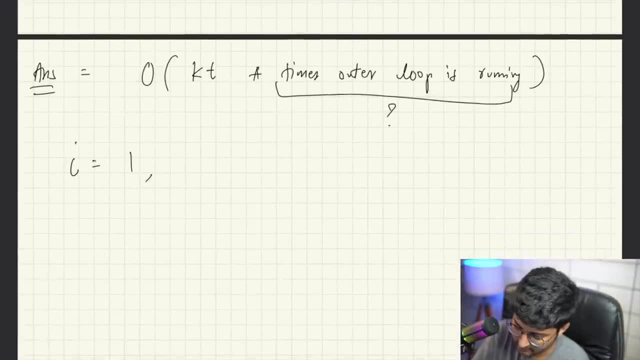 one, I. this loop will break when I is less than equal to n and I is incrementing with K. so let's say first the value of I is, let's say, equal to 1, then it will be 1 plus K, and then it will be 1 plus 2 K, then the value of I. 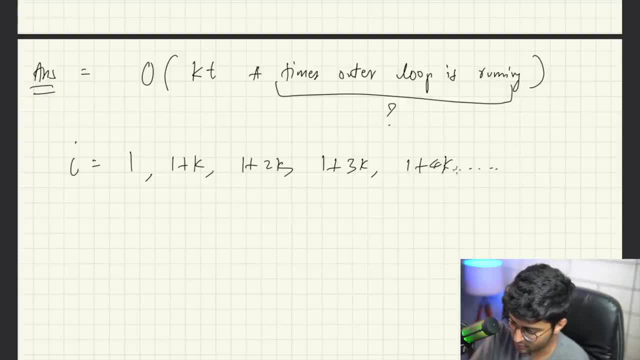 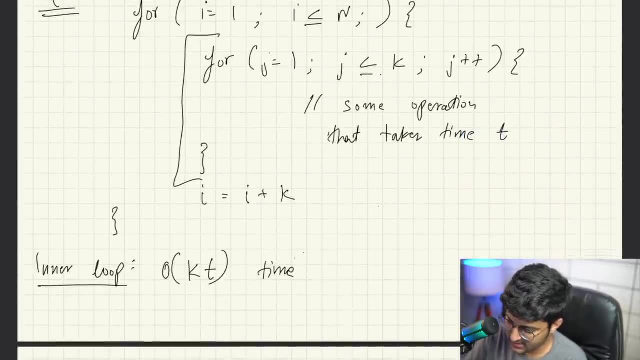 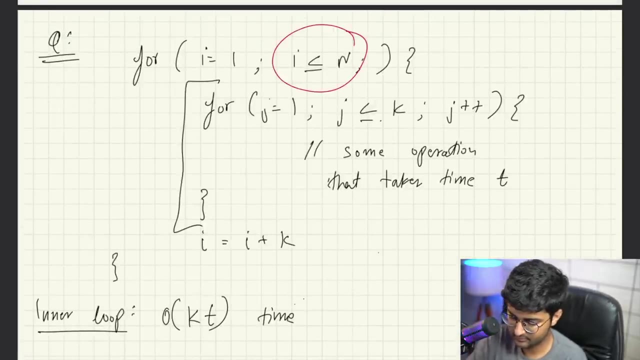 will be 1 plus 3 K, 1 plus 4 K, so on and so forth. in the end, the value will be, let's say, X. so I can say that if this last value is X, it means that this X is the last value that is satisfying this condition, can we not say that? hence I can say that X. 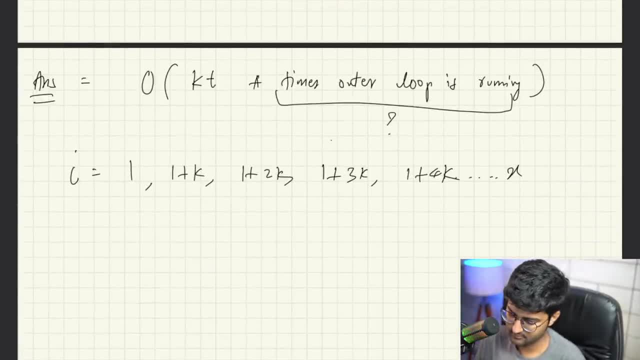 should be less than equal to n. we can say that okay. or I can say something like this: this is loop running 1 times, 2 times, 3 times, 4 times, 5 times. so I can see it's actually running. if I'm saying at the end, it's actually going to be running how many times, let's. 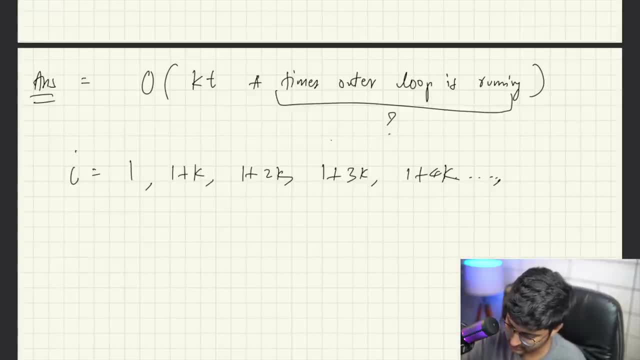 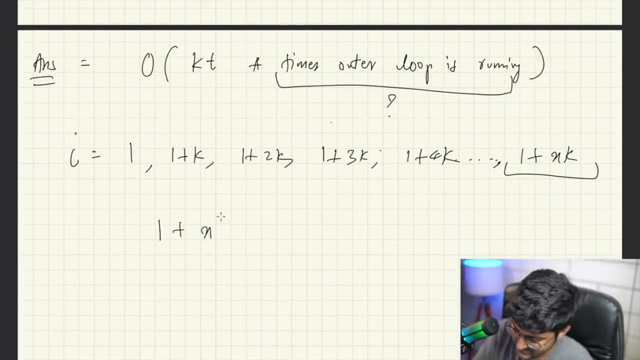 say this is after once, after twice running the third and fourth. then I can say something like: let's say it's running 1 plus X, K times and this entire value should satisfy this value, this particular condition. so I can say 1 plus X, K is the number of times you know the value and X is actually the number of. 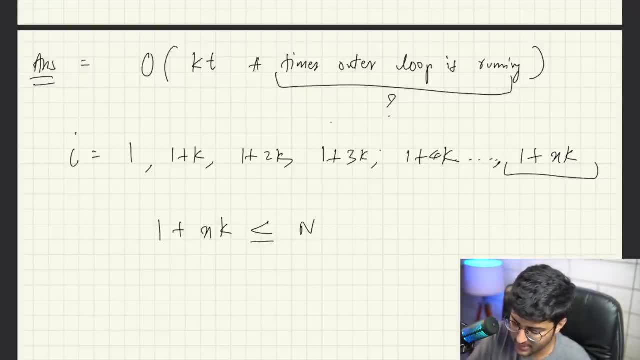 times it's running or something. it should be less than equal to n. okay, I can say X. K is less than equal to n minus 1. I can say X is equal to n minus 1 upon K, since this is the last value and this X is equal to. 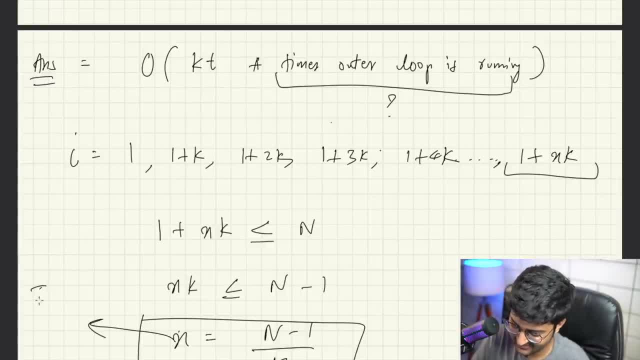 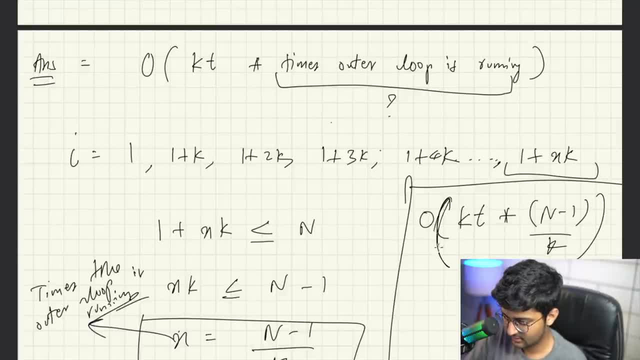 minus 1 upon K, the time complexity, right. so this is equal to what K and K gets cancelled. this is equal to like. also, we ignore the constants, so constants are removed. so this becomes big go off, big go off in, and this is equal to radio I né. 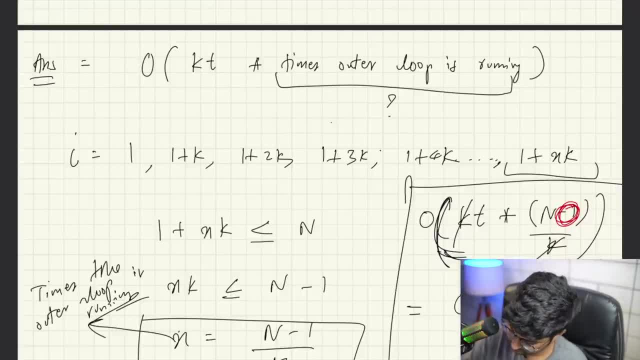 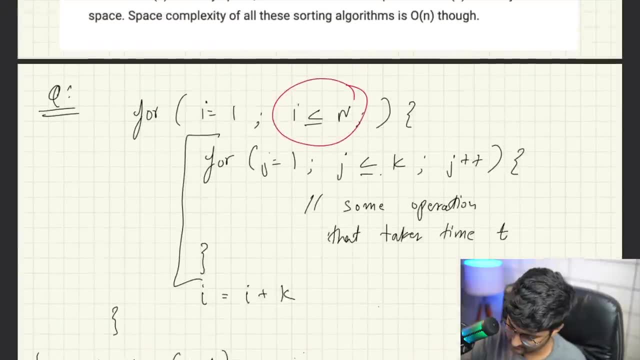 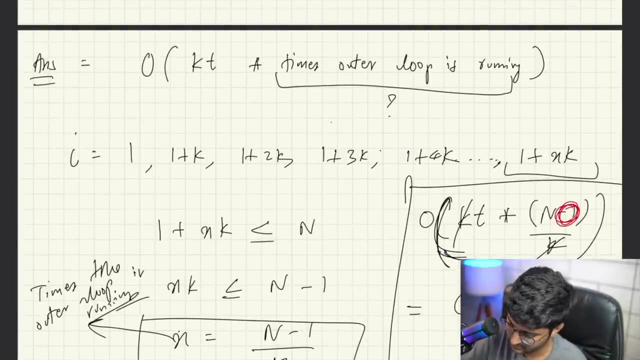 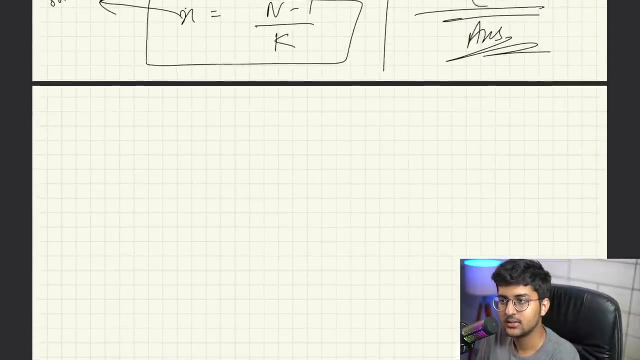 into t, big o of n, into t and t is some operation taking some time t. so i can say some operation that takes time t. this is constant. i can say big o of n or something. i can say n, t. no problem, that is my answer. that's the answer. very simple stuff, cool, all righty, let's move forward. now let's do a recap. 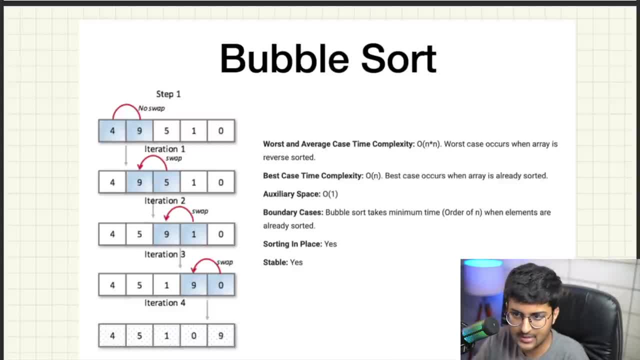 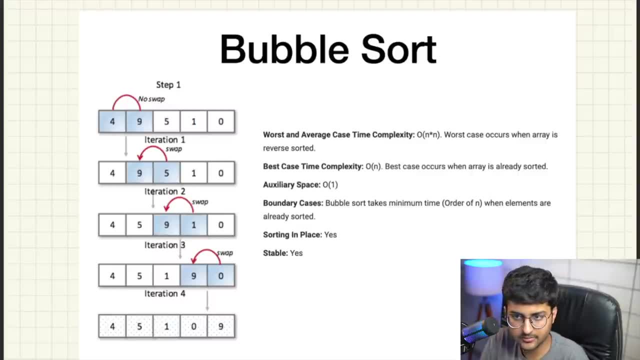 of all the sorting algorithms we have done already. so i know we have already done bubble sort. we know we already went through the complexity of it. in the worst case- average case- we can say that it's n squared and best case is o of n which is already sorted extra. 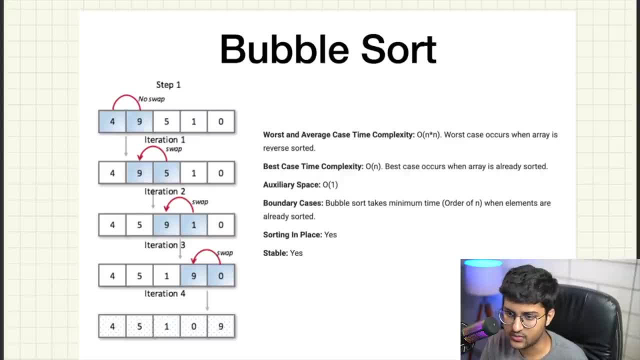 space means auxiliary space, which is constant, and all the things we have already covered. so if you want to look at the in-depth explanation of how we figured out the bubble sort algorithm, complexity and everything, check out the link in the description below. there's a video on that called bubble sort. 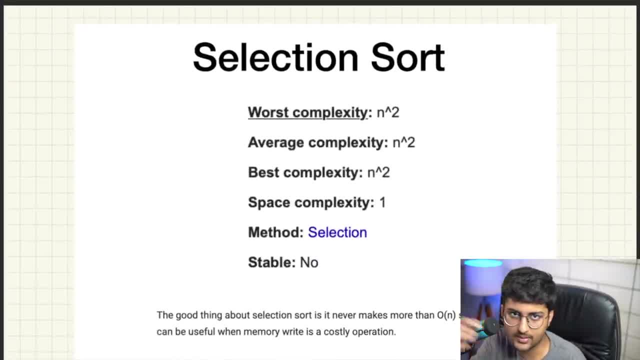 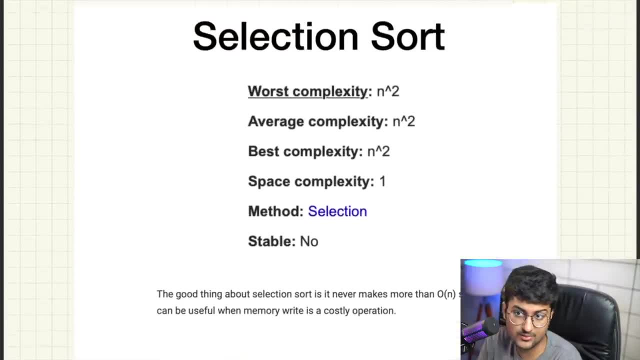 next one is selection sort. we've got this already as well, so we select an element, put it at the end. okay, so we've done this already. so, um, we've covered in details about this. i'm not skipping anything. advantages of these algorithms, comparison with different algorithms- everything is covered in. 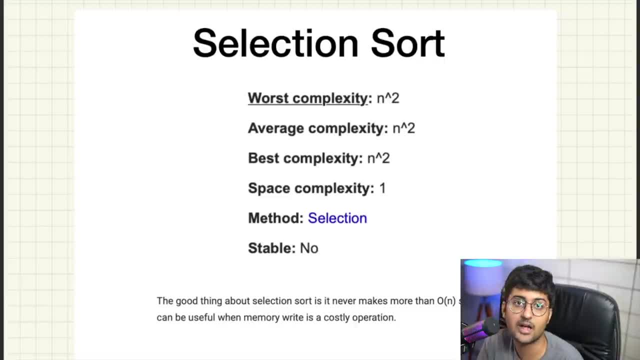 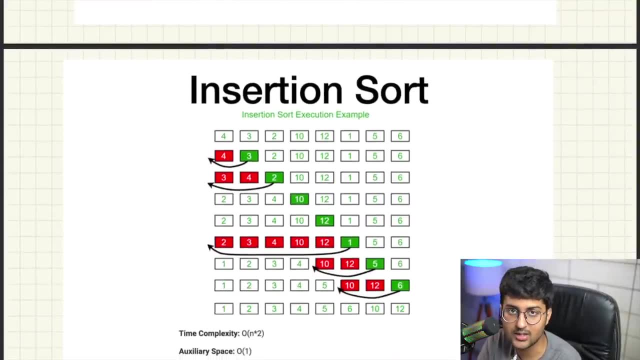 detail r and r long videos specifically on these topics i have made. please check out the link in the description. in that video we have also covered the complexity and i told you- i will explain in detail- what is big o or whatever. in that case we were talking about the number of comparisons and stuff. so that is similarly what we're doing over here as 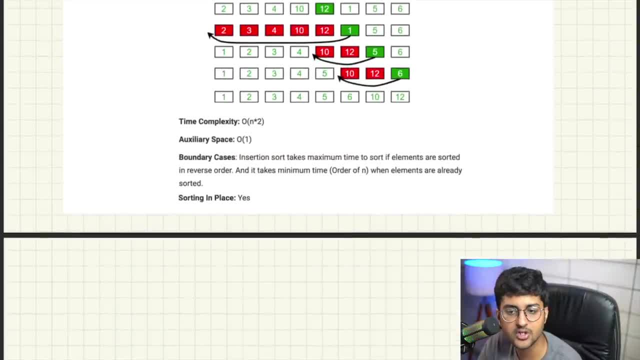 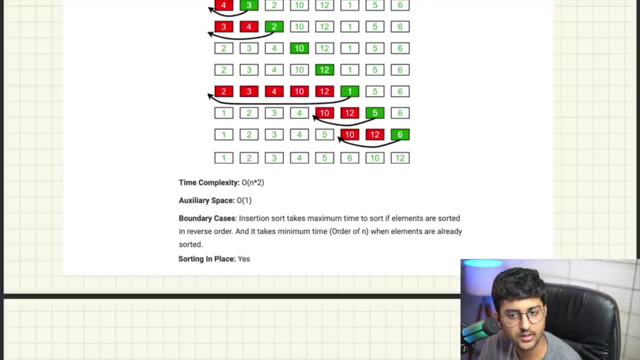 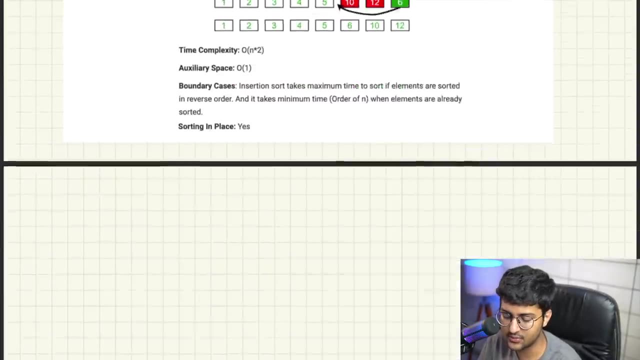 well, okay. similarly, insertion sort is given over here for your revision. okay. sorting in place basically means like no extra space is required, hence extra space, auxiliary space: constant complexity is constant complexity is o of n squared boundary case and everything is mentioned over there. so if you want to revise how these algorithms work, make sure you check out the link in. 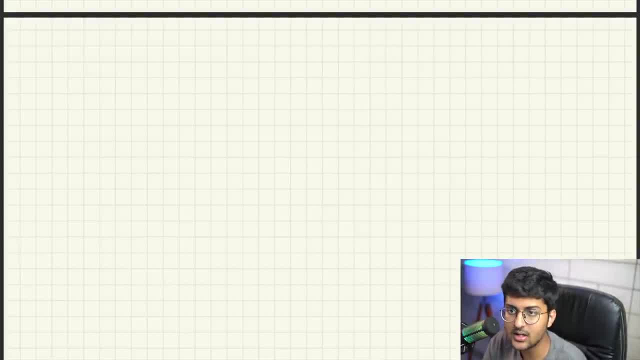 description. i made videos on this already. there's timestamps provided as well, so it will be easier for you to navigate as well. let's talk a little bit more about now. now we're talking about the important. one of the most important parts of new new section is starting now. pay attention. 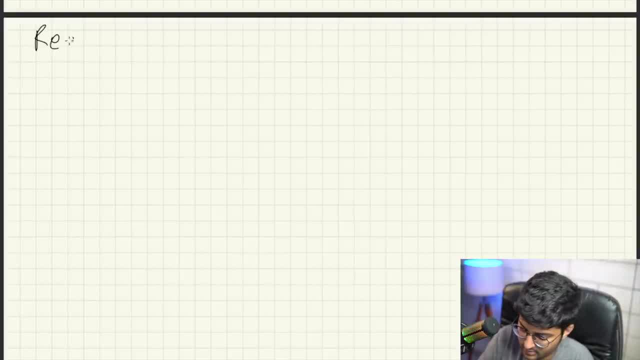 so we're talking about recursive algorithms. recursive algorithms- this is like an entire section, starting right now, on complexity and analysis of recursive algorithms. let's talk. look, take a look at the fibonacci example that we did previously. okay, so i say, if the favorite fibonacci number is equal to what? something we have done already in detail. 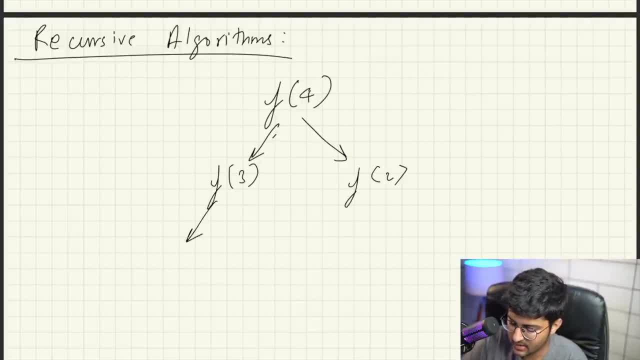 check out the previous recursion video if you are not aware of this thing. so this tree we drew over there. so already we made it right: f of one, f of zero. this is going to call f of 1 and f of zero. so my question to you is one thing i want you to notice when we're talking about recursive: 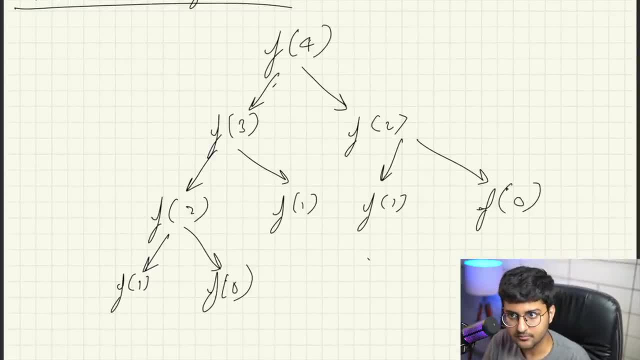 algorithms. let's first talk about the time complexity. okay, in this case it's taking. obviously, time is going to be taken for every single, for every single um function call, because all the function calls are getting evaluated. okay, so we are going to take everything in consideration. that's simple how we are going to take that. what is the time complexity actually? 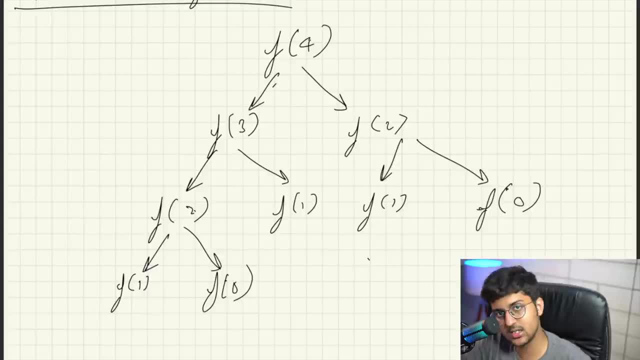 going to be and whatever that will look into the future of this video. like in this video only, i want to focus on space complexity. can anyone tell me what is the space complexity of this algorithm? what is space complexity? is it going to be constant in recursion programs? 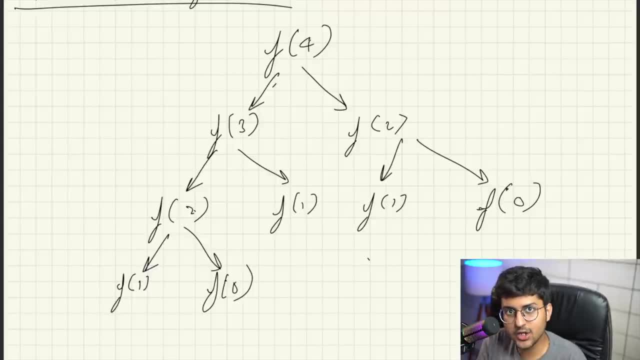 no, why? because in recursion you know that function calls are stored in stack. those function calls actually take some memory in stack. hence recursive programs do not have constant space complexity. then what is the space complexity over here? can you see that? what do we mean by complexity? please listen very carefully. very important point, otherwise you will get doubts. 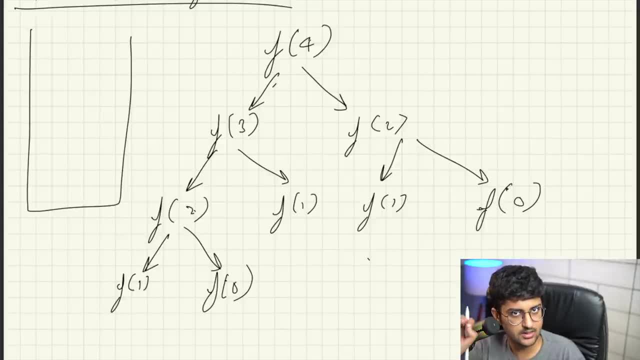 space, complexity of recursive programs. i'm going to tell you some points. this is very simple point, but i will tell you like in a very structured way, so please listen to it and repeat it yourself many times. point number one: when we talked about the flow of recursive program, do you think that at any particular level, if i take any level, let's say: 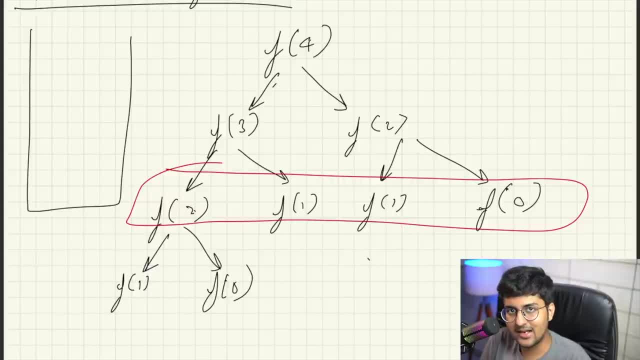 at any particular level. if i take any level, let's say at any particular level, let's say at any particular level, i take this level of recursion tree in this level at any particular point of time, in this level or any level you take of recursion tree, is there going to be a possibility for more? 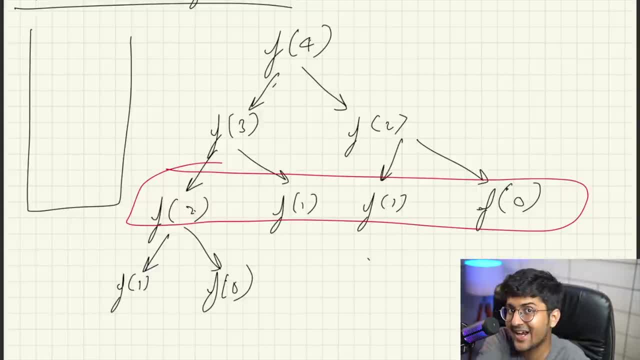 than one function calls in this level to be in the stack at the same time? can i say that this function call and this function call and this function call, or let's say, this function call and this function call, are in the stack in the same time? can i say that no, because this will not. 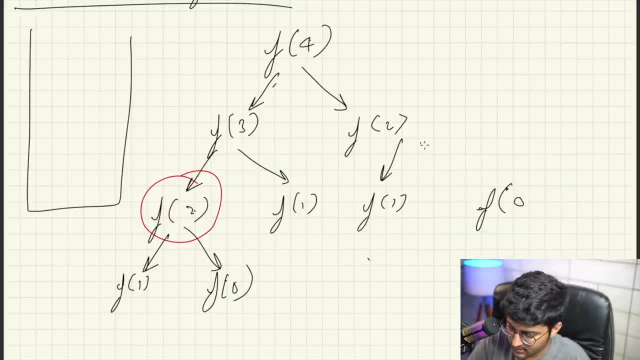 even execute. this will not even execute till this has finished. if i want to look at what is the, you know what is the flow of execution: first this will execute, then this, then three, then four, then five, then six, then seven, then eight, then nine. so this seven, eight, nine, for example, will only execute. 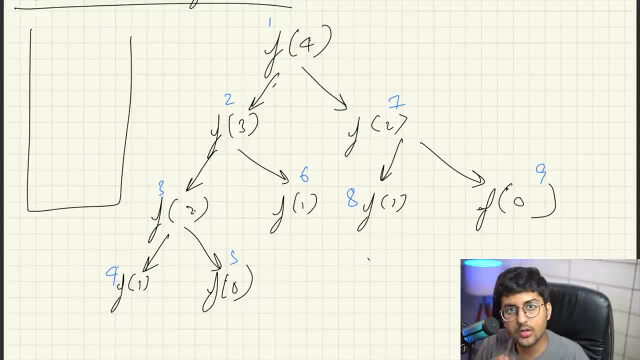 when the answer of three is given to us. if you are not able to understand it, then i will tell you the reason why you are not understanding this number one: you did not watch the recursion video. that's the only reason you are not understanding this. right now, everything in detail flow and 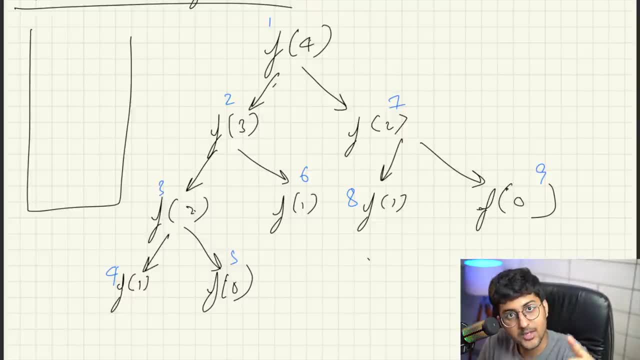 everything, how to understand the program and everything is covered over there. make sure you watch that video. that is the reason i did not make time complexity video in the initial days, because the recursion was important to understand this. okay, so in simple. what am i saying in simple? 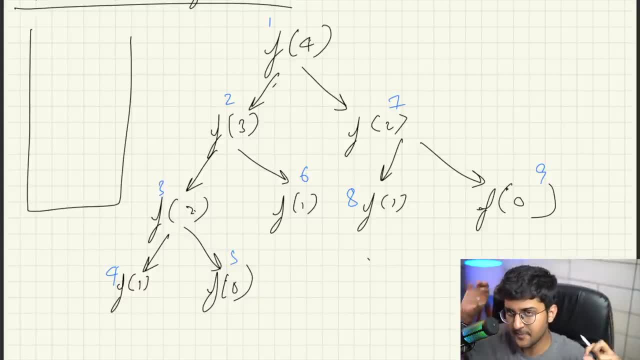 i will repeat it: code starting right now. code starting right now, at any particular point of time, with the common sense that we have already seen, you know the flow of program. we've already derived it. at any particular point of time, no two function calls at the same level of recursion, no two function calls at the same level of recursion will be in the stack. 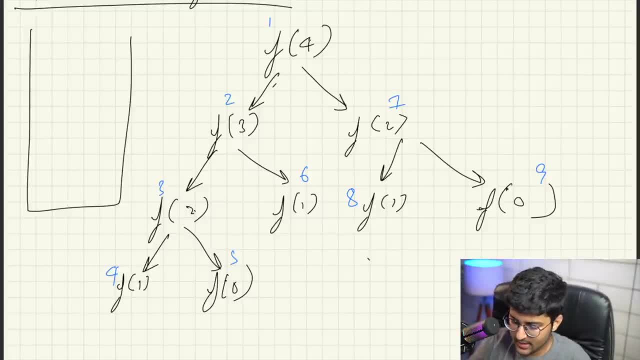 at the same time. it can be possible that one simple trick, trick, trick. what is the trick? to remember this: only calls that are interlinked with each other will be in the stack at the same time. interlinked will be in the stack at the same time. why? because very simple: in the stack. 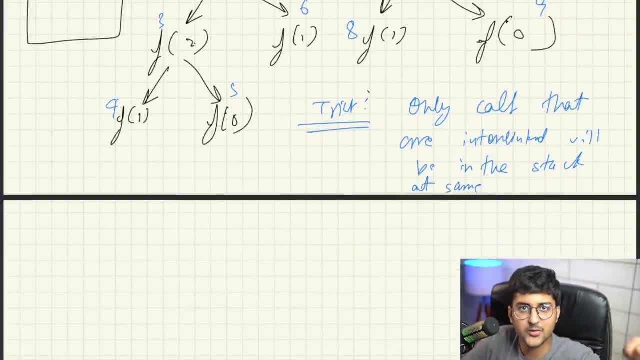 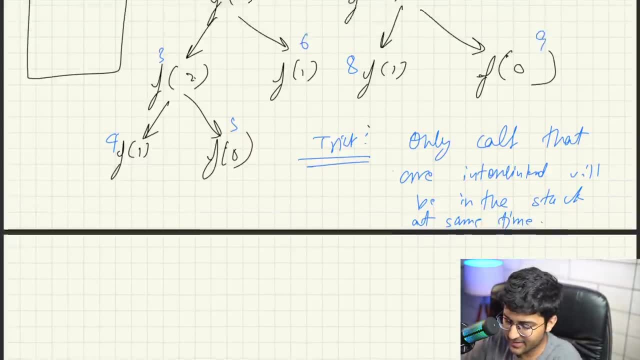 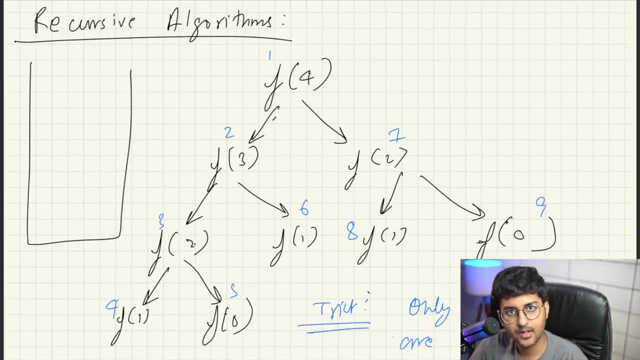 at same time because the previous one will be waiting for the next one to execute, next one will be waiting the next one to execute. these should be interlinked together same time because, for example, when function call number seven is executing, two, three, six, four and five have already finished. so if i'm talking about function call number seven, 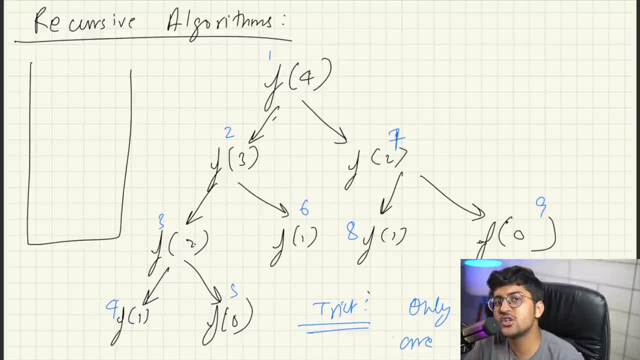 from this diagram, can you tell me which all function calls have already executed: two, three, six, four and five? why? because these are not linked with seven, for example, if i talk about linkage. so let's say, starting from here, these all function calls will will exist in the stack at one particular point of time, like this: 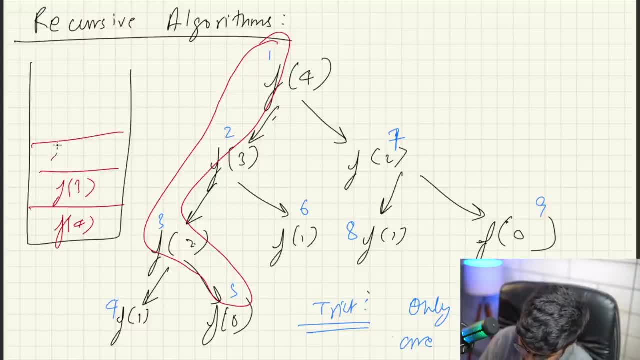 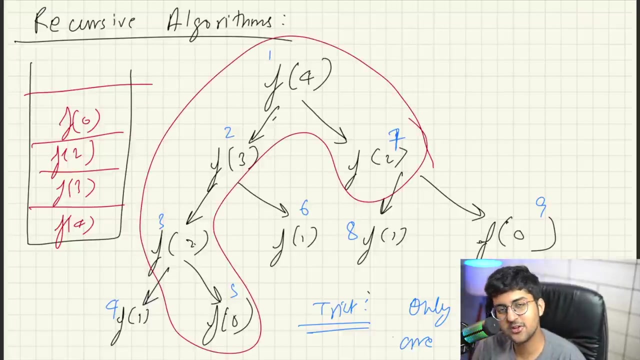 f of four, f of three, f of two and f of zero. this is possible. this is possible why? because these are all interlinked together. okay, and this should also be in a direction. it cannot be like you're doing something like this. it can't be you're interlinking something like this. that's not possible. 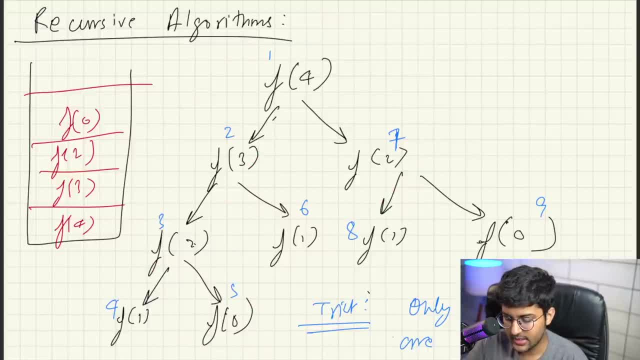 because now it's going up then down. that's not possible. it should be in just one flow. in simple terms, at one particular level. at one particular level, there will not be any more than one calls that are in the stack at the same time. so what is the maximum space that we will be taking? 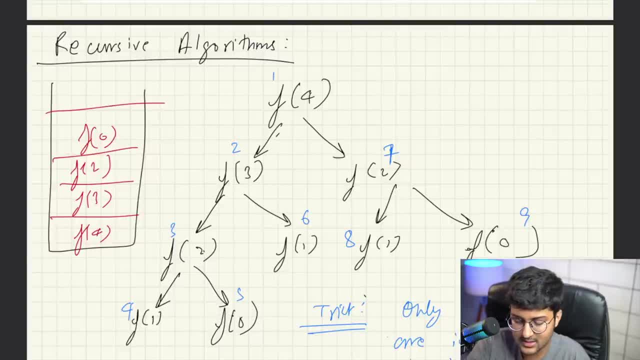 is it possible that all the nine function calls will be in the stack at the same time? no, no, we know that the longest chain, starting from the root till the leaf, starting from the first till end, leave whatever this or this or whatever, the longest chain. that is the answer. so space. 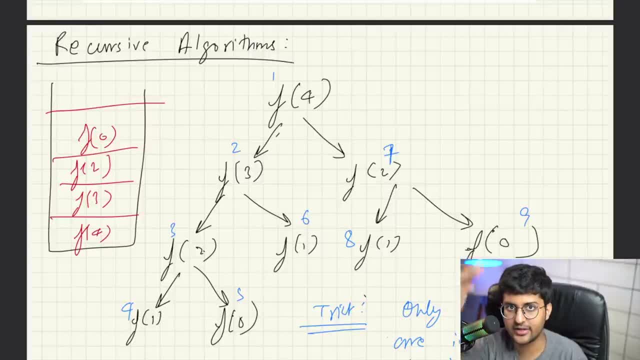 complexity is equal to the. the height of the tree, recursion tree, height of that is equal to space complexity. this is the space complexity. and what is this? equal to total number of elements in this particular program. how many do we have? if n is equal to 4, we have 4. space complexity auxiliary. 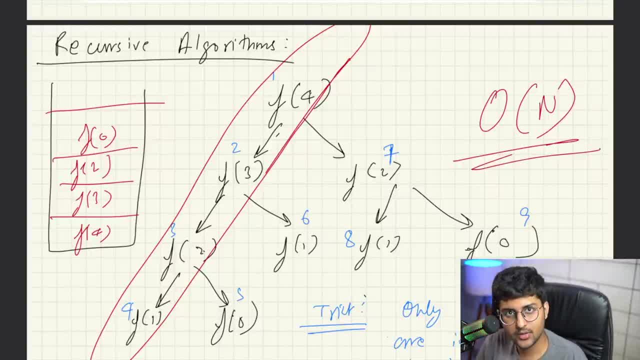 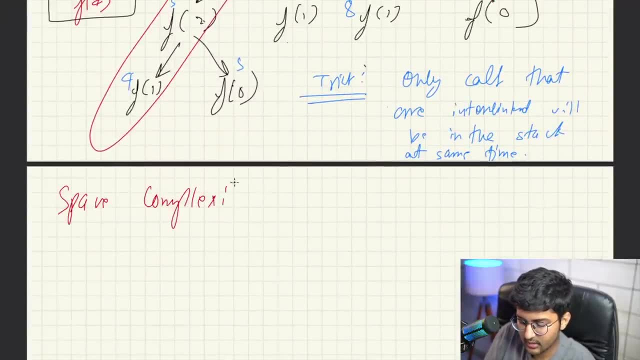 space is o of n in this case. i think you are able to understand. so, space complexity of recursive programs. very simple solution: space complexity is equal to height of tree. height is equal to the path, the path of tree, total number of nodes, or this these calls in path path. 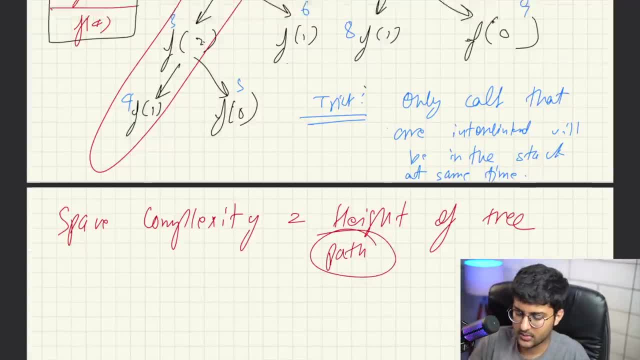 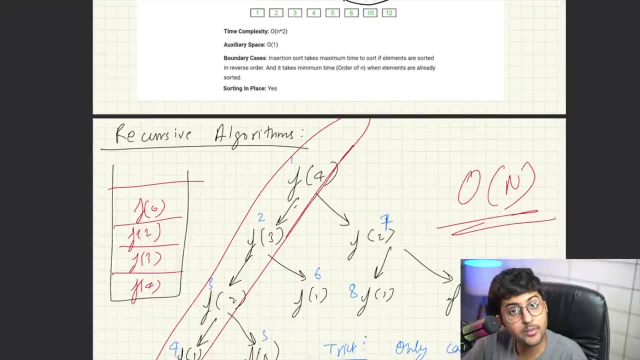 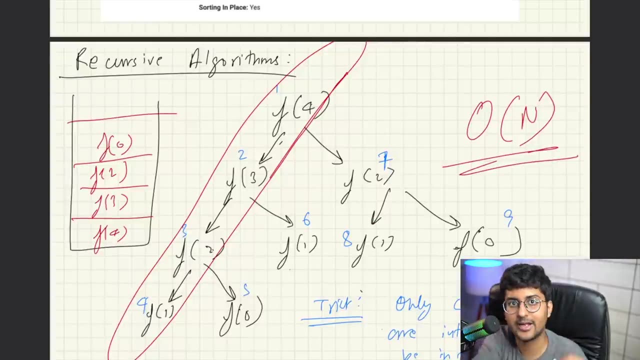 okay, so what is the space complexity when we are calculating? uh sorry, the auxiliary space, extra space required when we are calculating the nth fibonacci number o of n, because these all will be in the stack at the same time. it's maximum amount of space required at a time. okay, cool, let's move forward. okay, now we are. 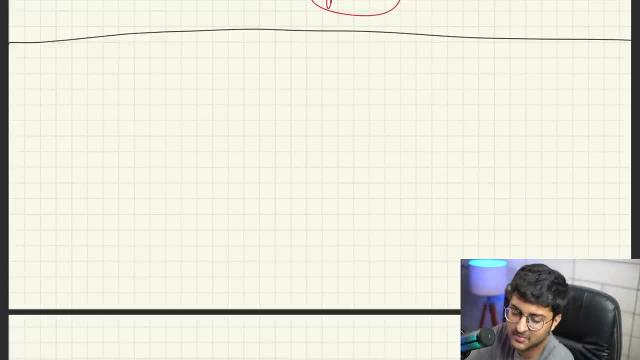 starting the section that makes this video special. please watch it very carefully, so we just want to make sure that you understand what we are talking about. so we learned about recursion. we've talked, we've talked about recursion before, but in this video we are talking about how to actually solve. 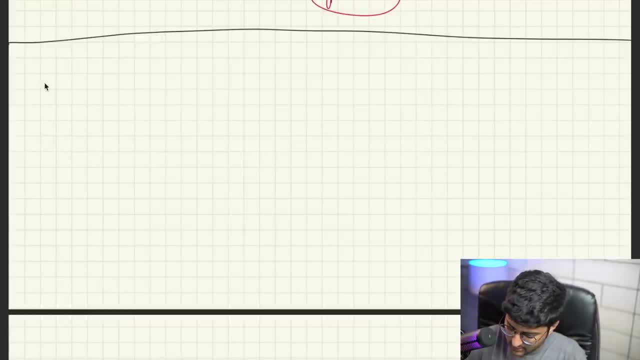 like recursion problems. like you know, there are two types of recursion problems. first of all, you know there are two types, two types of problems. so if you saw the uh one. second, let me just write it down: two types of recursions. so if you saw the recursion video, you already know about it. 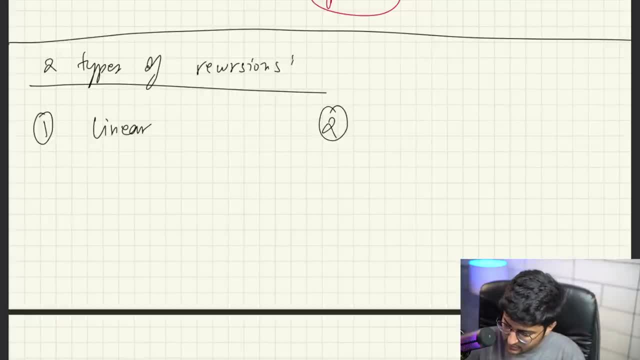 linear, like the fibonacci number. second one is what divide and conquer, like binary search. we already saw this. we also saw that these have uh recurrence relation, like the equations. so basically you can represent recursion in the form of a form of an equation. we did that previously. we said the nth fibonacci number is equal to n minus first fibonacci number. 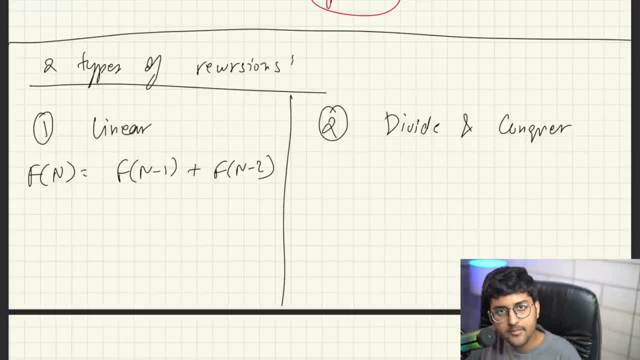 plus n, minus second fibonacci number. this is something we did already. we did the same thing. we said the time complexity for n, or i can say: you know, if i want to search for a in a function, uh, like a function for searching in the area of size n, this is: 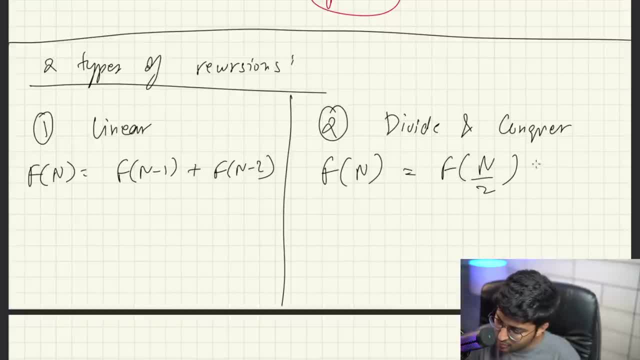 actually equal to what search in the array of size n by two plus a constant space complexity, constant time complexity. okay, so we know that there are like linear recurrences and there's divide and conquer references. so this is like the highlight of this video in this. now 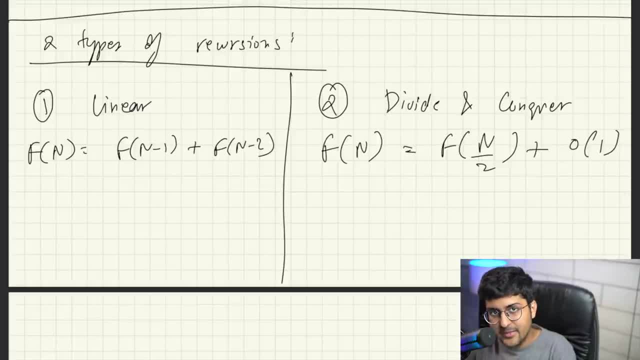 in this section we are going to cover how you can get the time, complexity, complexity and the formulas and basically the complexity, the final formula, big o, notation formulas of these equations. there are many ways to do it. in the college, in b tech, you might have heard about master's theorem, but i don't like it. it's not very efficient. you have to think about. 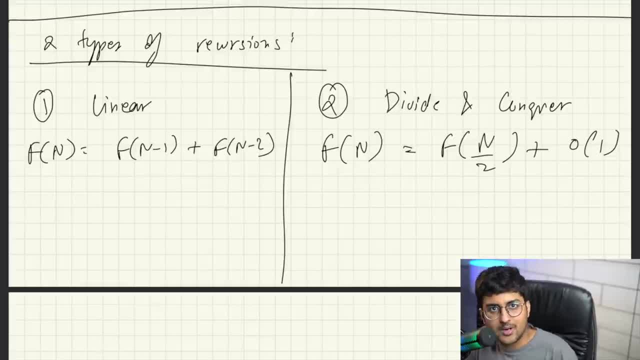 so many cases and all these things. ignore that. no need to do master's theorem. i will teach you something amazing that not many people are talking about, and no one literally talks about this in college either. you will also not find it in any b tech books. okay, so we will actually get. let's say, 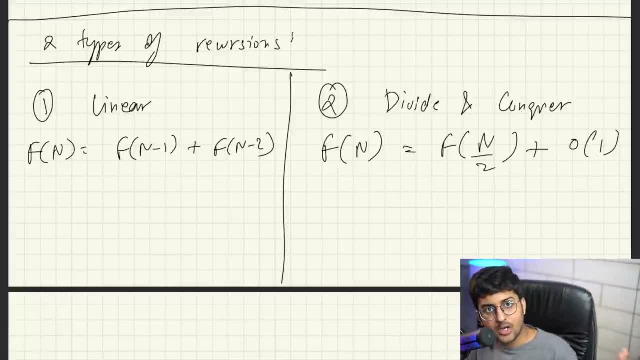 for example, the actual formula for binary search. i told you the complexity is 1.6. raise something, raised to power n, we will actually get that value. we will derive that value in such a simple way. i will teach you. you will be able to solve the most complex recurrence relations. okay, so when we do? 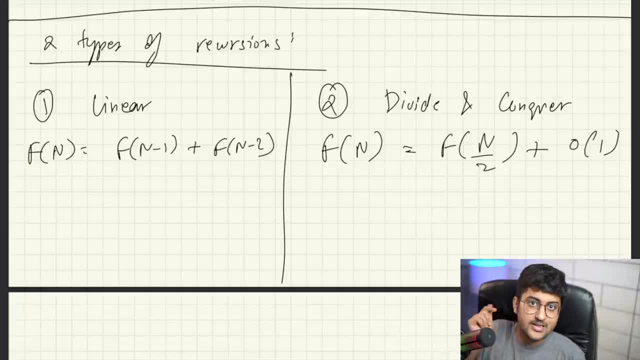 n queens, when we do quick sort, when we do merge sort, you will get the time complexity of it like this. this is also going to help you in your b tech. in b tech there's a, there's a uh, in there's. in b tech, there's a uh. there's a topic called 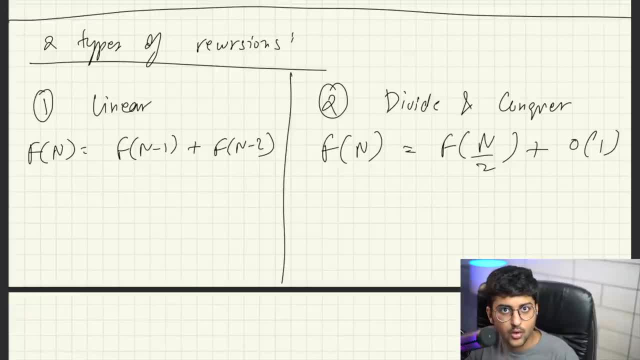 design and analysis of algorithms. okay, so there's a topic in that that calls for finding out the complexity and the uh equations of these uh particular recurrence relations. we will learn about that. this is a very you know, not many people are talking about it. this is in india. 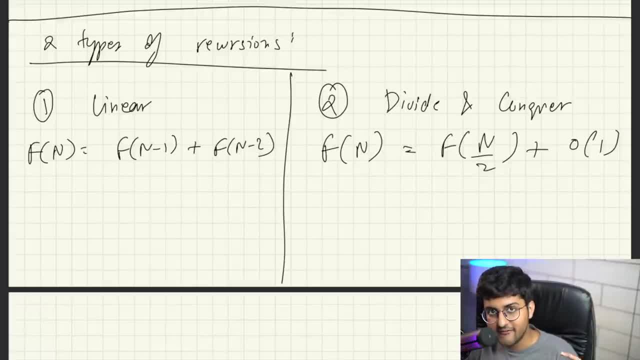 no one really talks about these methods and i will teach you it in a very nice way. let's get started first with divide and conquer recurrence relations, so we can see that these are both recurrence relations, just like over here. you can see it's like subtracting, adding or whatever, and then like: 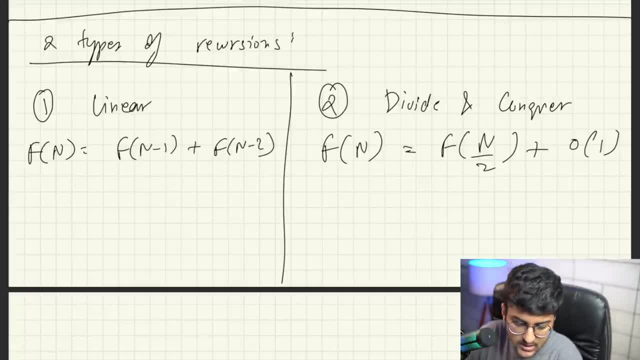 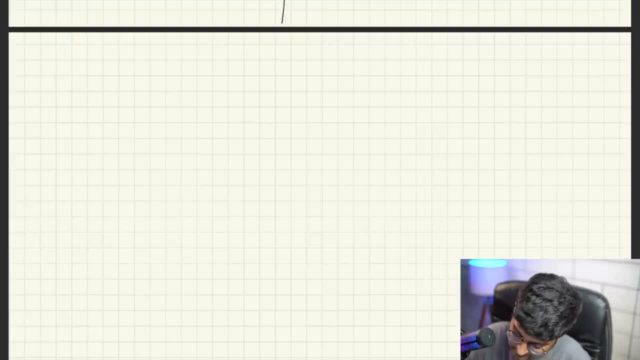 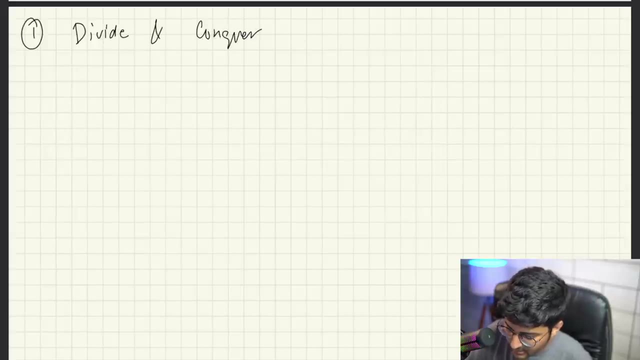 some linear way. here it's actually dividing it with a factor. so let's first say divide and conquer. okay, first we'll consider divide and conquer recurrences. okay, let's consider that first. first we will cover divide and conquer recurrences. divide and conquer recurrences- you will be able to solve any. 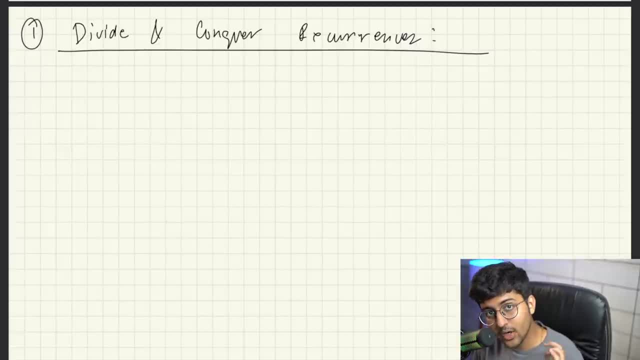 divide and conquer recurrence after this particular section. please watch it very carefully. it's really next level stuff. okay, it's going to be. you will be able to solve any question of b tech and all your problems and your cp or whatever you want to do. you will get time, complexity like this. 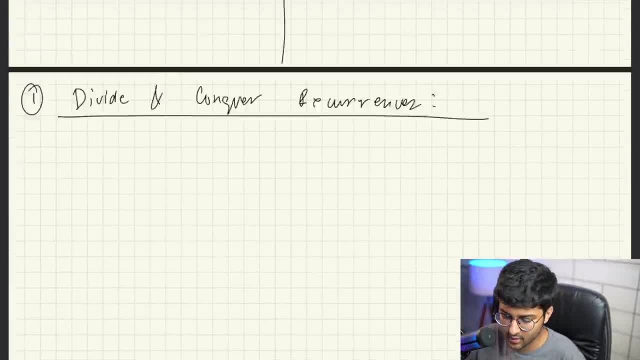 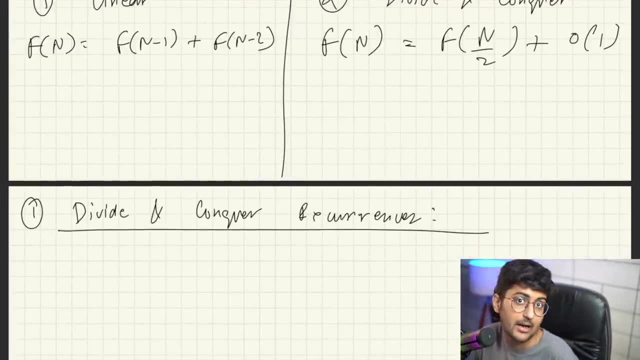 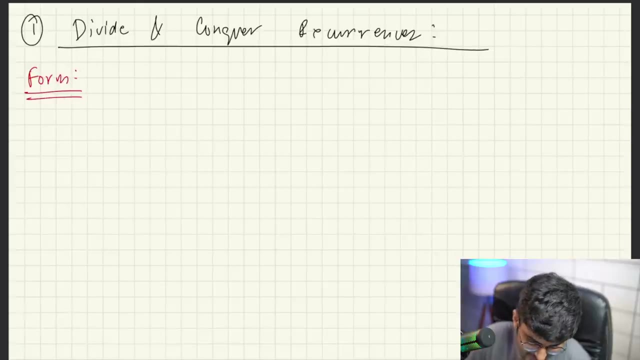 all right, so let's first look at what is the form of divide and conquer recurrence. this is a. how do we actually identify whether an equation is of divide and conquer or not? how do i? how do we identify that? how do we identify form? form is something like this: i can say t of x or n, whatever you want to call. it is equal to a 1 is. 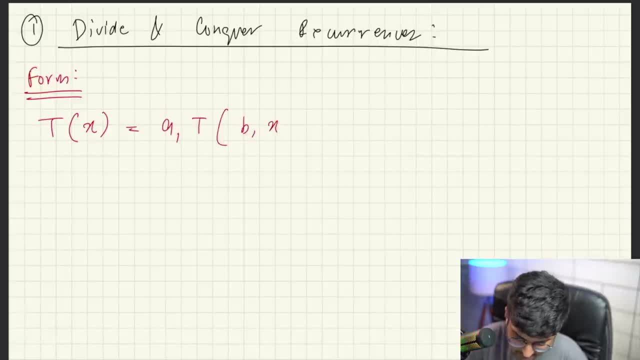 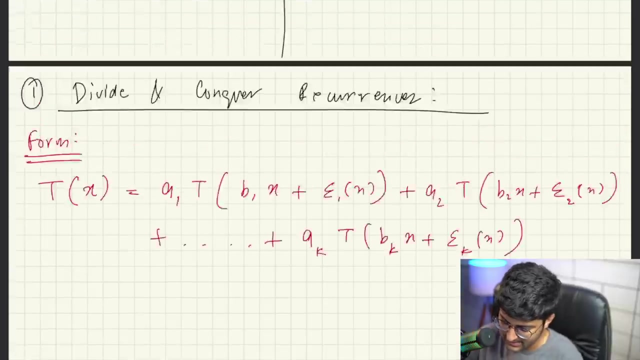 some constant t of b, 1, x plus some function x. okay, plus constant number two: t of b, 2, x plus some other function of x. it's just a simple form. okay, plus, plus, plus, plus, plus. you can go till a of k, into t of b, k, some some other constant into x plus into x. this is nothing confusing, it's. 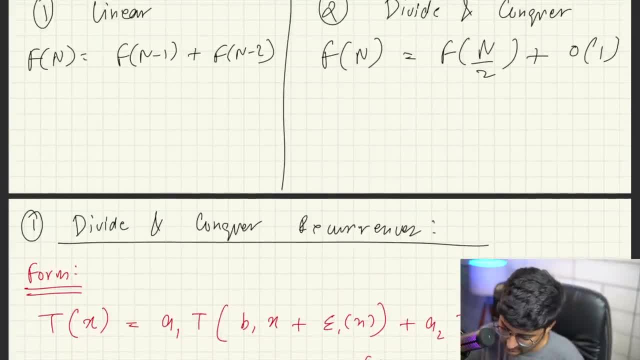 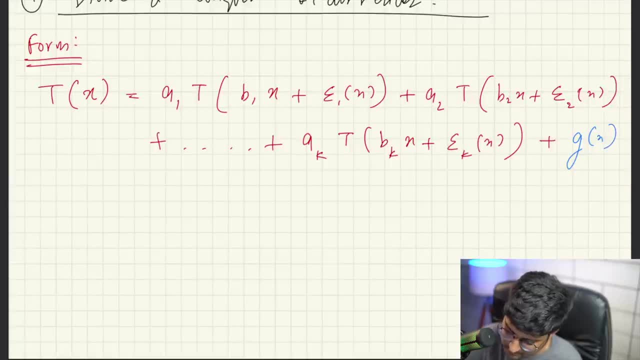 exactly the same representation of this here. let's say, a 1 is equal to- i'll tell you later on. i'll tell you later on, plus some other function g of x. okay, let's talk about it. this is actually for all x greater than equal to some constant x naught, this is some constant. 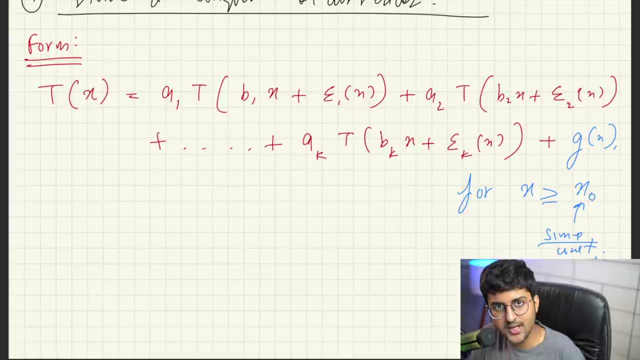 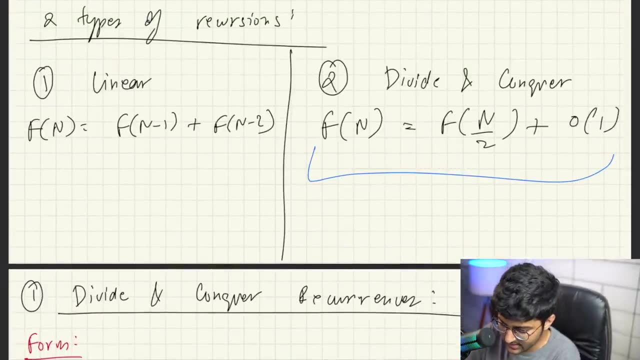 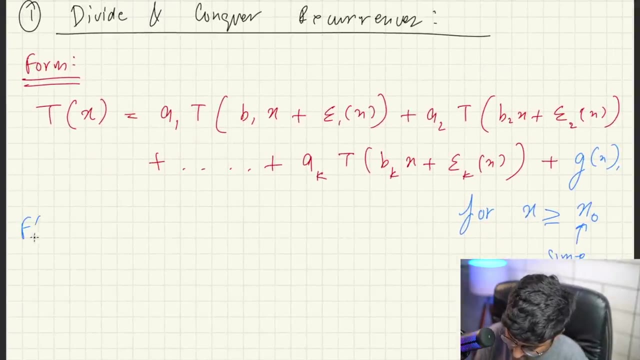 okay, you might be like: hey, kunal, this equation is very confusing. we have never done this before. you have, here you go this one. if i relate this with this, i can say: in um, in binary search. so i can say: if i have an equation like binary search, f of n is equal to or t of n is equal to. 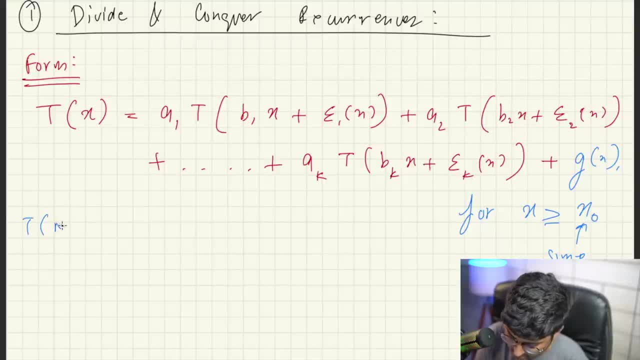 whatever, does not matter. f is equal to t or t times un. when you subtract that, i get equal to n character t. whatever you want to put, t of n is equal to t of n upon 2 plus some constant, some constant c if you want. so if i relate this equation with this equation, here i can say: a 1 is equal to 1. 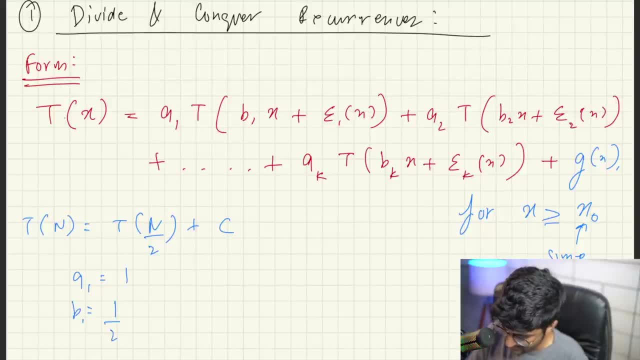 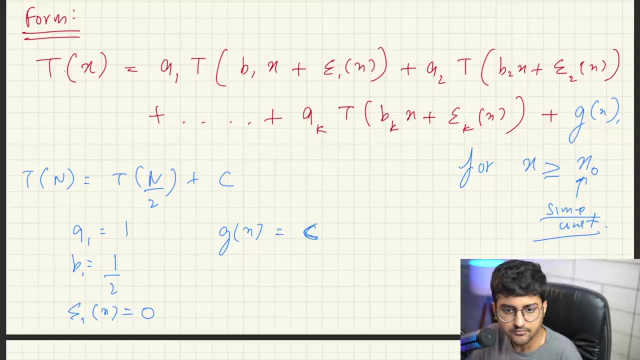 b 1 is equal to 1 by 2 and this is equal to 0, and g of x is equal to constant c. that's it. we don't have a 2, b 2 or whatever there's. your answer isn't this and this now. 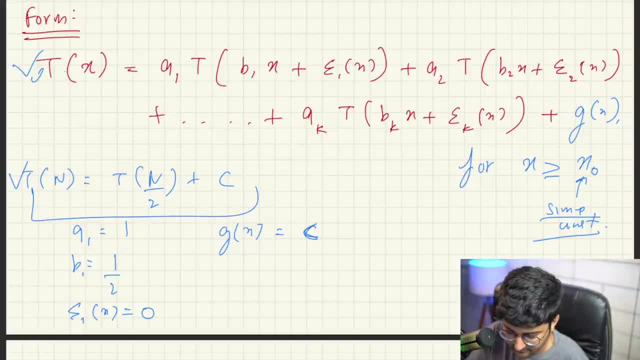 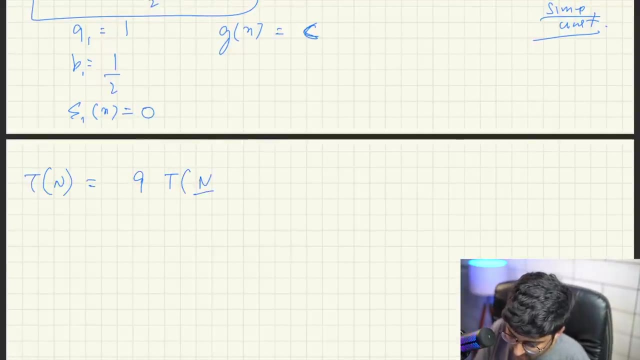 the same thing. isn't this the same representation of this thing? it is. are you able to understand? now? this is the form of divide and conquer, recurrence, your, your other relationship can be something like this: t of n is equal to 9, t of n by 3 plus 4 by 3, t of 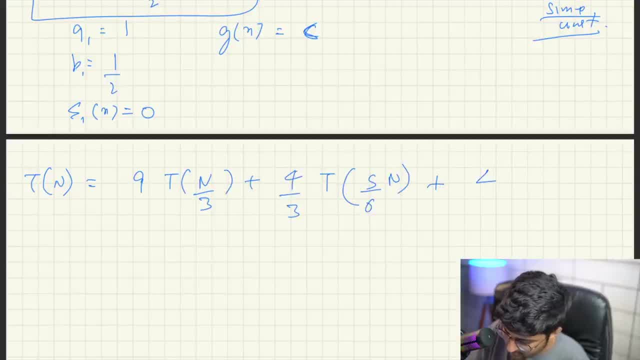 5 by 6, 6n plus 4n cube, something like this: this is a1, b1, a2, b2, g of n. that's it. how difficult is this? are you all able to understand? what is the form of divide and conquer recurrences? 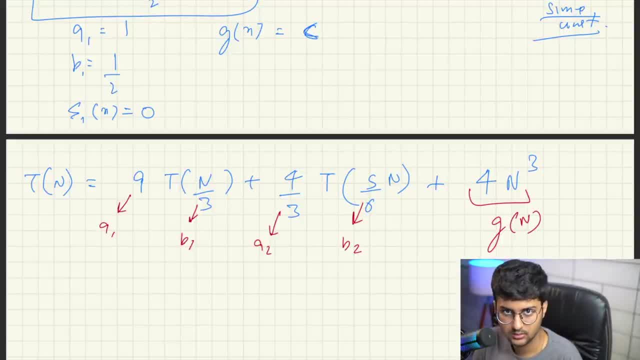 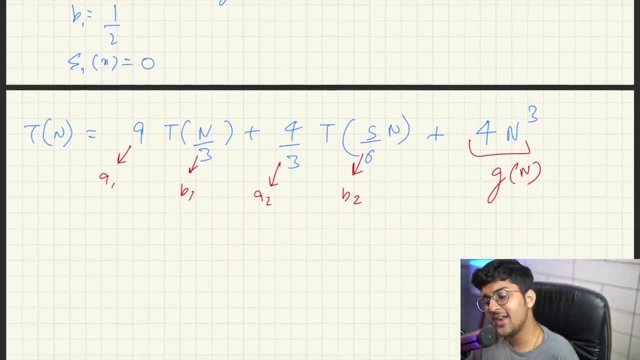 this is a simple formula. this is the form. okay, cool. now, what is this g of n? this g of n is basically um. this g of n basically means that. what is this g of n? so g of n basically means what g of n is like. uh. 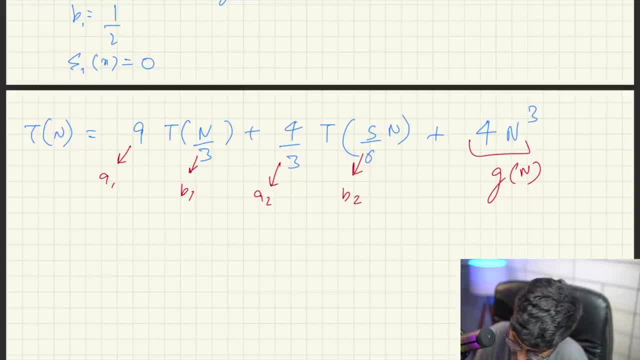 it's saying that, if i take something simpler, so if i say t of n, another example is equal to 2t of n by 2 plus n, or something like that. okay, or n minus one. so i can say: this is a1, this is b1, this is g of n. so this recurrence relation, in simple terms, what? 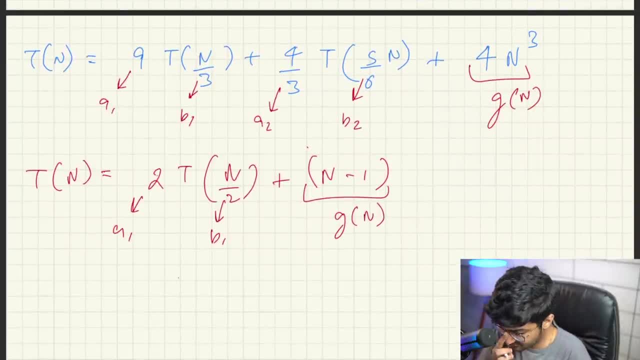 is g of n. i'm trying to make you understand the intuition in simple terms. it means that, okay, recursion is saying: sort, do something with half of the array, do something with other half of the area, because this is another example of g of n. it's saying that, if i take something simpler, so 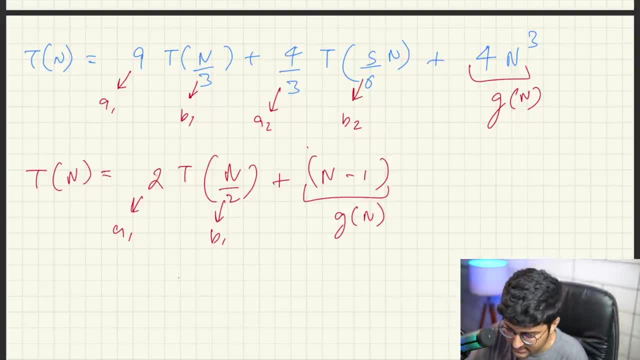 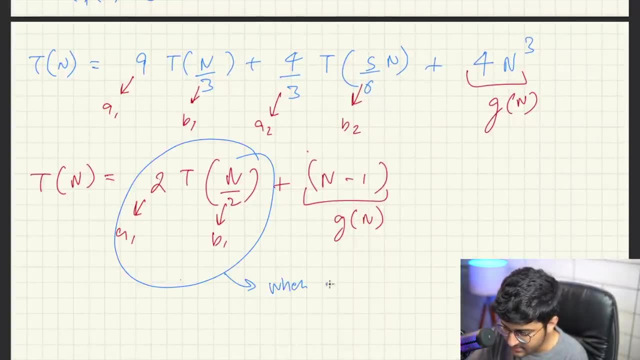 by 2 plus n by 2. when you get the answer from this, g of n basically means: when you get the answer from this, when you get answer from this recursion call, when you get answer from this plus what you are doing with that answer takes how much time. so example in binary search is saying: try to search. 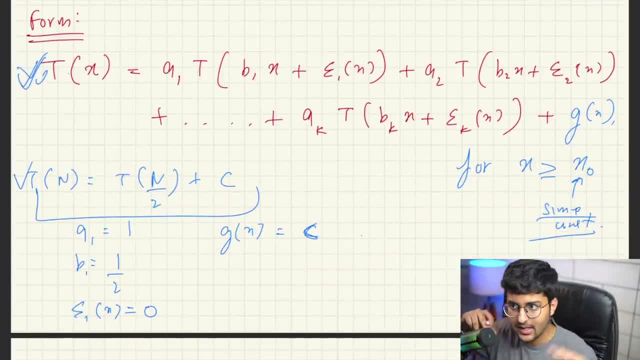 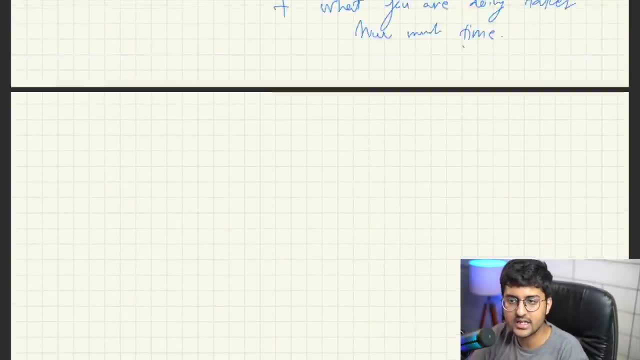 in, like you know the this one and like the half of the array, and what is? what are you doing once you start searching? you're just saying you're just comparing stuff. or if you're talking about some other algorithm that says, okay, let's say we do. some other algorithm that says, let's say, 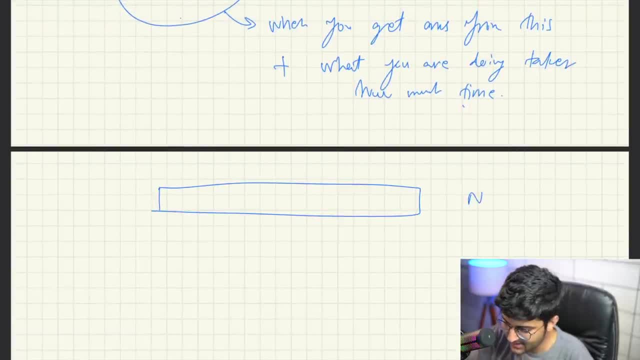 you have an array like this, okay, an algorithm of size n. you can say something like: uh uh, sort n by two of the array, sort n by two other half of the array. when this is sorted, and this is sorted by a recursion, merge these two. this is actually called merge sort, which we'll be doing. 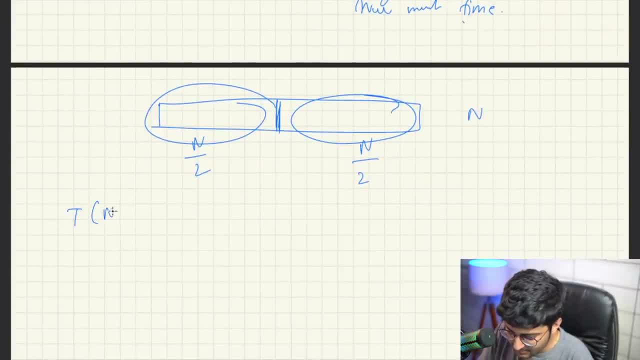 in the separate video. so this actually says time complexity. n is equal to solve the half of the array plus. solve the second half of the array plus once. once these both are sorted, merge the arrays. merging takes how many comparisons? n by 2 plus n by 2. if you want to merge, it takes n minus. 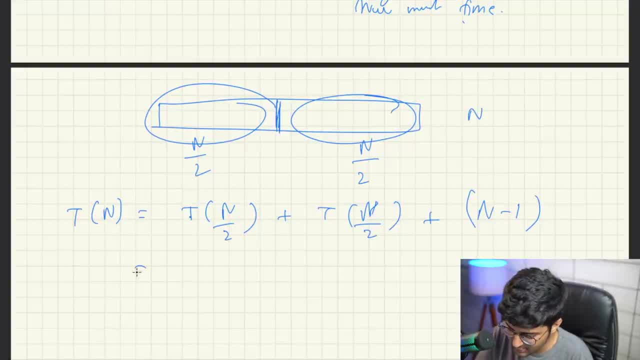 one. so you can do this. but if you want to solve half of the array, you have to solve the second one. comparisons: we will look into it in detail. this is actually equal to 2 t n by 2 plus n minus one. this is the recurrence relation of merge sort. separate video on this later on. okay, separate. 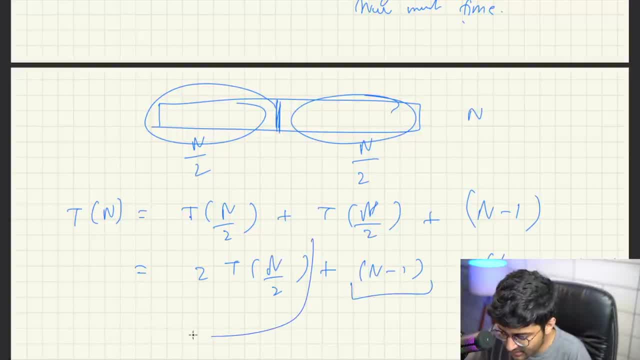 merge. sort video will come okay. so this basically means once this recursion call is over, then what amount of time complexity is required to do actually something with those recursion calls that are over right now? extra time required at that step in binary search. what is the extra time? 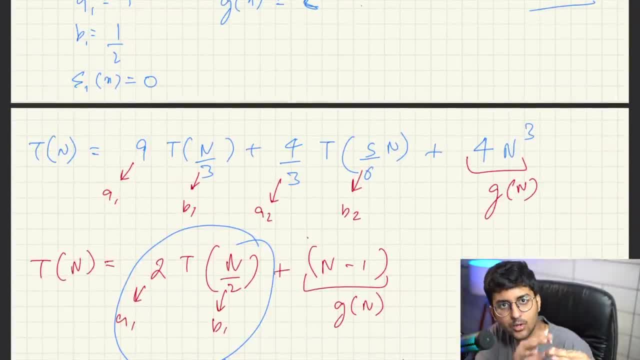 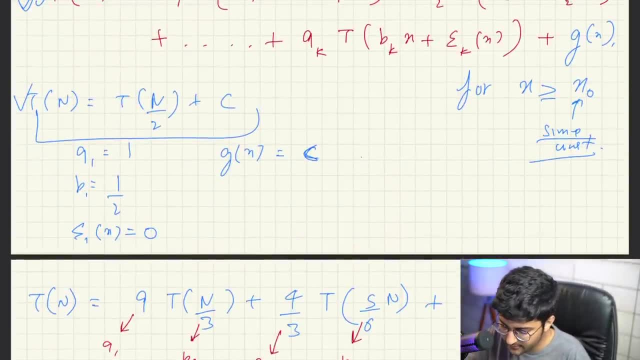 required at that step. extra time required at that step is just equal to checking whether a number is greater than, equal to or less than middle. that takes constant amount of time. that's why we have constant over here. this is something we've covered in detail when we were doing binary search. 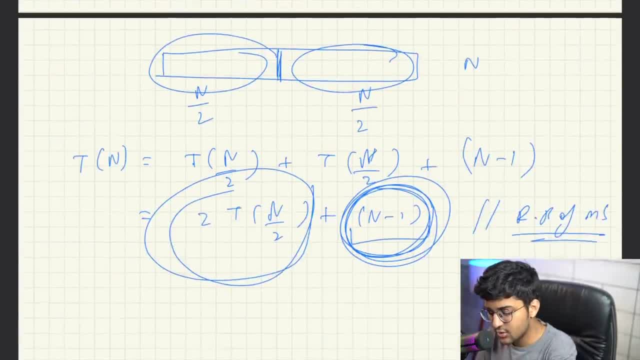 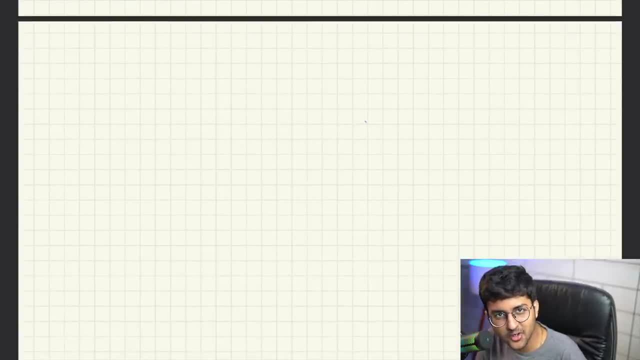 okay, cool, so you are given this recurrence relations, no problem. most important part, how to solve. we know binary search is o of log n. we know merge sort is n log n. how to solve: maybe we can do it in binary search, we can do it in binary search. we can do it in binary search. 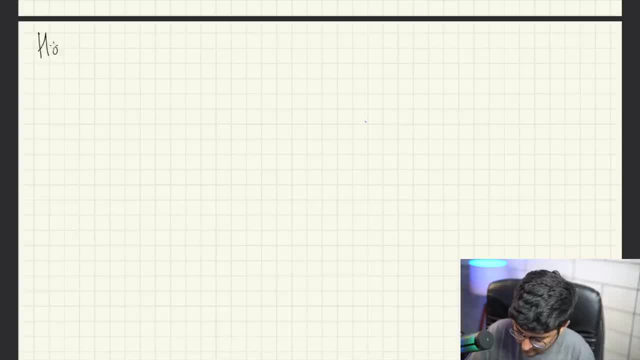 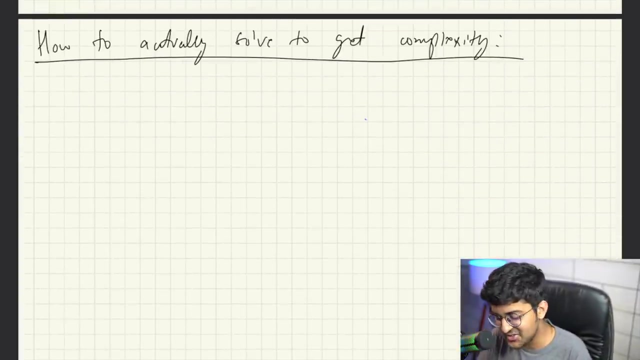 many ways to solve, how to actually solve, to get complexity. this is the highlight of this course. it will like- literally like you will be dancing with fun. please subscribe right now. this reminds me: subscribe right now. take a screenshot. take a screenshot when we do the, the formula that i'll be teaching you right now. so there are few ways. one you can do: 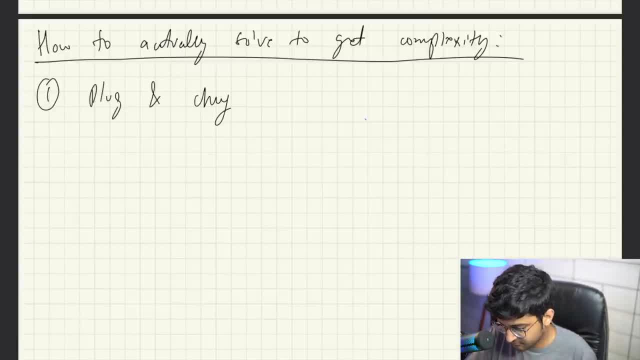 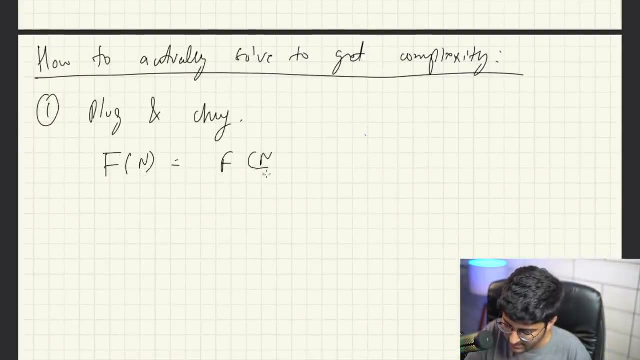 uh is plug and chug. plug and chug is basically just simple. we have done this in b tech also. i will not be teaching you this because this is not not not required, so you just basically take the formula. so basically the idea is, if you're given something like, f of n is equal to f of n by 2 plus 1 plus c. so this: 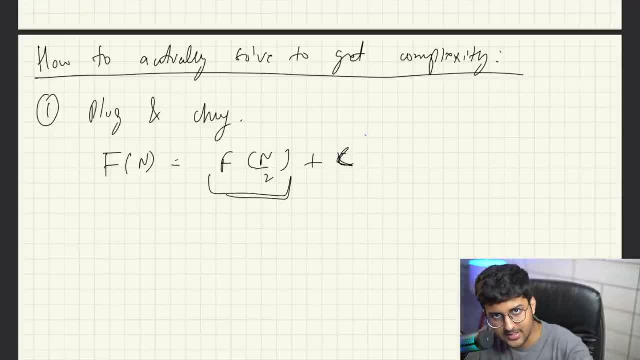 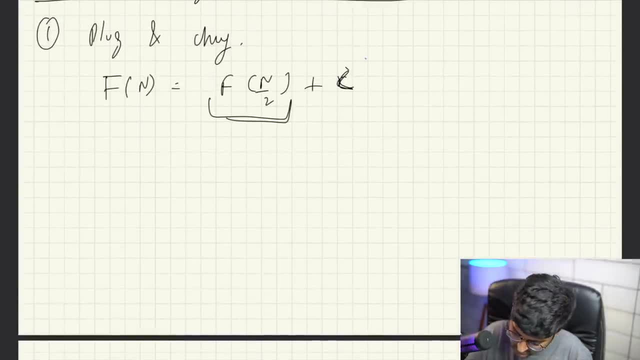 entire formula. you put it in this and then you keep on making the tree and then you combine that. it's a plug and check google it yourself if you want. but i would not recommend doing this. it's a waste of time. second one is master's theorem. i do not like this method, hence i will not be covering this. 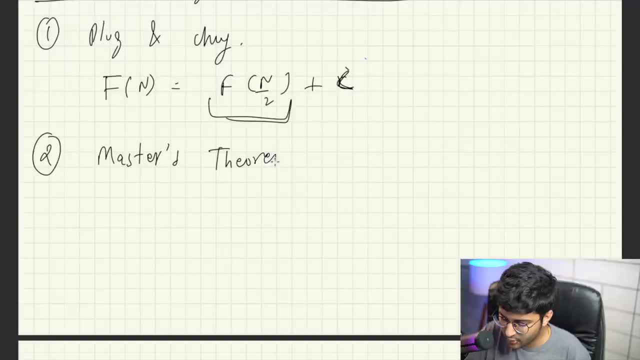 master's theorem. no need to do. you can totally skip it. no need to do master's theorem. okay, there's some cases or whatever. in btech they teach master's theorem. ignore it. best way. best way to do akrabazi formula. they were like two people from mit. they came up with this formula. 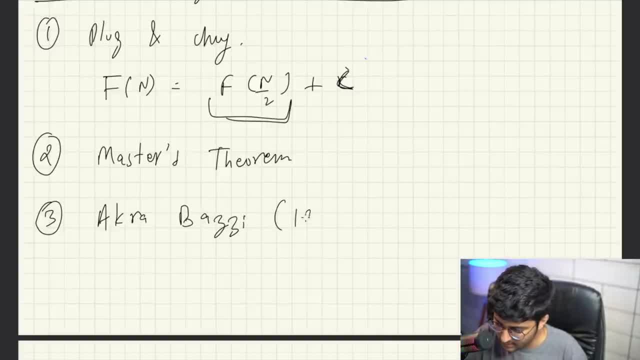 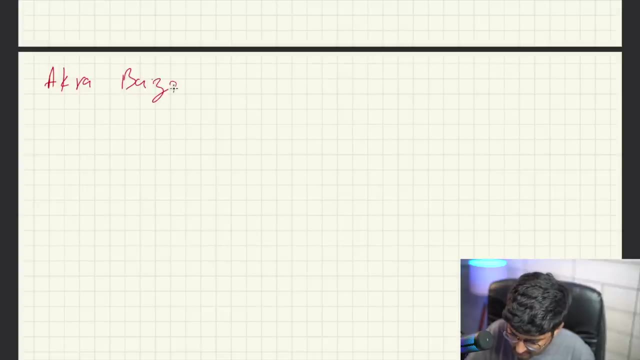 in this simple formula you can solve it. okay, it was divided in 1996. you can solve any recurrence relation: divide and conquer recurrence relation. let's look into it. akrabazi formula. this is something we'll be doing. akrabazi formula. okay, no problem. what is the formula? formula is that? 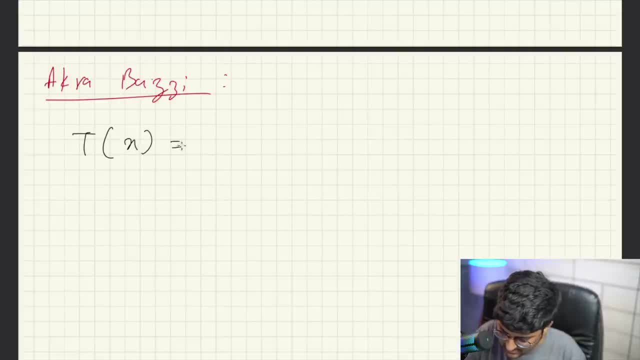 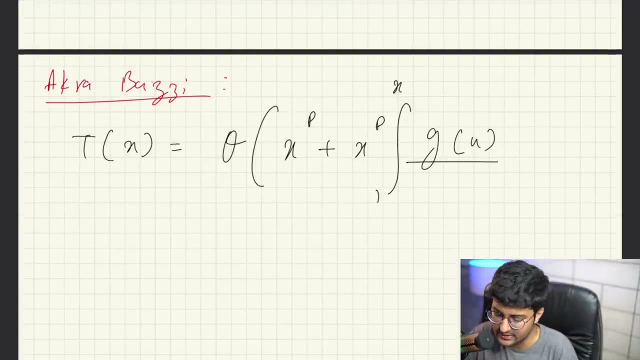 the time, complexity x is actually equal to theta of x raised to power p plus x raised to power p. integral of. please don't be scared with integral, because i will give you proof of why you should not be scared. g of u. this is: this is just the g function that we had previously: u raised to power p plus one d. 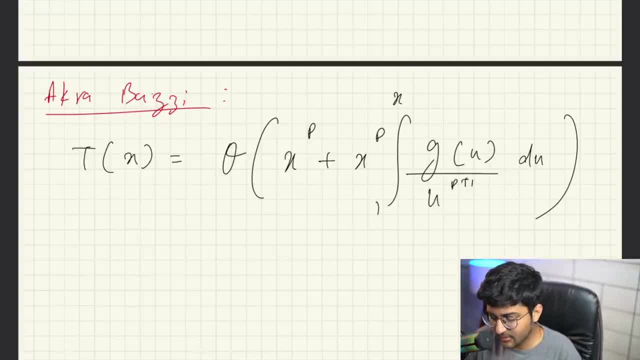 of u. okay, one thing i want to mention is why you should not be scared of this integral, very important point. you will be saying: kunal integration is not our strongest point. i will only use master's theorem. let me tell you why you should not be scared of this integral function. because this g of 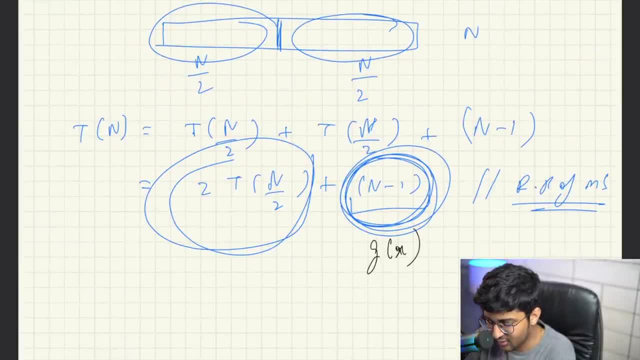 u, this g of n, u or whatever constant, the variable name does not matter. this g function is basically a time complexity itself. okay, it is time complexity itself, and we know that in time, complexity, like constants and more dominating terms, are ignored. so even if i remove minus one from 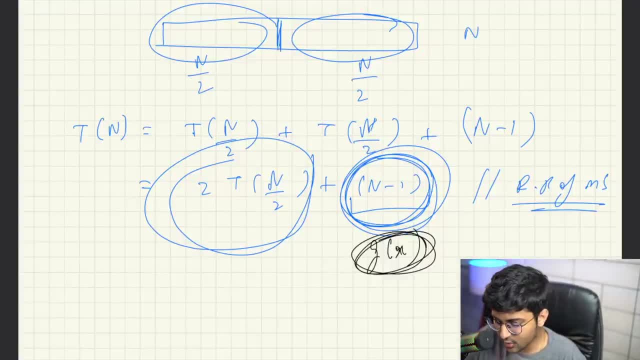 here. that is going to be totally fine. okay, so this is a time complexity. okay, so let's okay. so we know that this is going to be the simplest form of this function, because all the less dominating terms and all these other things will be removed, so this will be a very simple function. 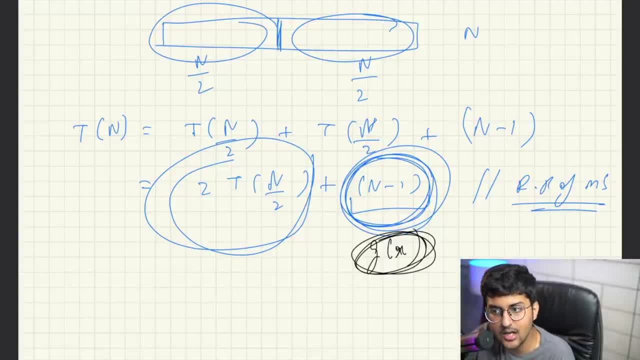 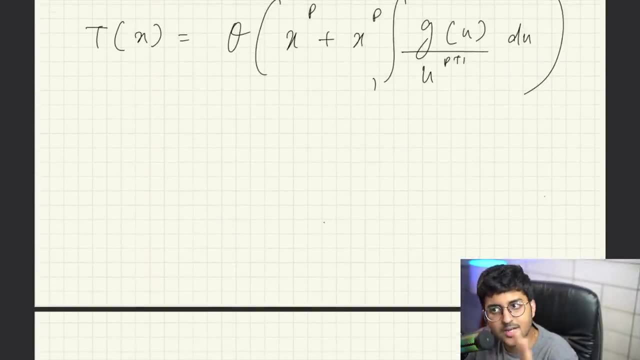 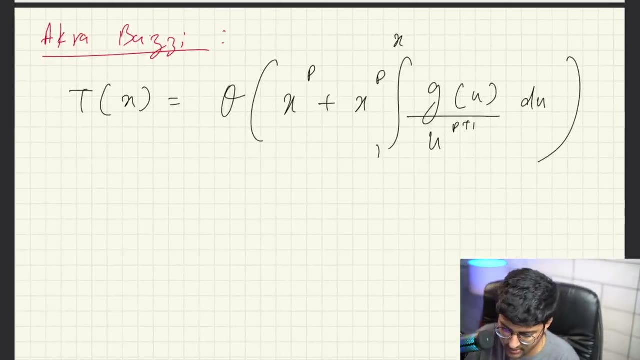 hence, integrating simple functions is going to be very simple. only you are going to be required are small, small, basic basic integration. uh, formulas, okay, nothing major. hence, anyone can do it. revise basic integration, you will be able to do it. okay, we all know basic integration, we know that uh. 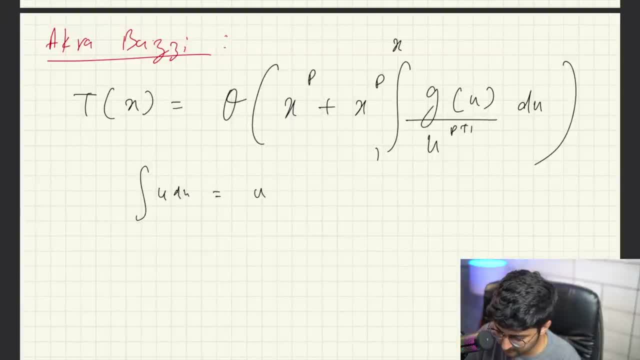 u d u is actually equal to u or u square by 2, something like that. okay, you can say u raise to power p. you can say something like u raised to power p d u is actually equal to raised by p plus 1 upon p plus. 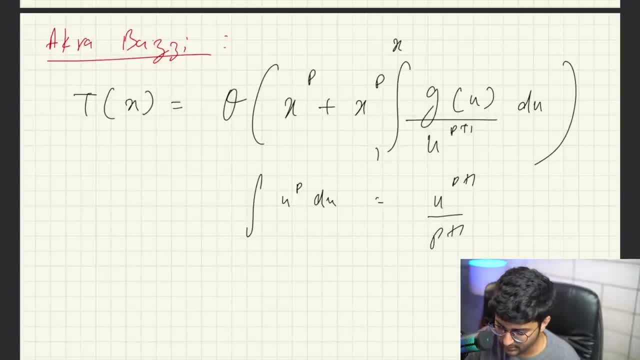 1. very basic formula of integration. that is what we will be doing over here. that is all that's required. what is p? very good question. what is p? so you have to p, you have to find p such that a1, b1 plus a2, b2 plus all the a's and b's that you 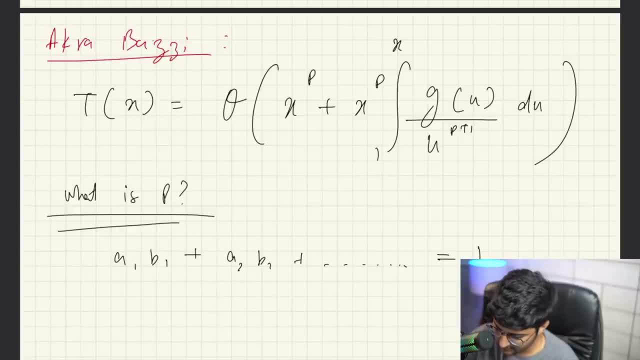 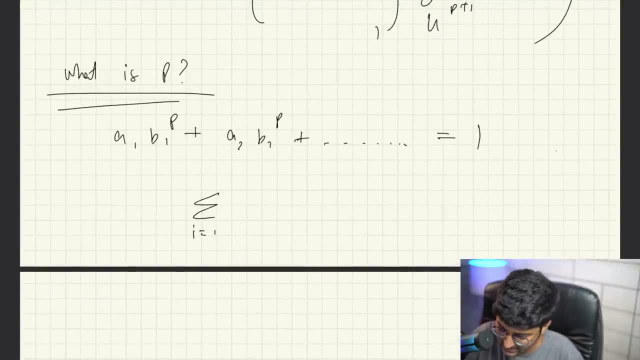 have should give me equal to 1. sorry, not a1, b1, actually a1 b1 raised to power p, a to b2 raised to power p. so basically, sum of for all i till k, a of i, b of i raised to power p, should give me equal to 1. 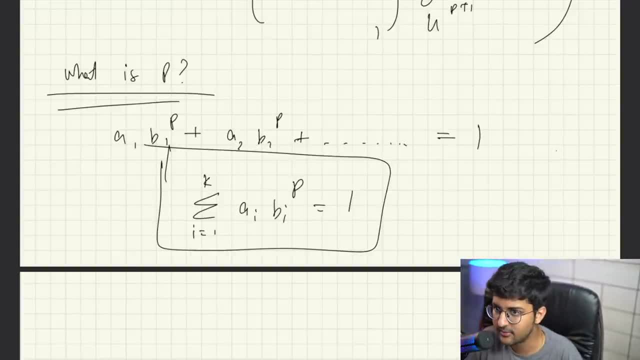 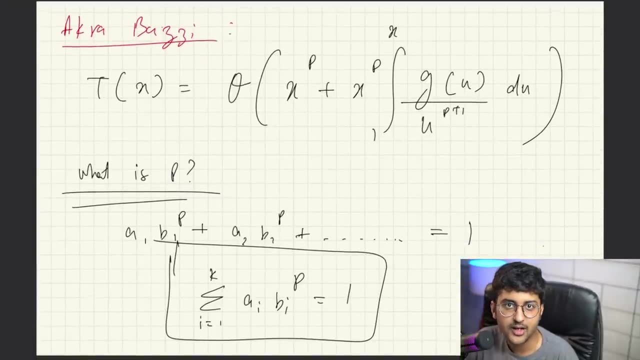 that is how you find p. i will tell you some tricks for this. well, right now it may feel overwhelming, but trust me, i was also a student. i was in my first year when i did this. math is not my strongest point. i failed iit. je okay, i was not a high scorer in maths. it. 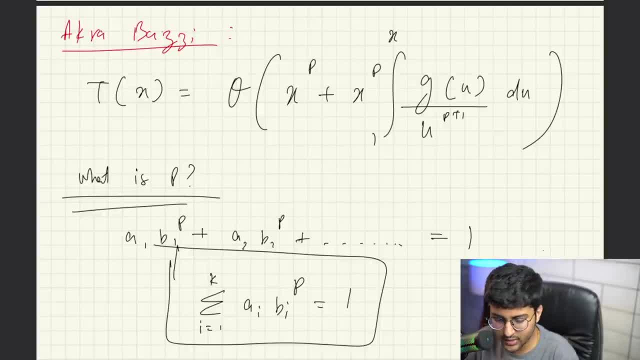 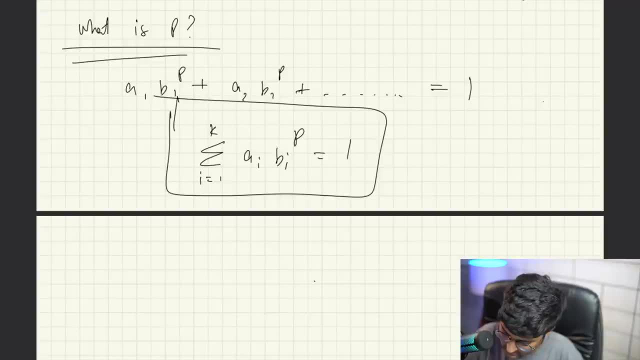 is very easy stuff. if i can do it, you can do it as well. let's look into it with an example. let's look at the example of binary search. what is binary search? binary search says: um t of n is equal to t of n by 2 plus 1 or some constant c or whatever. 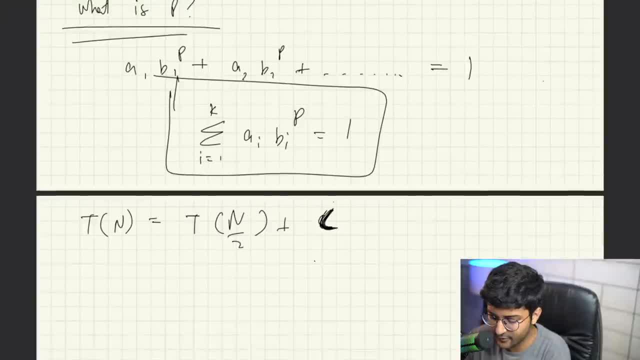 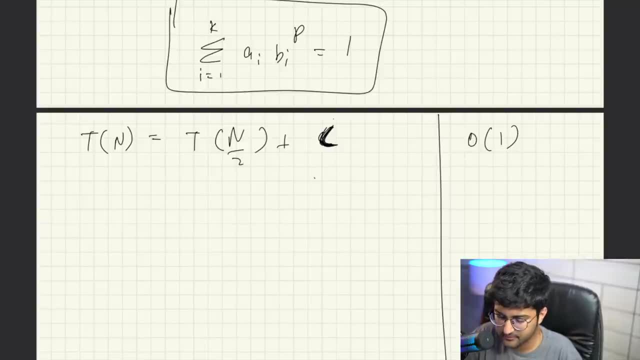 okay, um, by the way- this is also something i forgot to mention- with constant space, constant time complexity or constant complexity in constant, why do we write o of 1? because we don't really care about constants. if you say something like, we can write o of c. 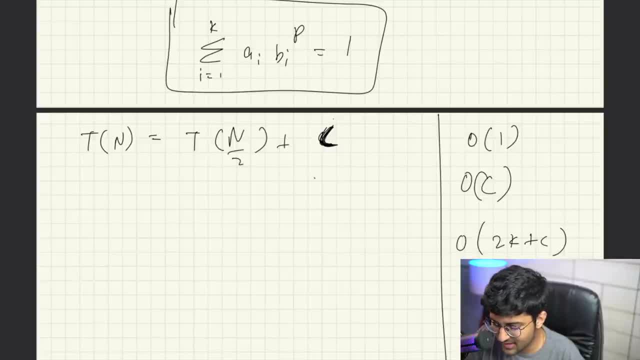 you can write o of 2k plus c. all of these are constants. i can say that we can ignore the constants. so this can basically be like this: multiplied by 1, anything multiplied by anything you can ignore, the constants has hence anything. anything in constant can be. 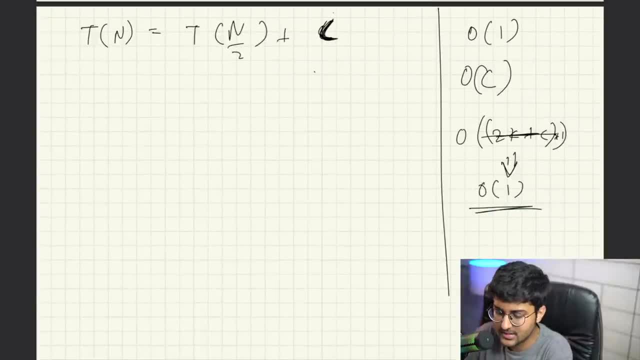 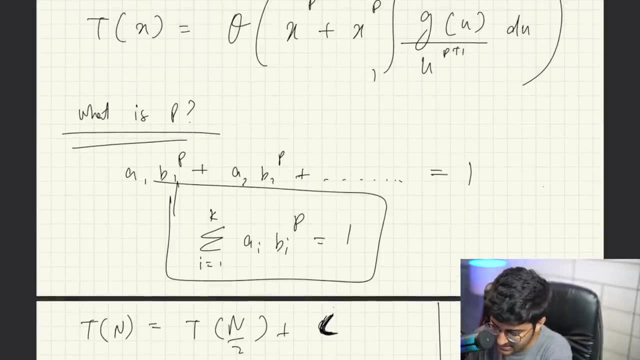 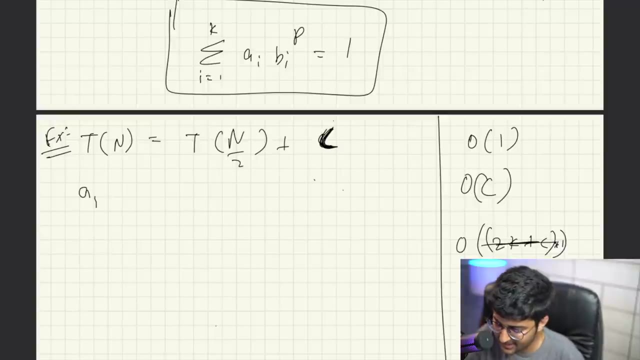 written as o of 1. that is why we write time, complexity, space complexity- there are constants- as o of 1. okay, so here, if i try to see even akrabazi formula, i can say a1. let's write example of binary search. i can say a1 is equal to. example of binary is very 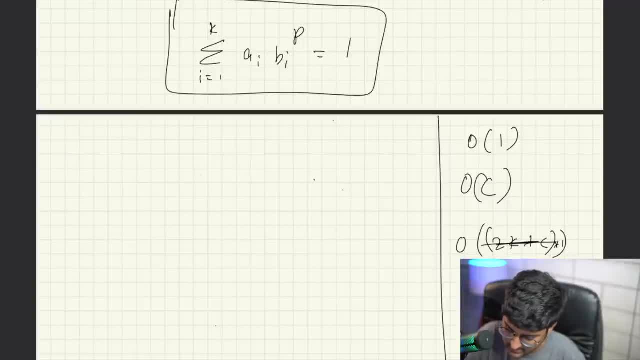 simple. i'll take directly merge sort. okay, let's take some random equation. i can say example. i can make something like: t of n is equal to 2, t of n by 2 plus n minus 1, something like this. okay, here i can say: a1 is equal to 2. 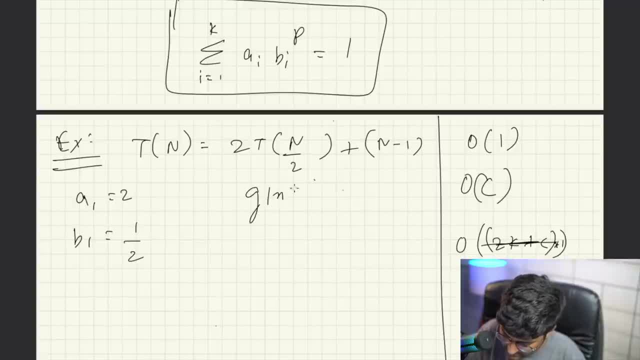 b1 is equal to 1 by 2, g of x is equal to x minus 1, and k is equal to what? k is just equal to 1, because there's no, no b2 or a2. okay, so i can say that, according to this formula, a1, b1 raised. 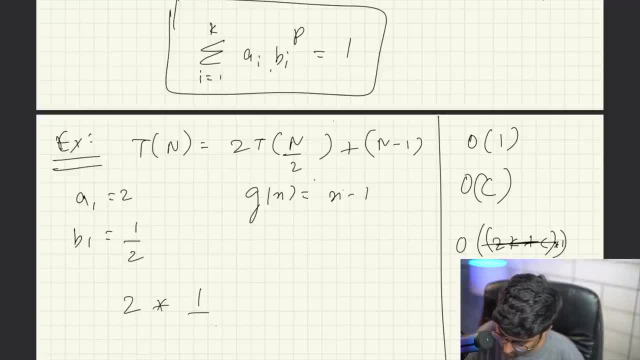 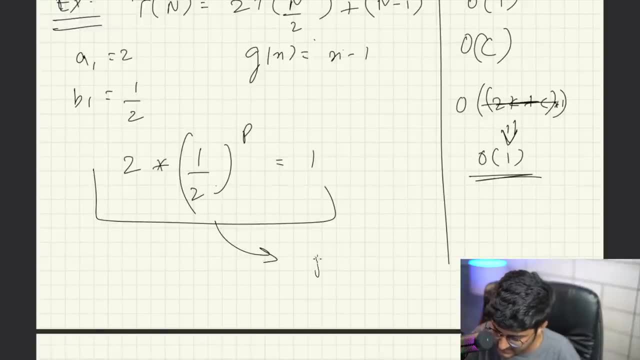 to power, p should give equal to 1, means 2 into 1 upon 2. raised to power, p should give me 1. via this i can say that by a hidden trial i can say p is equal to 1, because if i put 1 over here, then this: 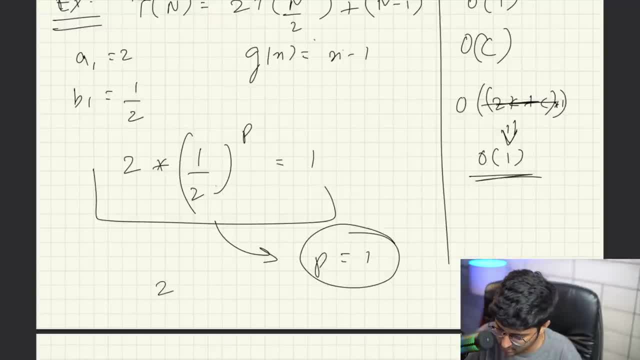 condition is satisfied. hence i know that p is equal to 1, because 2 into 1 upon 2, raised to power 1, give me 1. that's why p is equal to 1. now i have found my p. once you have found your p. 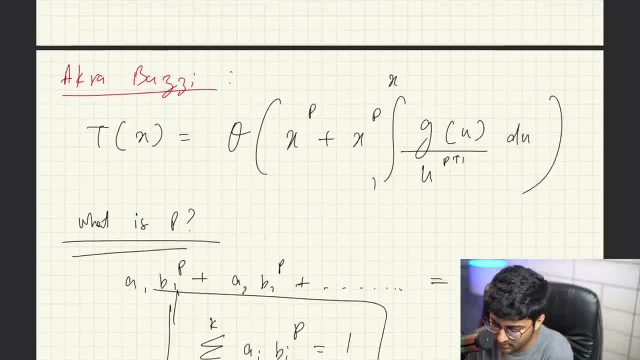 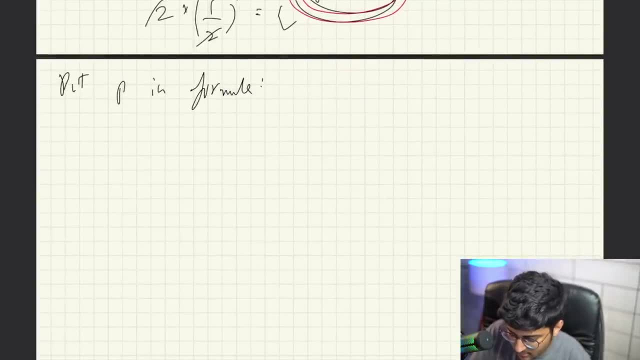 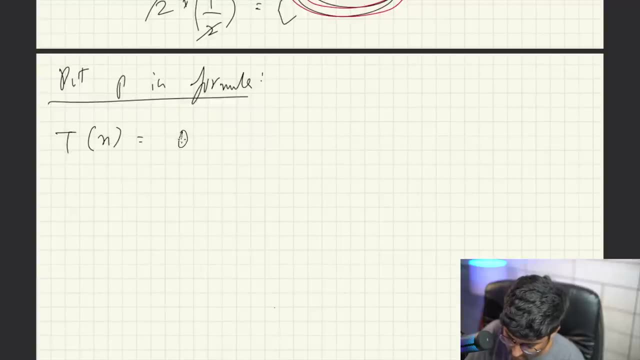 solution is over. all you need to do is put p in your akrabazi formula. so i'll just put it in formula. now, put p in formula. i'll put this in my formula. i'm going to say that what i'm going to say, t of x is equal to theta of 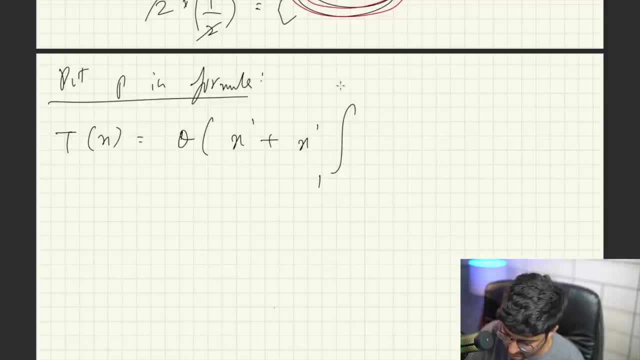 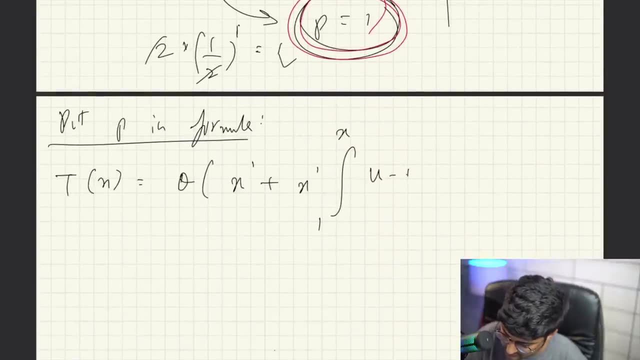 x raised to power 1 plus x raised to power 1. integral 1 till x g of u, which is equal to x minus 1, so this will be u minus 1. divide by u raised to power p plus 1, so it will be u raised to power 1 plus 1. 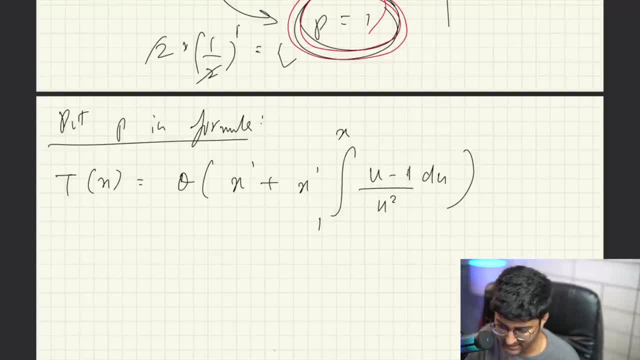 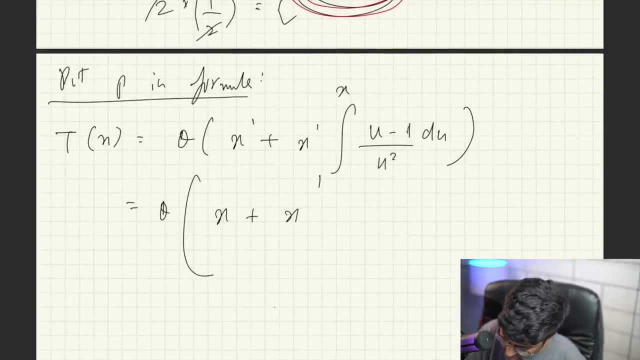 u square du. that's it. that is it. try to solve it. how do we solve it? just simple integration. i'll say x plus x, integral of 1 upon u minus 1 upon u square du. if i try to solve this thing, this is going to give me what. 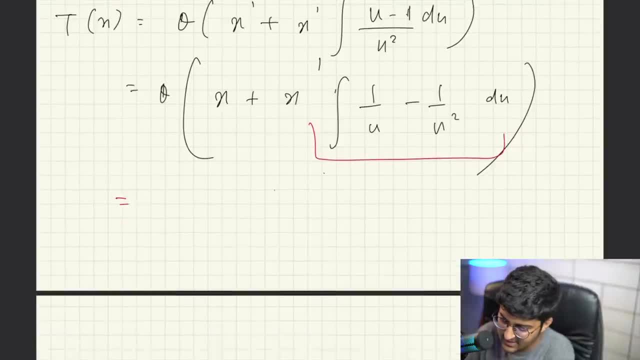 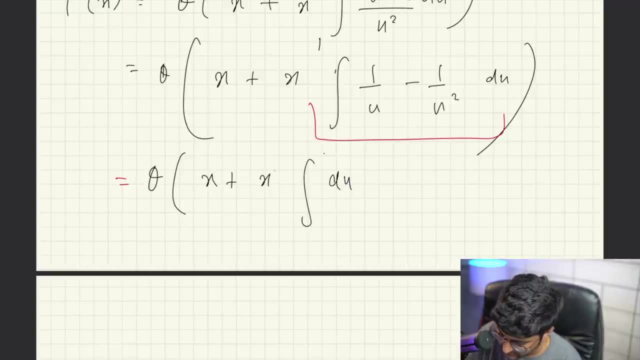 i. i don't know if i should do this like in detail, because this is very simple. uh, you know very simple stuff. so this is basically x plus x. integral of du upon u: 1 till x. integral of du upon u square: 1 till x. that's it. 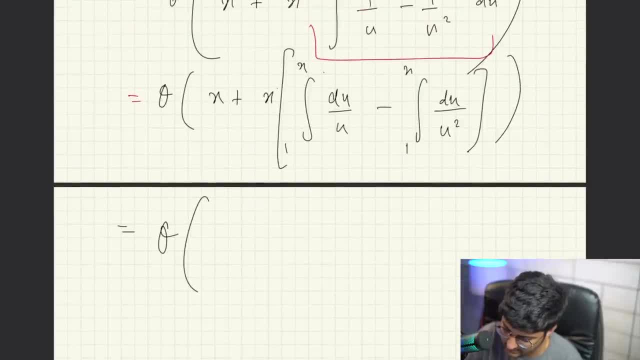 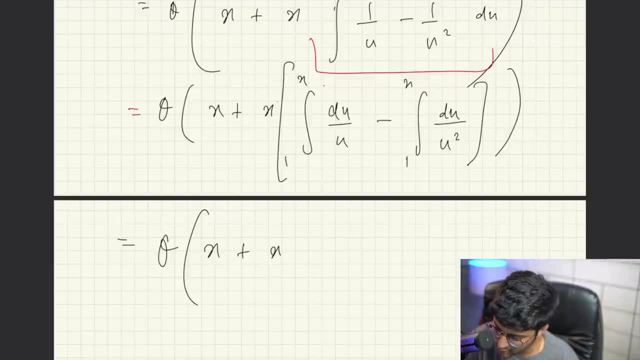 even though there are. there are so many steps, because i'm explaining everything in detail. this is nothing. you can do it in one line also. so what is the integral of 1 upon u? integral of 1 upon u is log u, so this will actually be equal to. 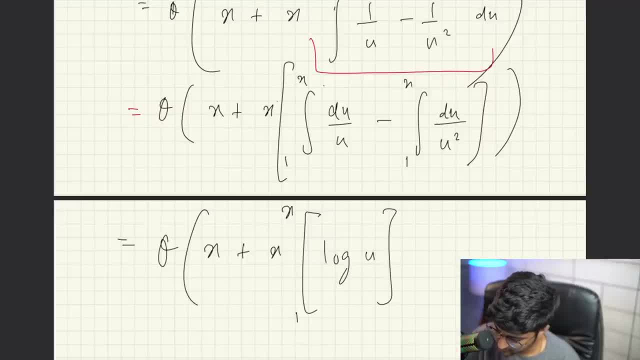 1 upon 1 into x. log u minus. you will be having something like: uh, this was an outer scope. we'll be having something like: what is the integral for this going to be? integral for this going to be u raised to power minus 2, so this will be equal to. 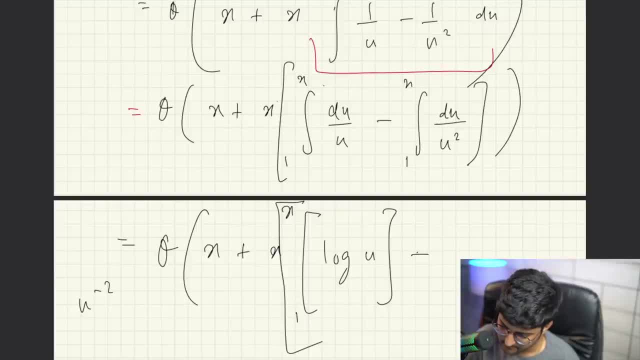 uh, what this is going to be equal to, what this is going to be equal to u, raised to power: minus 1 upon minus minus 1 upon u. that's it. so it's going to be something like this: minus minus 1 upon u, plus 1 upon u makes sense. all right, let's try to put. 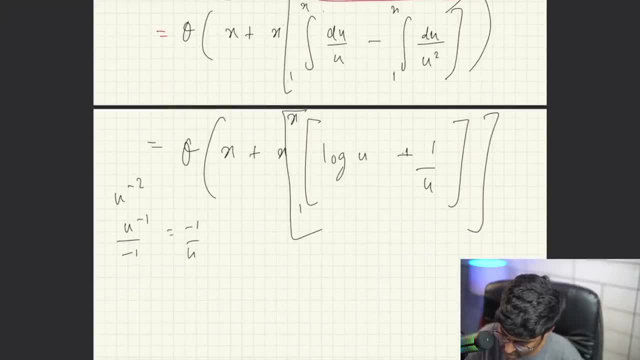 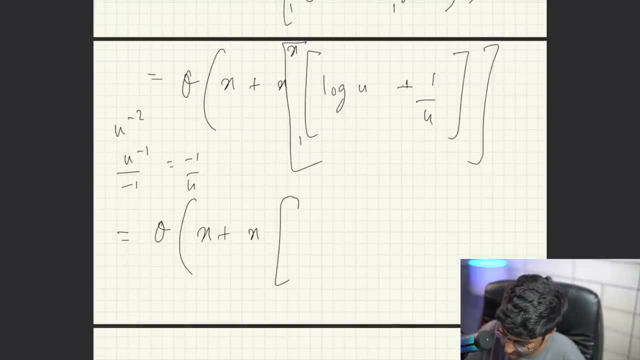 this formula in it. let's try to put the values of 1 and x, if i put the limits, some basic basic integration rules, x plus x, into. i can say first: i will put x log x plus 1 upon u minus log 1, which is 0. 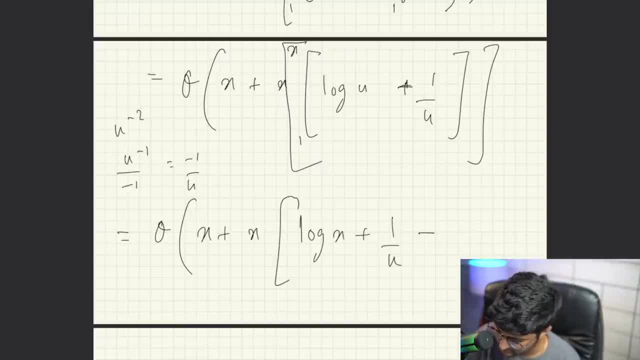 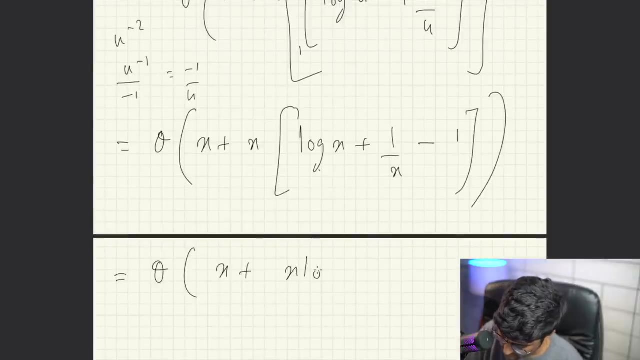 minus 1. so this will be something like: sorry, 1 upon x minus 1. that is it. that is it? if i try to open this formula up? if i try to open this formula, this will be something like this: will be theta of x plus x. log: x plus x minus x. sorry, plus 1 minus x. 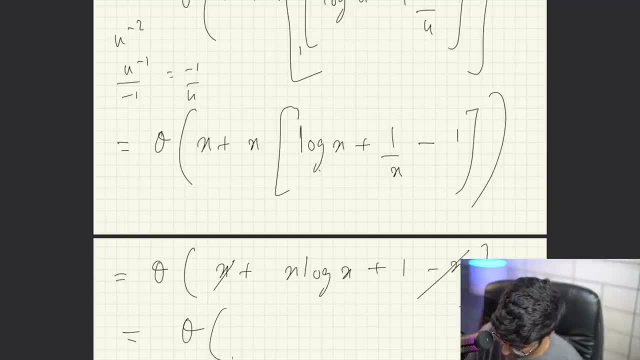 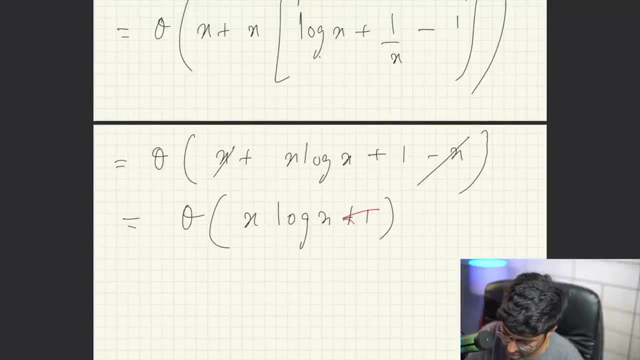 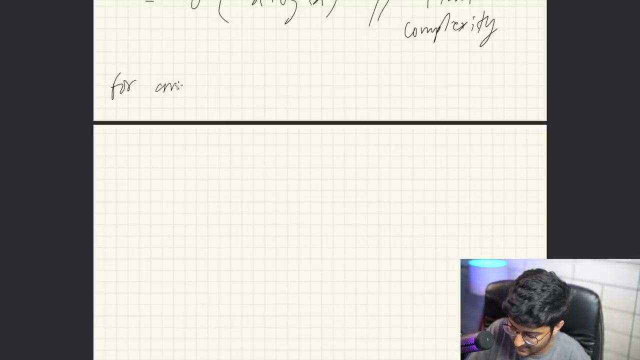 x and x gets cancelled, this is equal to theta of x log x plus 1. we know that constants are ignored, so i will ignore this constant. this will be now equal to theta of x log x. this is the time complexity. so, for an array of size n, for array of size n, 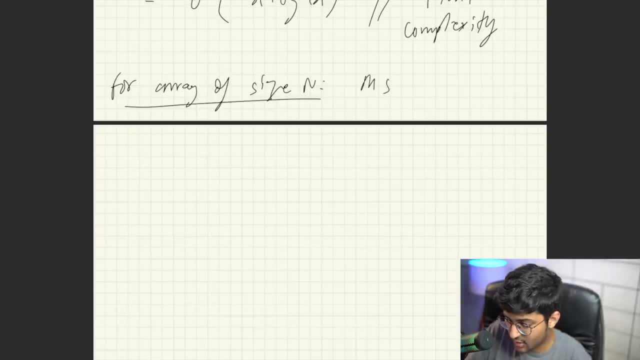 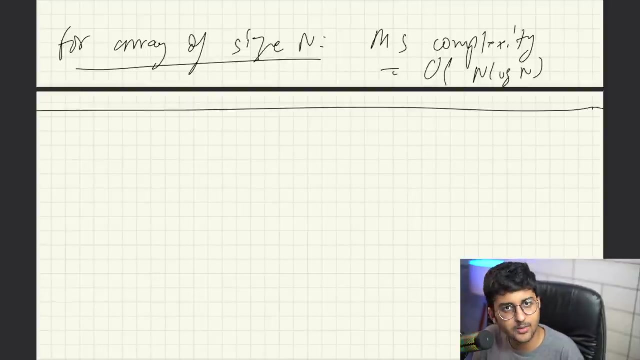 merge sort. complexity is equal to theta or big O of n log n. very simple. why akrabazi? very simple stuff, cool. now people will say something like: hey, kunal, why did you use master, why did you use akrabazi? and there's so much you know integration and stuff you are doing, even though you know smart people. 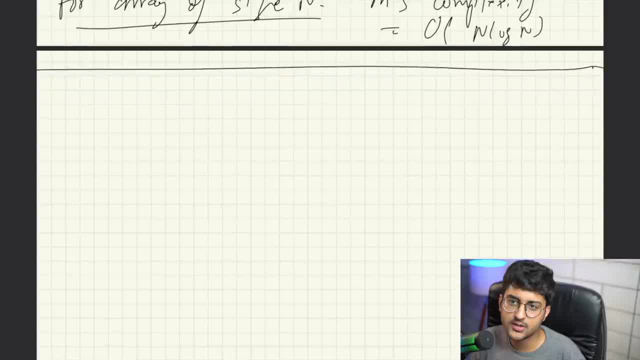 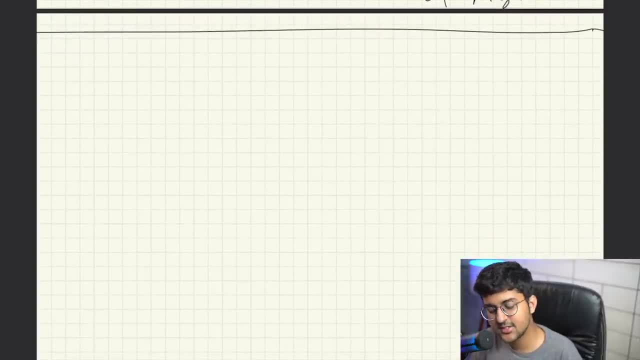 know that this is nothing, but people will say: hey, kunal, you want to sort, you want to get the complexity of merge sort? some people will comment on this video: just draw the diagram, kunal. you want the complexity? just use master theorem. just a few cases, via just a few cases, kunal, you can solve. 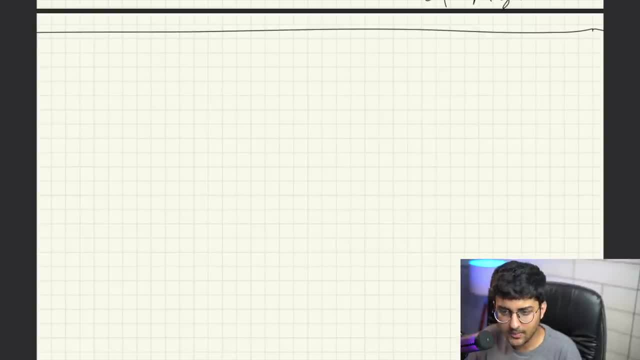 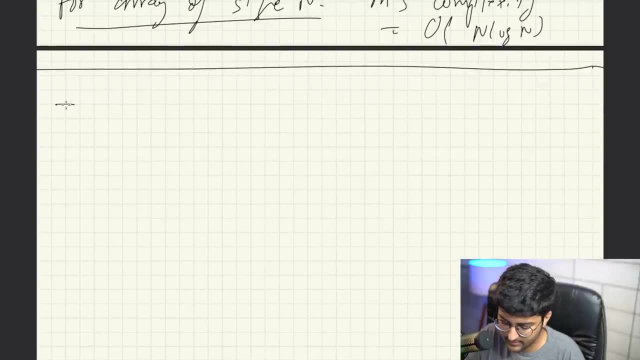 master's theorem, you can solve the complexity of merge sort. okay, people try to solve this using your- you know- tree method. try to make a recursion tree for this. if i make something like t of n question: t of n is equal to 2, t of n by 2 plus 8 by 9, t of, let's say, 3 n by 4 plus n squared. solve this with. 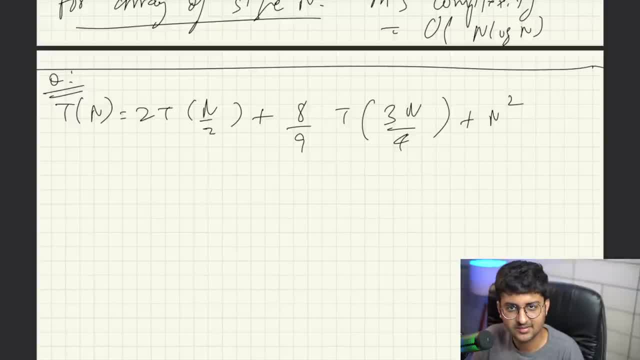 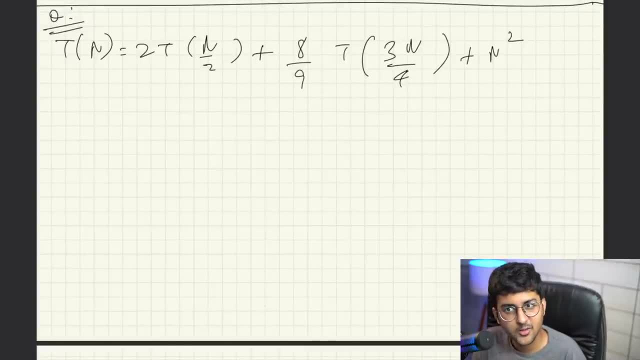 master theorem. solve this with master theorem. solve this via making a tree. these questions are asked in like btech also. solve this with tree. you will not be able to do it with akrabazi. i will do it just because i don't know how to do it. but i will do it just because i don't know how to do it. 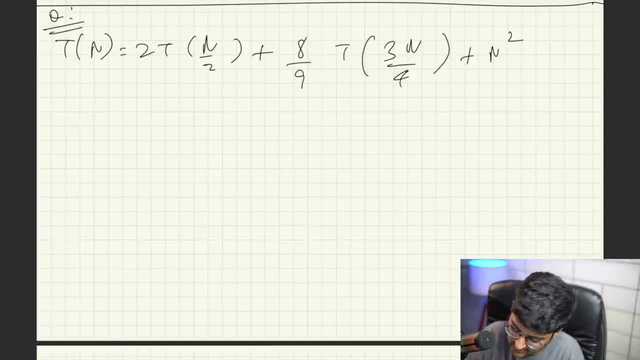 just like this, shall we? let's do it first. find the value of p. okay, finding the value of p a 1 is equal to this: a 1, b 1, a 2, b, 2. that's it. so a 1 into b 1, 2 into 1 upon 2, raised to power: p plus. 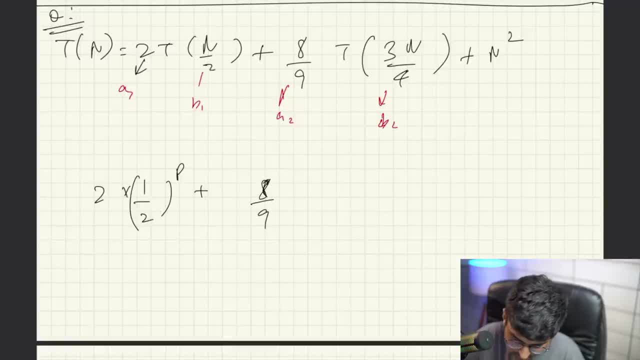 a 2 into b 2, 8 upon 9 into what is b2. b2 is actually, yeah, 3 upon 4 into 3 upon 4edu a for x a 2. b2 a one will be equal to six times a woods. Celsius current range is not this, but just. so let me just write this in this trunkasant function. so it is the 29thcı lagi commonide of lag boost, and that's what next is b2i volt. it will take the volume of a & b. so this is because we will number. 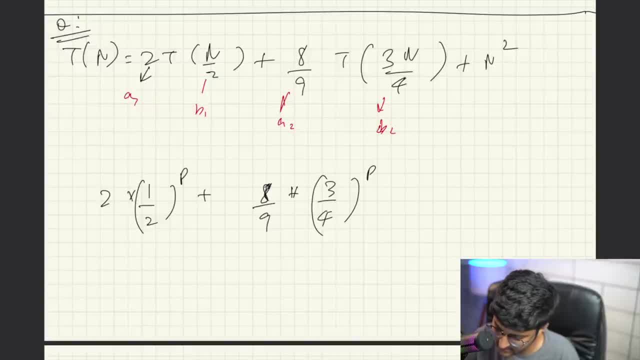 on 4 raised to power. p, that's it. we don't have a3 and b3 should give me one. so what is the value of p going to be if i put, let's say, p is equal to 2? it might be some. sometimes it might be possible. 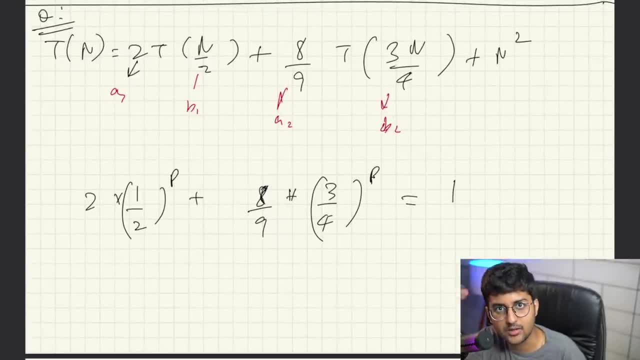 you will not be getting the value of p there. i will teach you very other simple way you will get without even doing any integration. you will get the answer without doing integration. you will get the answer. so next level techniques i'm teaching you in this video. please subscribe, i will highly. 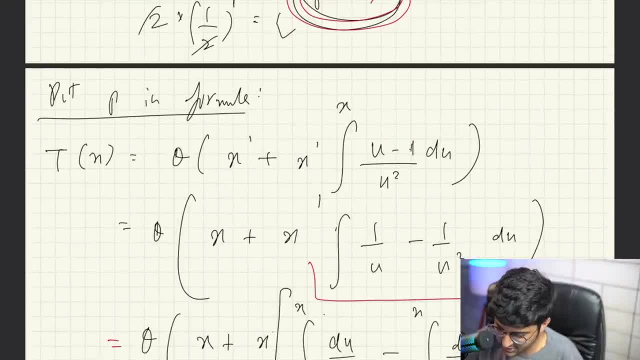 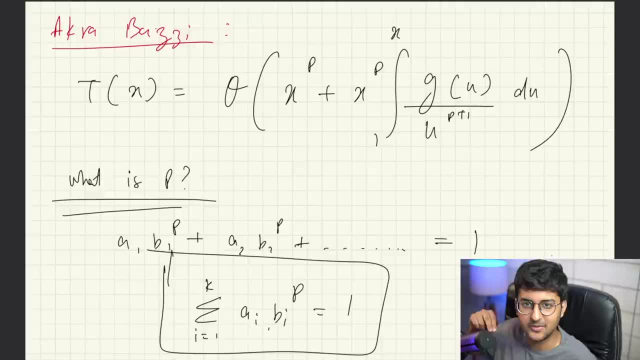 appreciate it and let's you know also. take a screenshot of this. take a screenshot of this and share it on socials so that other people can find out and share your views about akrabasi formula. all right, hope you took a screenshot and i'll now retweet and everything. 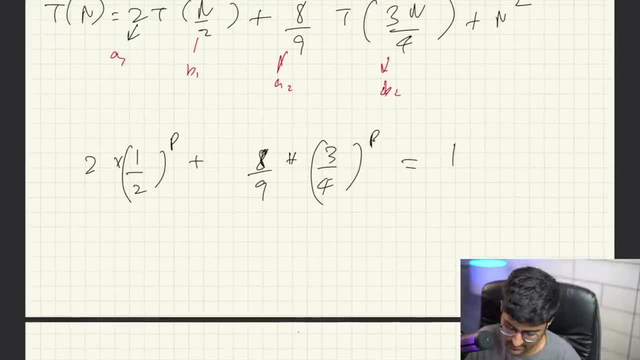 cool. so let's try to solve this very simple p. if i put equal to 2, it will be 2 into 1 upon 4, plus 8 by 9 into uh, 9 upon 16 should give me 1. that is true because this will be 1 upon 2. this will be. 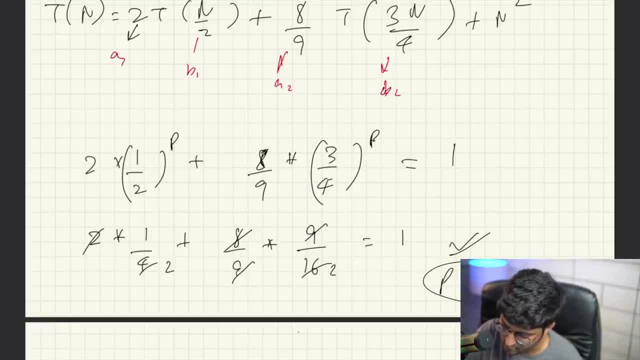 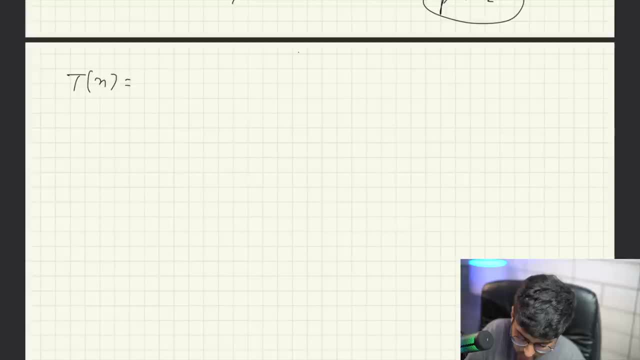 cancelled out: 1 upon 2 plus 1 upon. this is true. yeah, p is equal to 2. okay, p is equal to 2. let's try to put it in a formula so i can say: t of x is equal to theta of x raised to power p, which is this plus x raise to power p, integral. 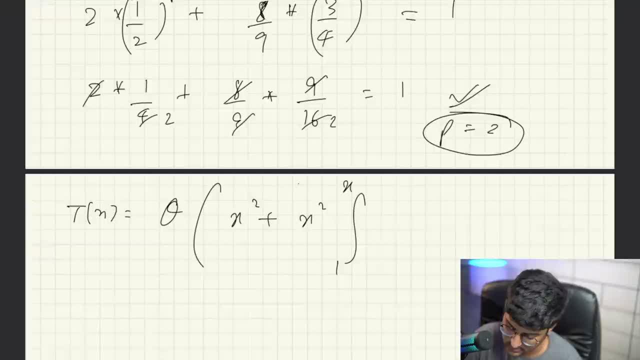 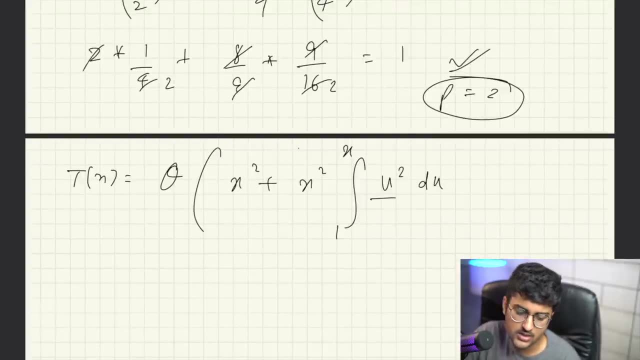 1 till x. uh d of u, which is uh, sorry. g of u, which is what is u? u is equal to n square, so u square d u upon u raise to power. p plus 1 means uh, 2 plus 1, which is 3 u cube, what is this equal to? 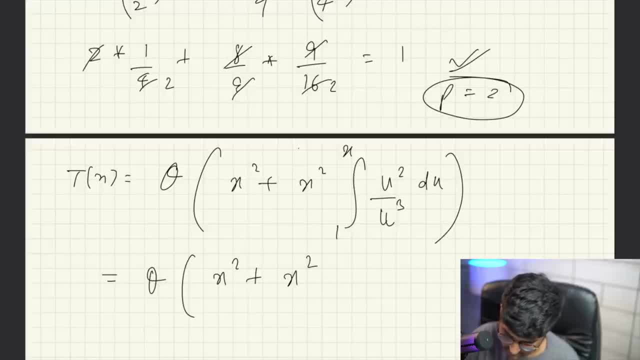 is actually equal to theta of x square plus x square. this is just 1 upon u, d u upon u, which is equal to log u. so 1 till x of log u gives me log x. this is going to be log x. ignoring the less dominating terms, this gives me theta of x square, log x. very simple, just three. 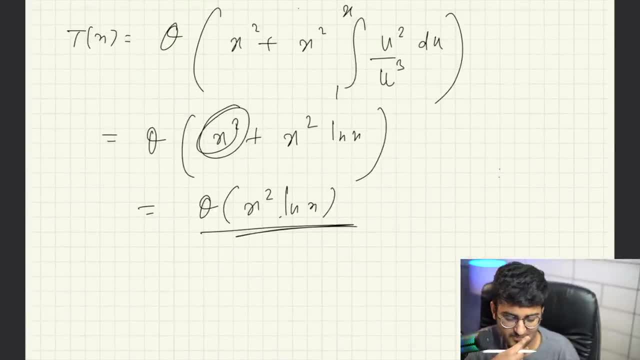 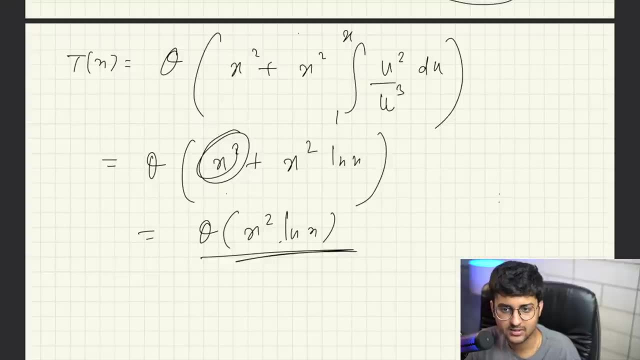 lines: that's it. that is it. how simple was this? in some cases you will get answers. you know, in b tech and stuff they ask something like: uh, i tell you a story. i was at a institute, i was like teaching over there, and they, there was this. 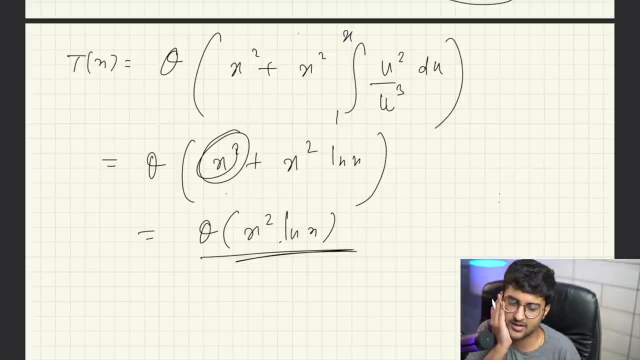 guy from dt. he was in final year. he was like i was like what happened? he was like they had my could, i had my exam and i did not. i was not able to solve these complexity questions and i'm like, okay, why didn't you? just, you know, it's very simple. and he was like why don't you do it? and i did it. 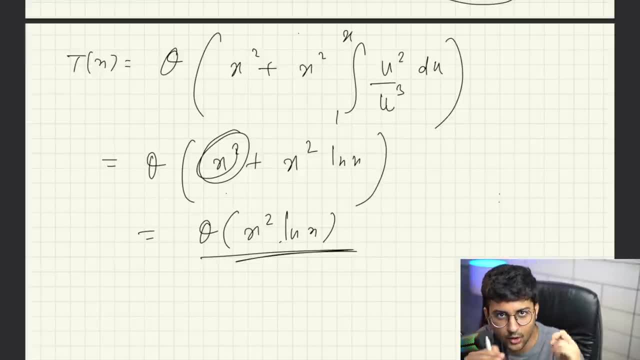 and actually got the exact answer. the exact answer was like log n raised to power, five upon eight was some answer. he was like dude, how did you even get five upon eight in the power? i was like it's simple, akrabasi integration. that's it. even the most complex answers, you will be able. 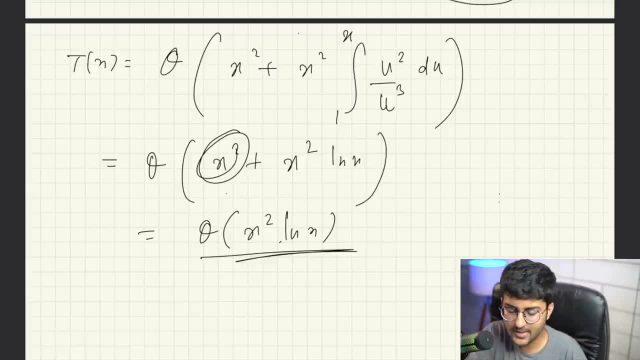 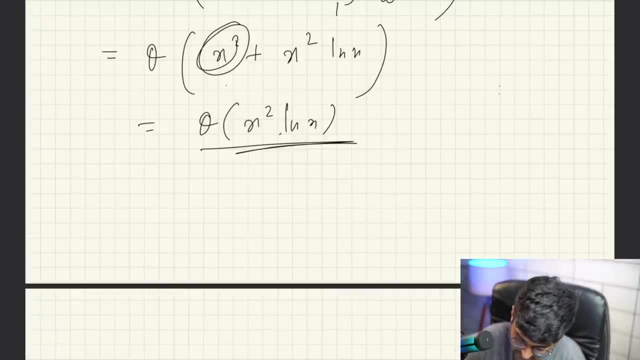 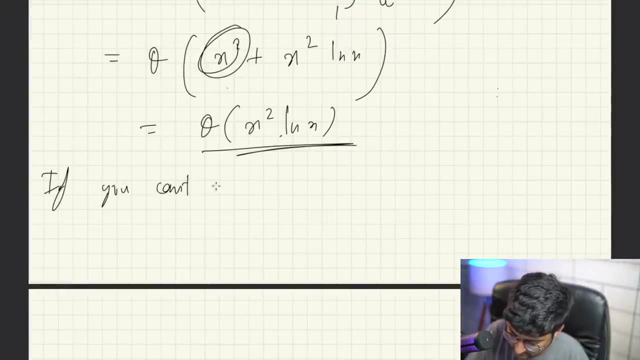 to get like this, so it's a very great technique. now it might be possible that you are running into a case where you are not able to find, let's say, the value of p. okay, that also might be a possibility. let's say, uh, if you're not finding value of p, i will cover that also if you can't. 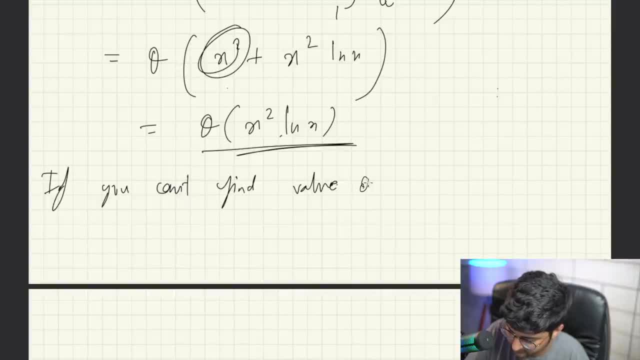 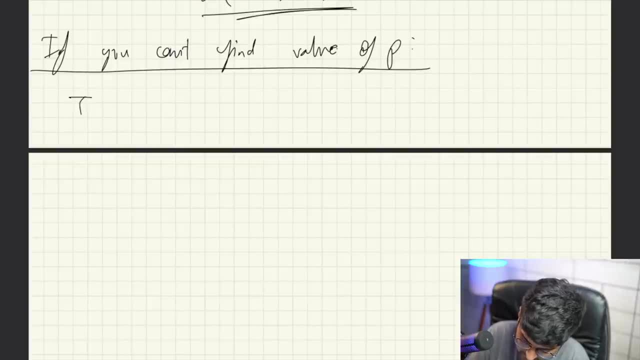 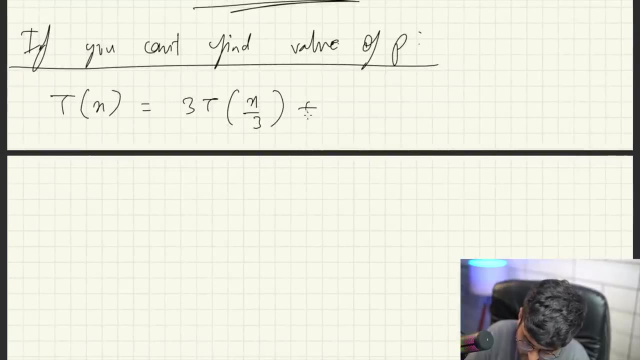 find value of p, then there will be a case where you can't find value of p. then there will be a case over here. okay, so let's say you're given a question like this. let's say you're given question like t of n, t of x or whatever is equal to, let's say, 3 t of x by 3 plus 4, t of x by 4 plus x squared. 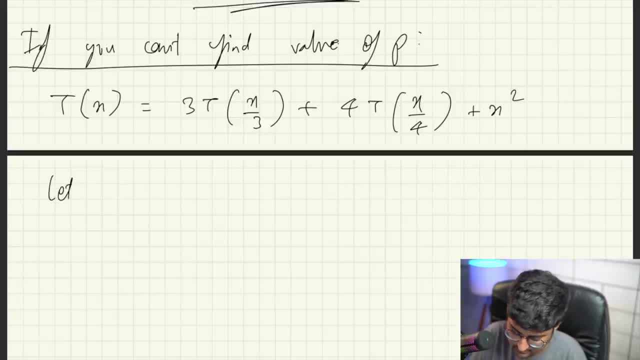 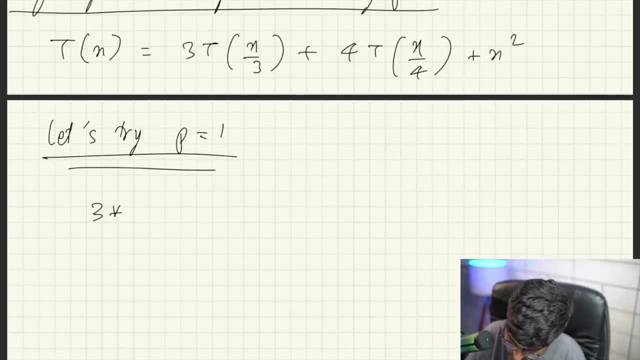 okay, so in order to finding t, let's try mm-hmm, let's try. p is equal to one, let's try. p is equal to to 1, so let i p is equal to 1 and 3 into 1 upon 3 raised to power: 1 plus 4 into 1 upon 4 raised. 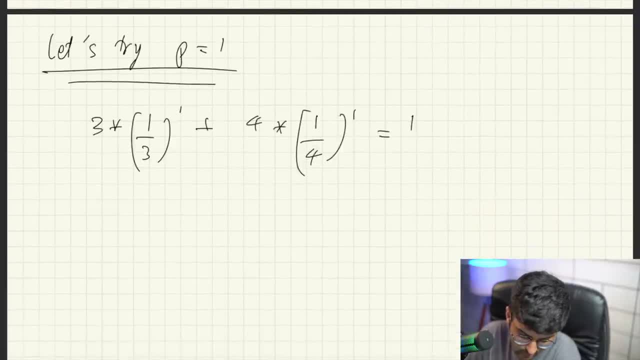 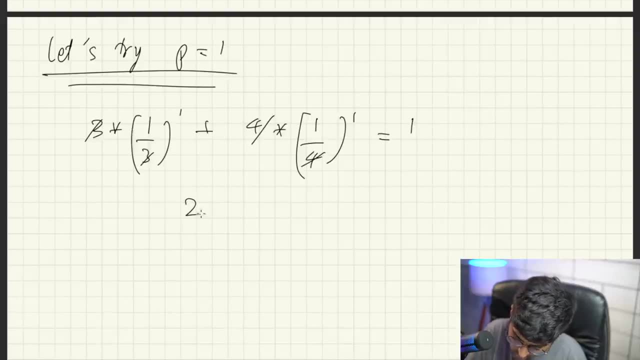 to power. 1 should give me 1. this is actually giving me equal to. what it's actually giving me equal to 2, and 2, i know, is greater than 1. okay, 2 is greater than 1. this means what i need to increase, uh, increase these denominators, right, and in order to for do for doing that, i need to. 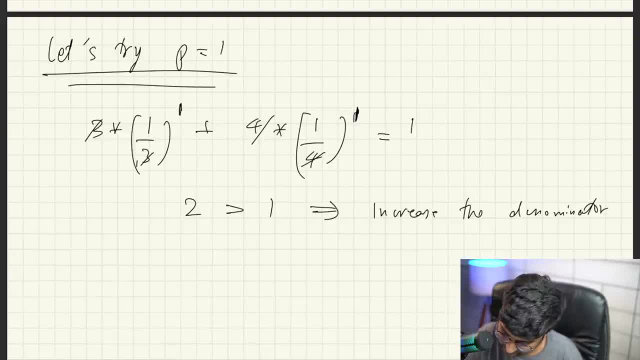 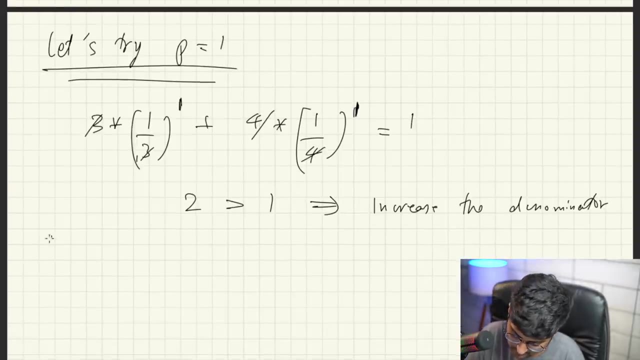 increase the uh, increase the power. if i want to increase the denominator, i have to increase the power. make sense. hence i know that p is definitely greater than 1.. make sense: p is greater than 1. that is the conclusion. p is greater than 1.. let's try 2, let's try 2. so if i say p is equal to 2, then i can say it's like 3 into 1 upon 9 plus. 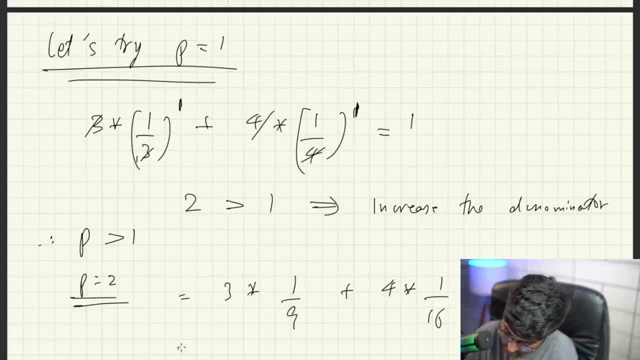 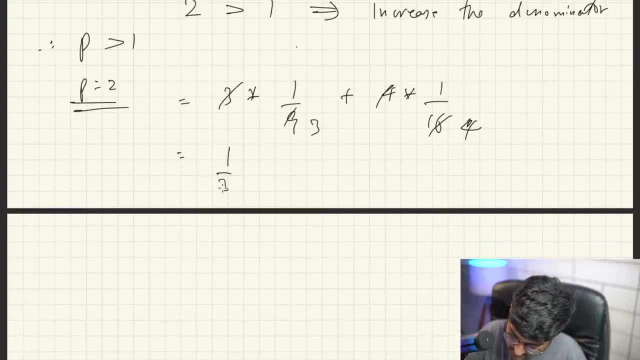 4 into 1 upon 16.. so this is equal to something like 1 upon 3 in plus 1 upon 4. so 1 upon 3 plus 1 upon 4 is equal to 4 plus 3 divided by 12. 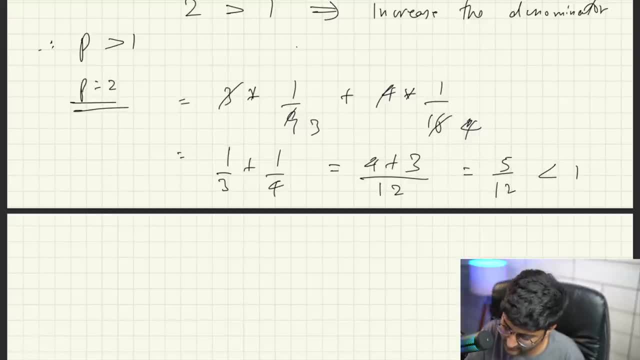 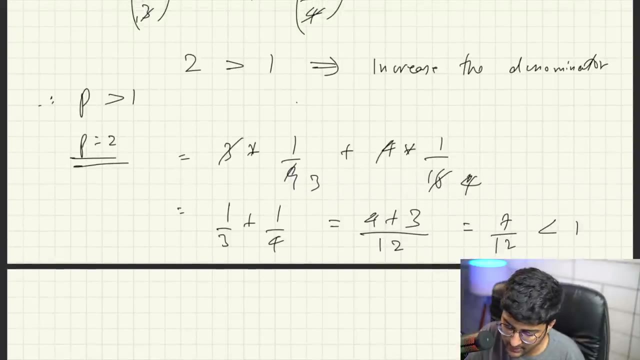 5 upon 12. this is less than 1, sorry, not 5 upon 12. 7 upon 12: still less than 1. okay, cool. so this means that i need to increase the value of these whole this, these particular thing, in order to do, in order to increase the value of a fraction, i need to. 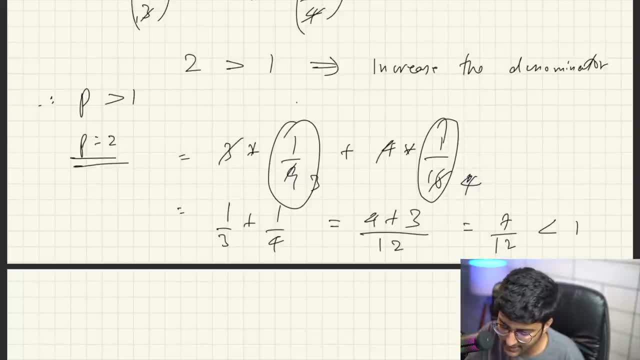 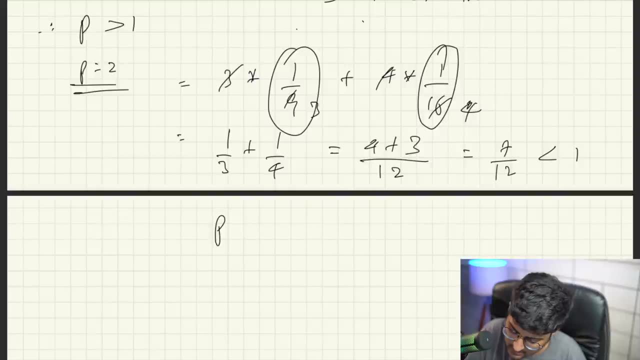 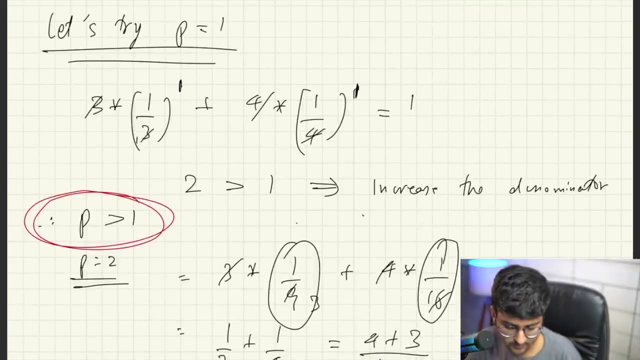 decrease the value of the denominator. if i want to decrease the value of denominator, hence i have to decrease the value of p. it's also very simple. hence i know that p is definitely less than 2.. hence i know p is definitely less than 2.. point number one. point number two: i know p actually now lies in my range one and two. 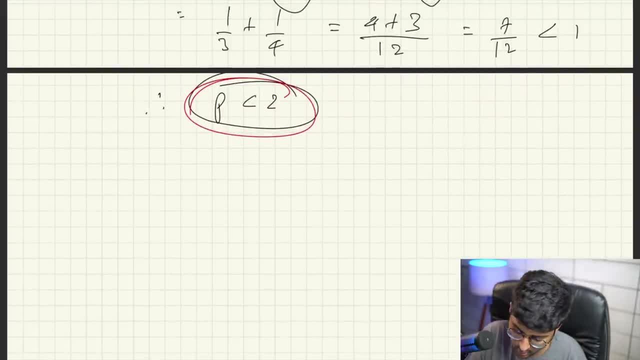 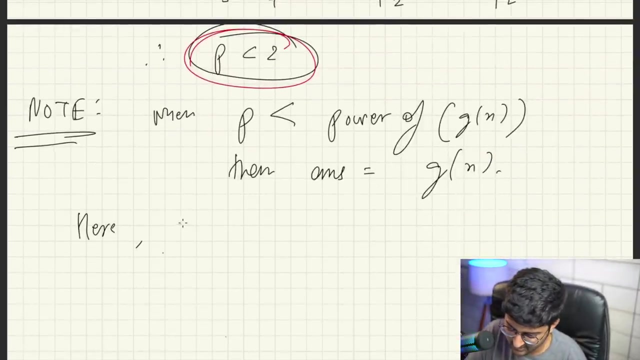 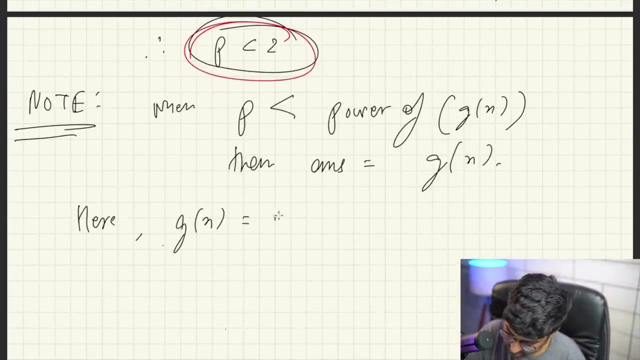 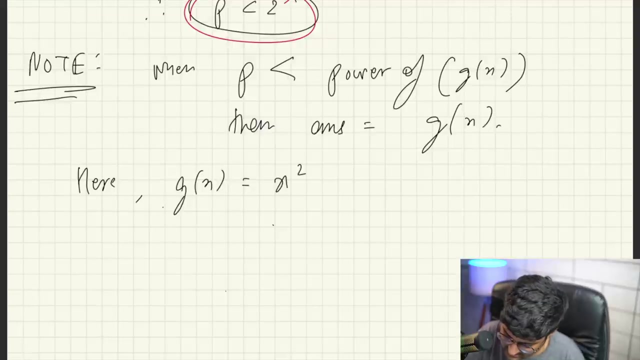 so the thing that you can note over here is what note: when p is actually less than the power of g of x, then answer is equal to g of x. here, what is g of x? here? g of x is equal to what? in this question, x square okay and p is actually less than the power of g of x means p is less than. 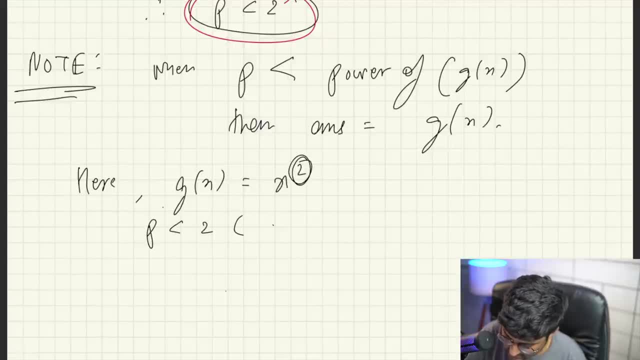 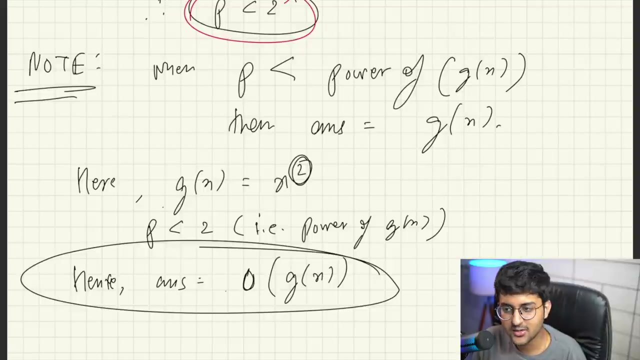 2. p is less than the power of g of x. p is less than 2. that is equal to p power of g of x. hence, answer is equal to big o of g of x. that's it. no need to do integration. very cool stuff, am i asking? you may ask questions like kunal, why. 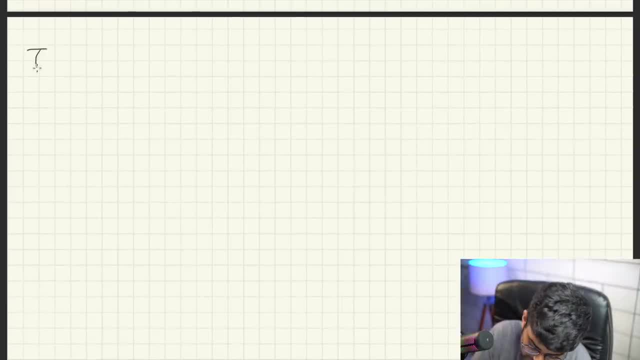 what might be the reason? okay, no problem. so let's say you have something like this, the acrabazi formula: x raised to power p plus x raised to power p, 1 upon x. what is, what is my g of x over here? u square, uh. u raised to power p plus 1. let's say: i don't know, i don't know what. 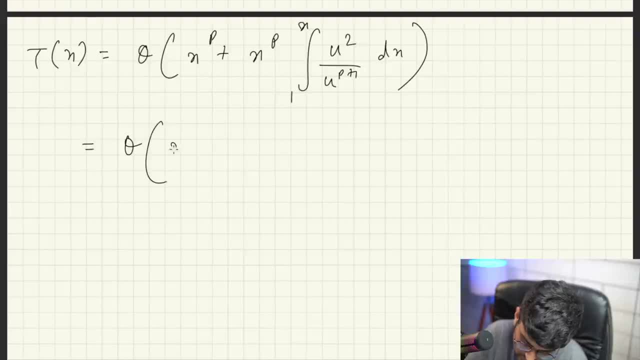 p is. so i am just putting p over here- is actually equal to theta of x raised to power p. if you solve it, x raised to power p. if you solve this entire thing, p it's going to be minus 1 minus p. 2 minus 1 minus p will be 1 minus p. 1 upon x, 1 into a 1, 1 and 1 till x 1 minus p du. if i try to solve this, 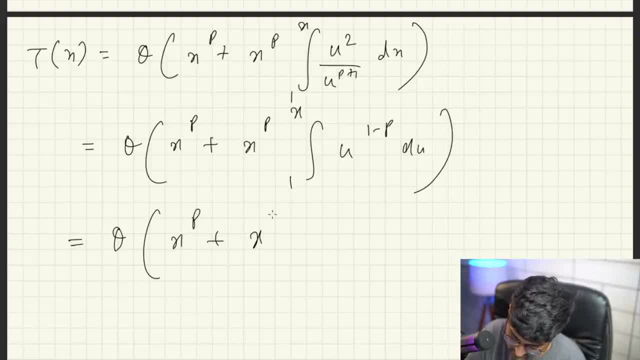 this is going to give me x raised to power p plus x raised to power 2. okay, and since i know, since i know that p is actually less than 2, this will become less dominating term, hence ignore. so answer is g of n is the answer. 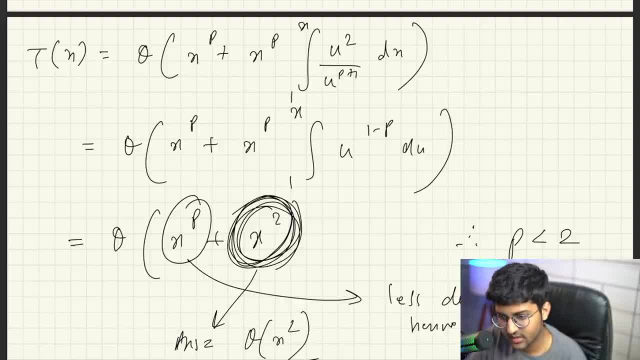 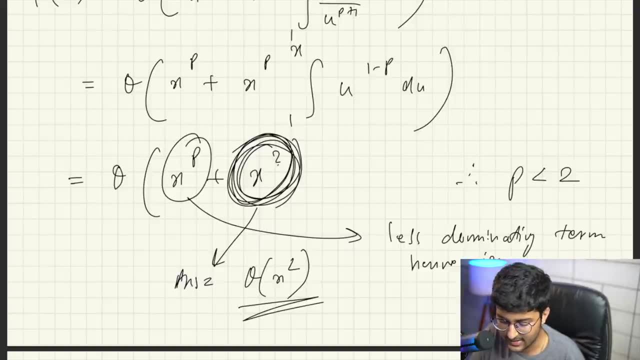 very, very cool stuff. it's very simple. i know p is less than 2, p is less than the power of this. in that case, just ignore very cool stuff. the answer here is g of x itself. all right, cool stuff, great. so that was how you can solve any. 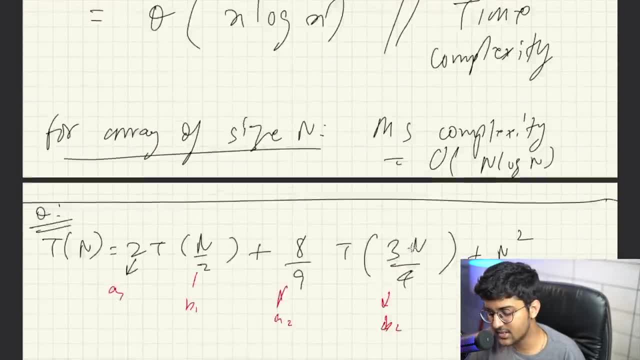 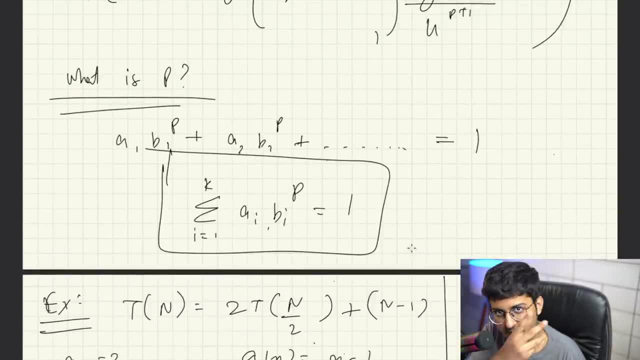 problem. so that was how you can solve any problem. so that was how you can solve any recurrence relation of divide and conquer. only thing remaining now is linear recurrence relations. this is very next level stuff. we will get a single formula for nth. when nth Fibonacci number, no need. 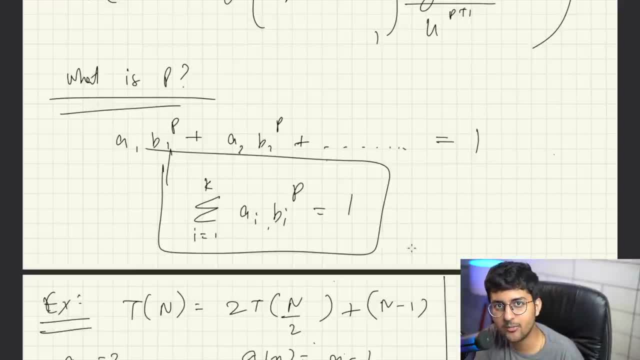 to run loop. no need to run recursion, just put the answer in that formula. you will get answer in one single step, the exact time, complexity of any formula and everything we will get. for just like we did for this, we will also do it for linear recurrence relations. all right, so that's the last. 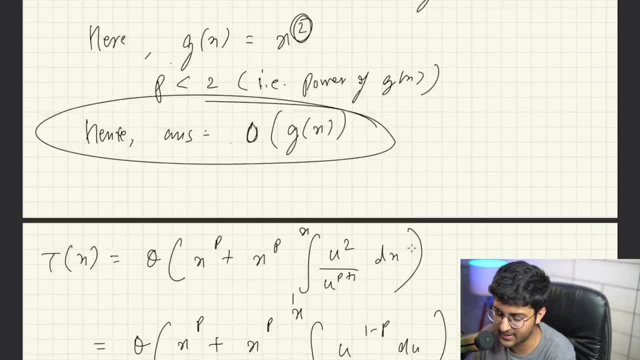 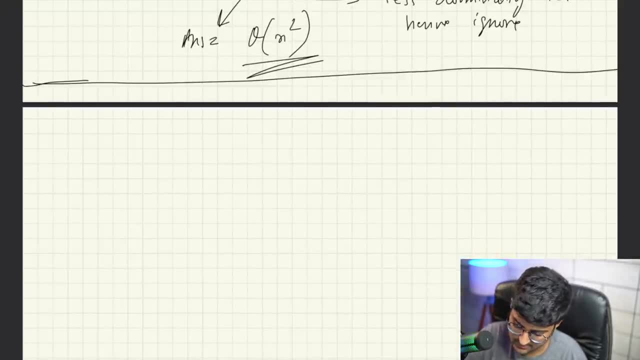 topic. please listen very carefully. it's a very important topic as well, even for btech, so definitely we can get started with that right now, which is linear recurrences- solving linear recurrences. we have another method for this. i hope you all had fun with akrabasi. now it's time. 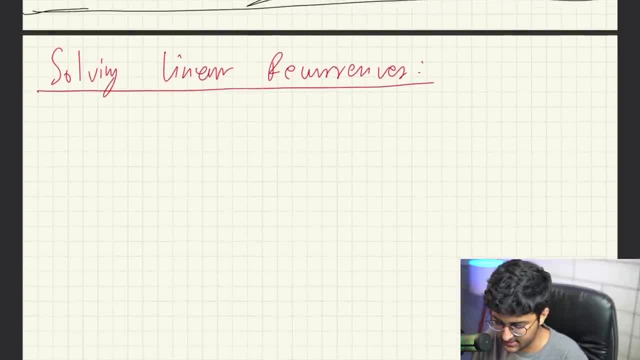 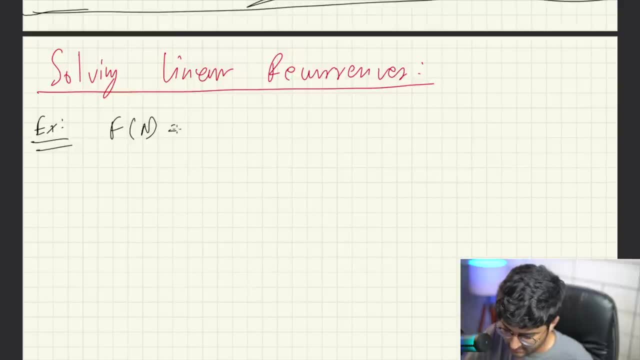 to solve linear recurrences. so let's try to solve linear recurrence relations. let's take an example. first, you, I had the Fibonacci number right. I said: nth Fibonacci number is equal to n minus first Fibonacci number plus n minus second Fibonacci number. that's very simple stuff. I just said like okay. 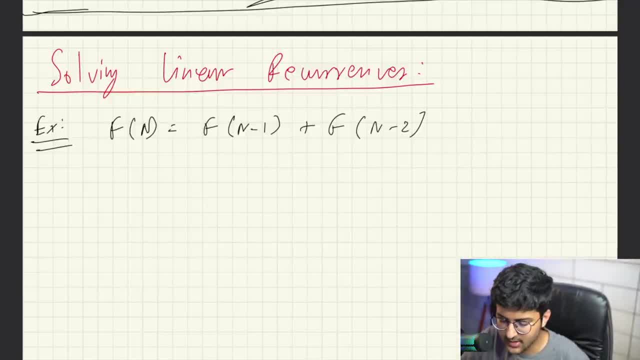 now, that's not divide and conquer, it's actually n minus 1, n minus 2 can be like there might be like a form for this as well. it's like we said there was a form for linear divide and conquer recurrence relations. what is the form of linear recurrence relations form? form is something like this: f of: 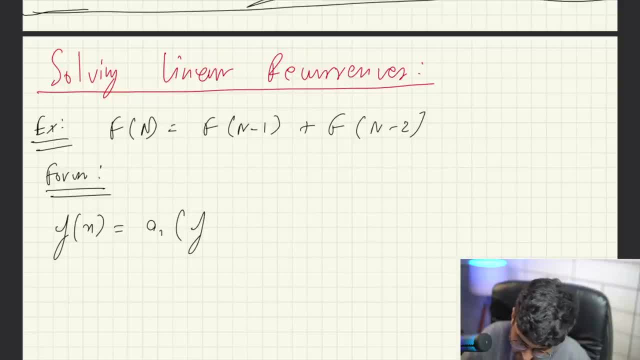 x is equal to a 1 f of x minus 1, sorry, so something like this, plus a 2 f of n minus 2, plus a 3 f of n minus 3 a of n oruser at least known as a 1 f of x minus 2kay, doesn't make so what we need. there's two more variables, which means that a 3 f of x close to n has to break, and it has to break is a n-n, and that's then. instead of a 1, we take a 1f of a 2f x minus 1 equals to a1 plus an x 1 minus 2 plus a 2f x minus 1.. 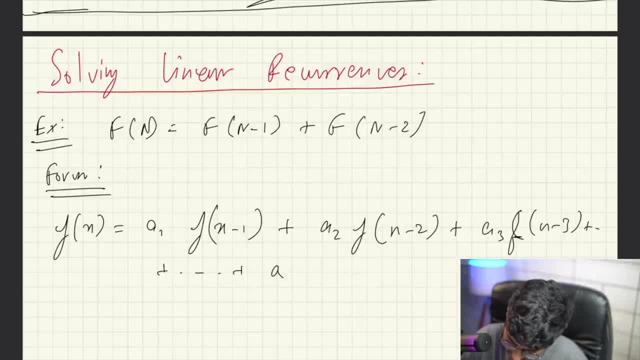 a of n, or, yeah, a x, x minus 3, a of n, x of sorry, a of n, f of x minus and something like that. okay, this can be like f of n. f of x is equal to i is equal to 1 till n can be like a of i. 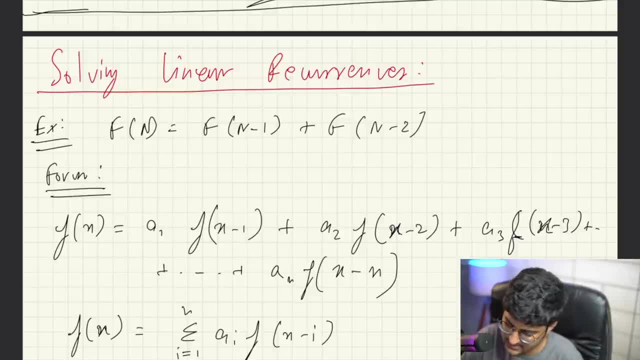 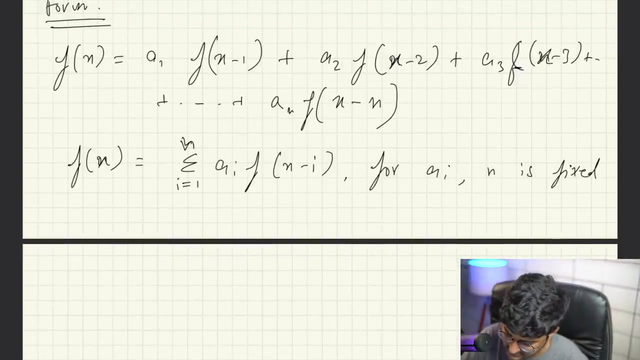 f of x minus i. that is it for for a of i, and, and this particular n is fixed, and i know that you might not be able to see it and i know that what is n, n is like the order order of recurrence, order of which we'll talk more about later. recurrence. 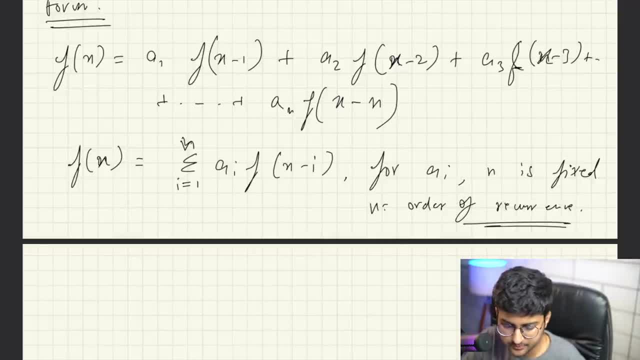 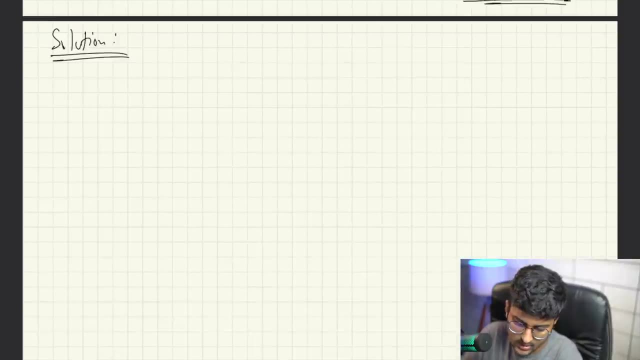 all right, cool. so how do we solve this problem? there are actually two ways which you can solve such problems. so let's see, let's see the solution. let's just not not just just directly. we can see the solution, so i will write this in the points: 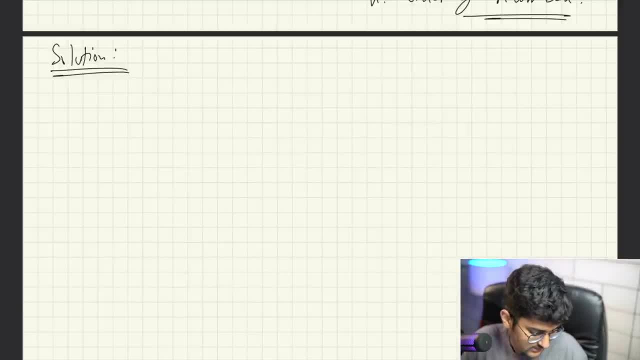 okay, so i'll write it in points and after that you can um follow these points and it will be good for revision as well. so i'm trying to solve this recurrence problem, which is, let's say, we're trying to solve solution for, let's say, fibonacci number. 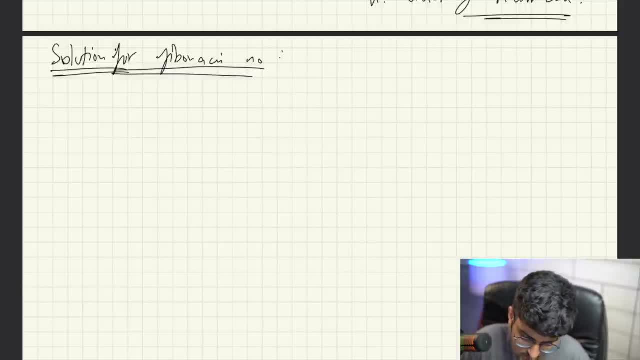 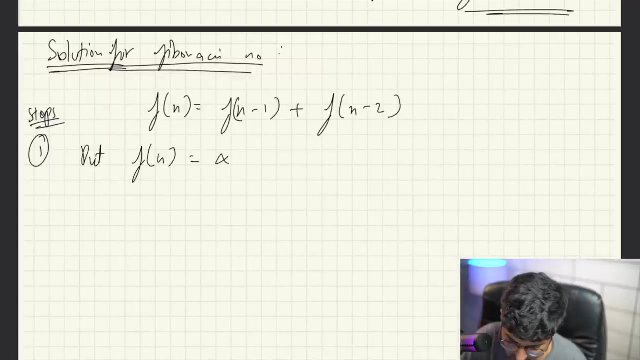 relation. okay, so you're saying okay, um, you can say f of n is equal to f of n minus 1 plus f of n minus 2. let's try to solve this. what is step number one steps? step number one is put: f of n is equal to alpha raised to power n for some constant alpha, we don't know the value of. 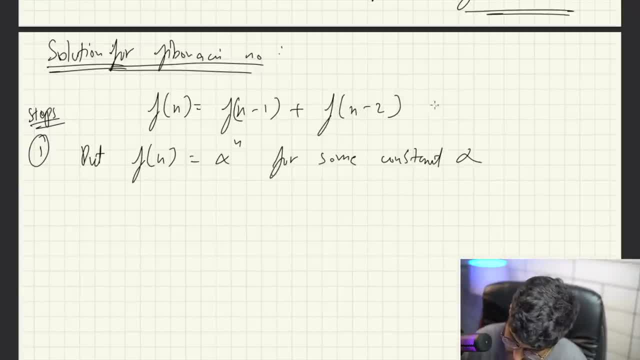 this, we're just putting it so we can put: okay, if i put this in equation number one, it will become what it will become: alpha raised to power n. this is going to be equal to alpha raised to power n, which is equal to alpha raised to power n minus 1 plus alpha raised to power n minus 2. because if 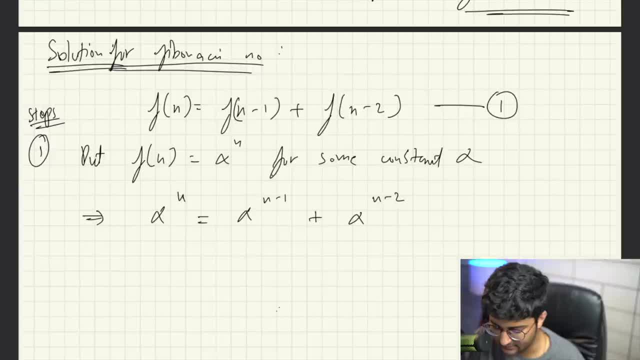 f of n is equal to alpha raised to power n. f of n minus 1 is alpha raised to power n minus 1. f of n minus 2 is equal to alpha raised to power n minus 2. okay, if i bring this over here, i can say: 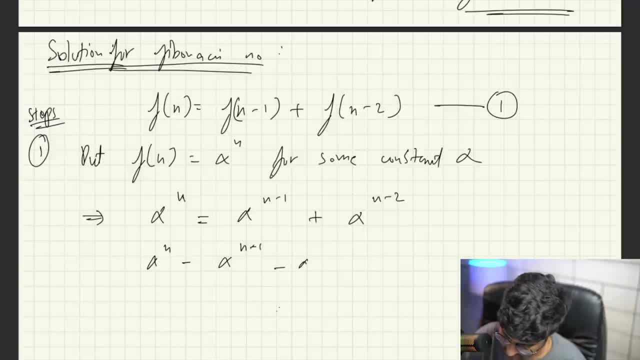 alpha n minus alpha n minus 1 minus alpha n minus 2 is equal to 0. i can divide this by n minus 2. if i divide this n by n minus 2, it will become what i don't think i should be able to elaborate. 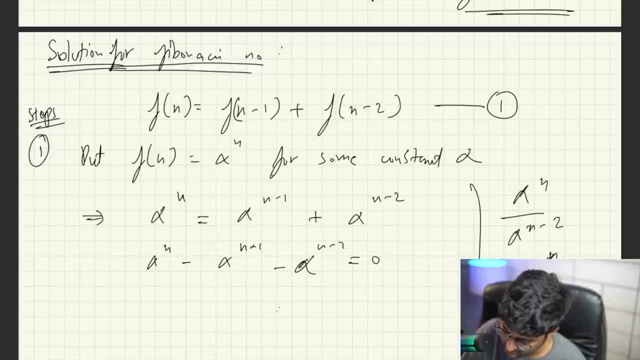 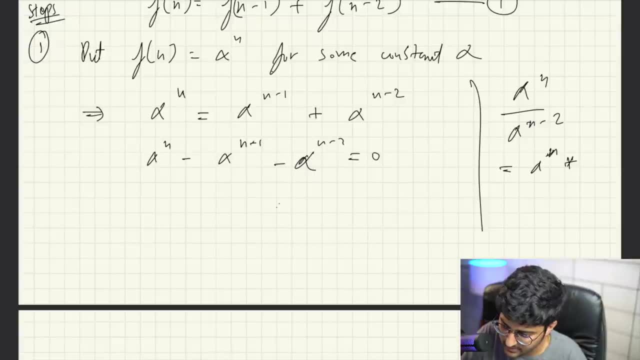 this, but n minus 2 is actually equal to alpha. n into n minus 2 basically means what? this is very simple, very simple math, mathematics. anything in the negative power. it basically means alpha square divided by n minus. let's just this alpha square. you know right, alpha raised to power minus 1 is equal to alpha. 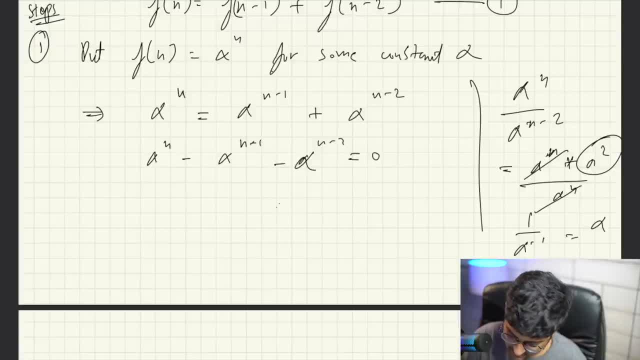 very simple mathematics. okay, this will actually then become alpha square minus. alpha minus n is equal to 0 if i divide by alpha n minus 2. okay, this is what it will become dividing lhs and rhs. so no value. no such will be changed as such, so this is actually equal to this. it's very simple stuff. now i can take step. 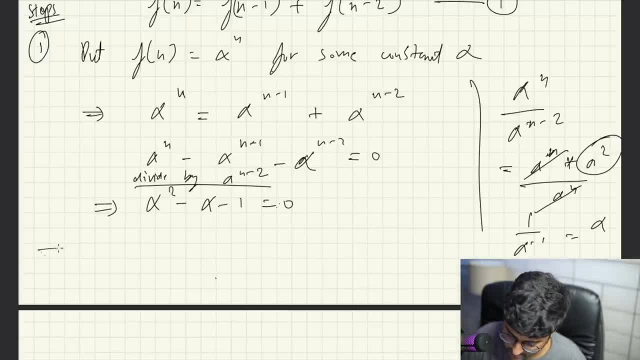 number two i can take like roots of this: what are the roots of this going to be? roots of this are going to be uh minus b plus minus uh b square minus 4ac divided by 2a. so roots of quadratic equation, roots of this equation, this quadratic equation, this quadratic equation we learned. 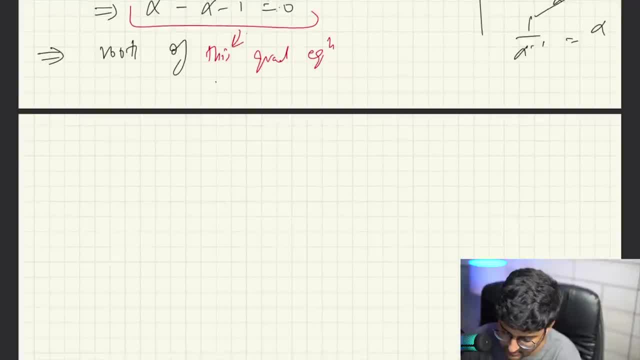 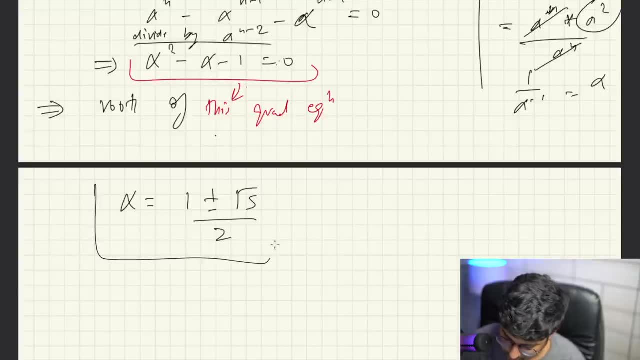 this in like high school 10th class, i think very simple stuff, or maybe before that, i don't remember- when we learned this. alpha is equal to, i can say 1 plus minus root, 5 by 2 from the formula of roots are equal to minus b plus minus b, square minus 4ac upon 2a. it's a very simple quadratic formula. 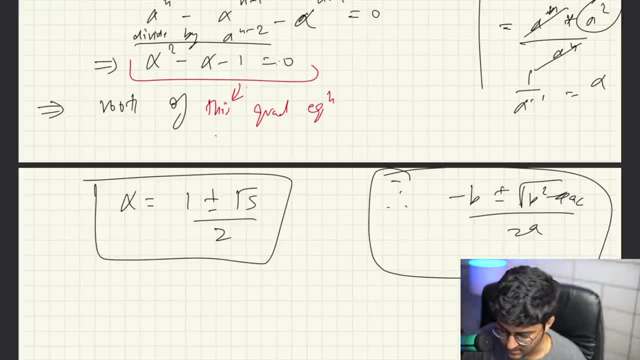 you can google this very simple. okay, a is 1, b is equal to minus 1, c is equal to minus 1. that's it okay. so these are the two roots. so i can say now, point number 2 is actually: you can write it somewhat like this: you can see two roots, so 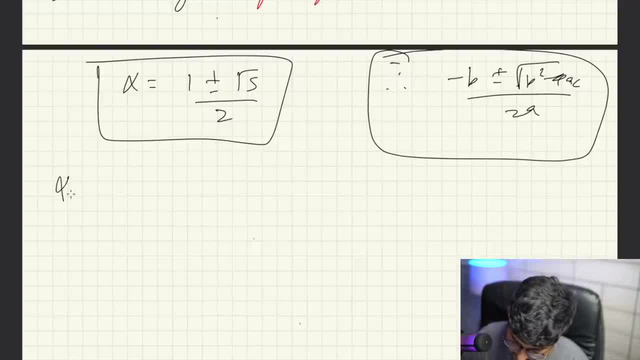 before point number 2. I can say root 1 and root 2. I can say alpha 1 is equal to, let's say, 1 plus root 5 by 2, and I can say alpha 2 is equal to 1 minus root 5 by 2. okay, so the fact is that if 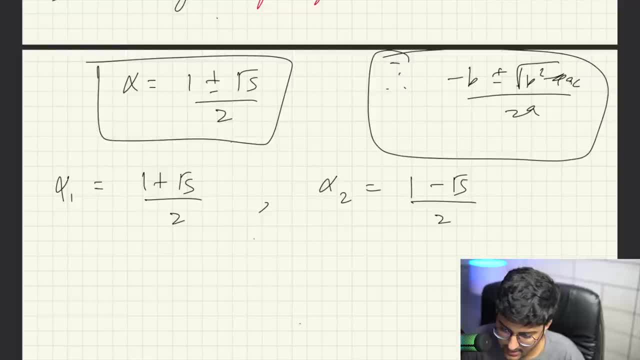 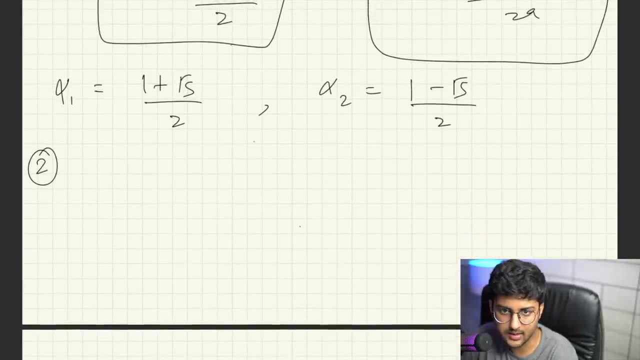 f of n is equal to, let's say, alpha alpha 1 raised to power n and alpha alpha 2 raised to power n, or whatever, are the solutions to this linear recurrence relation. okay, then I can say that point number 2- this is simple, like this- is mathematical part. so if you have 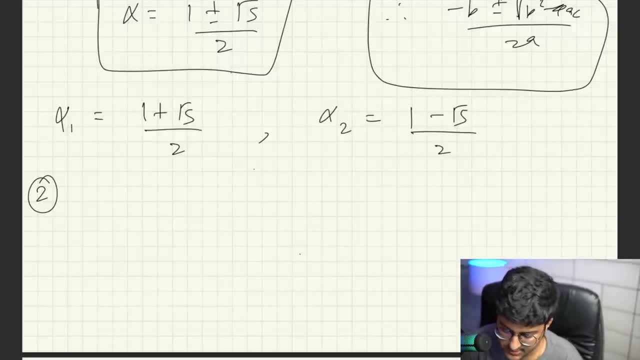 alpha 1 and alpha 2 as two roots. you can write the equation in such a way: f of n is equal to constant 1- alpha 1 raised to power n, plus constant 2- alpha 2 raised to power n. this is also a solution. 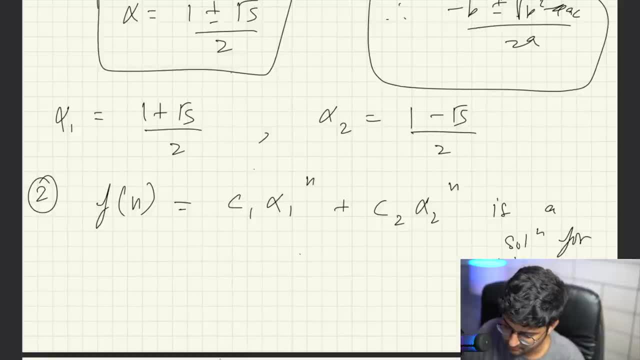 for Fibonacci. this is not just for this, any equation. you have the number of roots. okay, take that many number of constants and multiply that many number of roots with the power of n. add all that is going to be the same same. this is actually equal to f of n minus 1 plus f of n minus. 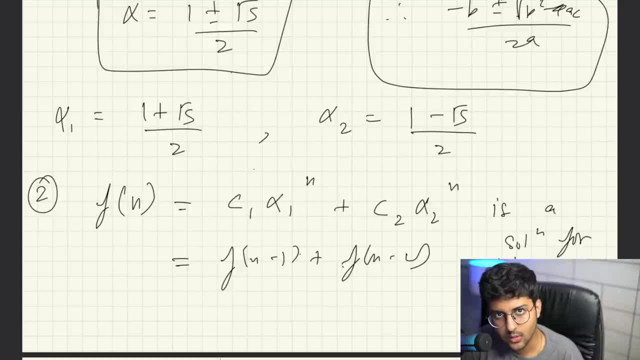 2. okay, sound good, cool. so for any constant, you can write the equation in such a way that if you have alpha 1 raised to power n, which is constant c1 and c2, so I can elaborate this into something like I can say: f of n is equal to. 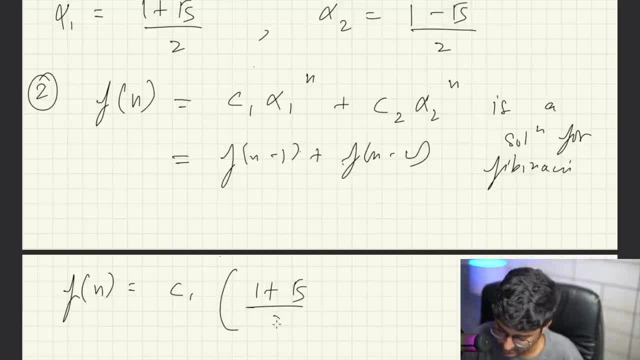 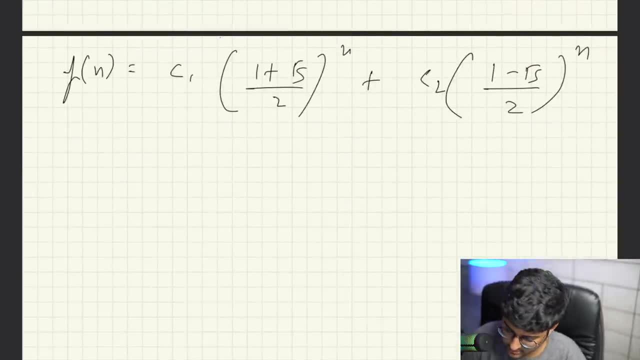 c1: 1 plus root, 5 by 2, raised to power n. plus c2: 1 minus root, 5 by 2, raised to power n. this is the equation that we have. equation number two: okay, so if you had three roots, if you had three roots, 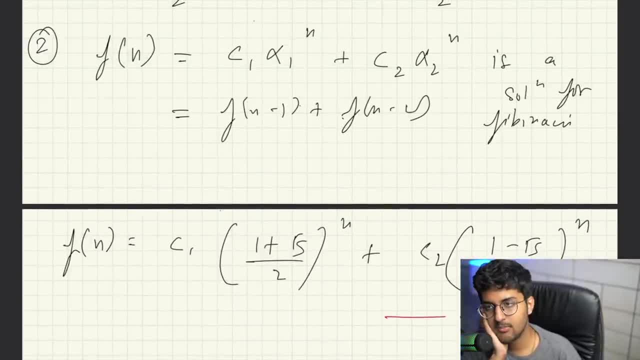 you will write something like c1 alpha 1, raised to power n, plus c2 alpha 2, which is root 2, raised to power n, plus c3 alpha 3 raised power n. very simple stuff, no problem, okay. third point. third point is very important. this is fact. 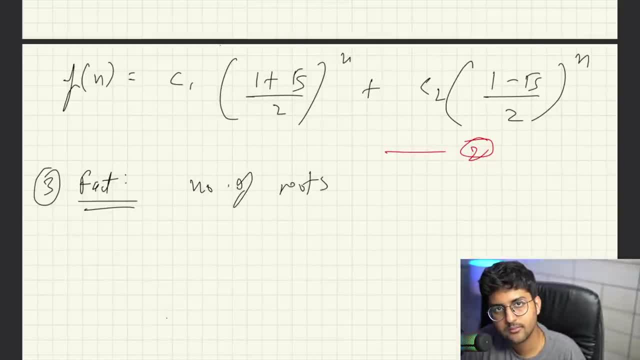 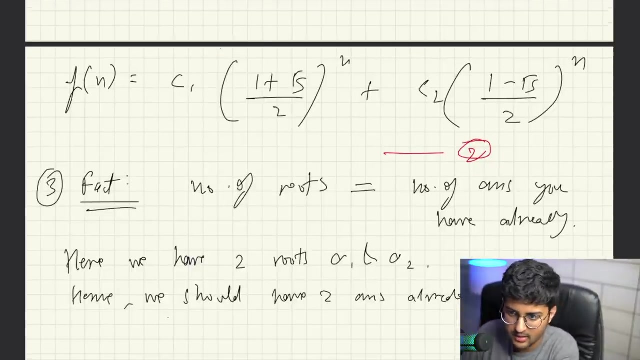 number of roots that you have. number of roots that you have is going to be equal to number of answers you have already. so here we have two roots: alpha 1 and alpha 2. hence, we should have two answers already, and we do. we do have two answers already. we know that. 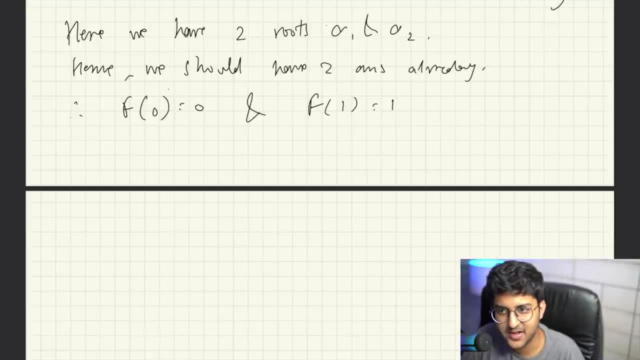 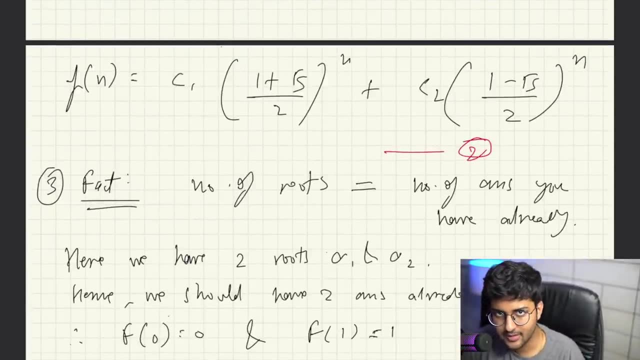 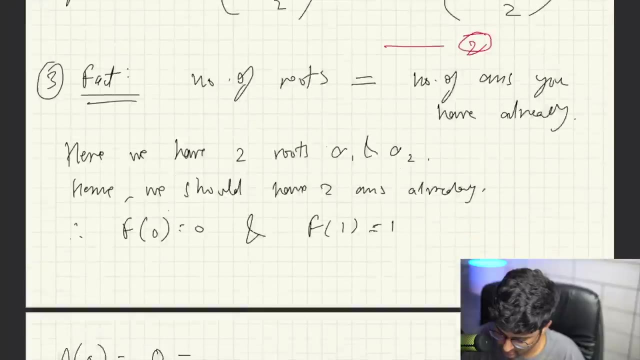 f of 0 is 0 and f of 1 is equal to 1. we have two answers already. this is another fact. when you have n number of roots, or any number of roots, you will have that many amount of answers already. i can try, for f is equal to 0, i can say f is f, 0 is equal to 0, is equal to, i put n is equal to 0. so 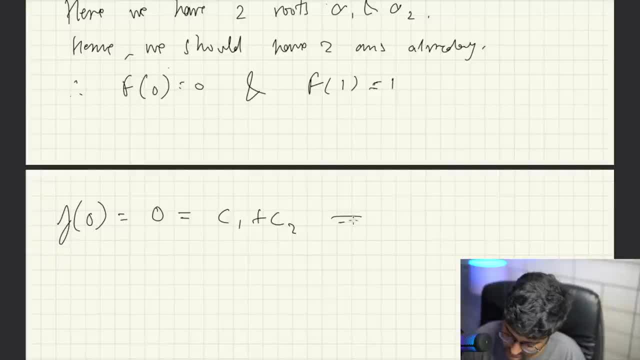 it will be c1 plus c2, c1 plus c2. this basically means c1 is equal to minus c2. question number 3: if i try, f is equal to 1. this should give me 1. this is equal to c1, 1 plus root 5 by 2 plus. 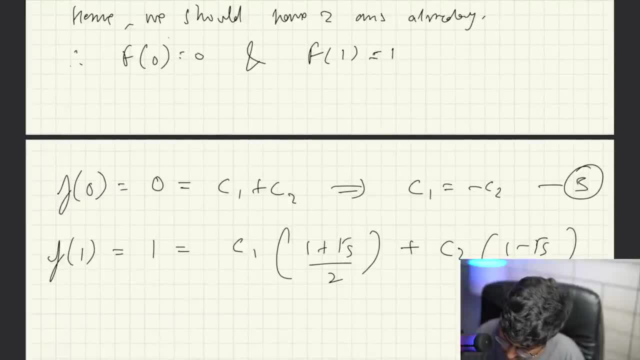 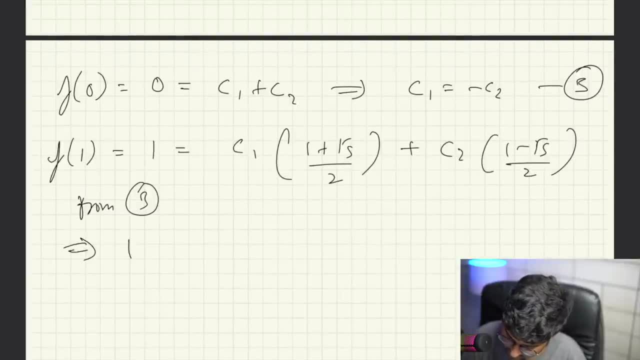 c21 minus root 5 by 2. right from 3, i can say something like this becomes: 1 is equal to c1, 1 plus root 5 by 2 minus c1, because c2 is equal to minus c1, 1 minus root 5 by 2. when you solve this, c1 comes out to be: 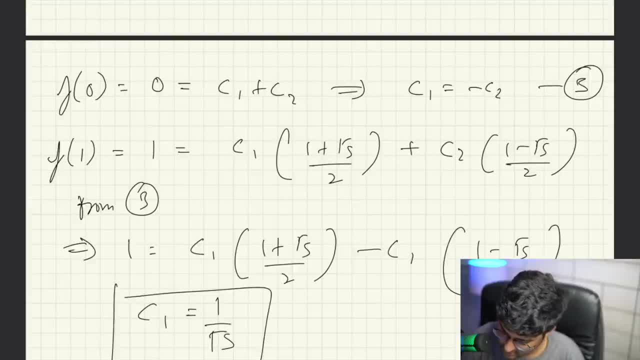 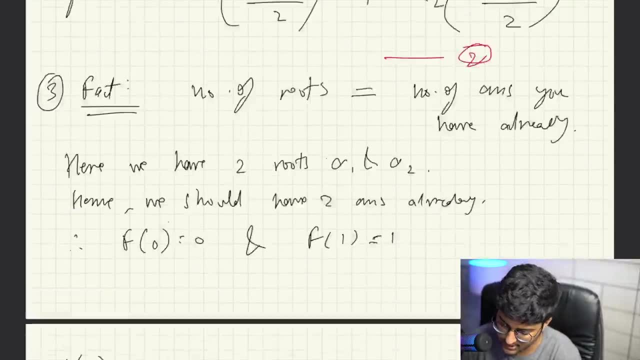 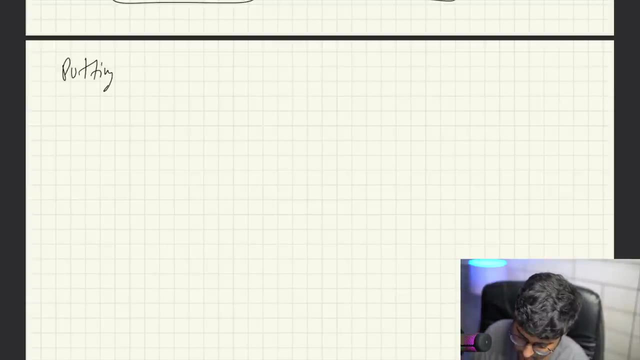 1 upon root 5 and c2 is equal to just the negative of this. c2 comes out to be minus 1 upon root 5. putting this the: putting this in my original equation, which is at: putting this in equation number 2. putting this in: 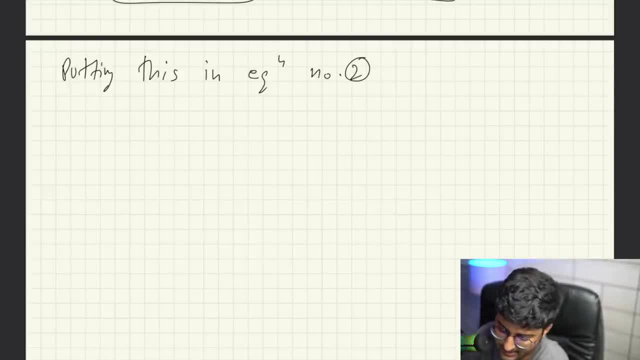 equation number 2, i get something like this: i say f of n is equal to 1 upon root 5, 1 plus root 5 by 2, raised to power: n minus 1 upon root 5, 1 minus root 5 upon 2. 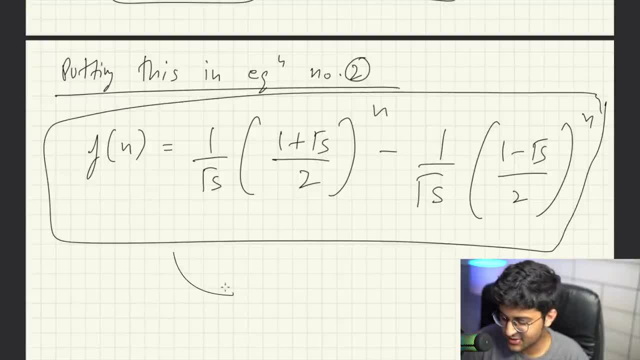 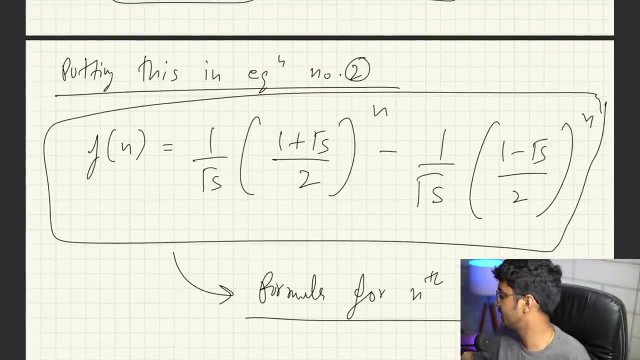 raised to power n. this is actually the formula for nth fibonacci number. how cool is this formula for nth fibonacci number? no need to run recursion, no need to do anything, just put the answer. just put the value in this answer and you will get. uh, just put the value of n over here, you will get. 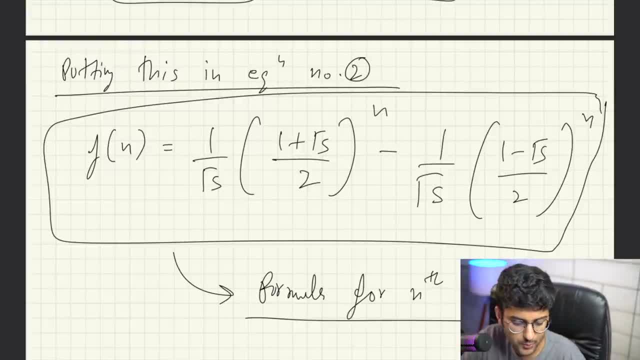 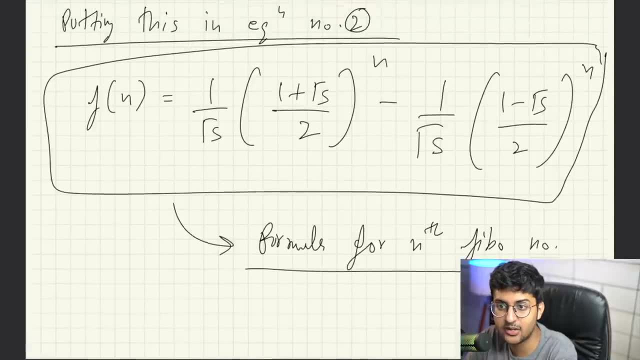 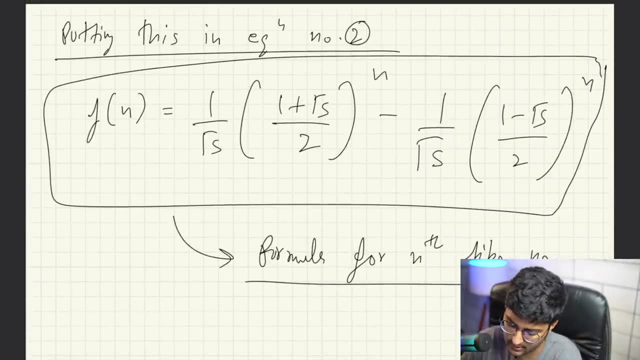 the nth fibonacci number. no need for recursion, no need to run any loop or anything, that's it. that's it. how cool is that? this is actually the formula for nth fibonacci number. okay, how do we get the time complexity from this? so if this is the nth fibonacci number formula. 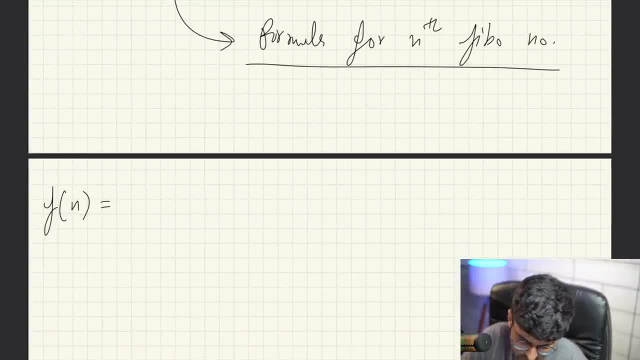 so you can see i can write it down something like this: f of n is equal to: i can take 1 upon root 5 common. this will be 1 plus root 5 by 2 raised to power n minus 1 minus root 5 by 2 raised. 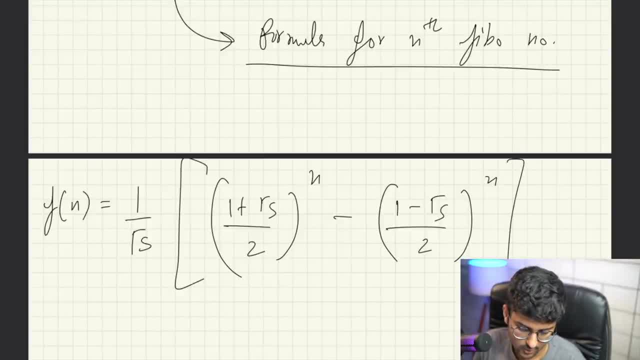 to power n? okay, very simple stuff. what is the actual value of this? what is the actual value of 1 plus root 5 by 2? um, what is the value of this thing if i'm talking about? what is the value of 1 plus root 5 by 2? it's 1.6 or something. 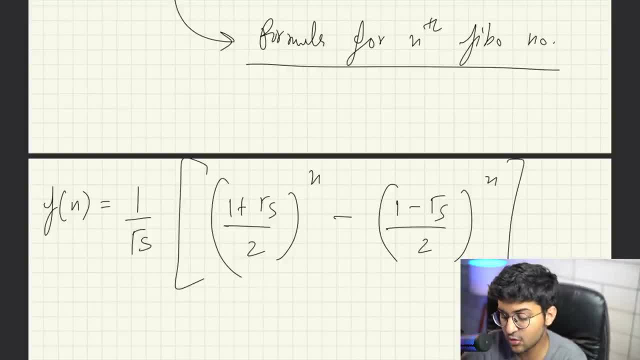 or if i talk about 1 minus root, 5 by 2, 1 minus root, 5 by 2 is actually equal to less than 1.. let's just try it out: 1 minus square root of 5, which is equal to actually equal to what is the? 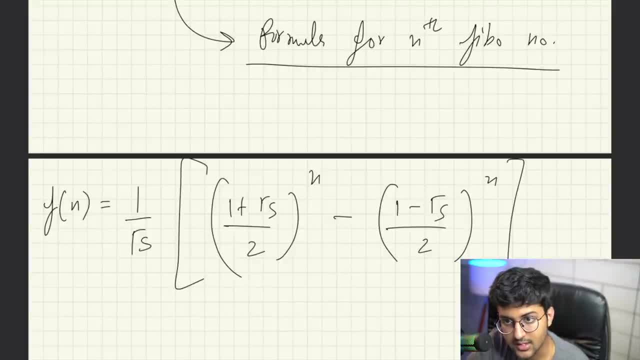 square root of 5, first of all. so it's actually negative. so 1 minus this entire, divided by 2, is how much? it's actually less than less than 1? it's 0.6, something okay. so i know that as n increases, as the value of n increases, tends to infinity. 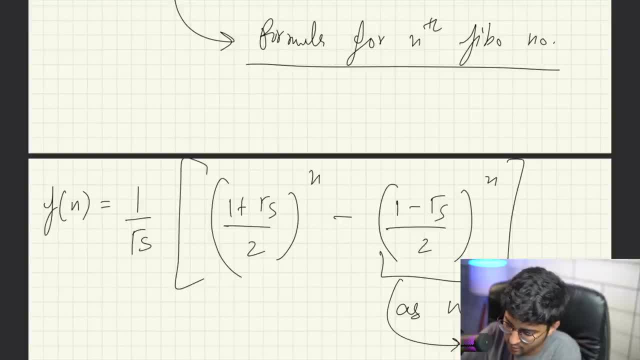 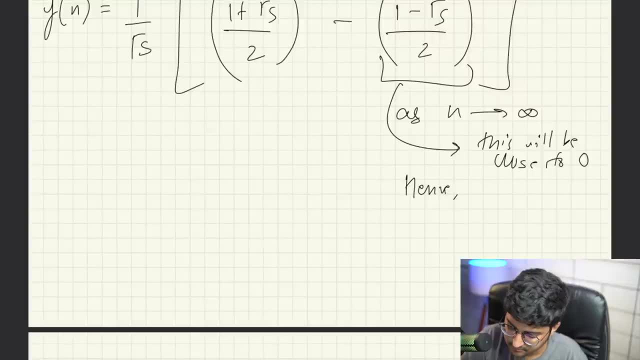 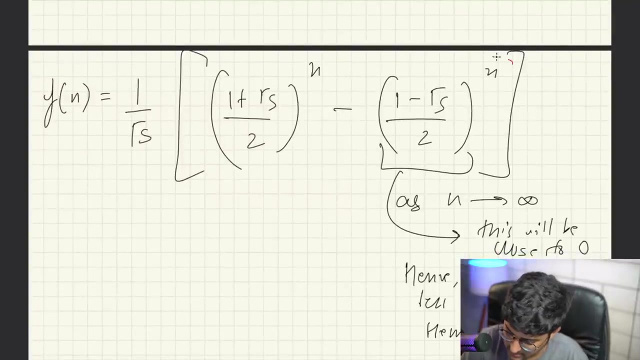 this will be close to 0. and what do we know about time? complexity: ignore: less dominating term, hence this is less dominating term, hence ignore. so i'm just going to ignore this. when speaking of complexity, this will be ignored. constants will be ignored. complexity is equal to. 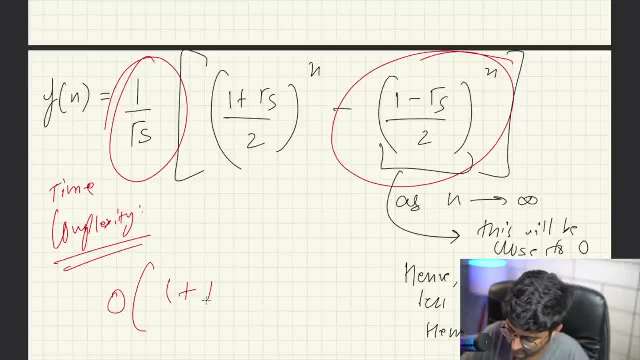 time complexity: big o of 1 plus root 5 by 2 raised to power n for nth fibonacci number answer. how cool is this? how cool is this thing? this is actually equal to what is not like when people say: you know, recursion fibonacci is 2 raise to power n exponential. that is incorrect. 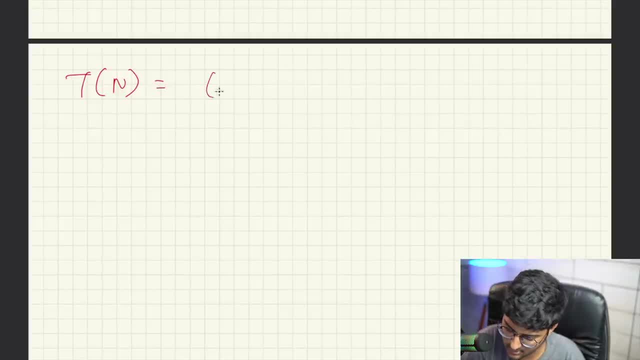 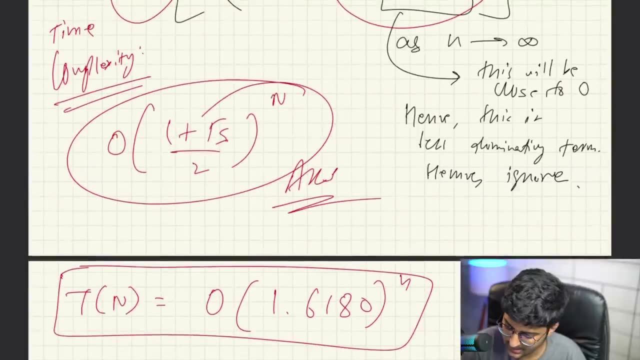 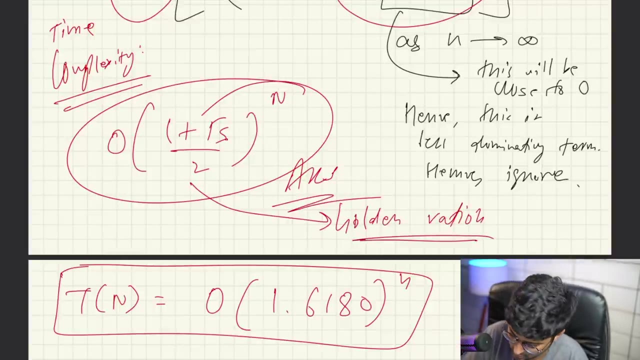 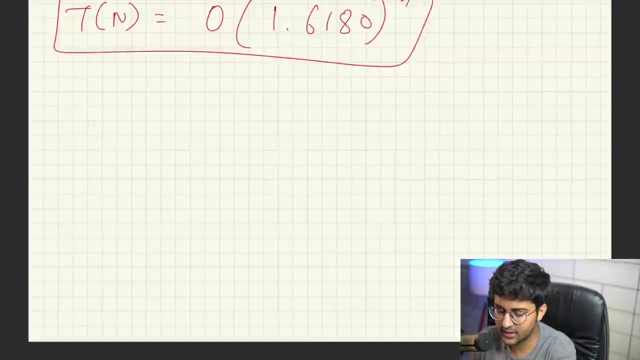 time. complexity is actually equal to foreign fibonacci number 1.6180. raise to power n. this is, i think, also known as golden ratio in mathematics. golden ratio- how cool is this? this is the reason that it was hanging, for the program was not giving answer, for n is equal to 50 or something, even for such small numbers, because exponential 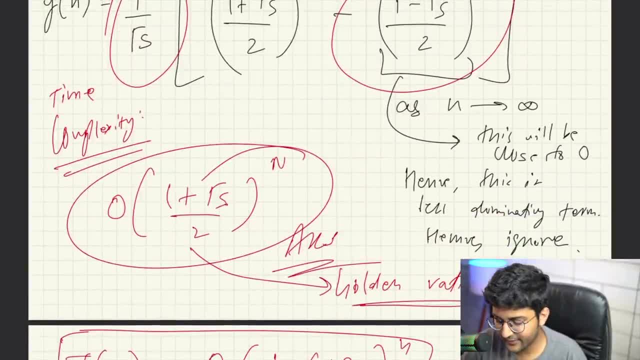 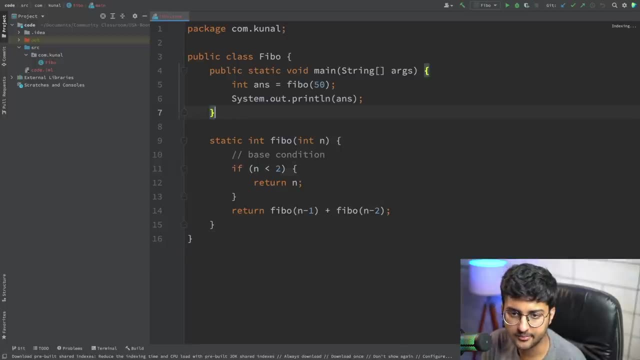 time. complexity is very bad. all right, what if i try to write this program for this nth fibonacci number for uh one plus root five by two, raised to power n? let's try that. okay, so i can say something like um static int fibo formula for a number n. all right, yes, uh, fibo. 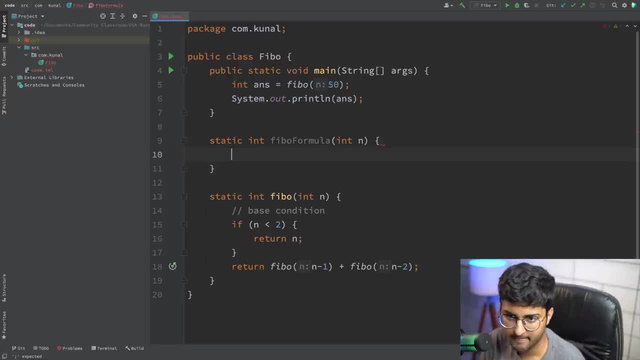 formula right, okay, so one plus uh answer is going to be equal to? what answer is going to be equal to one plus math dot, square root of one plus root five by two raised to power n. so i can say something like 5 whole divided by 2. 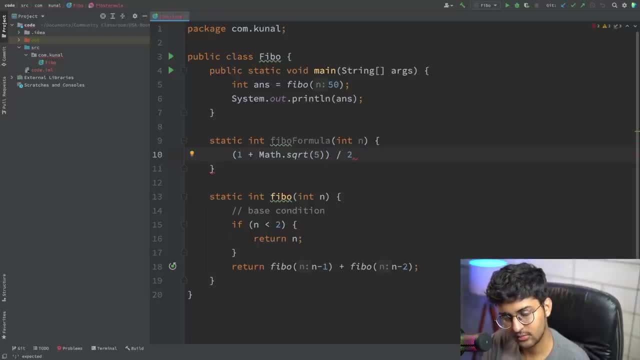 whole divided by 2 and whole raised to the power n, this whole raised to the power n, so i can see math dot power of this whole thing, one second, this whole thing raised to the power n, and i can cast this into an integer if i want no problem. please don't do it though like try to use. 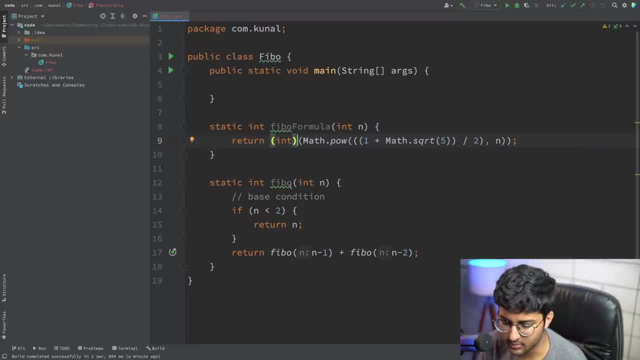 double or whatever. but okay, but this is not complete, like the entire formula is. let's say this is a time complexity formula. we want the actual number and we can't ignore the constants and anything. so actual one was, uh, root 1 upon root 5 was outside. so 1 upon root 5 is going to. 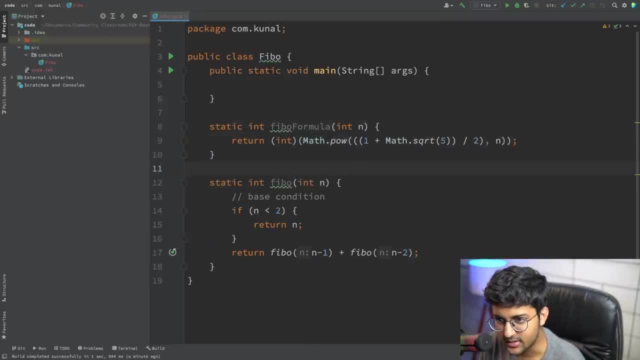 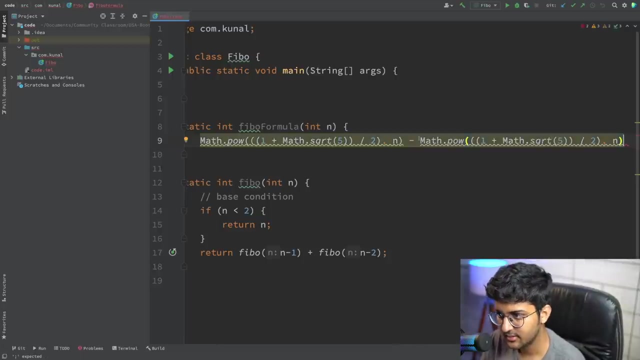 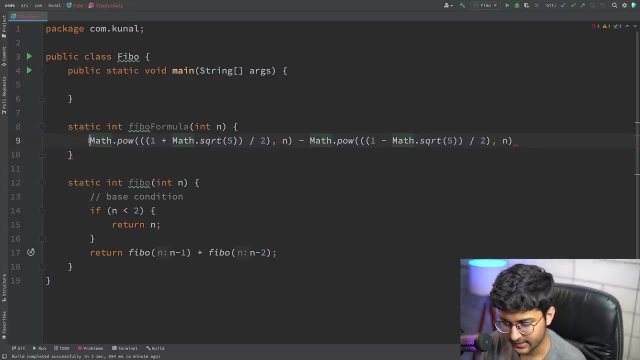 be looking very dirty, but it's going to be nice. so this is what this, actually this itself is. let me just remove this thing right now. this entire thing is 1 plus root, 5 by 2 raised to power n. i can say minus 1, minus this thing that looks good, and i can say this whole. 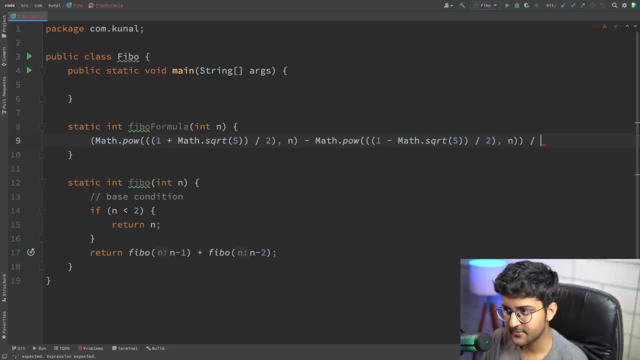 divide by math dot square root of 5 make sense. this entire thing is my answer. okay, now i can say sorry. i can say yeah, this entire thing is my answer. whole divided by root 5, that's it, yeah, and with this and this entire thing is my answer, i can just say: cast it into integer. for starters. 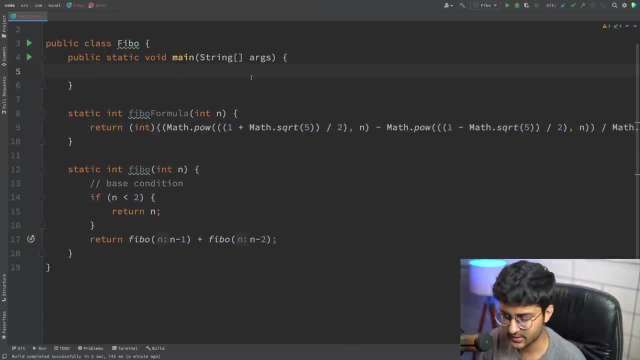 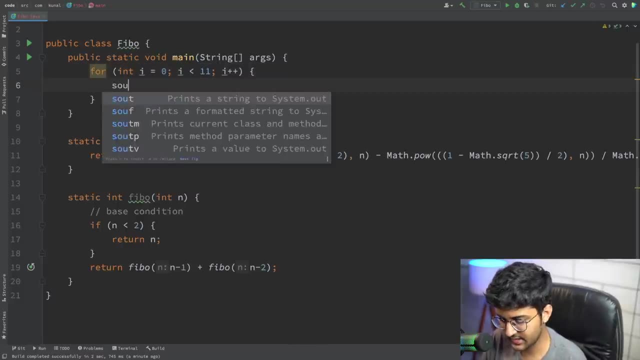 okay on it. okay. so now let's try to run this so i can say: 4i is equal to 0, i is less than let's say first of all. let's say 11 or something. there's the first 10 numbers. i can say: print the fibo. 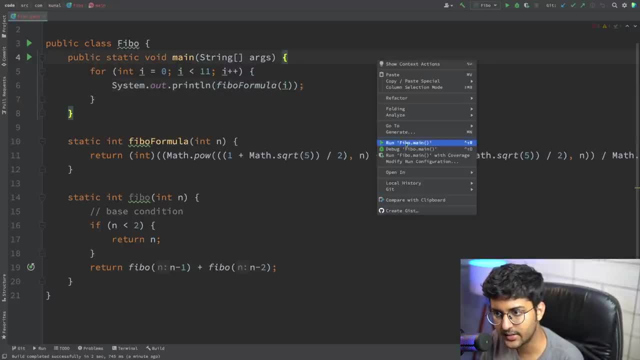 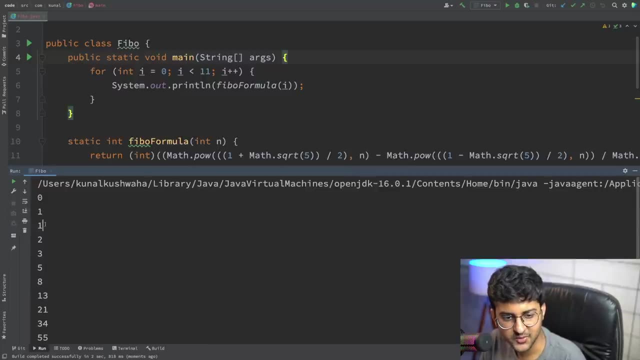 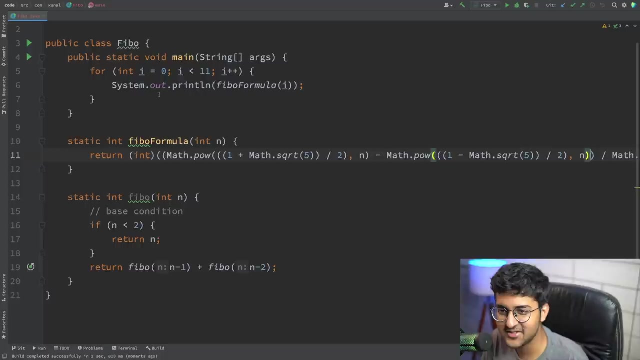 formula. answer of i see what we get pretty cool stuff: one zero, one, one, two, three, five, eight, 13, 21, 34, 55, yay, very nice stuff. so you can say, with just one single line of formula, let me make it much more easier for you. you don't need this thing, because this is uh, this is like less. 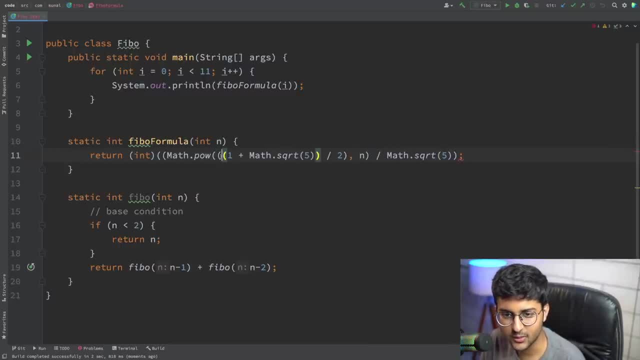 dominating term, so remove it. we don't need this. you can totally remove it. you can totally remove this thing. i can now remove this thing. this is also going to do the same thing, because that second one was less dominating term, so you can remove that same thing. now let's try what we were trying previously. 50th 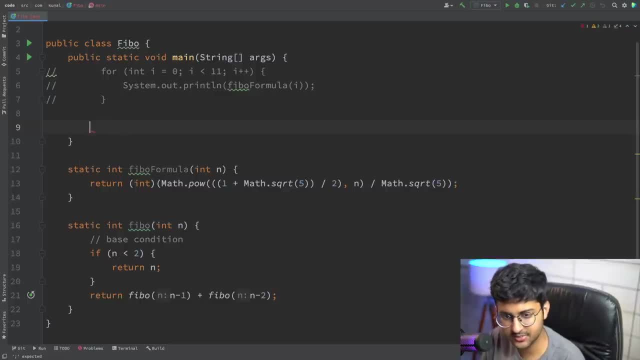 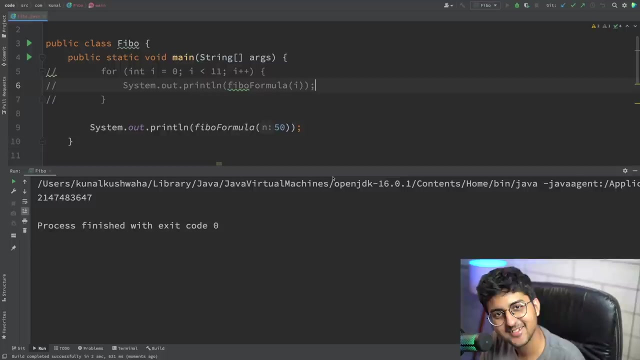 fibonacci number. it was not giving us the answer for 50th fibonacci number, right, let's try that. i can say fibo formula: 50th fibonacci number run very nice. so, even though the int range will exceed, try to use long or something. try to use long instead of. 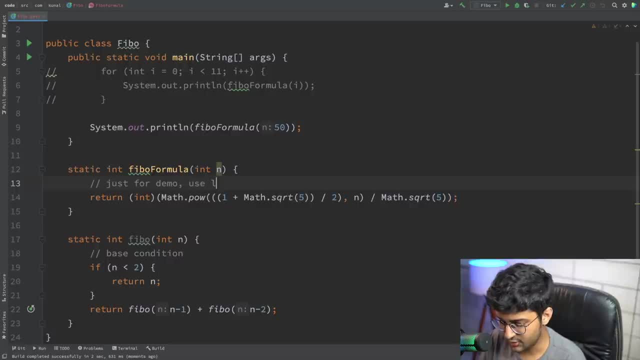 this just for demo. use long instead. how cool is this? with just one single line, you're able to get the answer. this is the time where you take a screenshot, subscribe like, comment right now. please comment right now. if you watched so far, if you loved it, and i, we derived the entire formula. 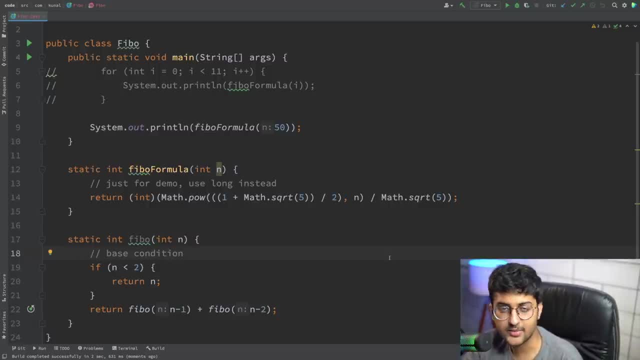 and subscribe to the channel, share with your friends. this is a really amazing thing. this akrabazi and stuff- definitely you will find it at like you know some small small videos and you can also find it on, like other international courses. like it's very like not many people know about it and all of these things. 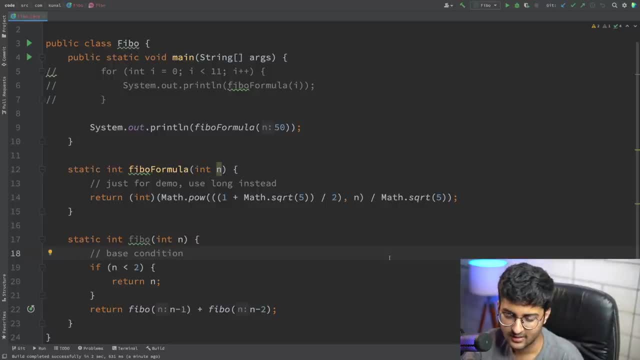 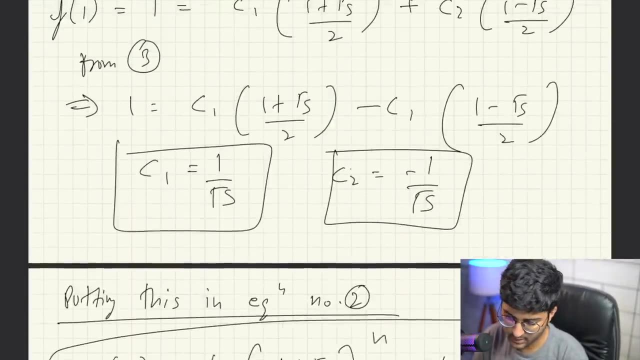 combined in one place, like a really nice course for you all. all right, so that's pretty cool stuff. um, let's, let's move forward, okay. so as a general answer, you can see like: uh, now you'll be able to solve any question in like recurrence relations and stuff. uh, for divide and conquer. so if i say 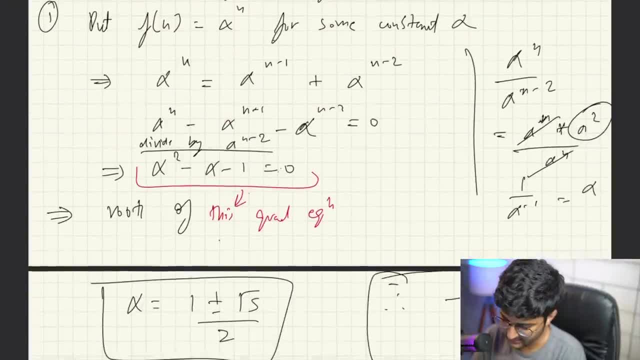 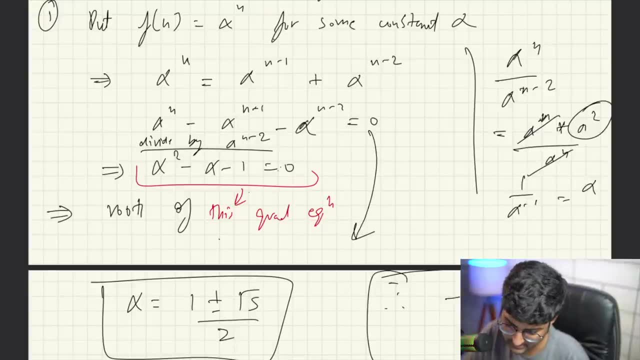 something like this one. you know, just take, uh, take alpha, raise to n. this is basically. this is known as a characteristic equation as well. so this is known as, by the way, character characteristic equation of recurrence. what is the spelling of characteristic? i think that's it: equation of recurrence. it might be. 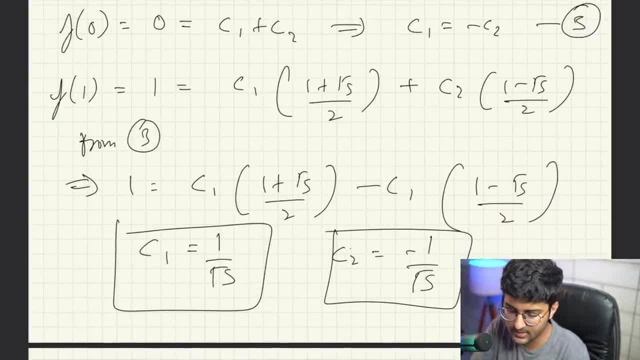 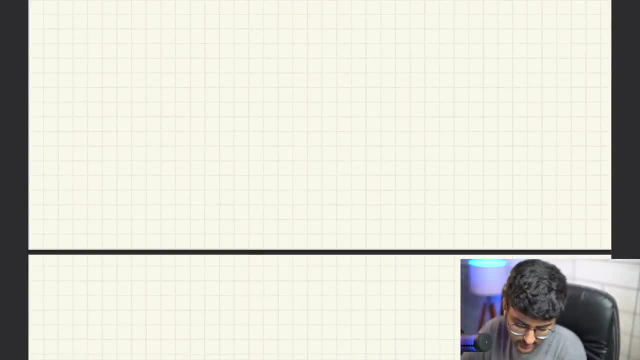 possible that sometimes you will get like equal number of roots. okay, that might be possible at well, let's try to see how we can resolve that. so when you get equal number of roots, so you will get question, let's say something like equal roots, you're getting right. so let's say you have a question like f of n is equal to 2. 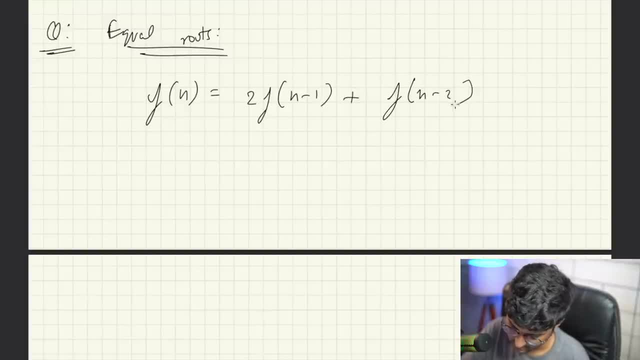 f of n minus 1 plus f of n minus 2. here you say put: f is equal to what is step number 1. f of n is equal to alpha raise to power n. this will be alpha raise to power. so this will be alpha raise to power. n is equal to 2 alpha raise to power n minus 1 plus. 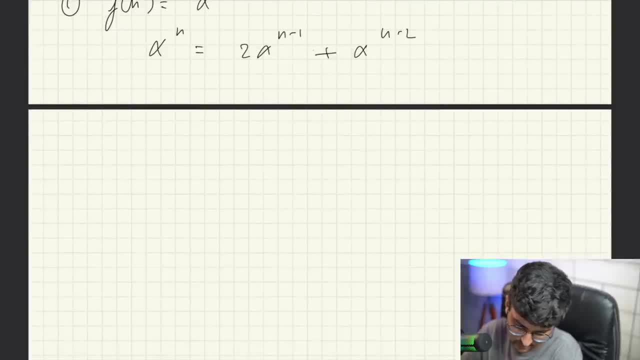 alpha raise to power n minus 2, this will be equal to what. this will be equal to: alpha raise to power n minus 2. alpha raise to power n minus 1 minus alpha raise to power n minus 2 is equal to 0 divide by alpha raise to power n minus 2. 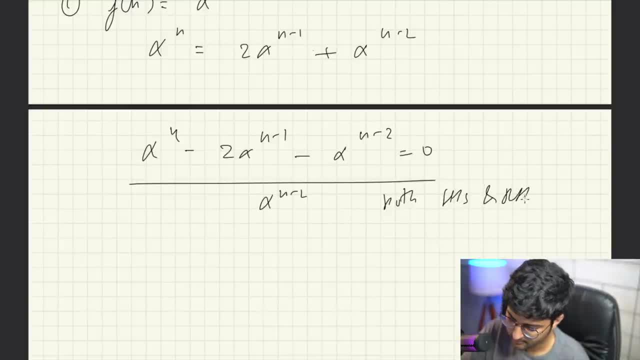 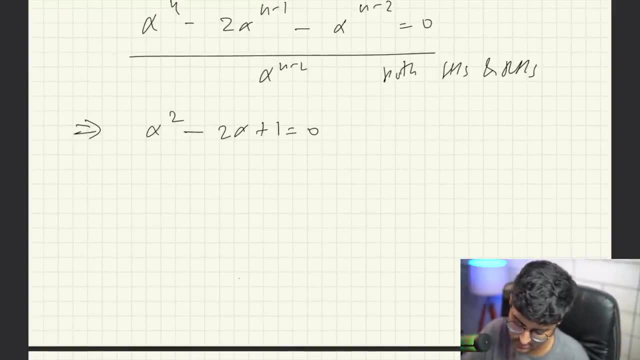 both lhs and rhs. this will give me, uh what? this will give me something like this: alpha square minus 2, alpha plus 1 is equal to 0. so very simple stuff. here i can say: alpha is equal to 1. no double root, it's a double root, double root okay. 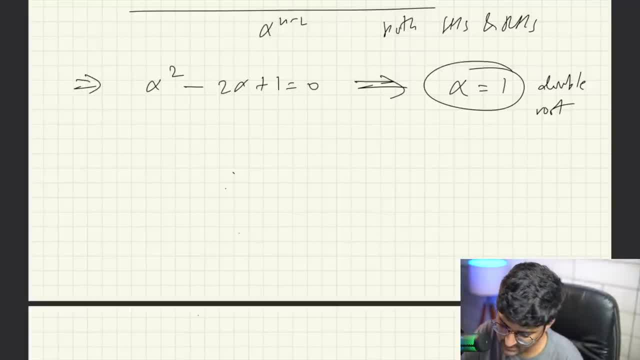 in such case, what will happen is that if this root is repeated twice, right, but let's say in a general case, in a general case, it's a very simple stuff. if alpha is repeated, let's say r times, then alpha raise to power n n. alpha raise to power n n. square alpha is to power n till. 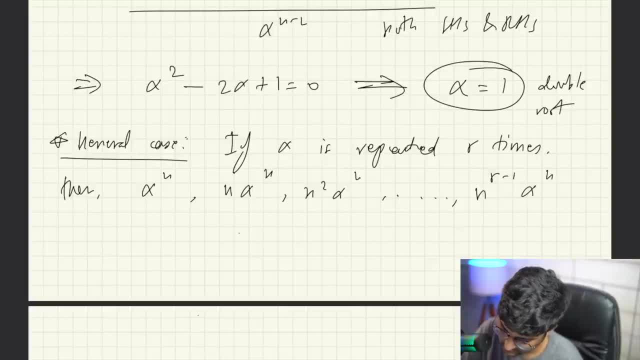 n? r minus 1 alpha i? n are all solutions to the recurrence. okay, to the recurrence. so we know that if the number of roots are 2, i know that there should be two roots, but i'm only getting one root. i can take extra roots from here, because these are also solutions. these are also. 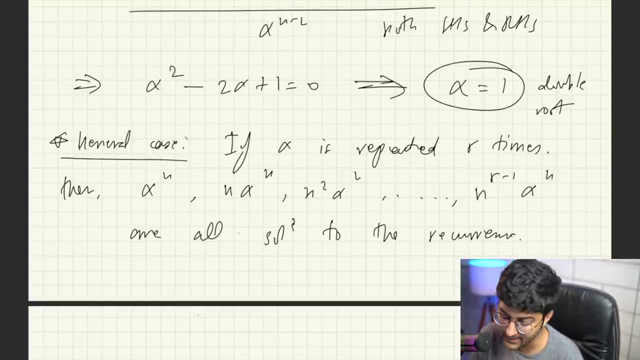 solutions, because i'm just multiplying some number over here, right, like the n over here. okay, so you know that n divides n, right? that's, that's the thing over here, that's the only that's the case, basic stuff. so i'm saying if a root is like you know. so basically the idea is that over here, 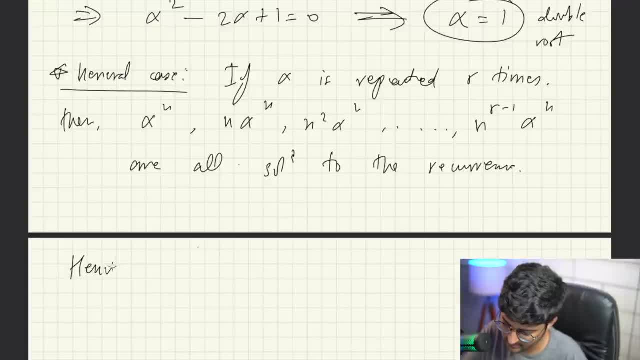 if you take two roots, hence i can take two roots, hence i can take two roots, as one is one itself. second one can be what n, n into alpha, raised to power n, something like that. okay, we know that alpha is equal to 1, so it can be equal to. 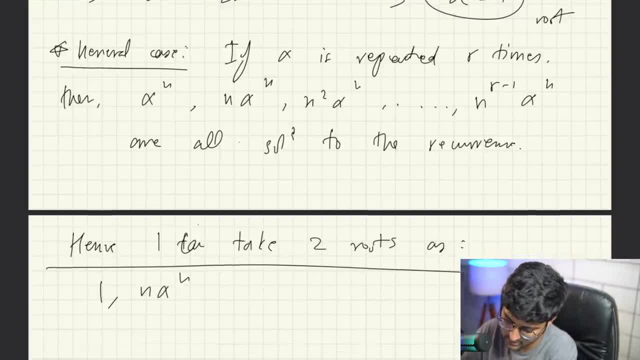 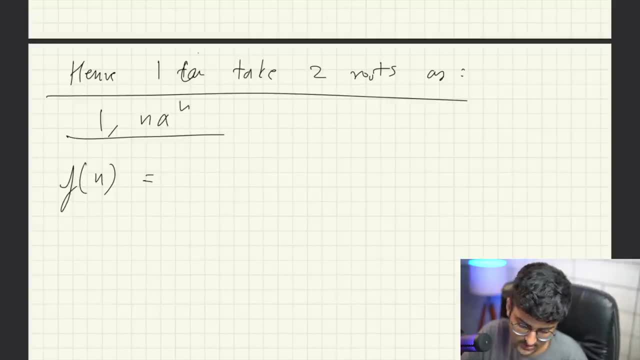 1 comma n, something like that. let's try to put it in formula before jumping to conclusions. so we put into a formula i can say f of n. putting in formula i can say f of n is equal to c 1, 1 raised to power n plus c, 2, second root and alpha n. so alpha raised to power n plus c, 2, n alpha. 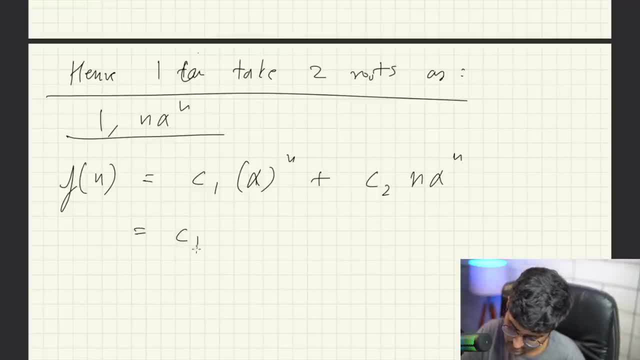 raised to power n, something like that. this is equal to c 1 plus c 2 n, something like that. let's say the answer is given to you is f of 0 is equal to 0 and f of 1 is equal to 1, so i can say f of 0. 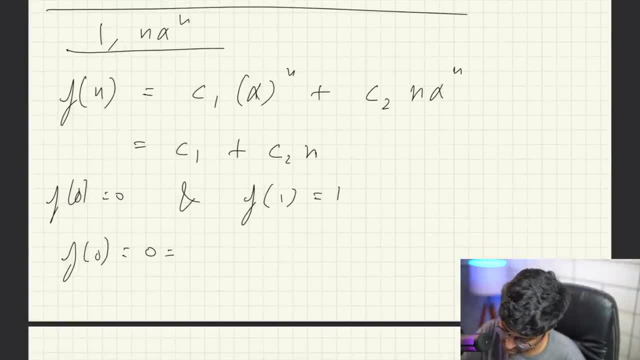 is equal to 0 means what? it means that this n is a 0. put over here c 1, c, 1 is equal to 0. that's the first question, first equation. second one is basically saying: f of 1 is equal to 1, f of 1 is equal to 1. 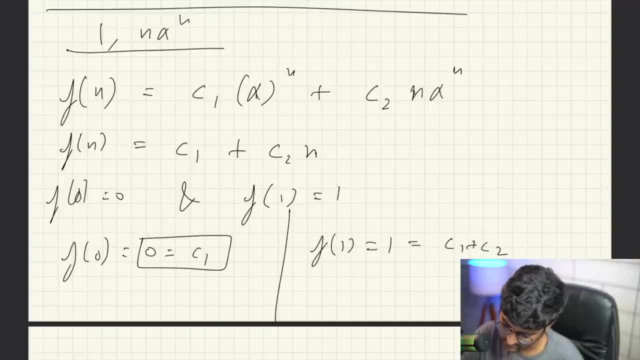 means c 1 plus c 2, because this is 1. this is c 1 itself. i know c 1 is equal to 0, c 2 is equal to 1, very simple mathematics. so if i put c 2 as 1 and c 1 as 0, i can get my answer, as f of n is equal to n. 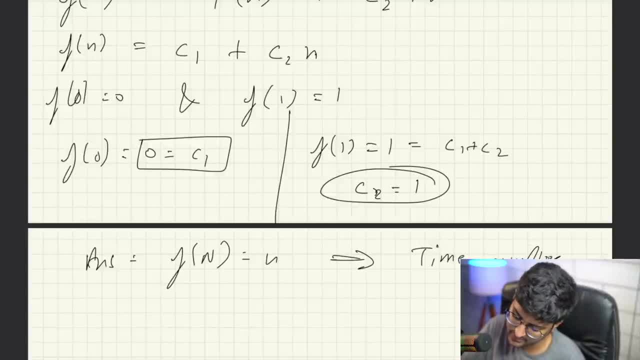 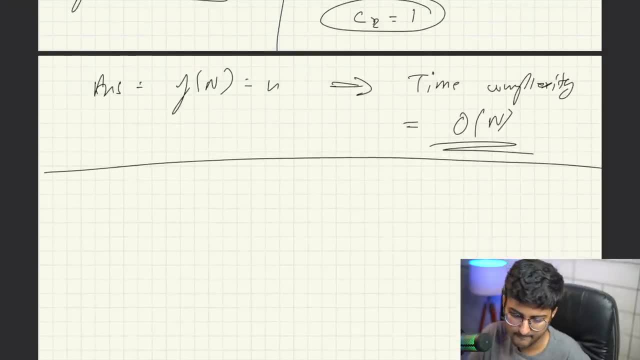 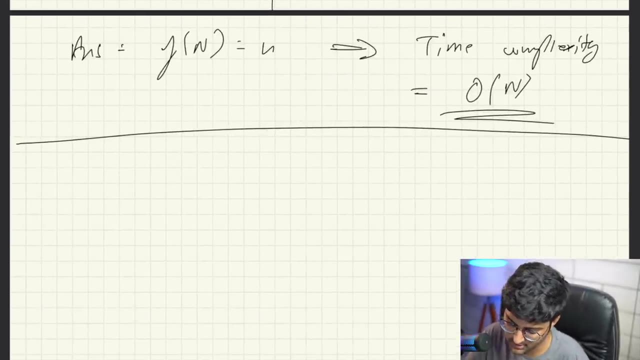 i can say time complexity of the above relation is equal to what we go often. that's it very cool stuff. okay, that's how you can solve any particular in: uh, homogeneous, oh sorry, homogeneous, linear recurrence. homogeneous is the first time i've mentioned it. what do you mean by homogeneous? 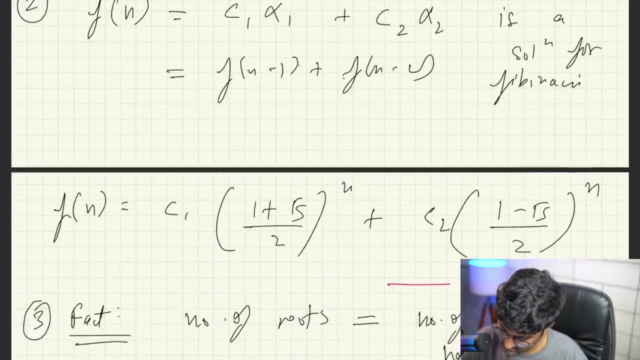 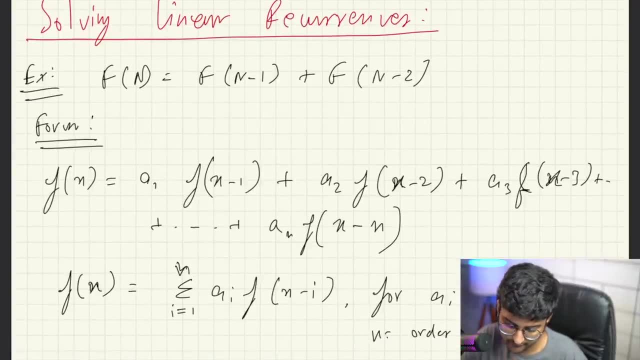 so by homogeneous i mean something like this: this is what i mean by homogeneous. so this is like the, the form of- uh, recurrence relations. right here you do not have a particular other function like g of x that we were having previously. there's no separate function over here like g of x. that is why this is homogeneous. 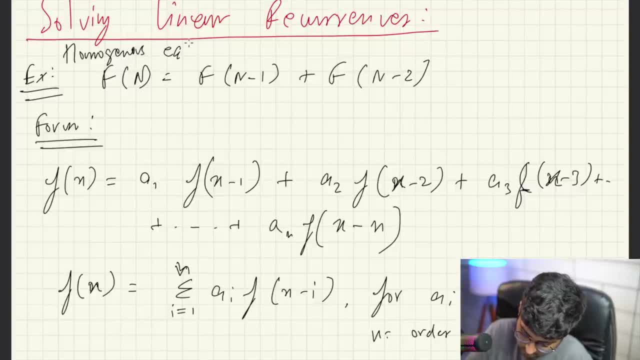 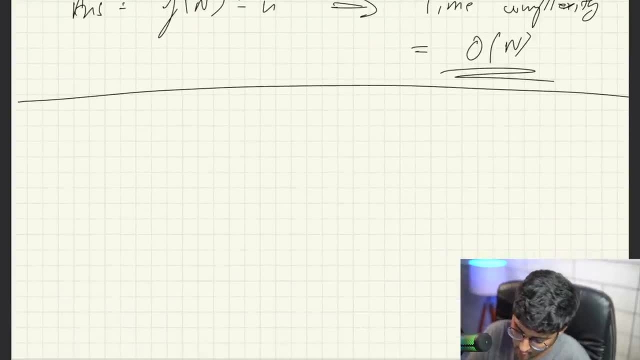 homo genus equations. what are non-homogeneous? let's see, non-homogeneous are also same thing. now i can say non-homogeneous linear recurrences, non-homogeneous recurrent linear recurrences. so i can say that the previous one, i can say f of n. 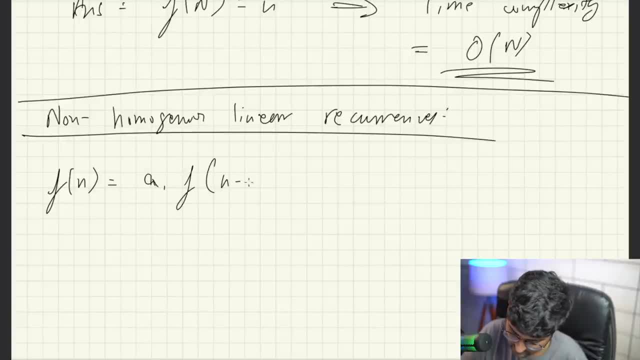 is equal to a 1 f of n minus 1 plus a 2 f of n minus 2. similarly, the same thing we were doing previously: f of n minus 3 or whatever right. plus plus, plus, plus, plus, plus, uh, plus plus plus. over here it's going to go till plus plus plus a of uh. let's say, i take some other d or whatever, just the. 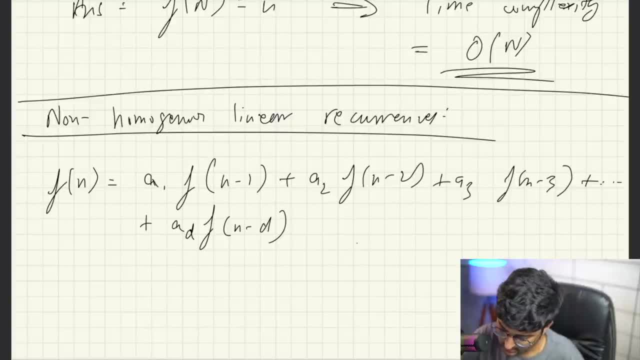 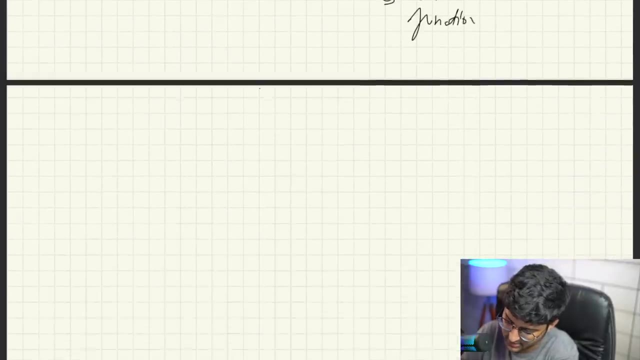 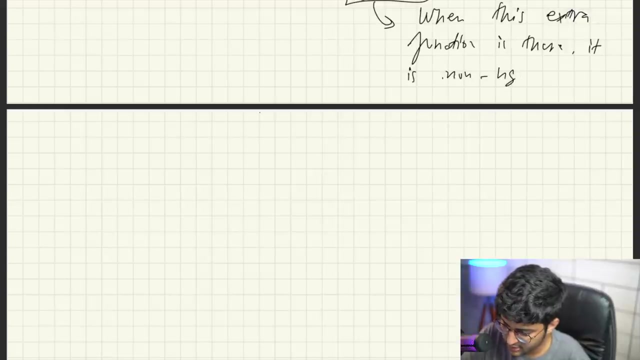 names are changing, everything is same: f of n minus d plus g of x. so when you have this extra, when this extra function is there, when this extra function is there, it is non homogeneous linear recurrence. all right, how do we solve this? it's very simple. it's going to use the previous approach only. step number one: replace g of n. 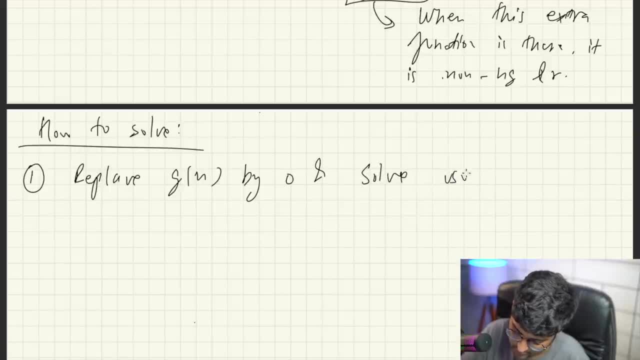 by 0 and solve usually like you usually solve okay. so if i'm given something like let's say f of n is equal to 4, f of n minus 1, plus let's say 3, raise to power n, okay, and you're given an answer. 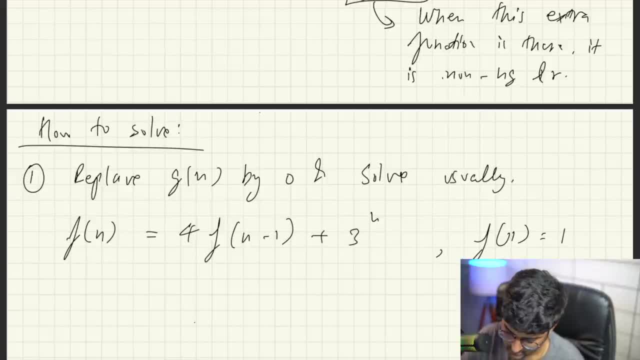 like f of 1 is equal to 1.. it's the answer you're going to get. if you're going to solve it, then you're given. so i'm just going to say, okay, uh, put this equal to zero. so i put this equal to zero. this. 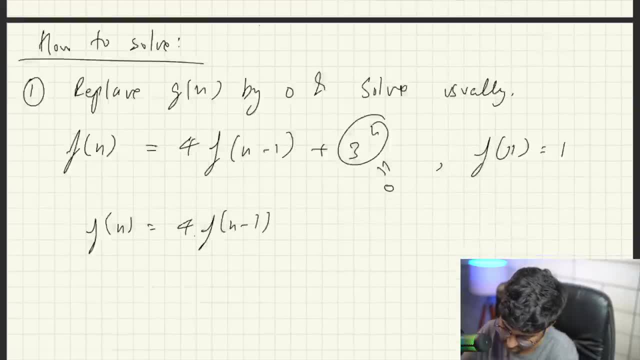 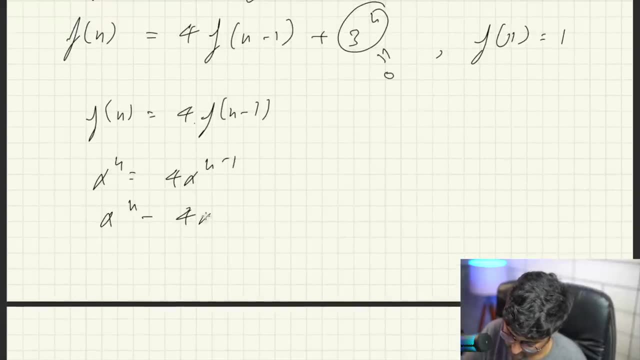 will now be: f of n is equal to 4, f of n minus 1. alpha raised to power n is equal to 4. alpha raised to power n minus 1. i can say: alpha raised to power n minus 4. alpha raised to power n minus 1 is equal. 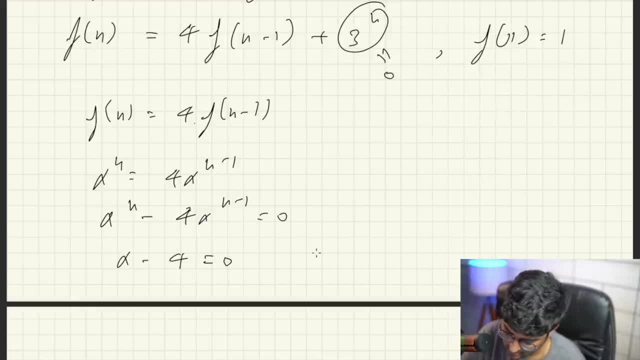 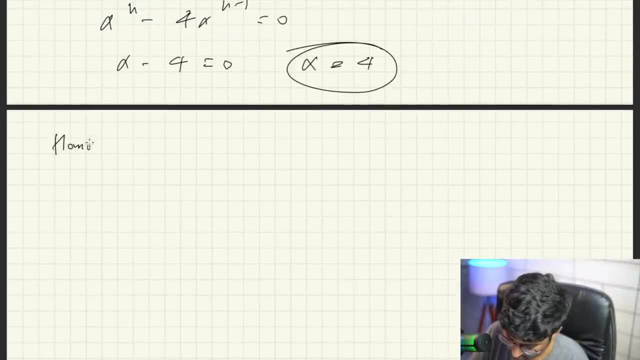 to 0. this becomes alpha. minus 4 is equal to 0, alpha is equal to 4.. very simple stuff, okay. homogeneous solution is going to be what homogeneous solution? like we did previously? similarly, it's going to be like something i can say: f of n is equal to c1. alpha raised to power. n means 4 raised to power. 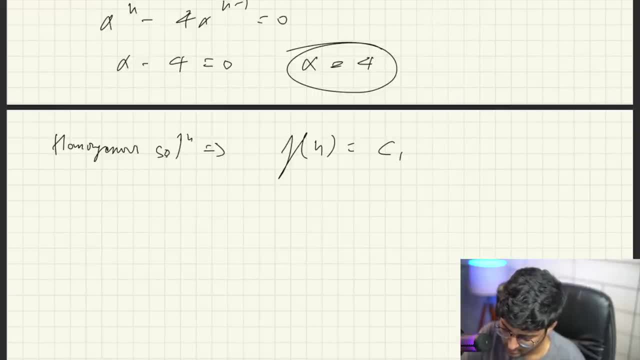 n. i can just write it completely also, no problem. if i raise to power n, this is going to be equal to f of n is equal to c1, 4 raised to power n. okay, so step number two, that's like the homogeneous solution. this is what we have over here, homogeneous solution. 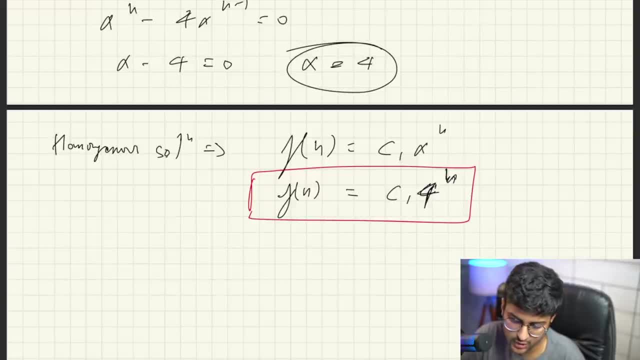 okay, step number two is find particular solution of uh. so basically, step number two is: take g of n on one side and find: but so right now, till here, till this red box, nothing is new. i put this as 0, so this particular equation is only now equal to the one that we have solving previously. 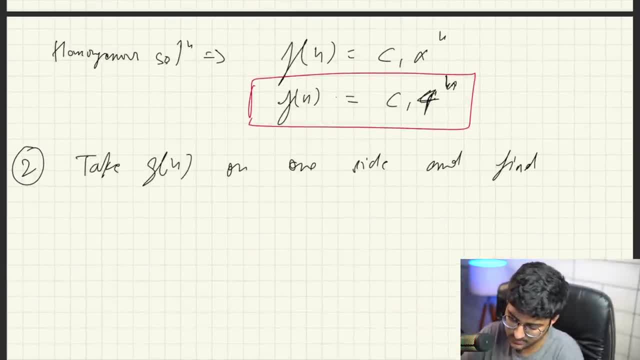 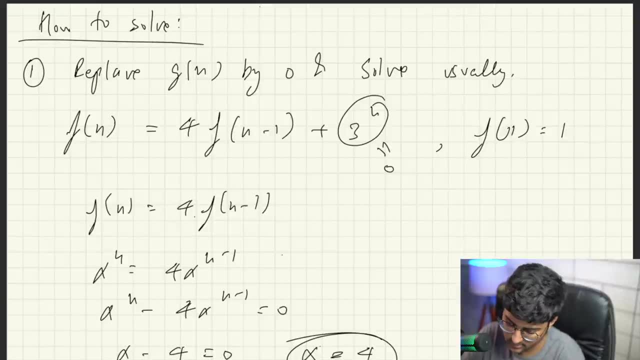 that is why i don't not have to explain anything. but now i will explain, because the previous one is like just, we have already solved this is a homogeneous equation. we already know how to solve it. just put: alpha is equal to uh. so just put: f of n is equal to alpha. raise to power n. but now 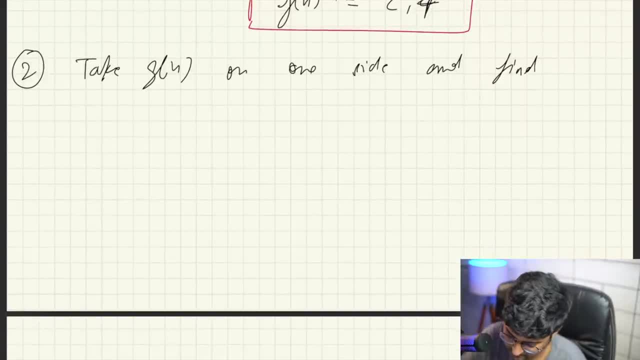 put g of n on one side and find particular solutions. you can do that, no worries. let's try to see how we are solving it. putting g of n on one side means three years to power n on one side. so i can say it's going to be equal to f of n minus 4 f of n-1. 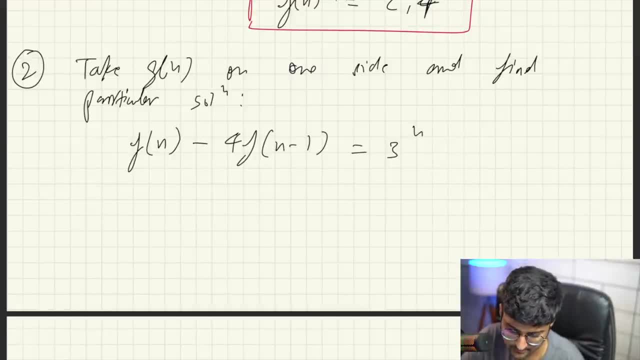 is equal to 3. raise to power n. i put this on the other side. what do we need to do? we need to guess something that is similar to g of n. this is known as particular solution. i will also teach you how to guess this general. you know this particular solution, so i'll write this in red: guess, i will. 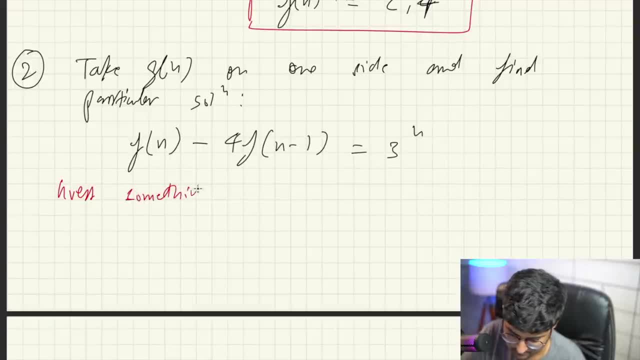 teach you how to guess. okay, guess something that is similar to g of n. okay, for example here: if g of n- let's say, for example, g of n- is equal to n square, then guess a polynomial of degree two. you can guess anything if you want. so i can guess something like: uh, you know? 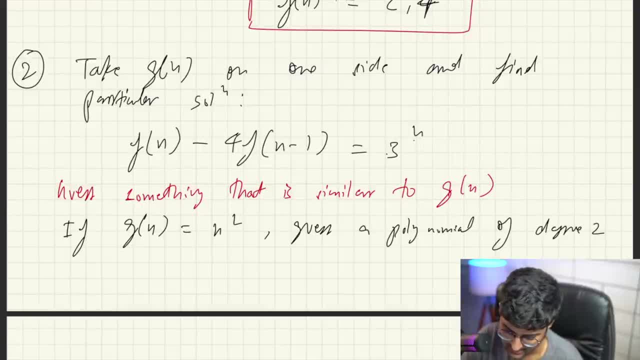 uh, for this particular case, if it's three days to power n, i can guess something like my guess. i will write it over here: my guess, this guess thing, guess of the particular solution. i will teach you how to guess. don't worry, i'm not taking this out of random. i. 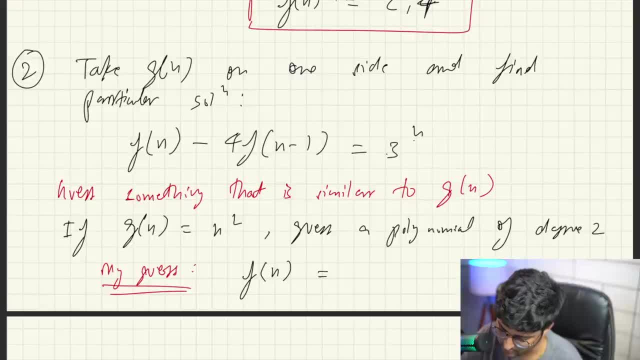 will teach you right now how to guess. let's say i'm guessing f of n is equal to. i have g. n is equal to 3 raised to power n. something similar to this can be some constant into 3 raised to power n. okay, now i just put this in this formula, put this over here, so this will become: 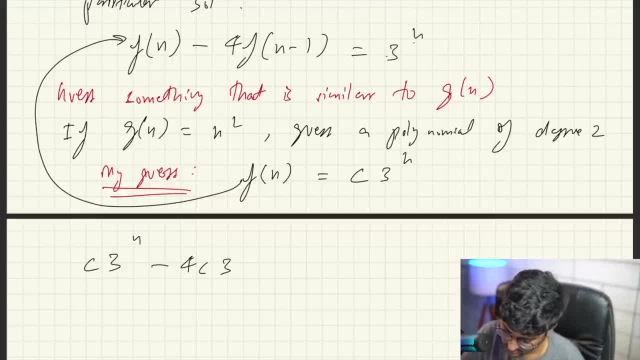 c into 3 raised to power n minus 4. 3, 4 c. 3 raised to power n minus 1 is equal to 3 raised to power n. after solving this, i get something like 3 raised to power n will be cancelled. i can get c's value. 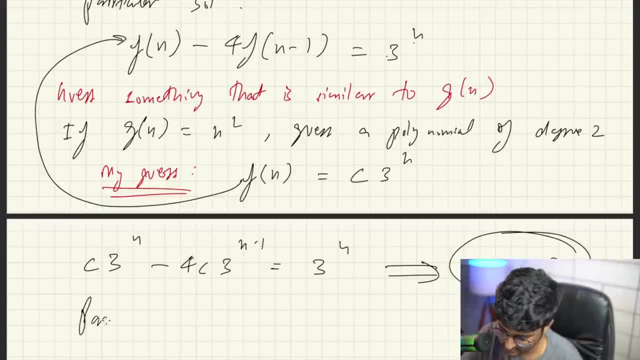 c is equal to minus 3.. so particular solution becomes what putting the value in this particular solution becomes: f of n is equal to minus 3 raised to power, n plus 1.. just put the c in this, put c in this over here. only thing i have not explained right now is how do we guess this particular function? 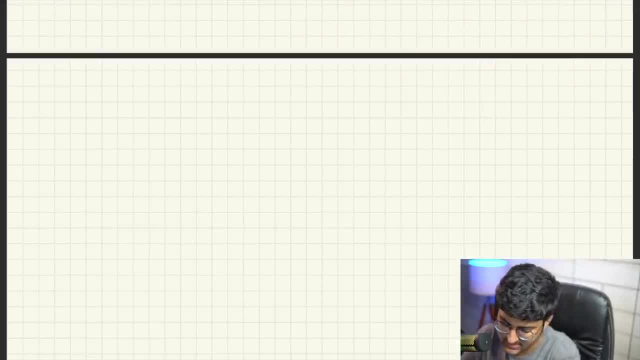 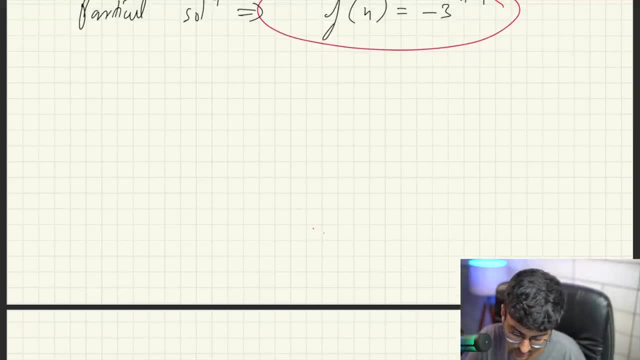 how do we guess this? i'll explain it to you later on. okay, but let's say you have your particular solution. now your no general solution is going to be: add the homogeneous and particular solutions together. next step, step number three, add both solutions together. this will be what f of n is going to be equal to what was the first one, this one, c1, 4, raised to. 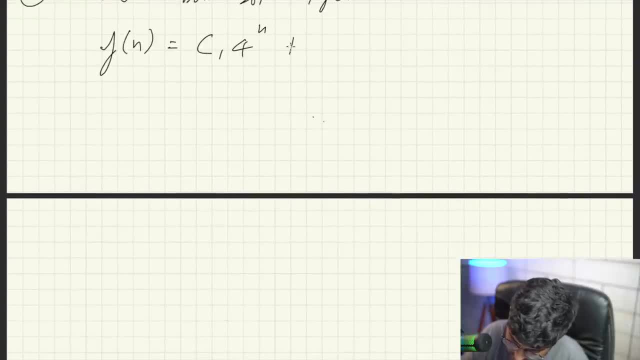 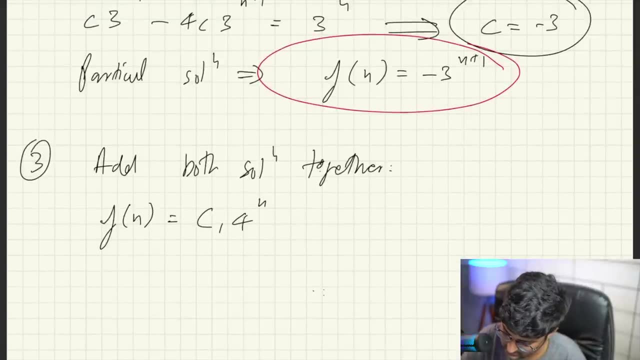 power n c1. 4 raised to power n plus. what is the second one? minus 3, uh, raised to power n minus 1. so i can just write it over here like this: minus- i can say plus, minus 3 raised to power n plus 1. 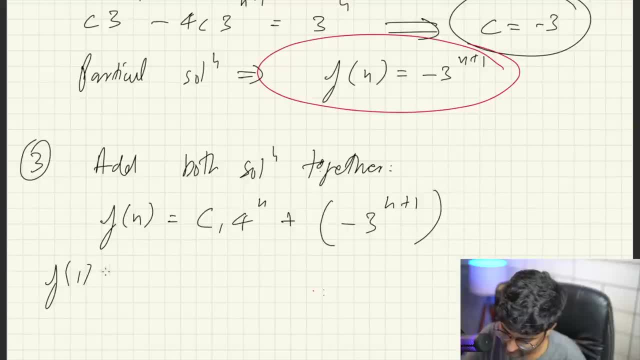 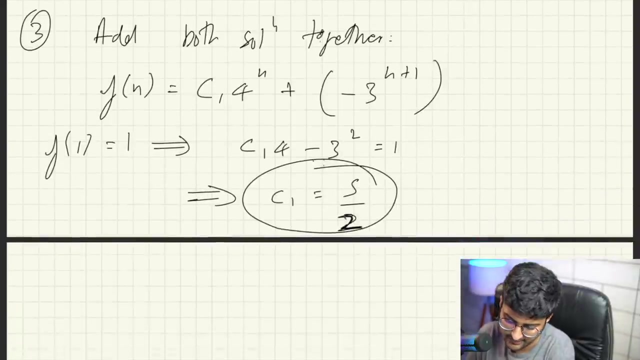 okay, i know that f of 1 is equal to 1. this basically means that this basically means that c1, 4 minus 3 square, is equal to 1. by this i know that c1 is equal to 5 by 2. if you try to solve it, you will get: c1 is equal to 5 by 2. put the value of c1 in the original. 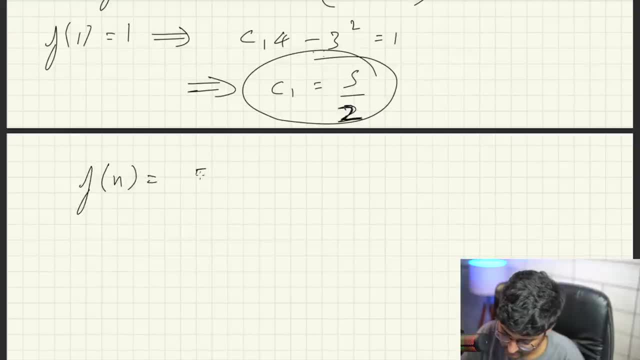 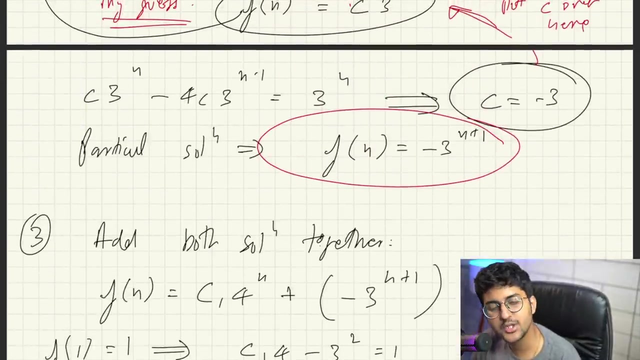 equation f of n is going to be equal to 5 by 2, 4 raised to power: n minus 3, n plus 1. answer, answer, that's it. but the only thing remaining now is how do we guess the particular solution? right, so everything is covered. we take the normal solution first. put g of n is equal to 0. take 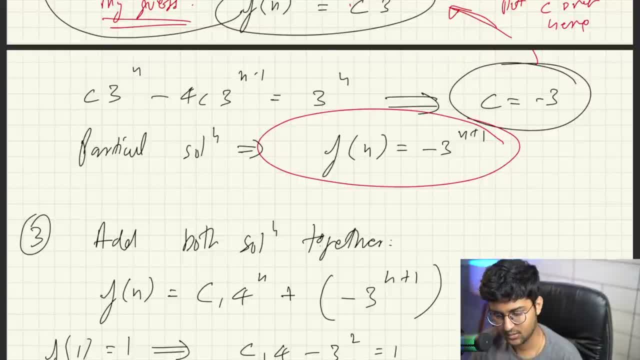 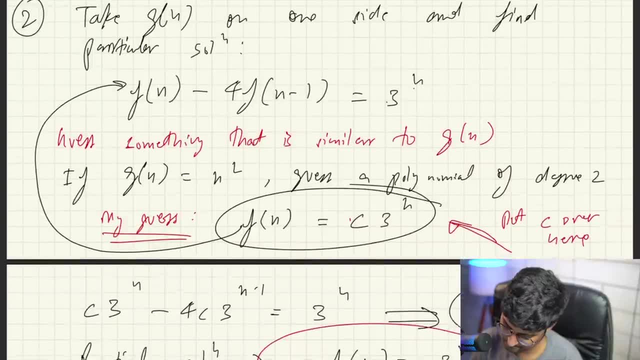 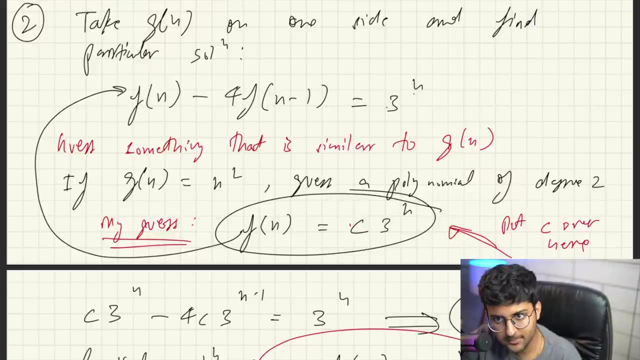 the normal solution, then guess the particular solution. okay, get the answer for that. after that, um, after you have guessed the particular solution, yeah, so basically put the g of n on one side, guess the particular solution. put that particular solution in the equation. where you have g of n on one side, you will get the value of c and then 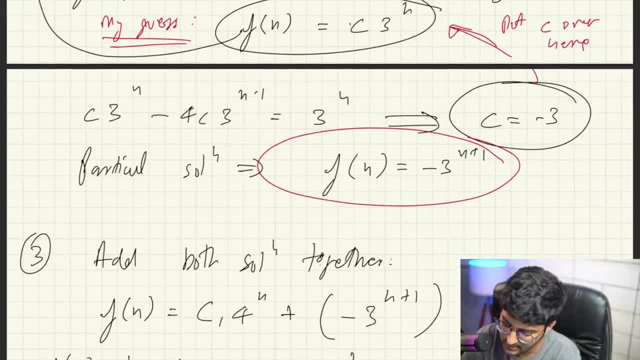 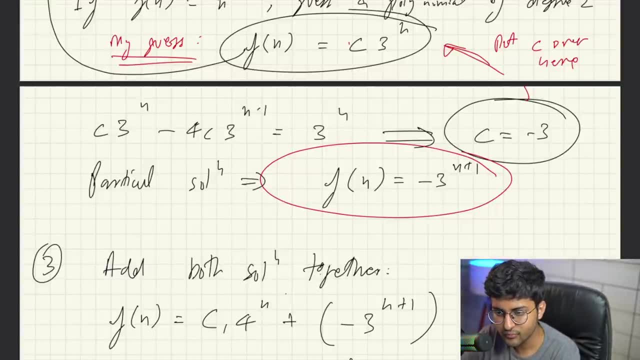 you can just do. you know your like the things we have done previously. like over here, put this over here. i got the value of c. put it in the original equation. like over here in the particular solution, got your particular solution. okay, um. so basically what i'm trying to say is: it's right in front of 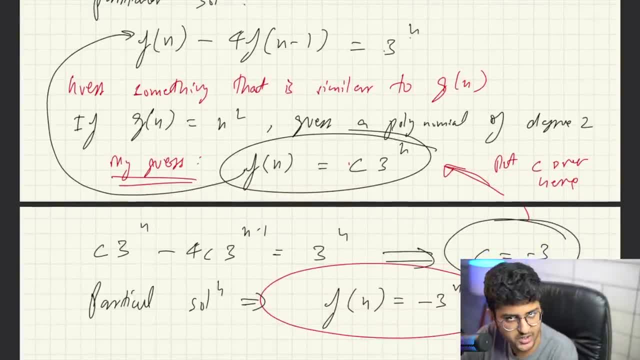 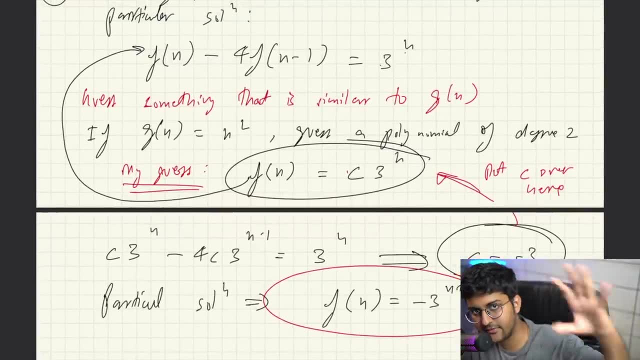 your eyes the guess that i made. i put this in the equation that i had originally and by that i got of c and then i got my final answer of the particular solution. then just add the first equation with the particular equation and put the the answer that was already provided to you. 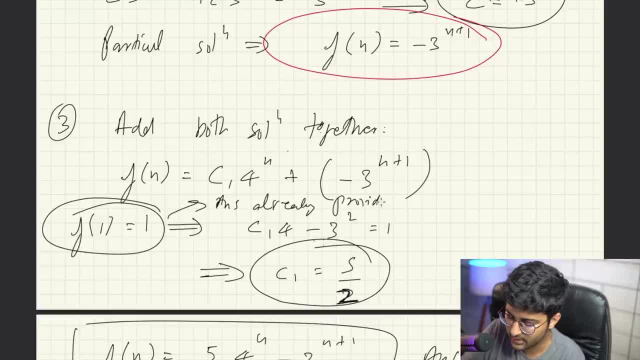 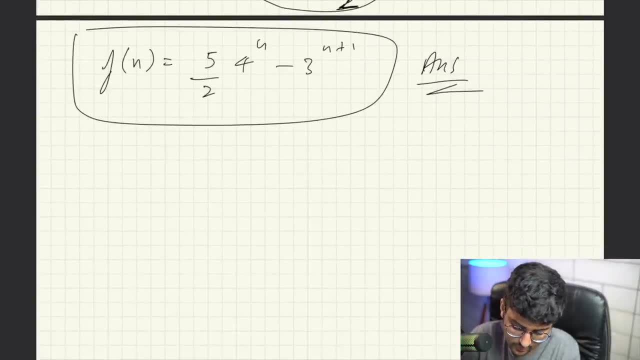 answer already provided. use that over here, then you will get your original answer, like the entire answer. only thing remaining is: how do we guess a particular solution? okay, that's a good question. write this in red color: how do we guess particular solution? how do we get this, guess, this particular solution? so, for example, i can: 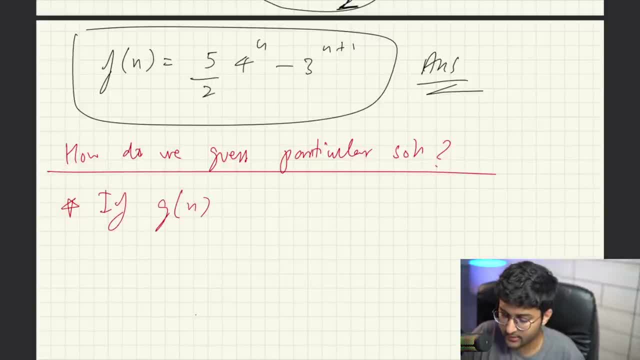 write it over here, if this is, by the way, you can find it on mit open courseware. so i had a very long lecture, that's, that's what i learned it from. so if the if g of n is exponential, so so in our case, you know. so guess of same type. 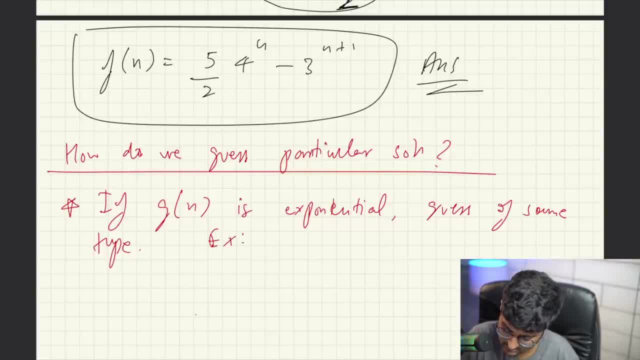 okay, guess of the same types. for example, if you have something like g of n is equal to 2 raised to power n, plus, you know, 3 raised to power n or whatever. so your guess can be something like similar to this, just add constants over here can be that f of n is: 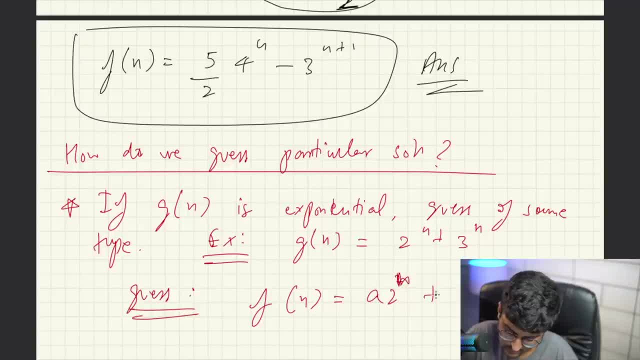 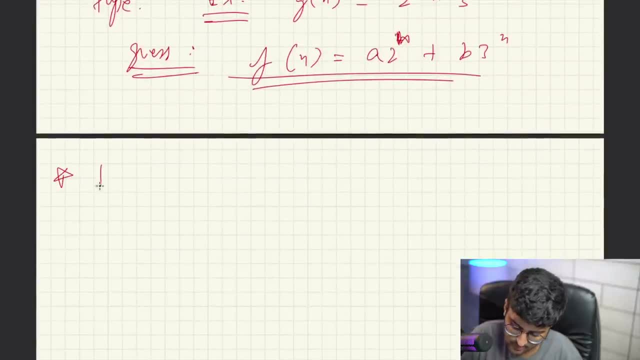 equal to a into two days to power two raised to power n, plus b into 3 raised to power n. that's it, this is your particle solution case. but if it is polynomial? if it is polynomial, g of n in g of n is polynomial. in that case, guess of same degree. 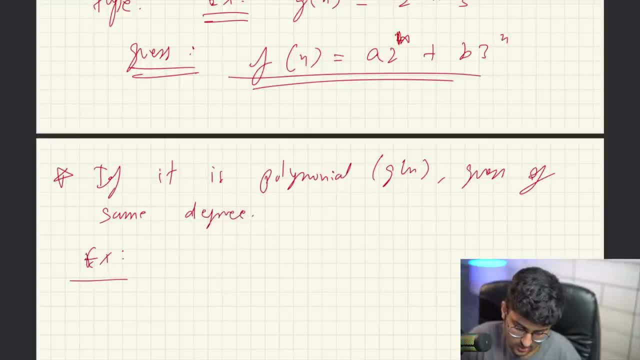 if guess, okay. so for example you have, let's say, g of n is equal to, let's say, n square minus n to the square n power plus a plus b times n squared minus a to the power of一直排ani às2 Saf a, this estable solution, but if it is polynomial, if it is polynomial, if it is polynomial g ряд of g of n, in that case guess of same degree. 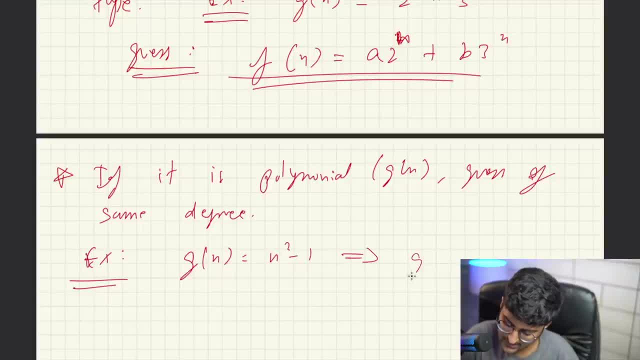 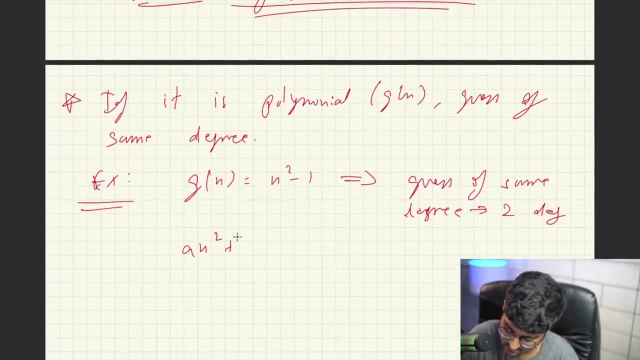 n is equal to, let's say, n square minus n. so you are going to guess of same degree, in this case 2, degree 2. what is a equation of degree 2? a, a, x square a, n square plus b, n plus c? this is my guess, okay. 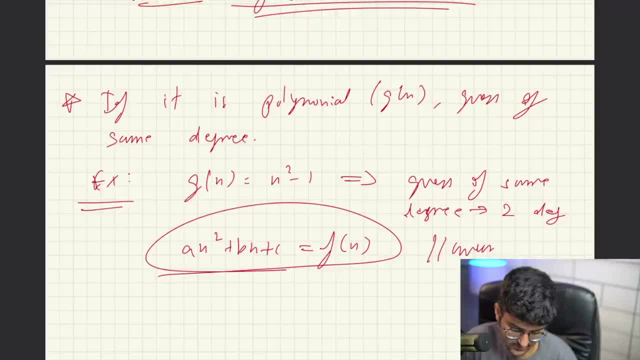 what if they? what if there is a combination? what do you have? something like, uh, you know. you have something like: let's say g of n is equal to 2 raised to power. n plus n is a polynomial also, exponential also. so you can say f of n, you can guess: f of n is equal to first for 2 raised to. 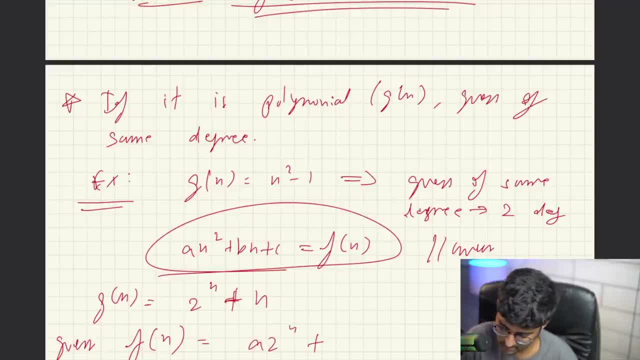 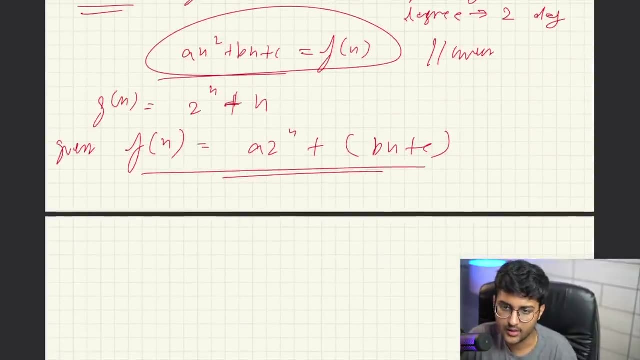 power n, it will be a into 2, raised to power n, then for the polynomial of degree 1, which is going to be a? n plus c, a n plus b or something. oh, sorry, a is already taken- b n plus c. that's it, very simple stuff. you can have combinations as well. it is an exponential. 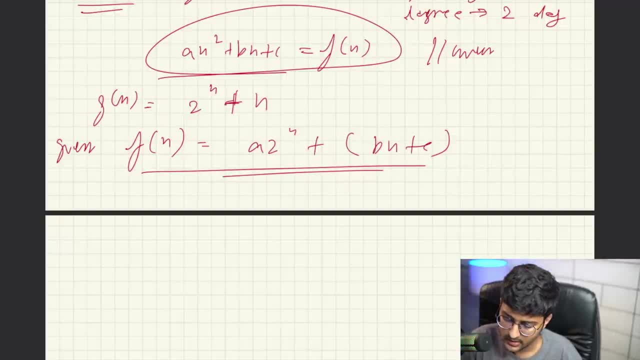 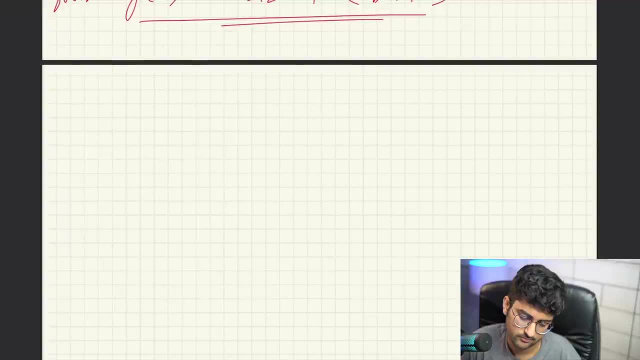 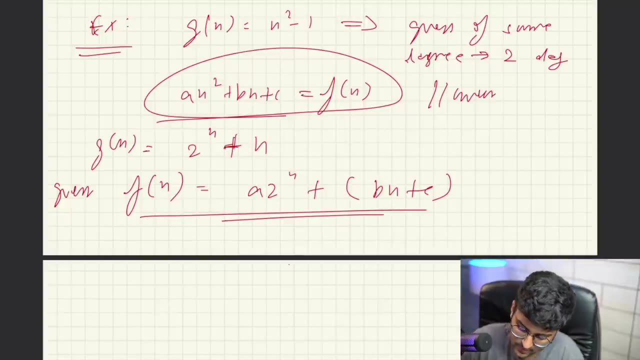 just uh, multiply the constant if it's a polynomial. take a equation of that degree, that's it. that's how you guess the particular solution. okay, cool. one more thing would happen is that let's say you guess the uh, let's say you guess the particular solution, and you guess the particular solution and you guess the particular. 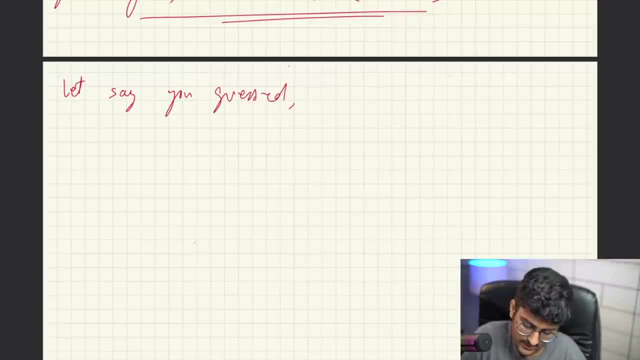 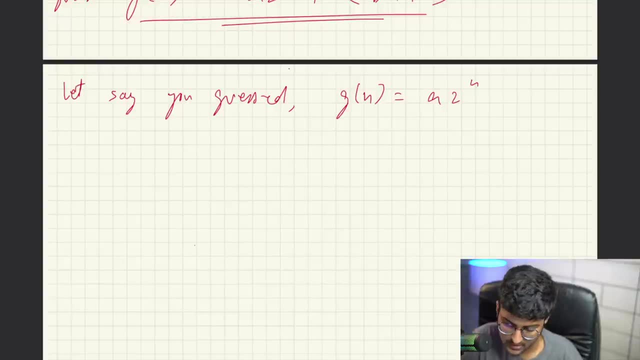 you guessed something like g of n is equal to, you know. uh, let's say a into 2, raised to power n. you guess that and it fails. sorry, f of n is equal to a into 2. responses: this is the guess that you made fails. okay, then try. 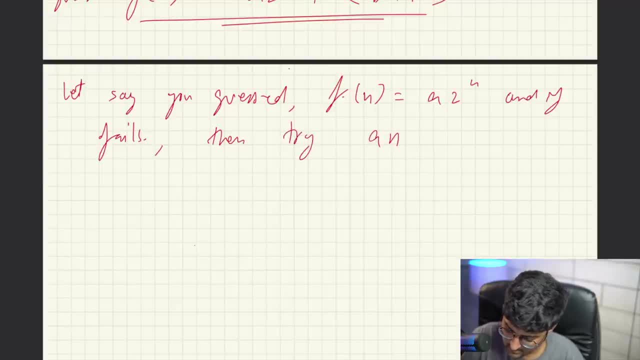 instead of a, just write a n plus b, 2 raised to power n. if this also fails again, if this also fails- ignore, sorry- increase the degree of this particular constant that you are putting like. first you had a constant, now you have like an equation. so if this also fails, increase the degree again. increase the degree this will be of. 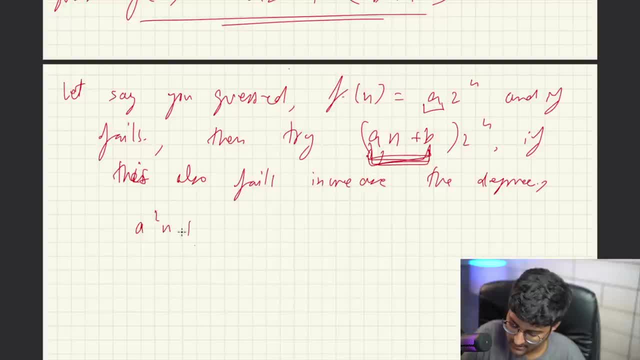 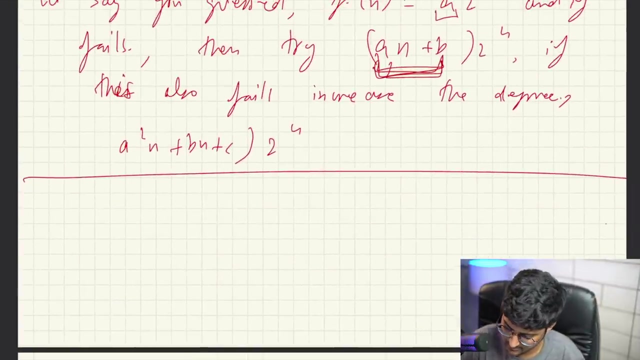 degree 2 now. so it will be a square n plus b, n plus c into 2, raised to power n. okay, keep trying that. all right, pretty cool stuff. let's do another example of this and then we can wrap things up, by the way, like: share comment very important, will really help me. so example you can take. 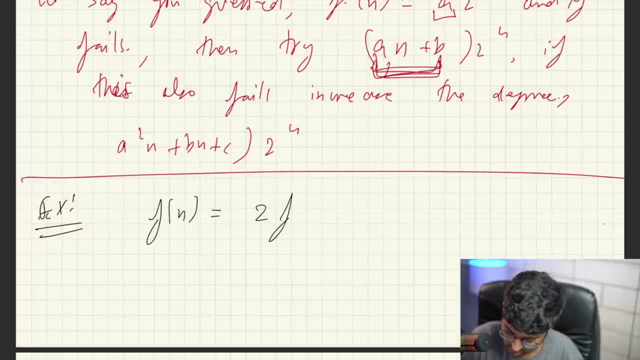 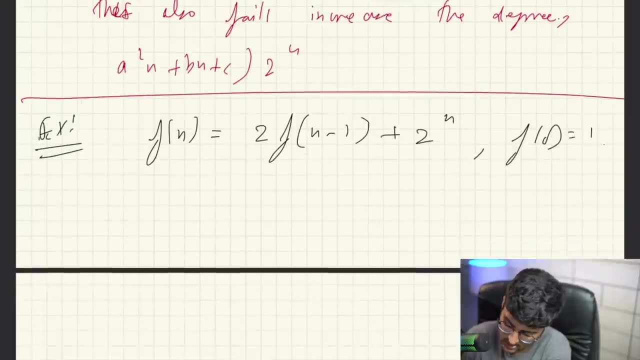 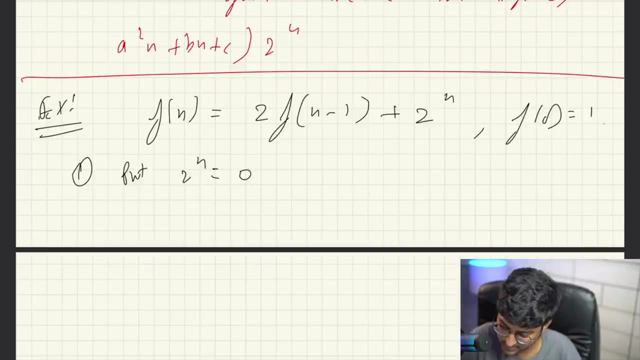 something like: let's say f of n is equal to 2, f of n minus 1, plus let's say 2 raised to power n, and we are given f of 0 is equal to 1, so homogeneous solution will be what f of n is equal to 2, f of n minus 1? i can say f of n is equal to alpha raised to power. 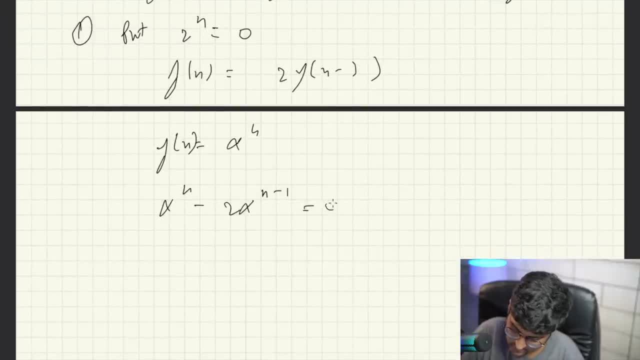